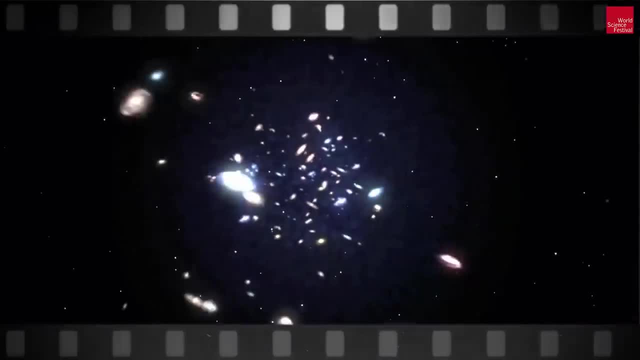 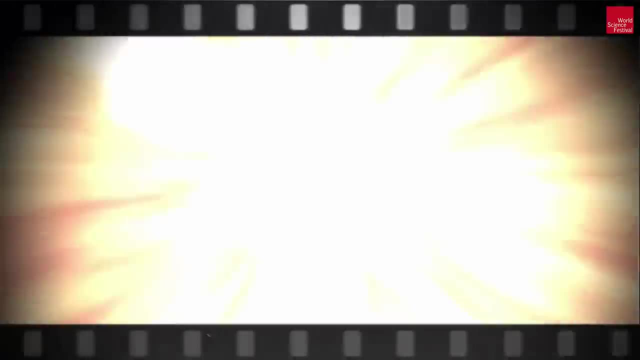 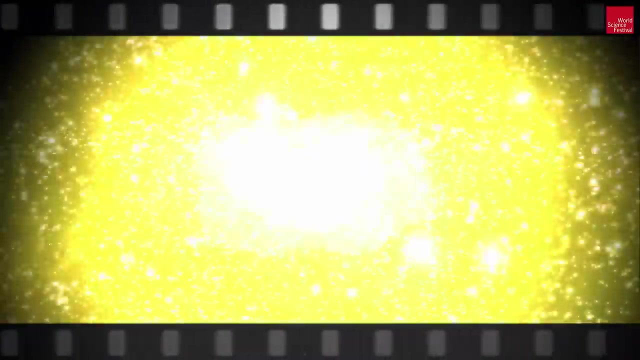 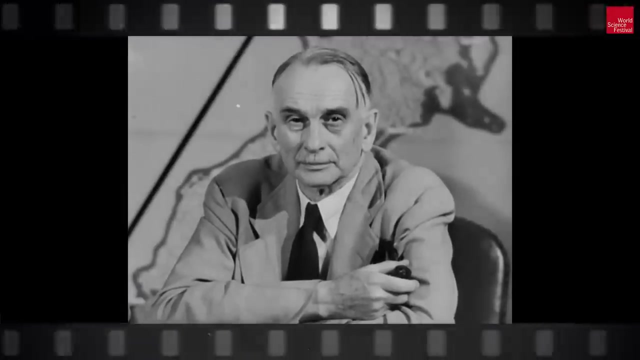 And so running the Cosmic Film Bank, suggesting a singular event from which everything emerged in a violent swelling of space: the Big Bang. The Big Bang and its further refinements has become the dominant scientific paradigm for cosmology. But in the 1940s the physicist Richard Tolman introduced the scientific possibility of a cyclic universe. 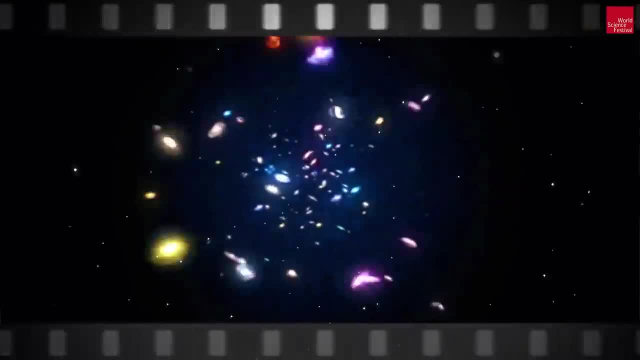 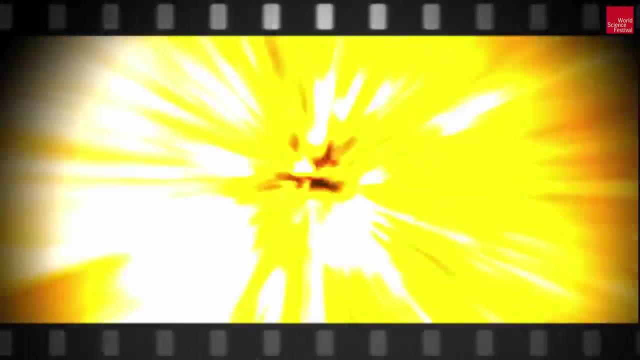 imagining that the Big Bang might be followed by an era of space, By an era of spatial expansion that would one day end, leading to spatial contraction and the recreation of a dense universe that then expands anew through another Big Bang, and the cycles repeat. 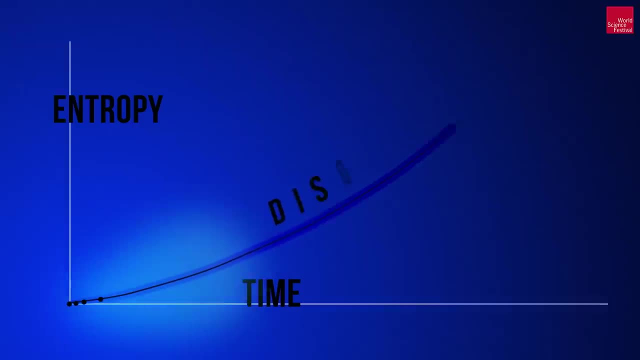 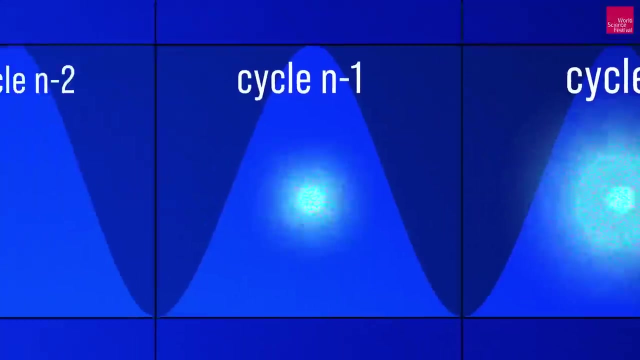 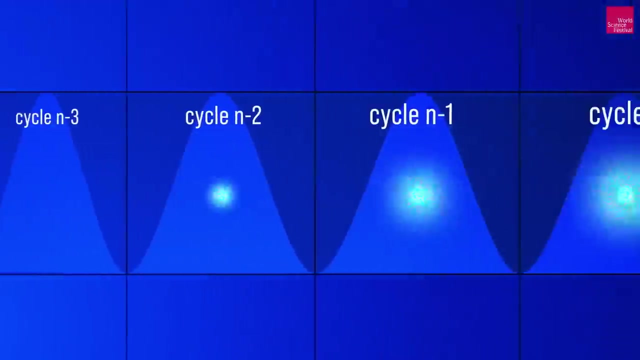 Further research, taking into account the relentless rise in entropy or disorder dictated by the second law of thermodynamics, revealed that such cycles could not have happened infinitely far into the past. The cycles themselves must have had a beginning, But an incarnation of a cyclic universe has more recently been proposed. 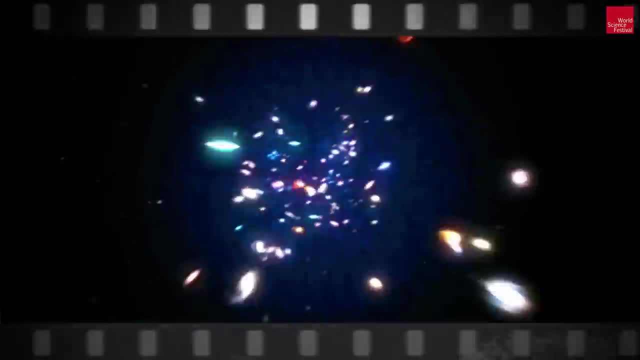 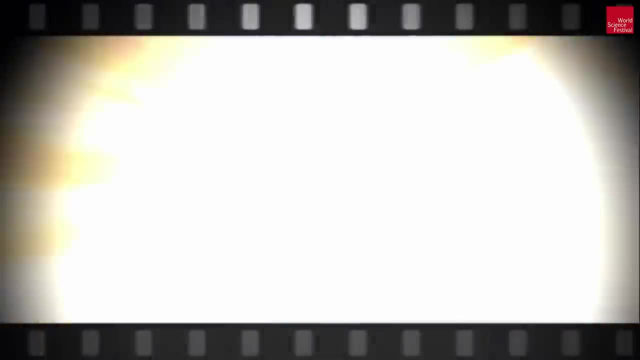 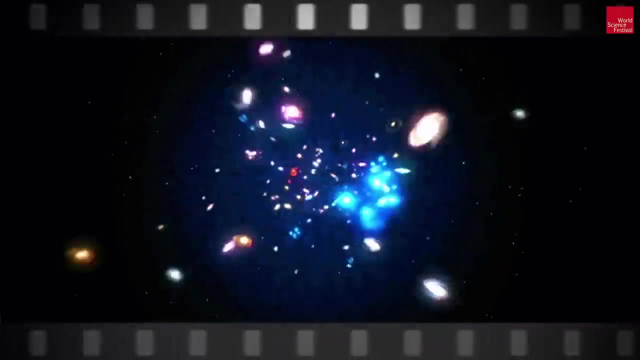 and its proponents argue that the cycles in this version could have been happening arbitrarily far back, indicating that the universe would not have had a beginning, And, if their calculations prove relevant to reality, their current cycle may come to an end sometime in the far future. 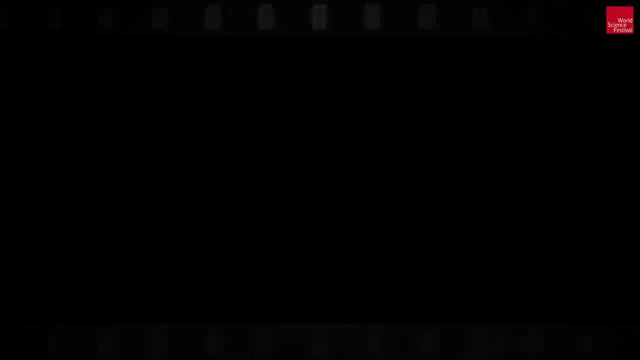 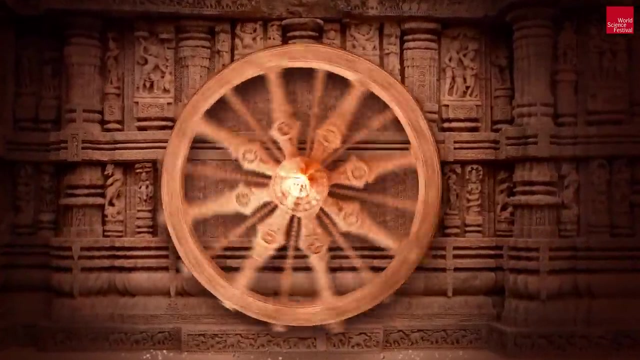 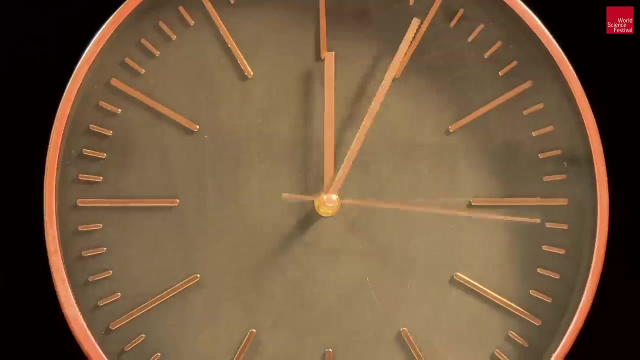 This new perspective on time and cosmological development offers a controversial competitor to mainstream cosmological thinking and, if correct, will harken back to ancient wisdom that encourages us to reimagine time and consider a reality not subject to the usual organization of beginning, middle and end. 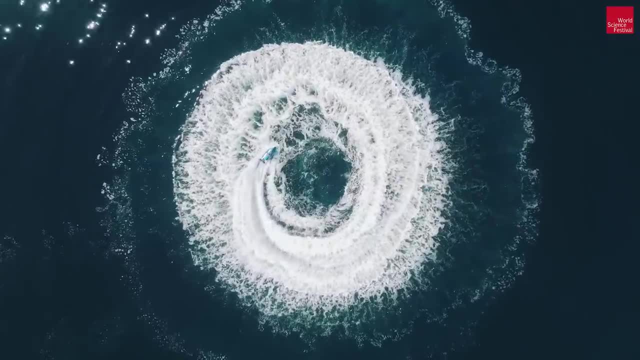 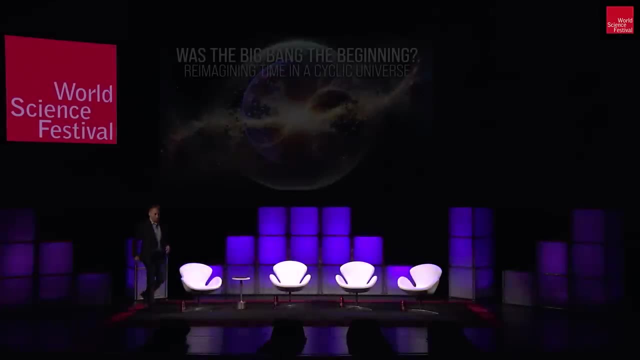 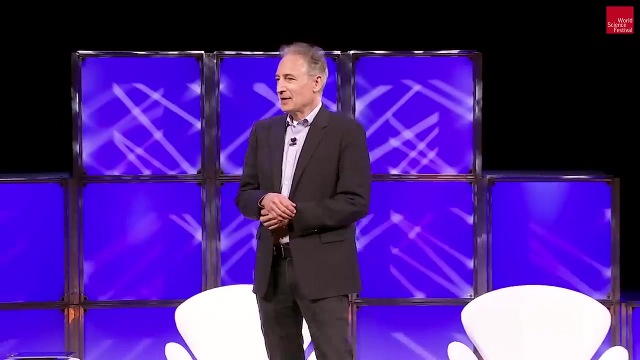 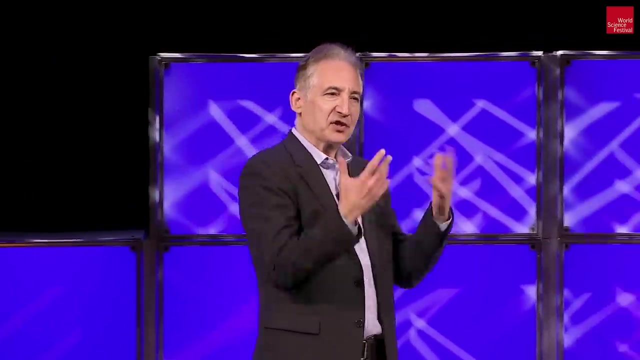 A reality that, in this view, may surprisingly be our reality. Good evening, Thank you. You know, we in science we work often within paradigms, certain established ways of thinking about this or that quality of existence. 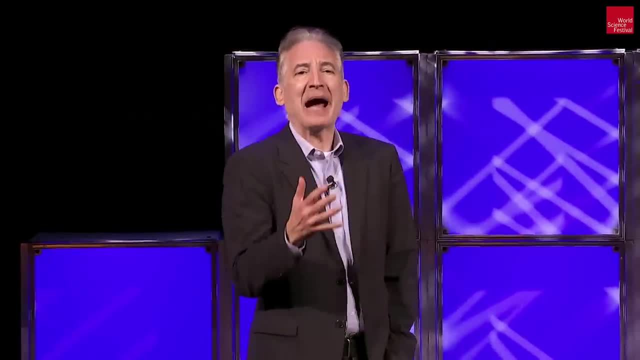 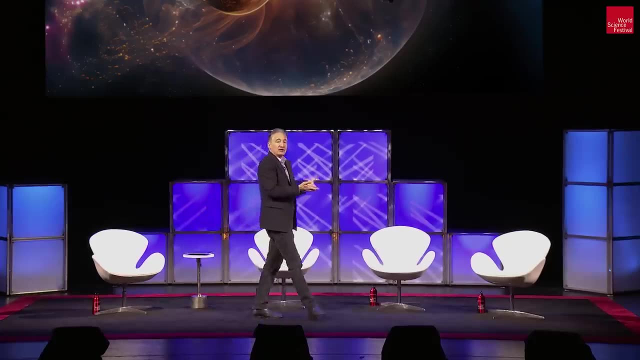 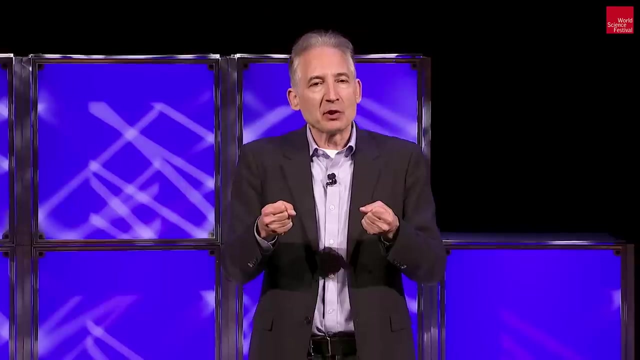 And these paradigms can be quite useful, quite fruitful, quite powerful in guiding our research, what we focus on and the way in which we analyze and interpret data. But every so often we learn that the paradigm needs to be looked at anew. 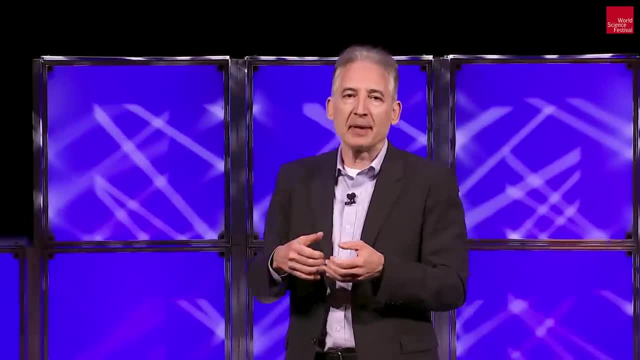 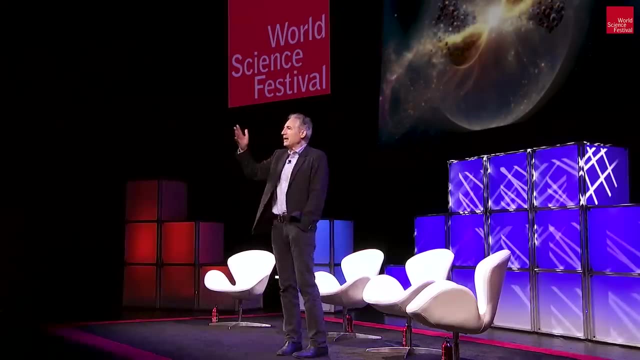 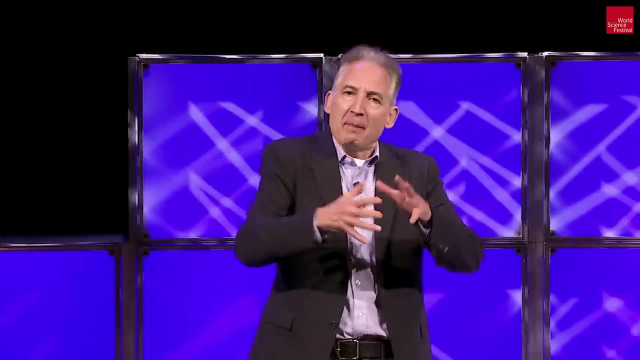 Sometimes we need to take a kind of sledgehammer to the paradigm and break it and start fresh, to free up our thinking. And when it comes to the big questions of cosmology, how did the universe as we know it come to be? we may potentially be en route to that kind of rethinking. 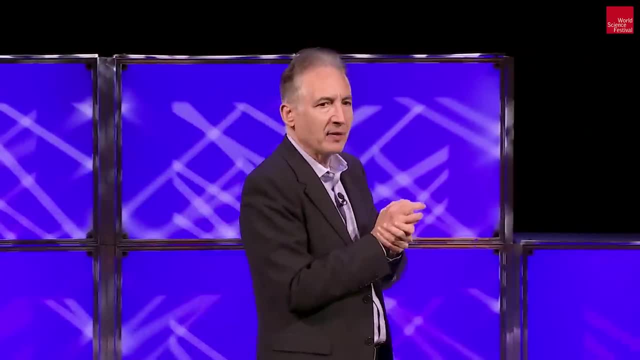 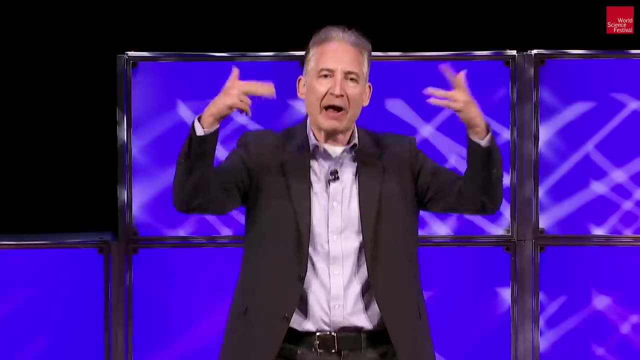 at least according to some of the scientists that we will have on the stage here in just a moment, Because, as we just saw in that piece, even Albert Einstein went through a radical change in thinking, initially anticipating that on the largest of scales, the universe was fixed. 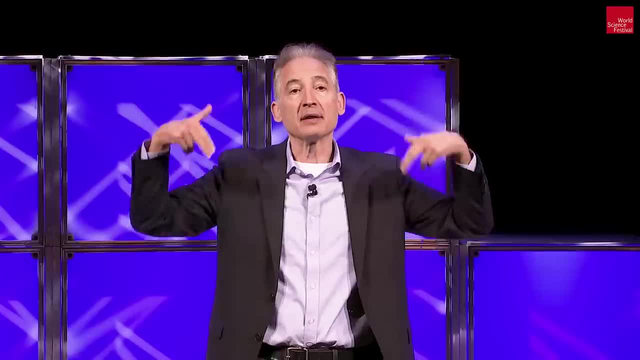 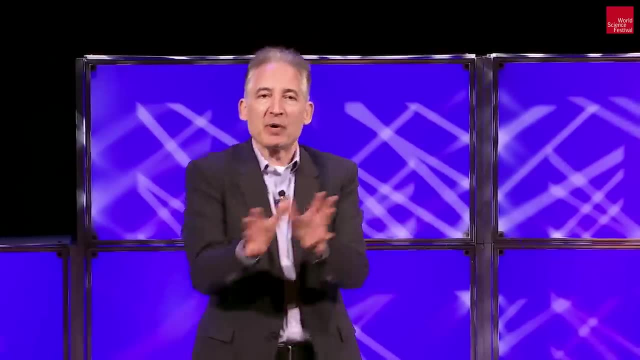 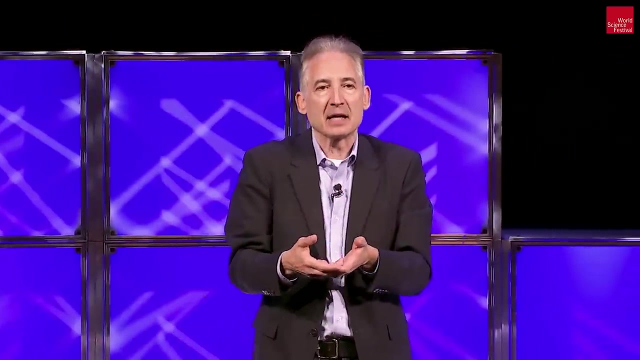 eternal, static and unchanging, And then, ultimately, through observations that actually comported well with his own general theory of relativity, Einstein did an about-face and came to recognize this idea of a beginning as being relevant to reality as a whole. 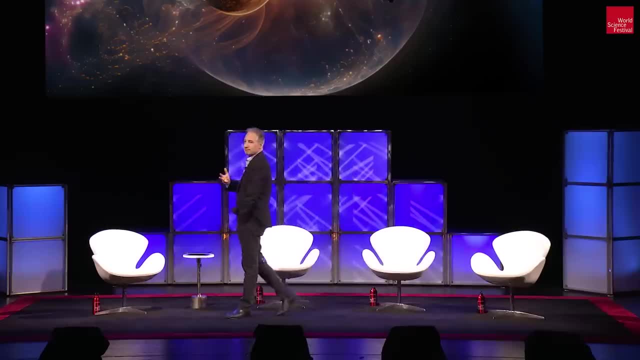 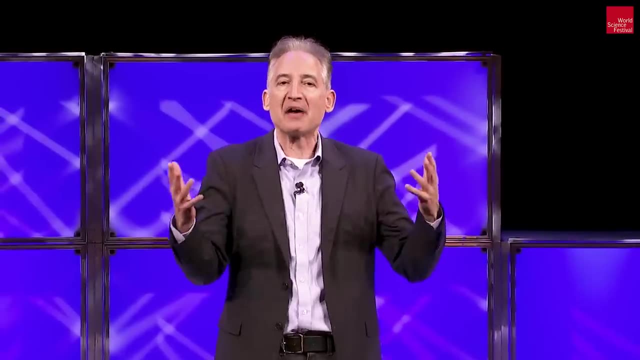 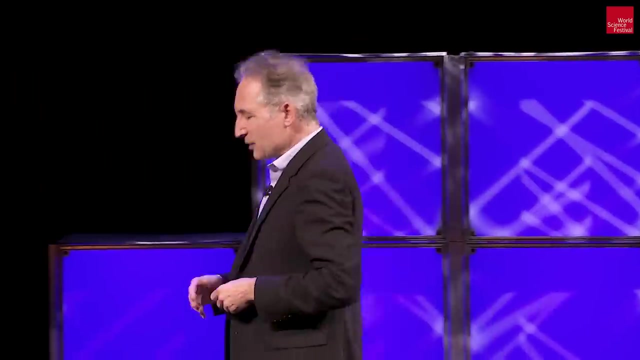 But just because Einstein believed it and just because there's been a great deal of evidence supporting it, it doesn't mean that we don't want to entertain alternate possibilities that might fit the data just as well, And indeed that's going to be the subject. 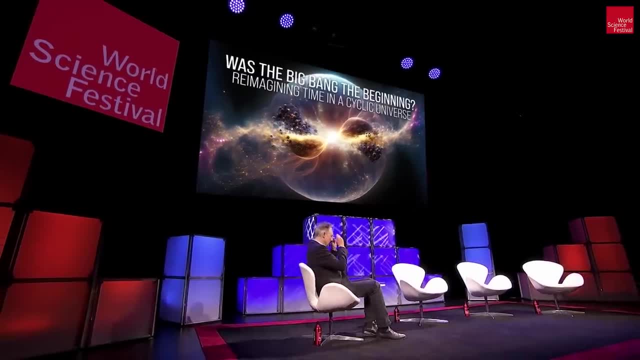 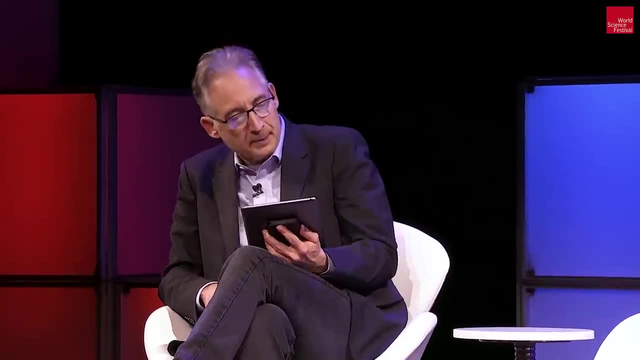 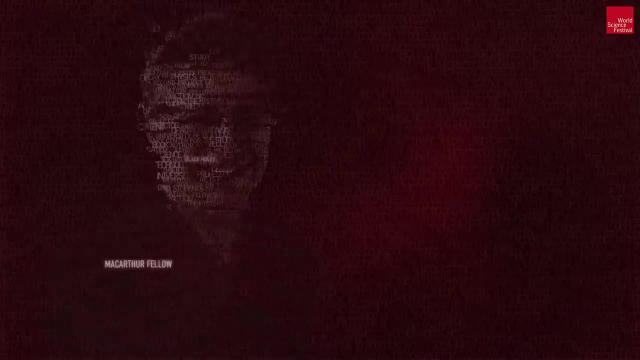 that we are going to explore here this evening with some deep thinkers who have spent a lot of time thinking about these issues. First up we have Peter Galison, who is the Pellegrino University Professor of the History of Science and of Physics at Harvard University. 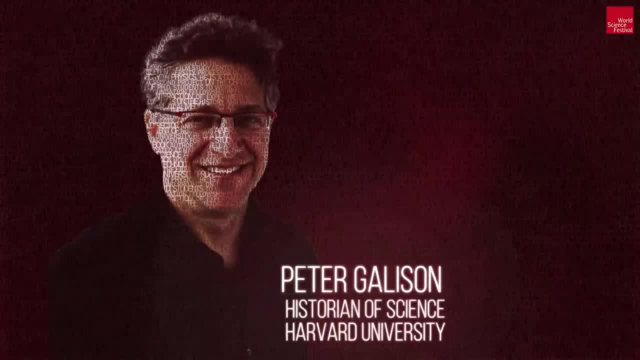 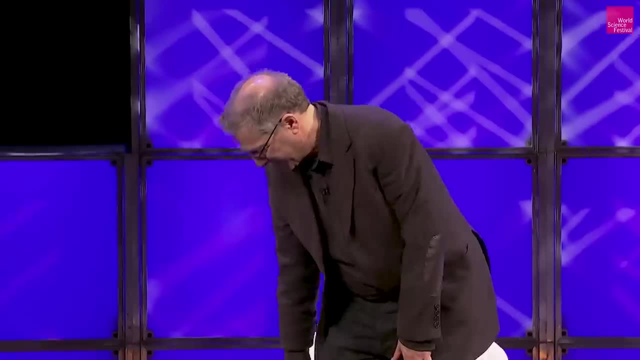 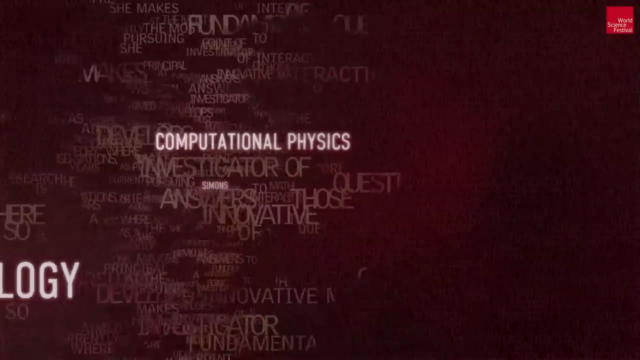 He's a leading historian of science, whose research explores the interaction of experimentation, instrumentation and theory in physics. Welcome, Peter. Nice to see you, Brian. Next we have Anna Iyash, who is a senior research scientist at New York University. 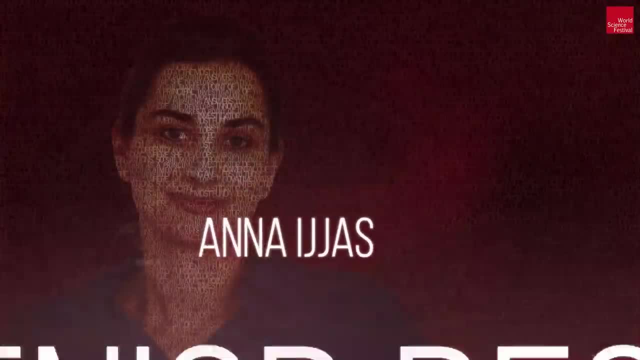 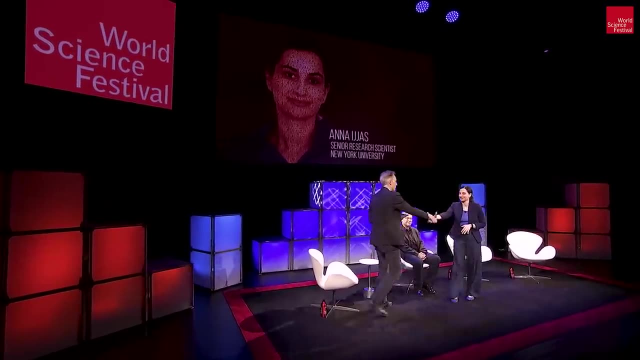 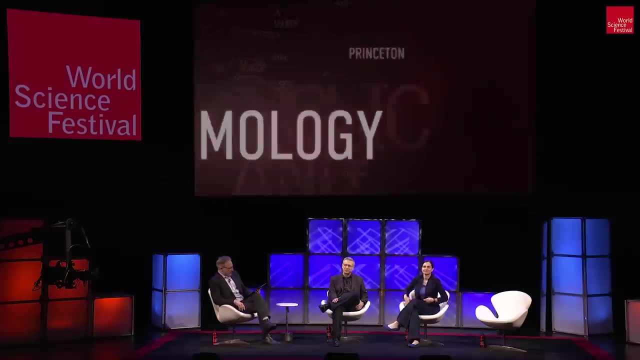 and a principal investigator of the Simons Initiative, New Directions in Cosmology and Gravitational Theory. In her research she studies the origin, structure and evolution of the universe. Great to see you. And finally we have Paul Steinhardt. 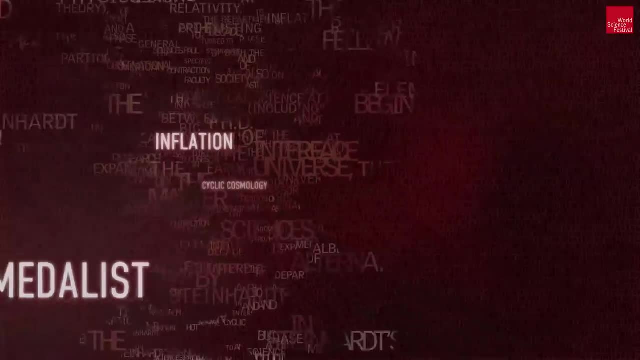 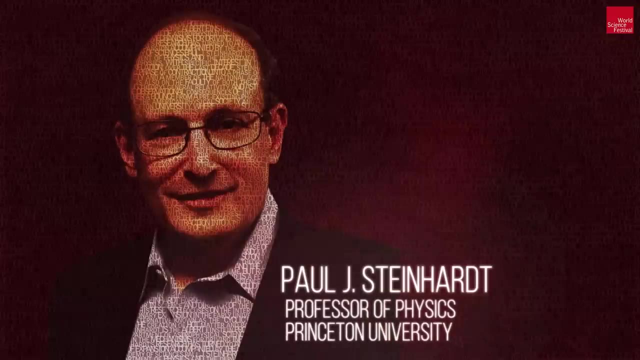 who is the Albert Einstein Professor in Science and Director of the Center for Theoretical Science at Princeton University, and a prime architect of our leading cosmological theories. In 2002, his contributions to science, Steinhardt was awarded the prestigious Dirac Medal. 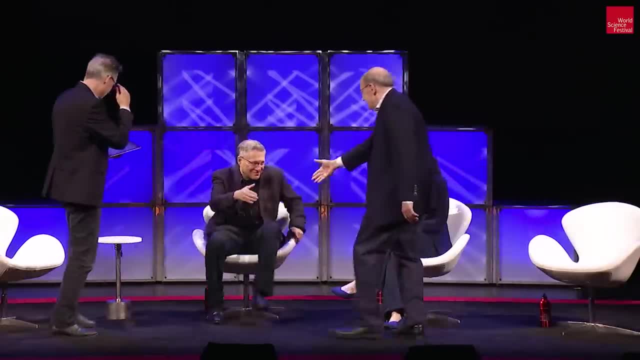 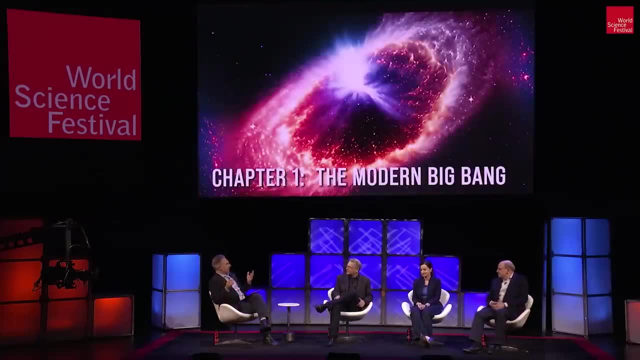 Thank you, Good to see you. Good to see you, yeah, Good to see you. Good to see you. All right, let's just maybe begin with a big sort of overview of the human urge to understand origins. I mean, we see it across cultures. 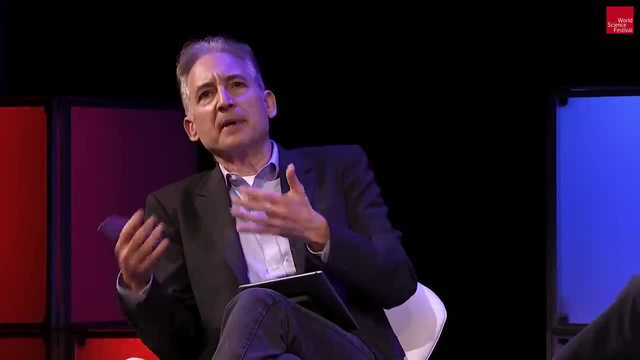 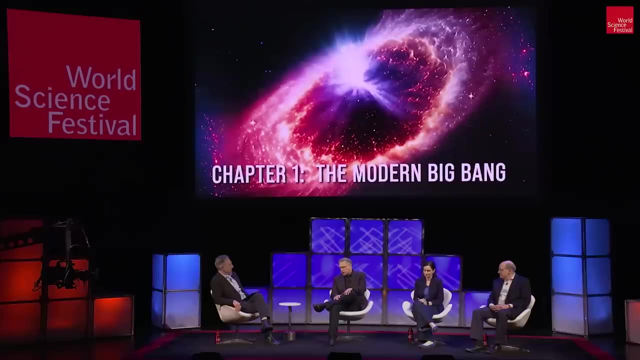 There's almost no culture that doesn't come with some kind of creation myth, creation story. Where does this urge come from, Peter? I think that the attempt to understand the structure of the universe as a whole, to see the stars and to look at the Earth. 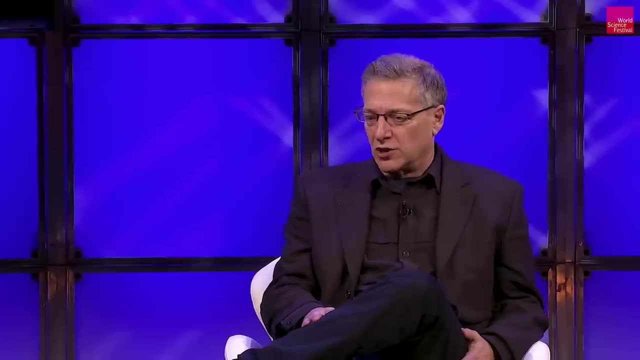 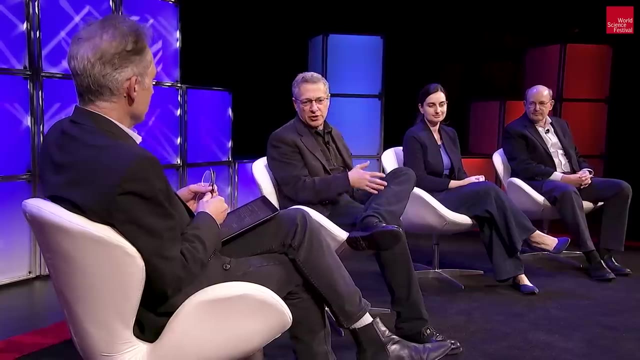 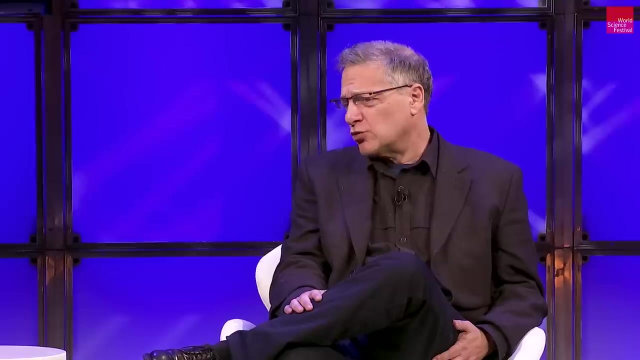 the plants, the objects, the peoples around us has always seemed to cultures something that had to be accounted for, And sometimes that's done with images, sometimes with stories or accounts, sometimes in books and poems. But it is a universal drive to understand why we're here. 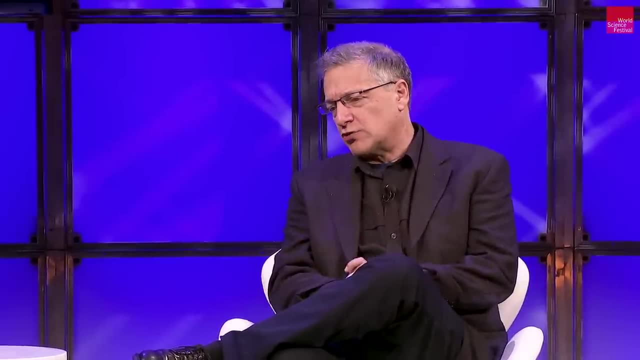 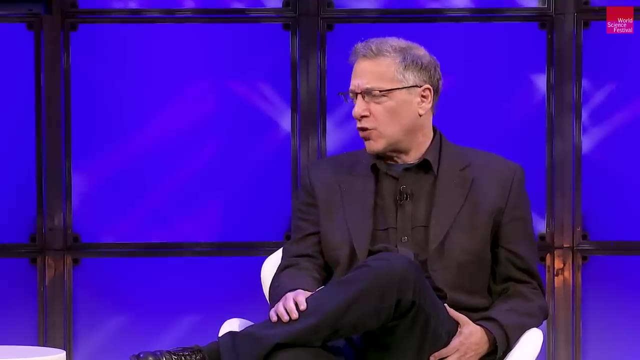 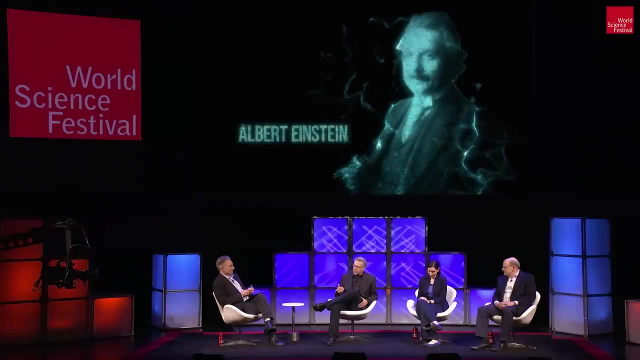 In the case of the scientific tradition that we're enmeshed in right, the study of the universe as a whole is a fairly recent affair, And it's really with Einstein, And one of the things that's so surprising is that he finished his General Theory of Relativity. 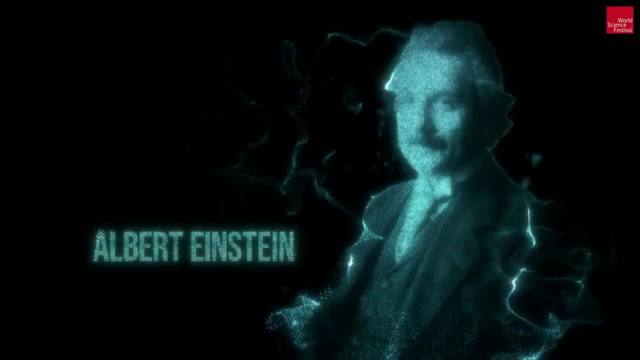 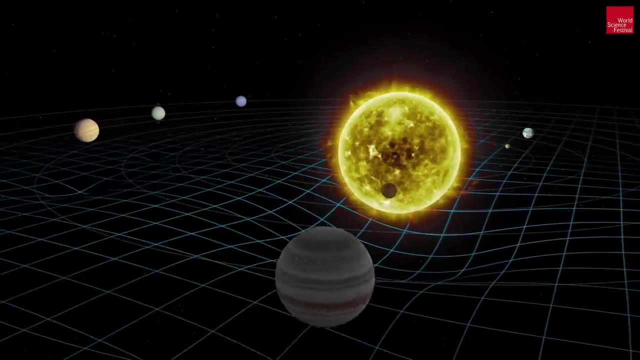 in 1915, 1916. And it was only a year after that that he began to write down a theory of the whole, of saying this account about gravity and our experience of it, our solar system, and so on and so forth. 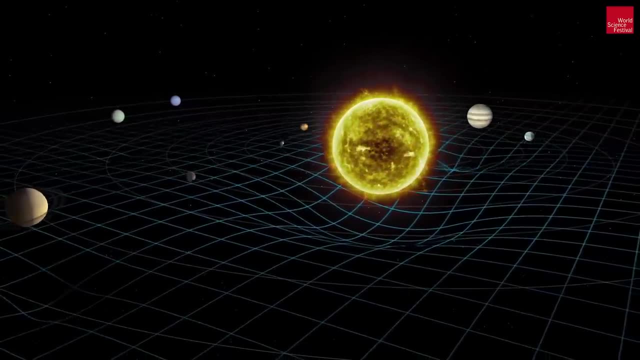 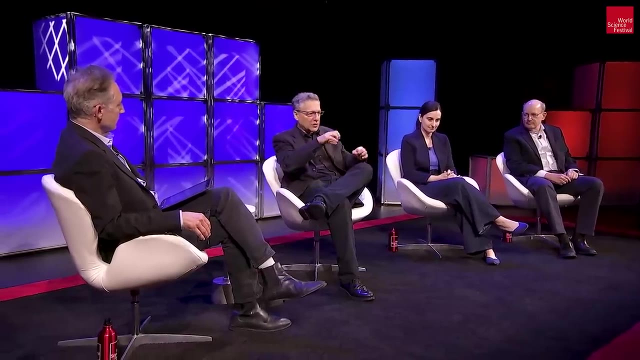 Perhaps a larger structure still was something that could be thought of as explaining and accounting for the universe widely considered, Not looking at the little clumps of matter that make up Earth or Saturn or the Sun, but imagining mass and energy spread out over the whole. 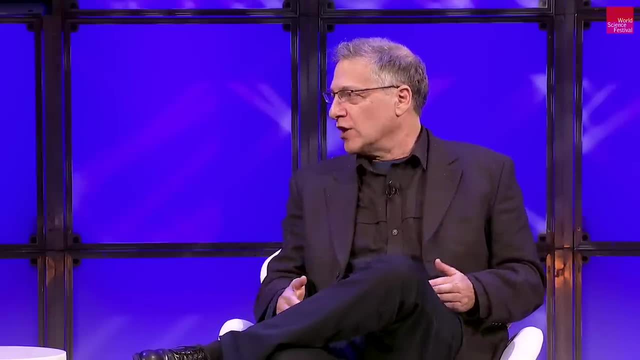 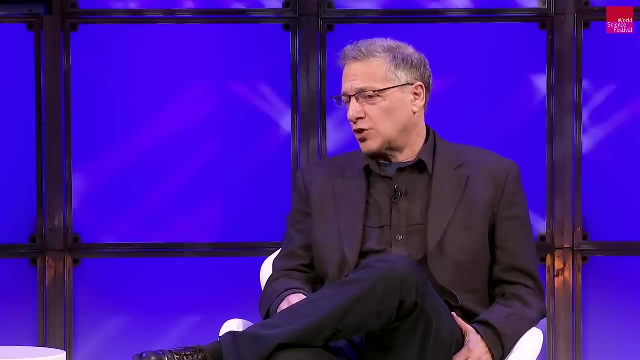 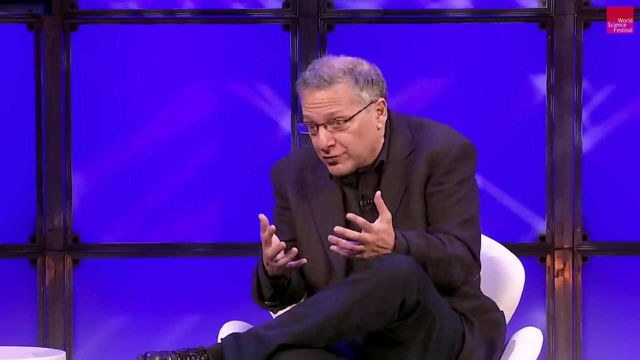 and thinking of this as having a geometry. This is really the birth of a modern observational science of cosmology, And that's So. we're still in early days. We're just over 100 years into a history of cosmology, even if the drive to understand the universe 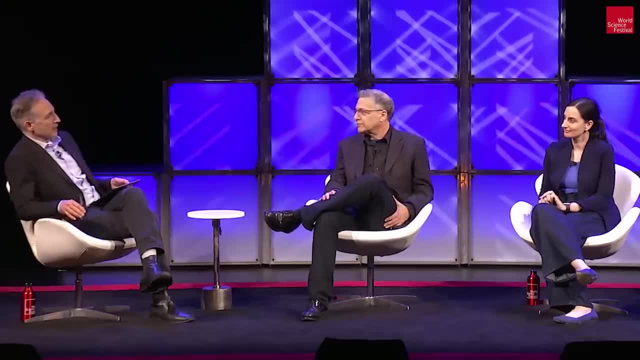 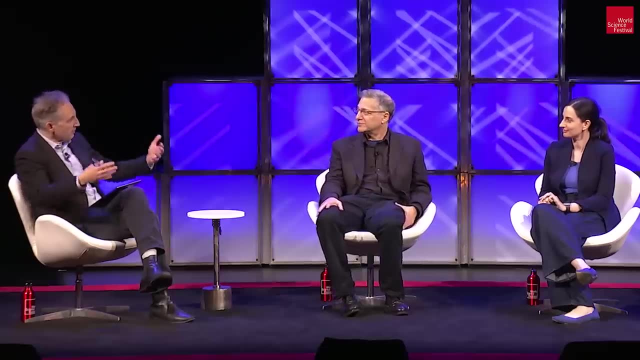 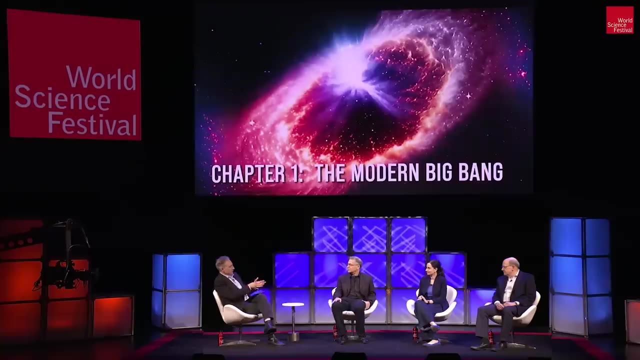 goes back many millennia. Yeah, So, Anna, in your scientific career, you've spent a lot of time trying to push the boundaries of our understanding of cosmological thought When you think back on the eras that preceded ours, with people like Lemaitre and Friedman and Einstein. 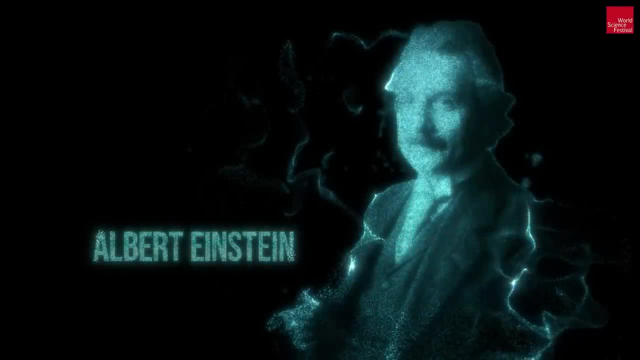 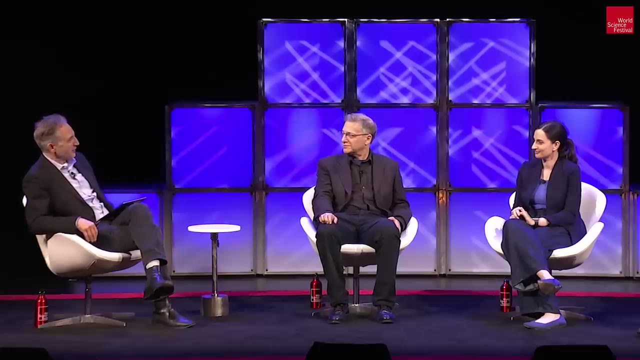 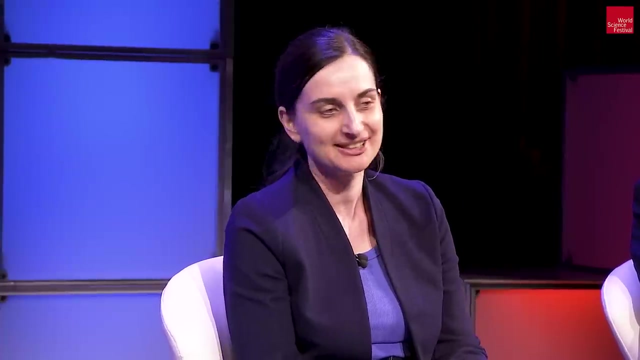 we'll perhaps talk a little bit more about their contributions. do you see yourself following in their footsteps or do you see yourself as trying to blaze a completely new path? Oh, definitely the first one, Definitely the first one. So maybe I'll get to that, but you know, 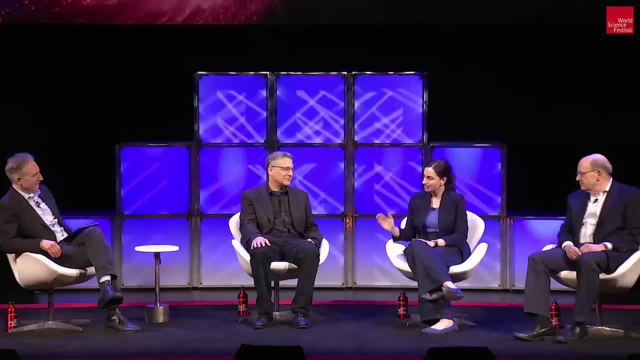 and I'm sure that Paul will talk about it. when cosmology really took off in the 80s, right then it became your field. Particle physics made it to an experimental science And I believe you know, a few years ago. 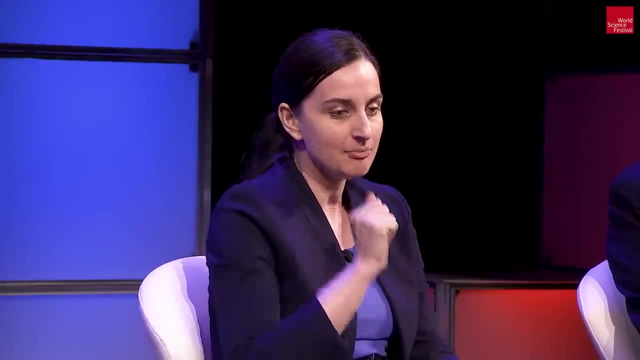 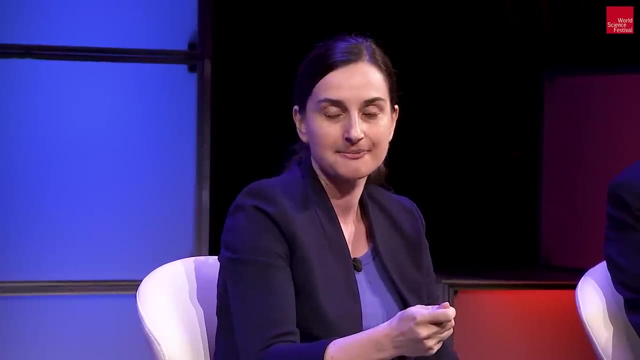 and we will get back to that too. we might have reached, you know, the limit how far we can push the boundaries of cosmology and our understanding by just using particle physics, And what I have been doing a few years ago is actually going back and seeing. 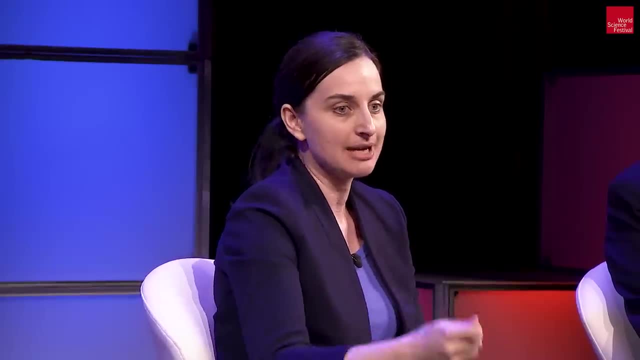 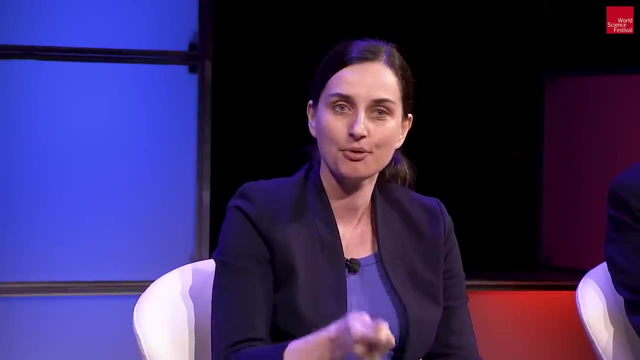 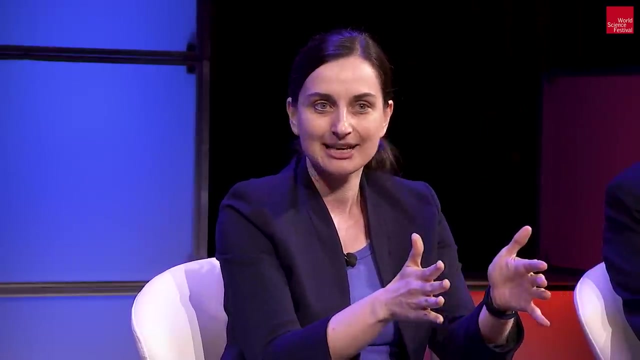 maybe we missed something: what we can learn by using general relativity, especially using the modern tools of computer simulations, and maybe understand more. So I definitely see myself much closer to Lemaître and Tormund and Einstein than maybe most of my colleagues. 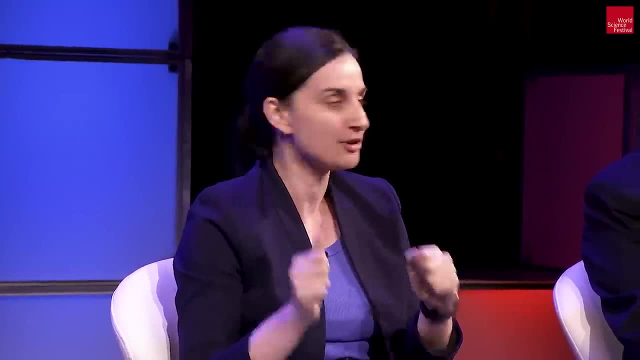 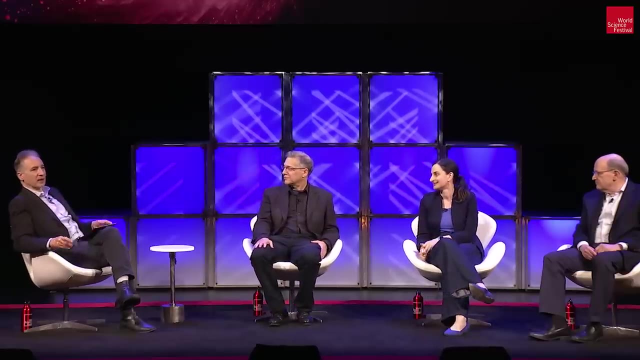 who are doing particle physics-inspired cosmology that was funded by Paul- are doing. So definitely the first one. Yeah, that's an important distinction to make. It is the case now that cosmology is a field that brings in people from all over. 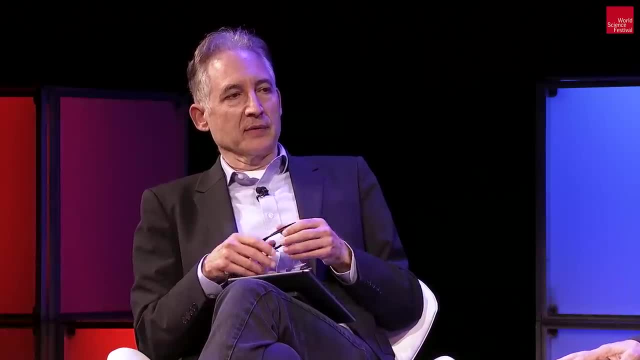 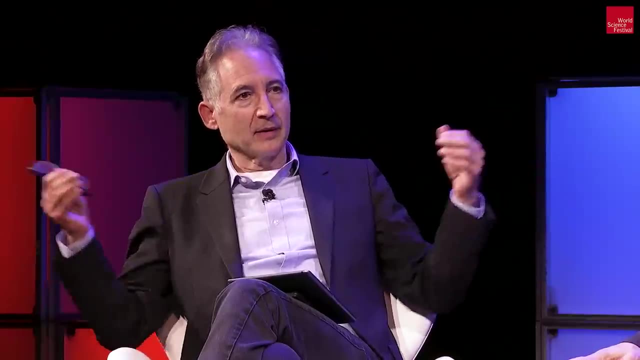 but certainly particle physics, gravitational physics, and in the early days it wasn't so obvious that someone working on the elementary particles would have something to say about the largest structures in the universe. So, Paul, before we get into sort of the more modern story of cosmology, 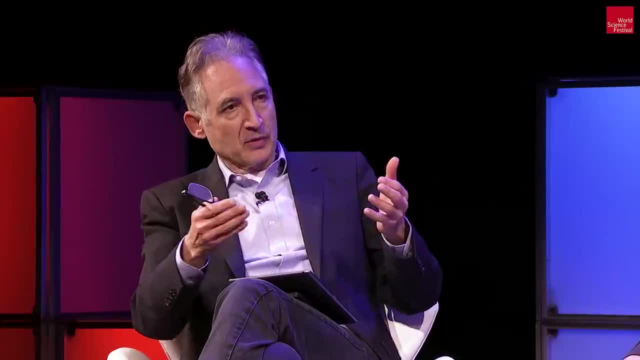 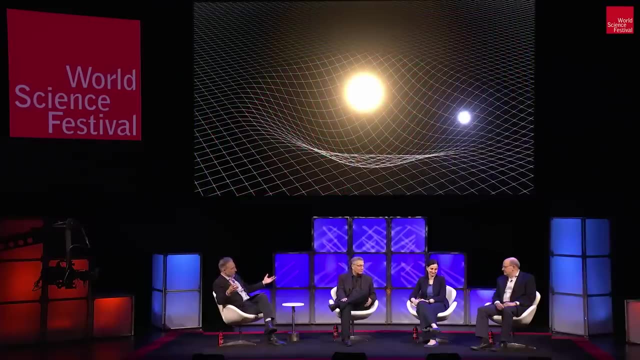 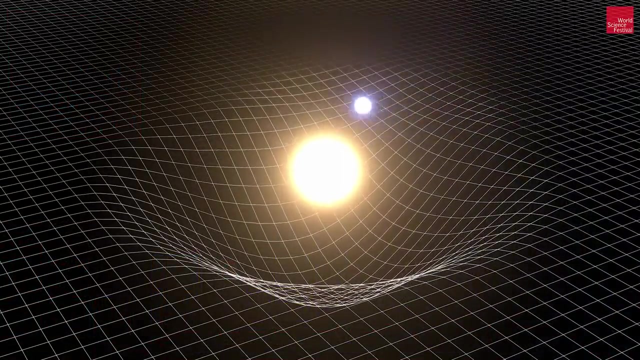 where you make a tremendously important mark. can you just give us a thumbnail sketch, going from Einstein's new view of gravity in terms of a flexible space-time that can stretch and swell and so forth, the ideas that that then take that picture and turn it into a cosmological story? 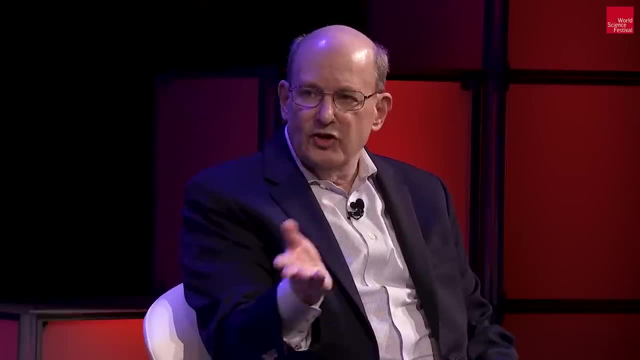 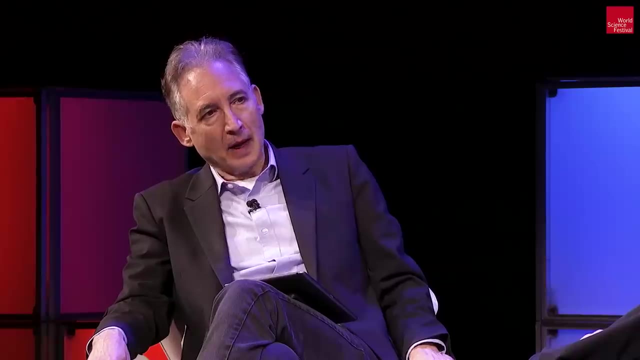 Can you just give us a feel for how that went Sure? I mean, it's curious that Einstein had a theory that space was elastic and could change with time, but came up with a static model- Yes, isn't it- in which it was as boring as possible? 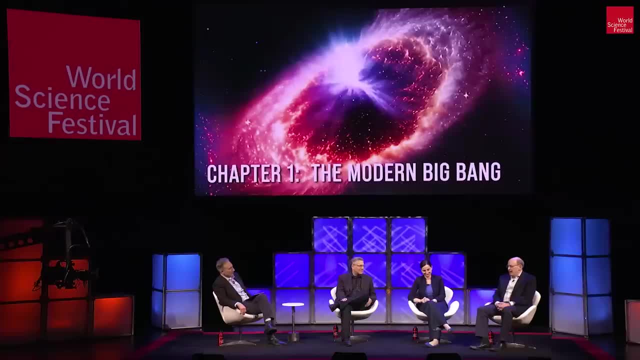 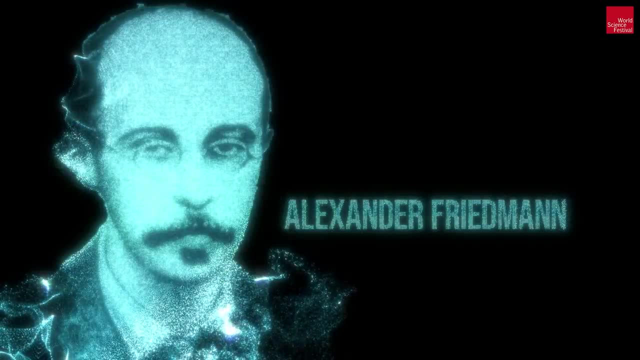 Yeah Right. So there's this kind of weird contradiction. And when, a few years later, Alexander Friedman showed that the same equations, the same Einstein equations, allowed for the possibility for an expanding universe, or a universe that would expand for a period, and reek and reek and contract. 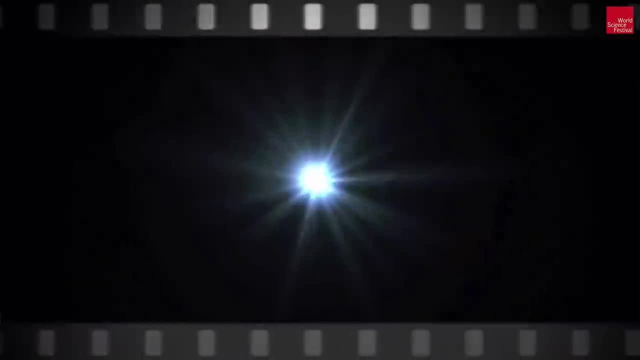 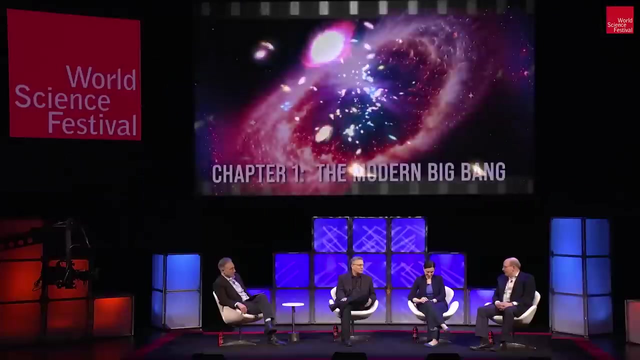 and maybe a bouncing universe that would repeat this cyclically. Einstein rejected that. Yeah, He thought it was Well. first of all, he thought it was mathematically incorrect. He even wrote a little piece that argued that it was mathematically wrong. 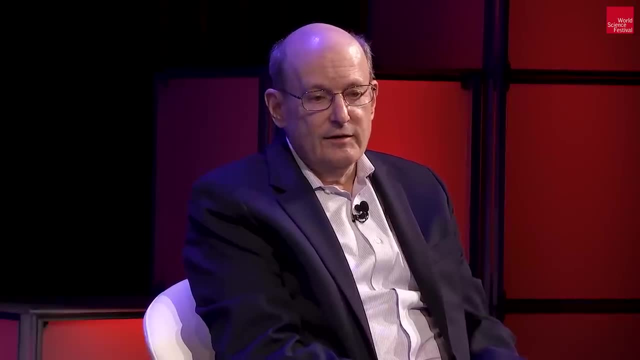 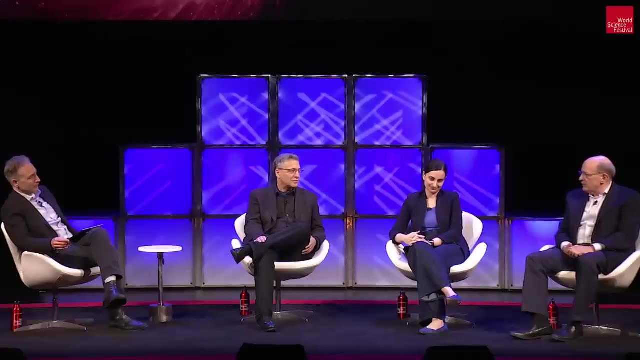 and had to retract it. That's right. Yeah, That's right, And obviously it was because it bothered him philosophically. Yeah, So the early days of cosmology. we also have to respect the fact that the early days of cosmology 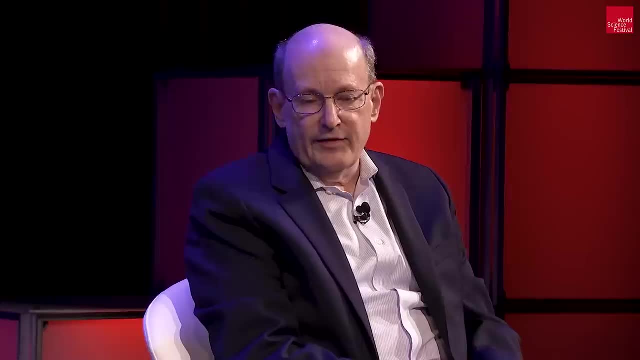 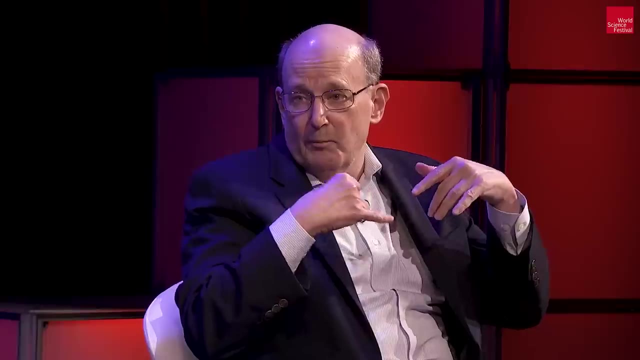 were not well informed by observations. Yeah, At that time we didn't even know there were galaxies. That was first around contemporaneous with Friedman, And then the idea that there were millions- no billions- of galaxies out there and they're moving in all kinds of complicated ways. 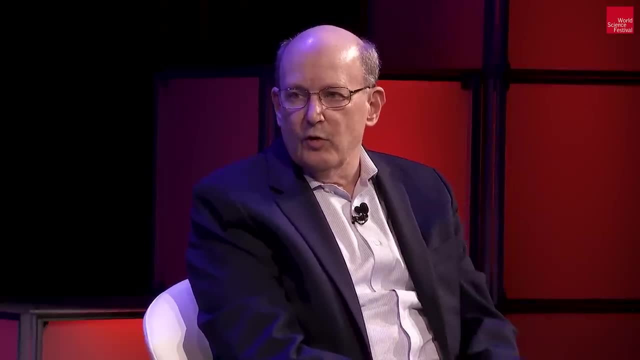 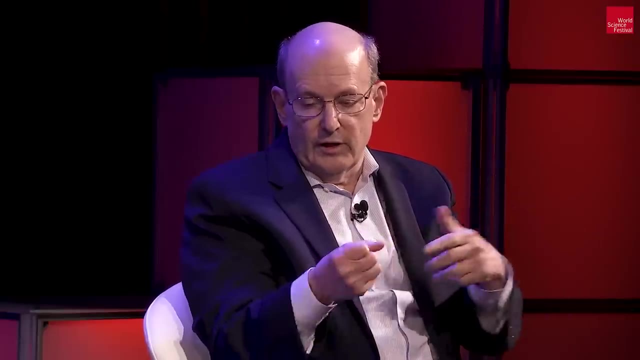 is something that developed over the course of the next decade. Yeah, And showed us that the that, in fact, Friedman's idea and Friedman and Lemaitre's idea that the universe might be moving and it might be expanding was once hot and dense. 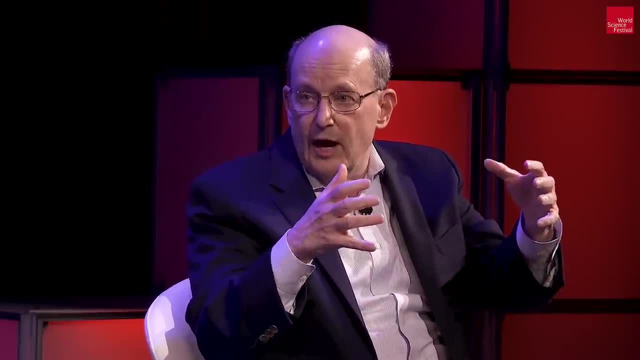 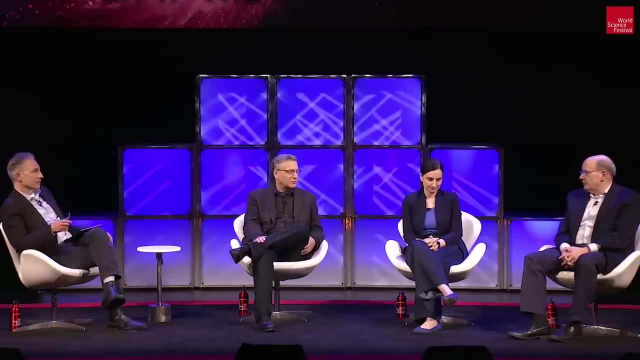 and has been expanding and cooling seems to be consistent with the observations at that time. Yeah. And then, over the course of the century, we've obtained more and more observational information that reaffirms that part of the story over and over again, Yeah. 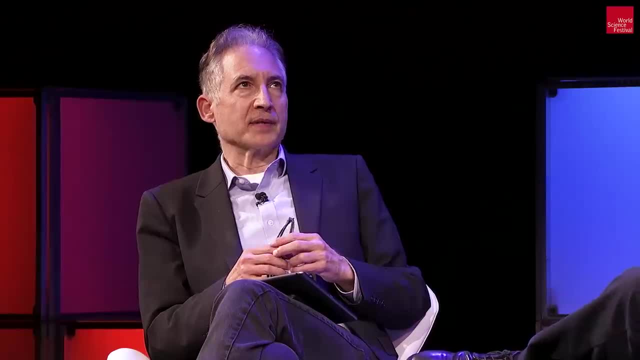 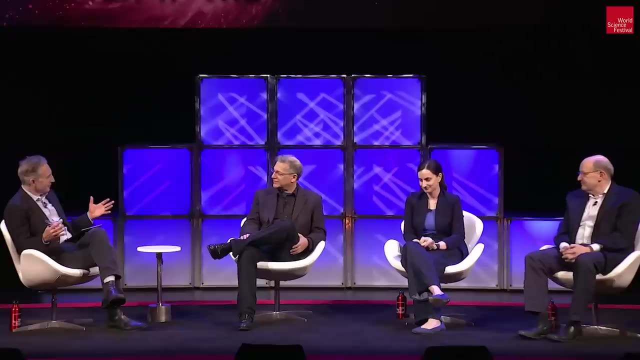 And so, Peter, I just want to drill down a little bit, and I don't want to psychoanalyze Einstein per se, but here's this radical thinker who gives this radically new theory. as Paul was mentioning where gravity is now, Who would have thought? 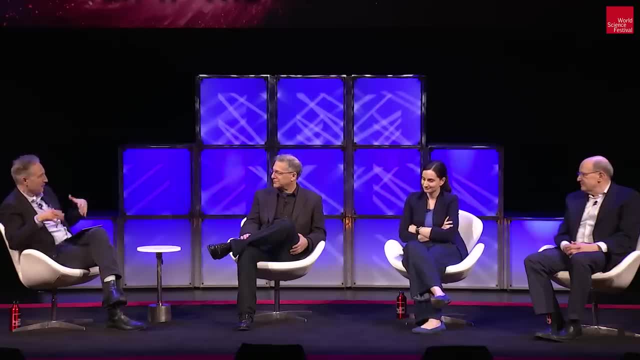 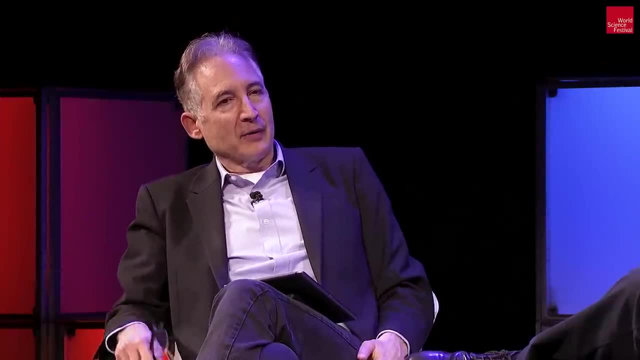 Gravity is geometry, warps and curves in space-time. It's flexible, And yet when the math suggests that flexibility applies to the entirety, he recoils. Now there is some evidence, and I wonder if you have a sense of this. 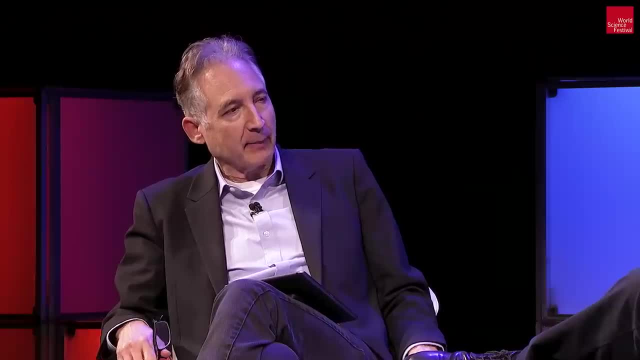 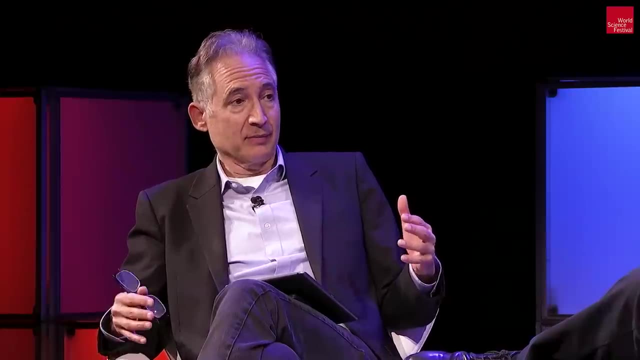 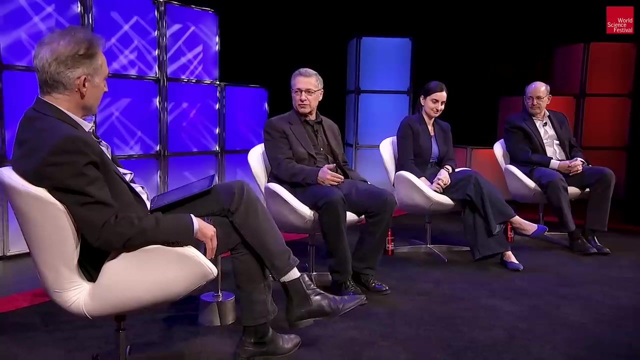 that Einstein did not like the idea of a dynamic universe because it suggested a beginning, and a beginning to him felt too religious, too theological. You know, I think the idea of a beginning has been attached to religious accounts for a long time. Yeah, 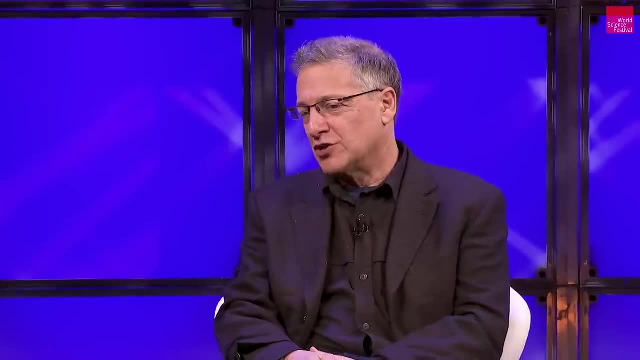 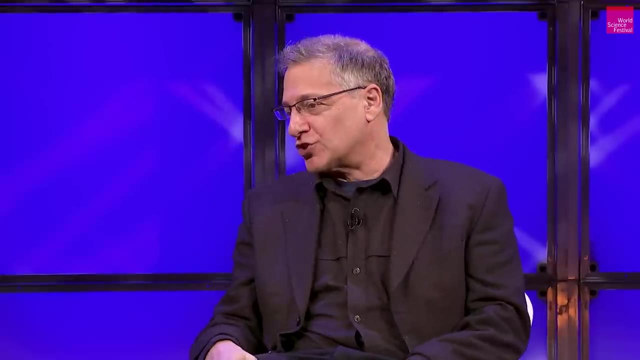 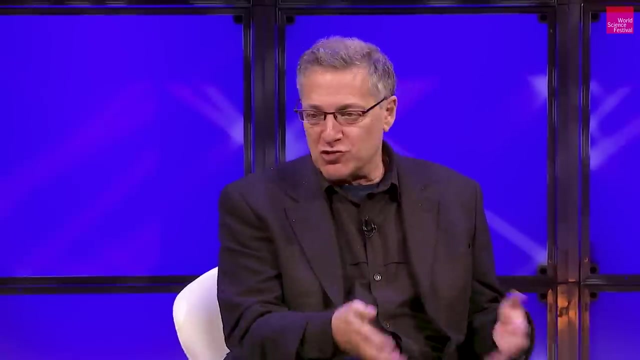 And in the dispute, for example, between those who advocated for a steady-state universe, that matter was popping into existence all the time versus the idea that there was a Big Bang which was only resolved with discoveries in the last decades. this cosmological microwave background. 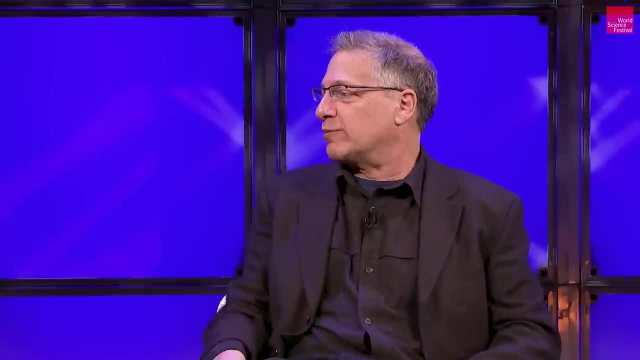 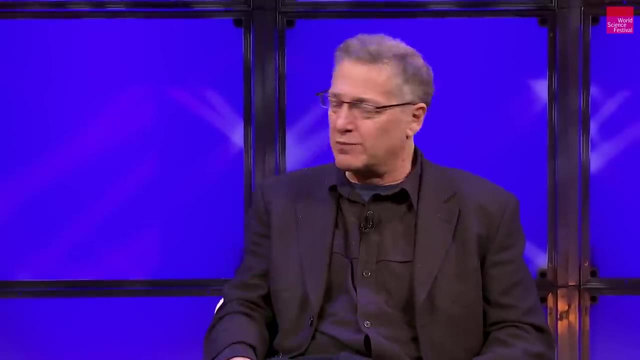 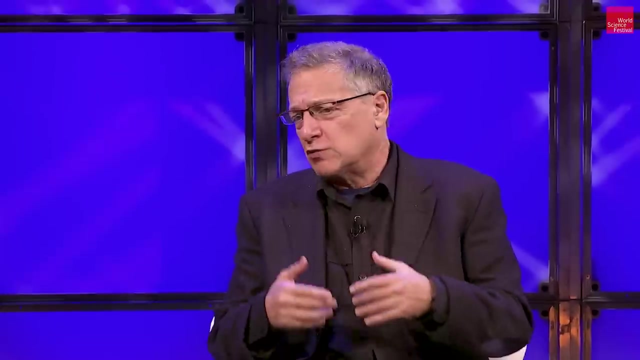 that suffuses the universe and echo of the Big Bang was a big shock- and in fact got theological endorsement- the Big Bang by the Pope and more recently again by Pope Francis- that somehow the idea of a beginning was consonant with biblical genesis. 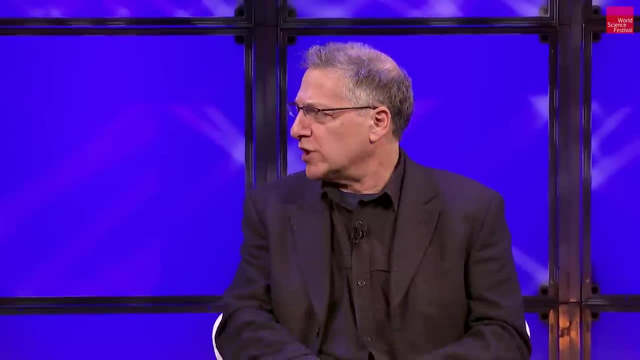 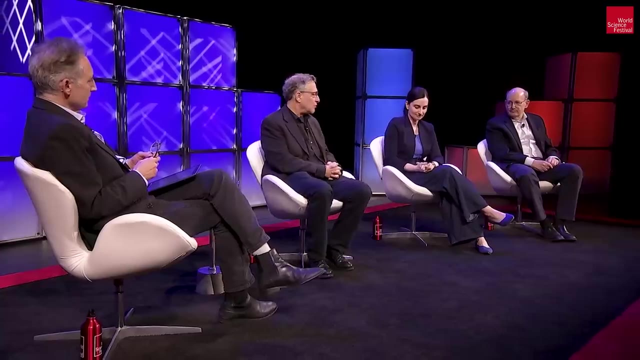 So these things had a deep root in culture and philosophy, I think for Einstein too. Einstein did care about experiment and observation, and the standard view was the stars are fixed, and it wasn't until the work of Edwin Hubble that you really started to have an idea. 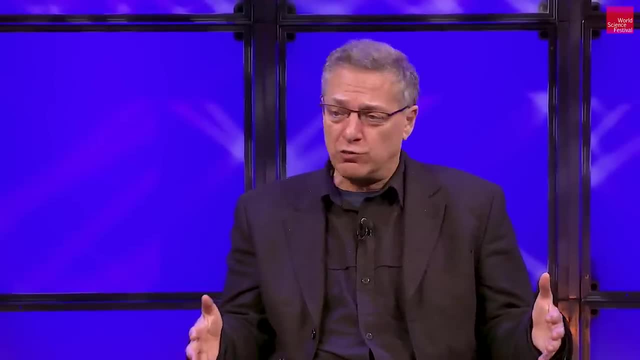 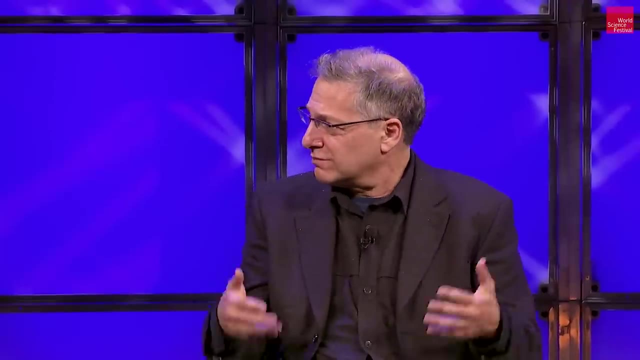 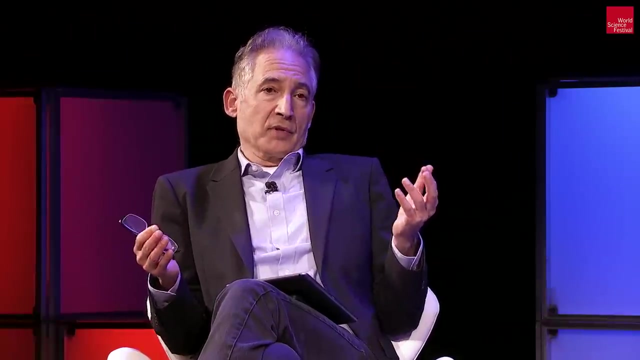 that things were expanding. So I think Einstein thought he was saving the phenomena, as they say. He was doing what he had to do to the theory to make it consonant with what he thought was standard observation at the time, And certainly was the case. 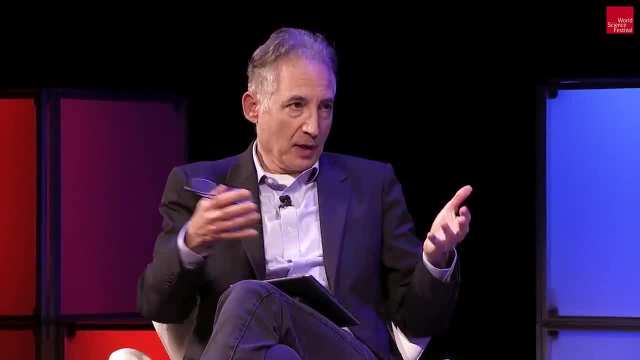 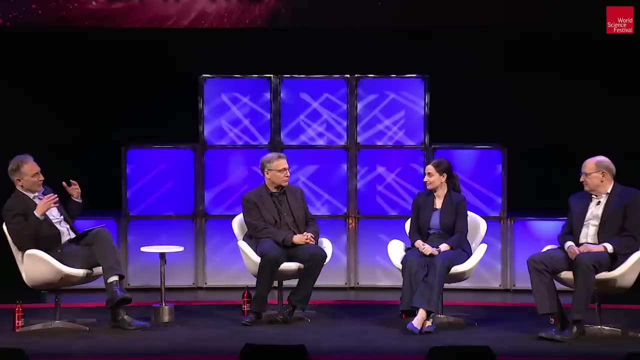 when the observations were overwhelming, he didn't stick to his guns. He absolutely turned around very, very quickly on that point. So, Anna, by you know, 1930, there's general- or by 1933, let's say: 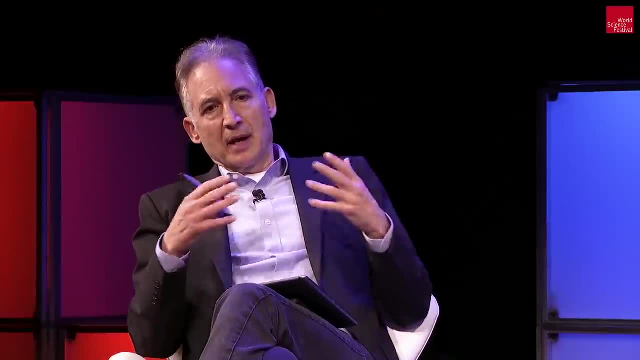 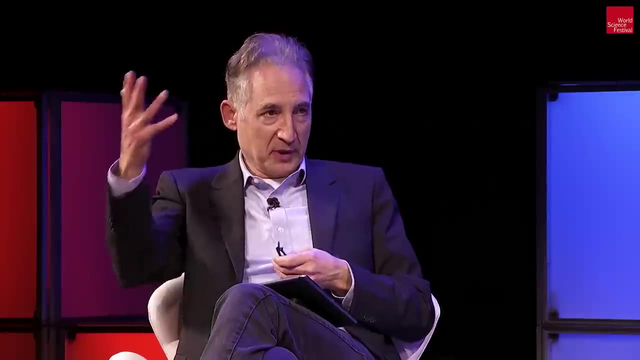 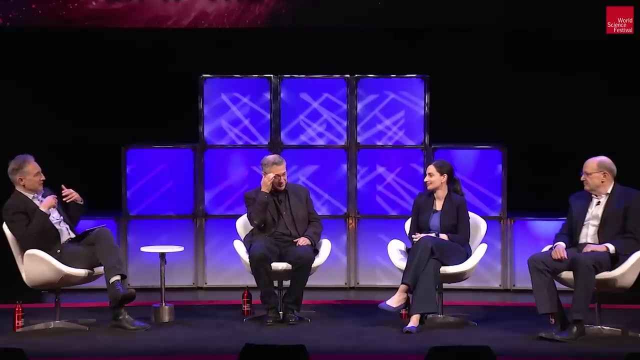 there's general consensus that the universe is expanding. Einstein's theory in broad brushstrokes agrees with this idea and you could even say predicts it, although it wasn't accepted in that particular temporal order. But as people begin to think more deeply about this idea, 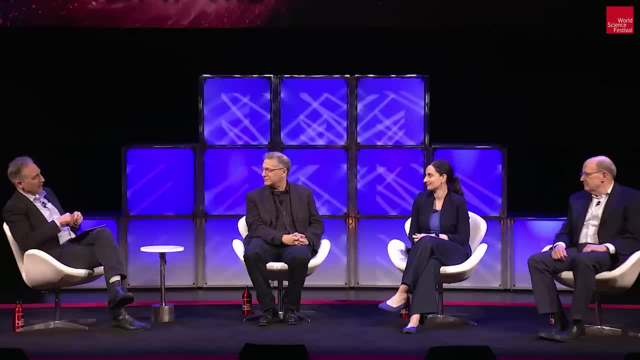 of a big bang beginning and everything swelling. from that point, cracks begin to appear, or at least issues begin to arise. They often go by the name of, say, flatness problem, horizon problem. Can you just give us? take one of those? 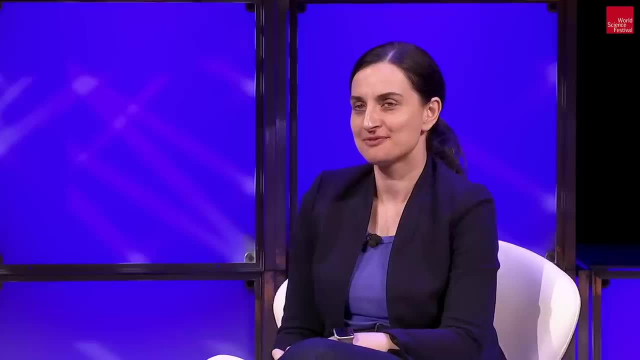 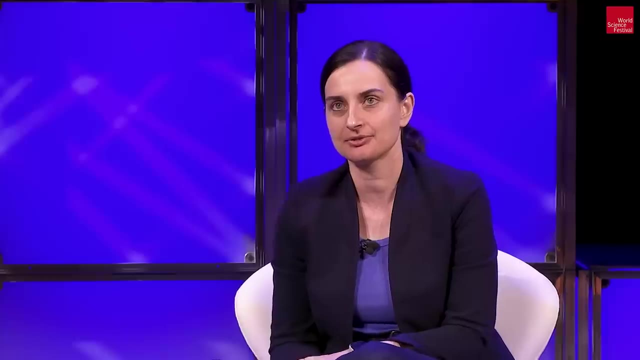 and just give us a sense of what the issue is. So this is tough, This is, this is: we still haven't really solved this problem. So this is really. these are the problems at the heart of modern cosmology that you just have to deal with. 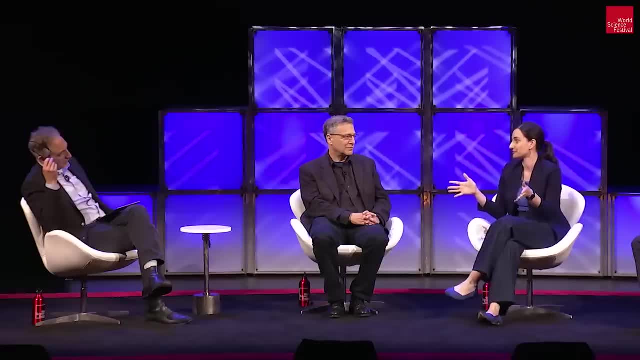 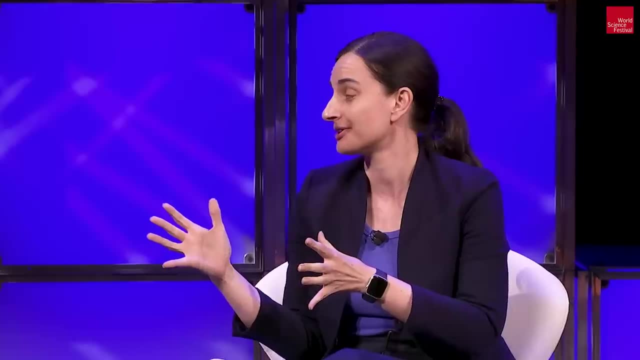 So let's start with the big bang. Yes, So I don't pick up your problems first, but let's just start with the big bang and say: why does an expanding universe imply a big bang as a beginning? Yes, How do we know that? 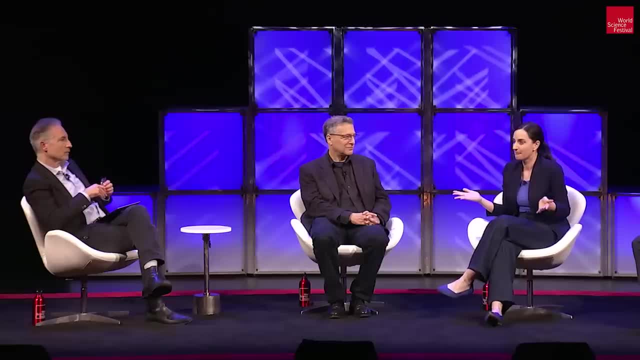 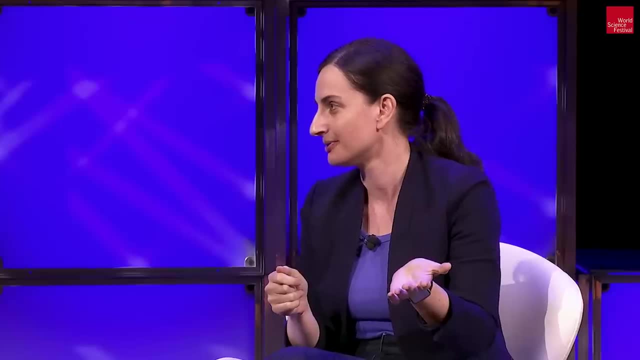 Well, the answer is: I think we all agree. We actually don't. We are all being told it that if the universe started to expand 13.8 billion years ago, then it had to have a beginning. But that's an extreme extrapolation. Just because the universe at some point started to expand, it doesn't imply that it had to have a beginning, because the extrapolation from when the first element started, when the universe was already cool enough, back to something that we might call the beginning is actually bigger in temperature. 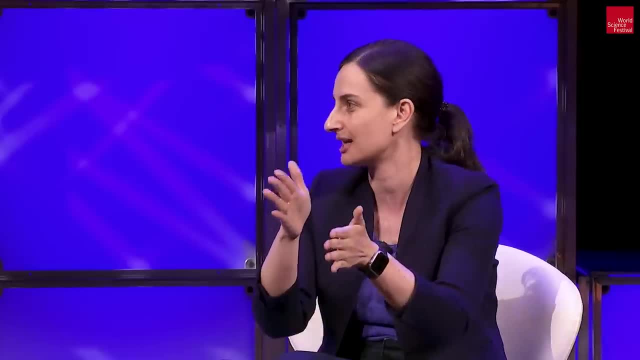 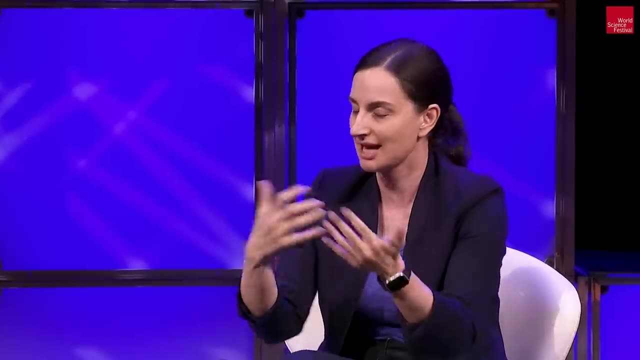 and energy and everything, And we actually don't know the theory that would describe that phase, because that would require the marriage of quantum physics and general relativity And we don't have that theory. So just to quickly jump in, just to clarify: 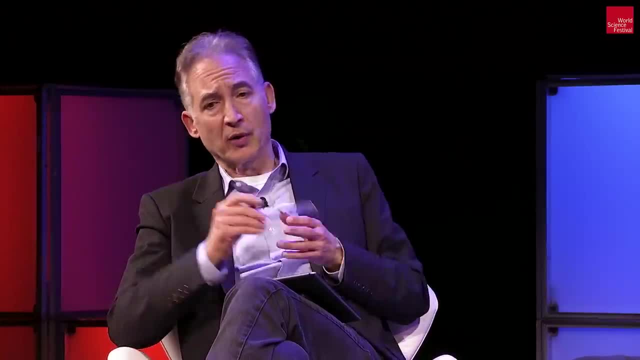 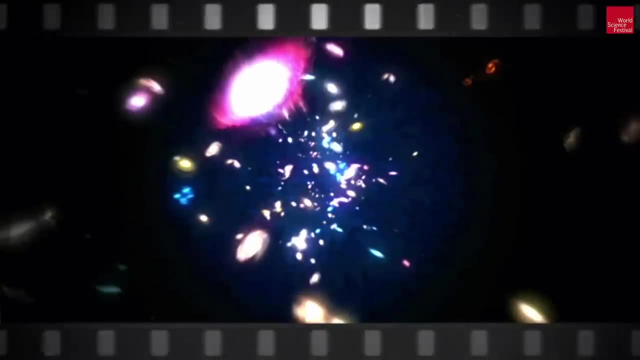 I mean the normal, the usual thinking or the usual lore is, if the universe is expanding today, you just kind of wind the cosmic film in reverse right And going back it gets smaller and smaller and smaller, And so it does suggest. 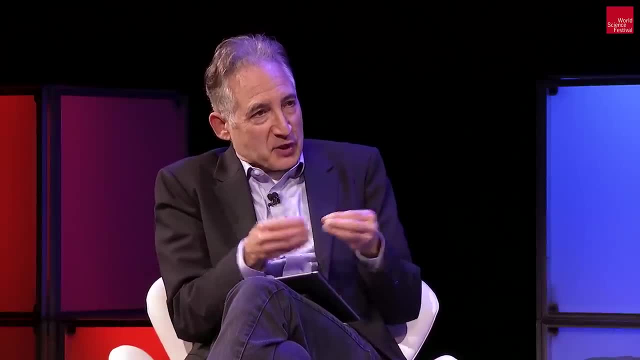 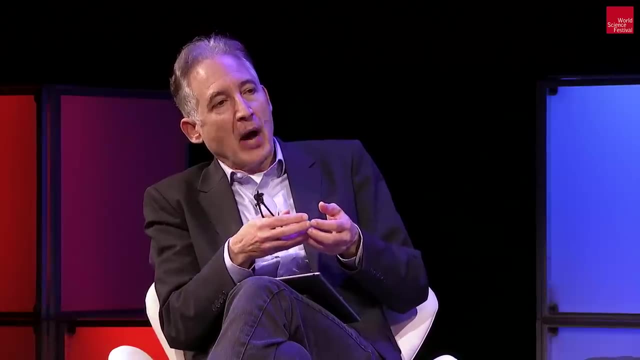 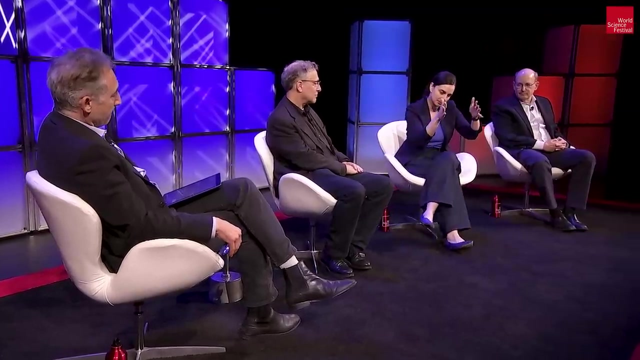 that there was some beginning where everything was small. everything is on top of everything else. But I gather you are suggesting that that's taking that winding the film backward maybe too far. Yeah, that's the point, Because just because something, if you wind back the film to 13.8 billion years ago. 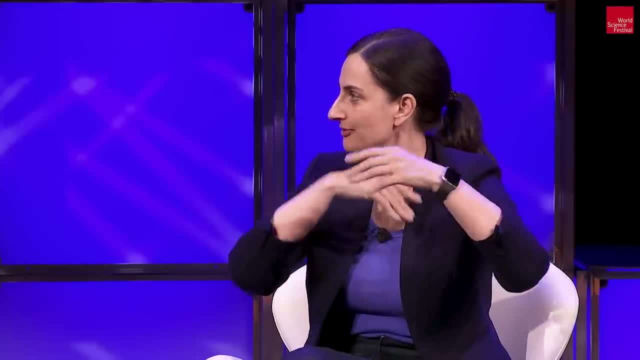 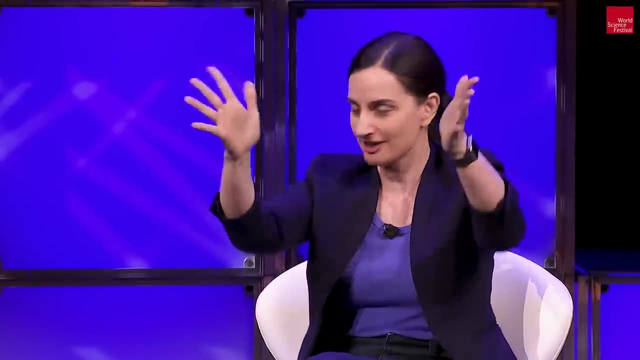 it looks okay, but only because we observe it. It could have turned out that we shoot up the satellites. look at space, because when we look far enough, that means we look back in time and we see something else. That's why we are scientists. 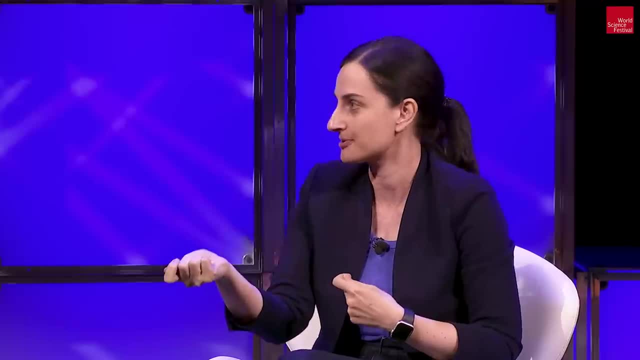 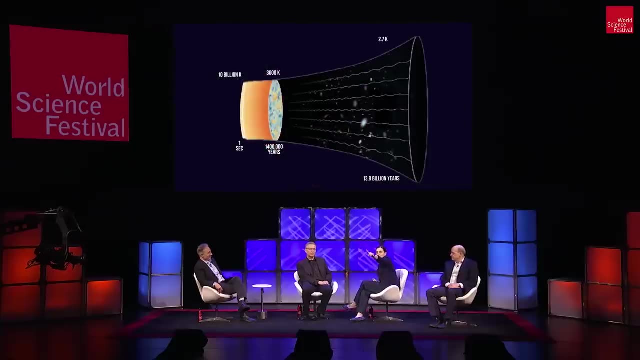 We assume something, but then we check. We check by observation, And if something else comes out, then we would have to conclude with something else. We're wrong. So we know that, because we check. That's what we know. So we know how cold. 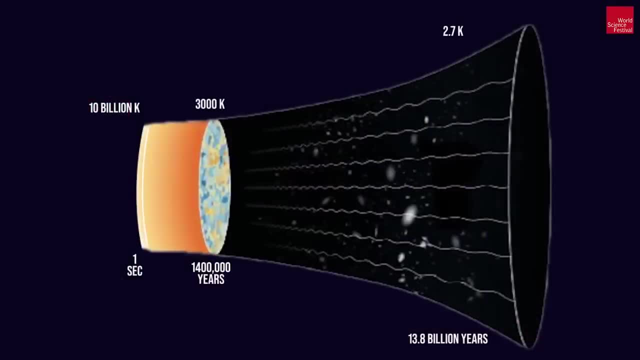 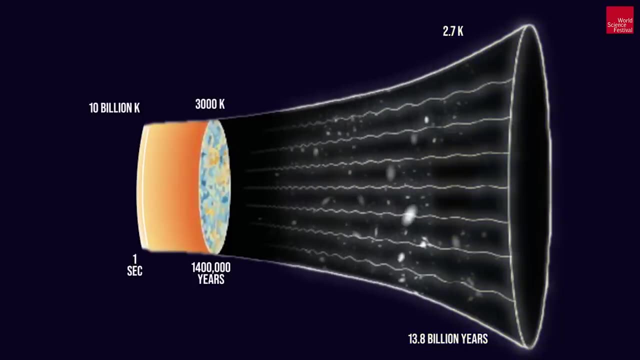 and vast the universe is. today That has overall temperature of 2.7 Kelvin, so it's super, super cold. And then we extrapolate backwards in time in 13.8 billion years, then we see how hot it was. We see the one-second mark. 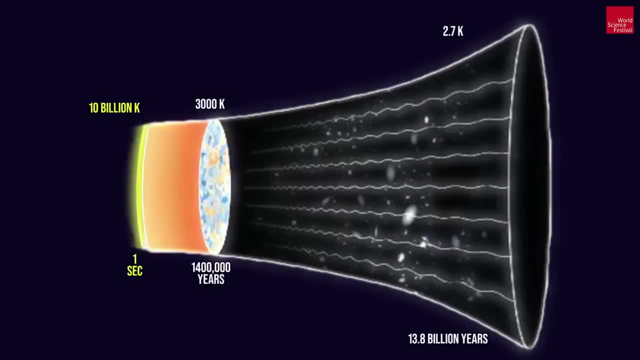 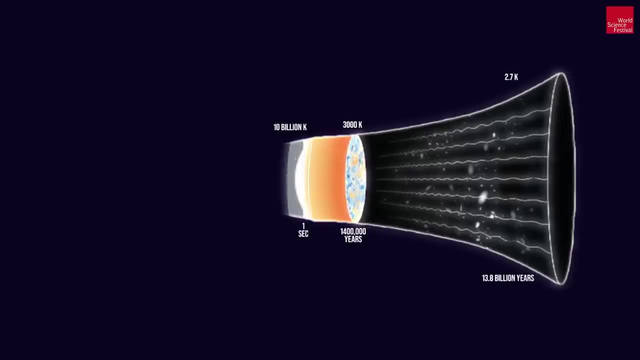 so one second after the beginning of expansion it was 10 billion Kelvin. But what you're saying now is- it's actually worth looking, when the next slide comes- by how much further in energy or in temperature we would have to extrapolate backwards from the first second mark. 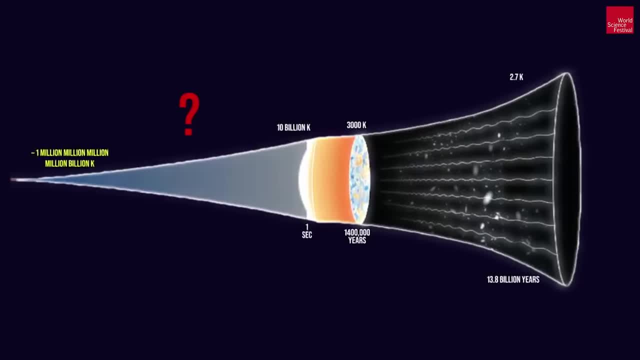 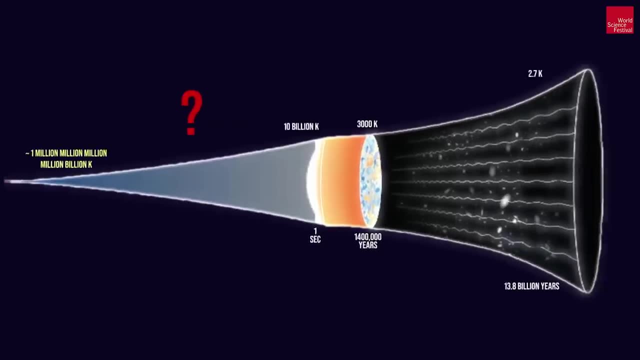 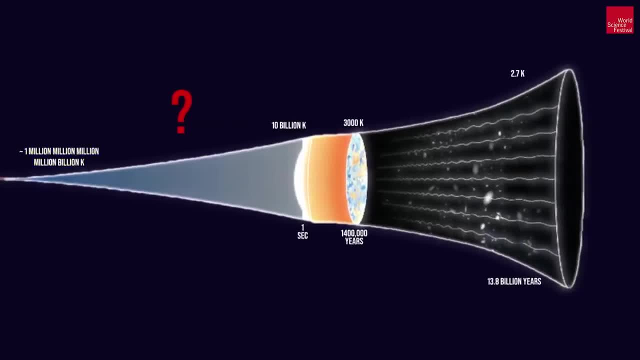 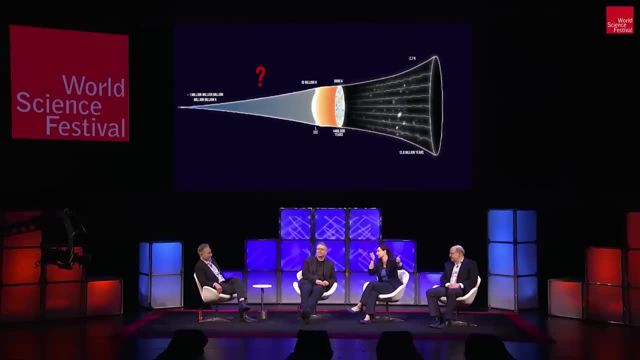 and the first second. So if you say, oh, it is just a little bit going backwards, no, that's just being thought wrong, Right, Okay, So you actually it's further away from the first second to whatever it takes. 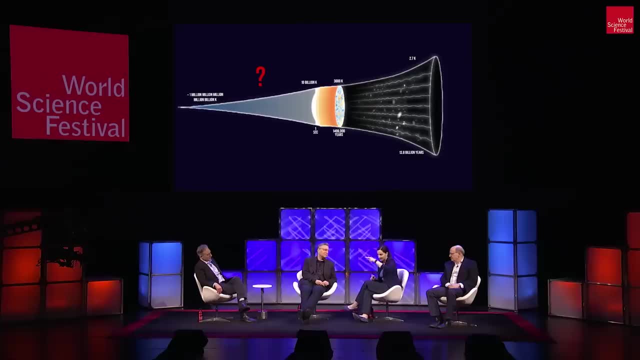 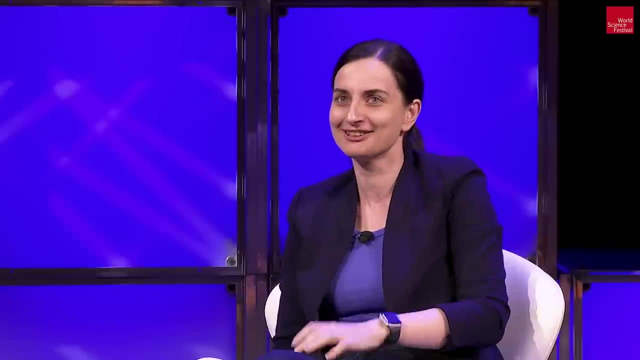 Plus, we don't have the theory. So maybe just the first thing, and now it will get to your question. Well, actually before, I love the direction you're taking this. Okay, Can we just follow on that? I think it's actually great. 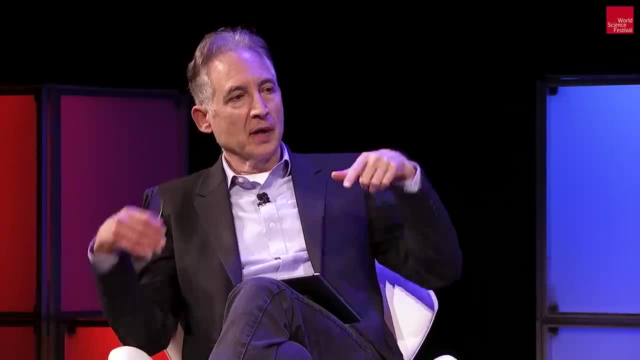 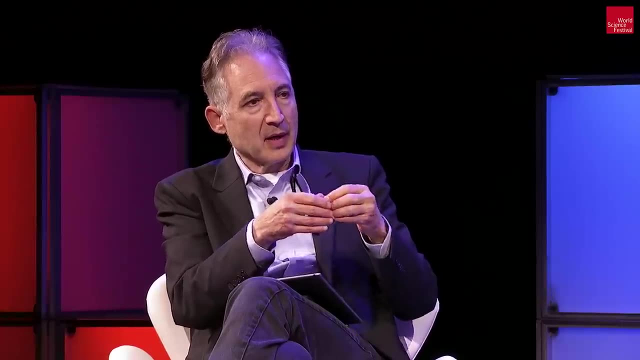 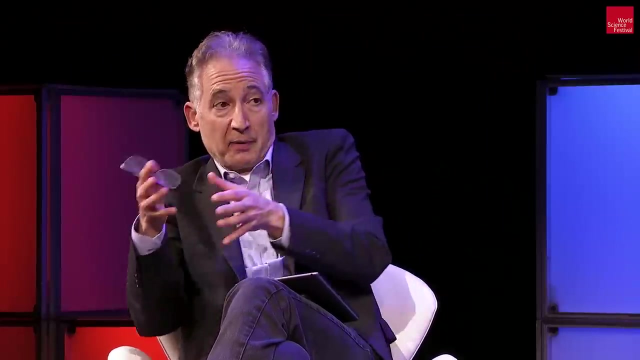 Okay, So you've now encouraged us to question the intuitive lore that just because we're expanding today, it had to have all come back together early on. So that raises the question of there may have been a singular time for a Big Bang. Perhaps there's something else. 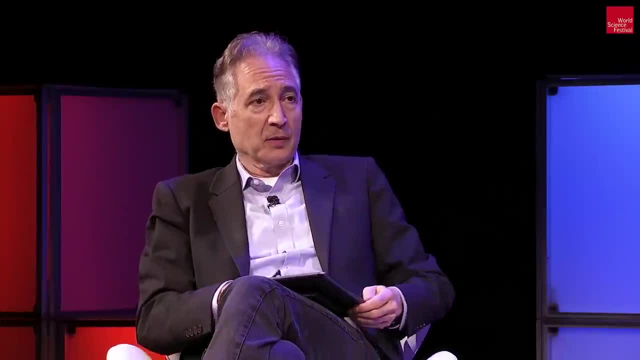 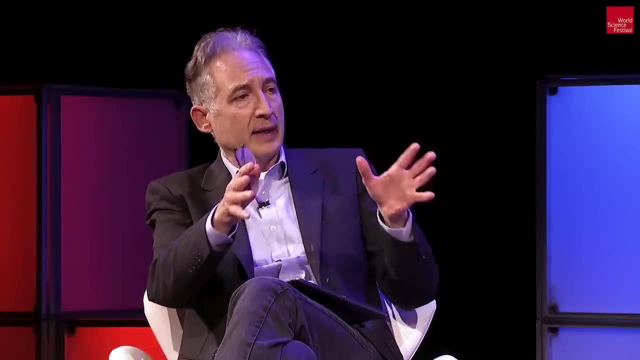 and you're going to suggest something else As we go forward. not to spoiler alert here, but I'd like to continue on the more traditional trajectory in order that the new ideas that you're going to suggest have a counterpart to bounce off of. 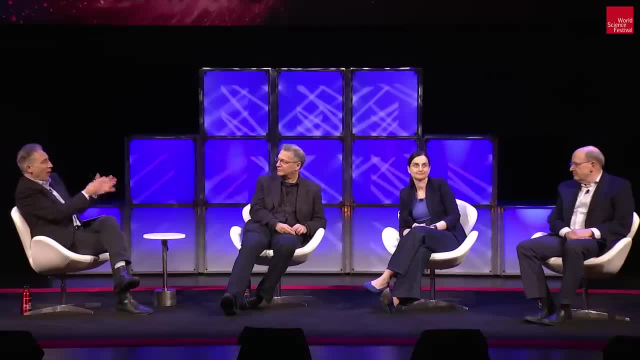 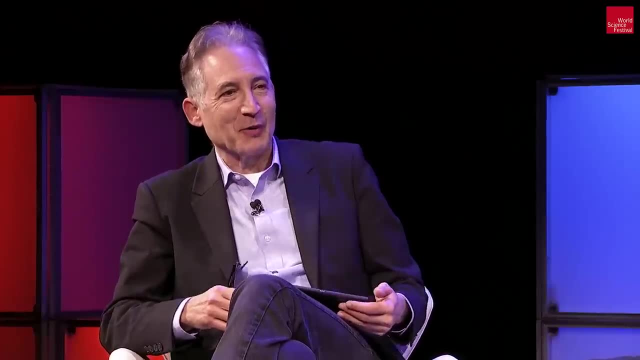 especially because, Paul, you're one of the architects of the other theory that your new theory is going to try to undercut. So it's a very, you know, interesting situation that we find ourselves in. So when it comes to ideas of the Big Bang, 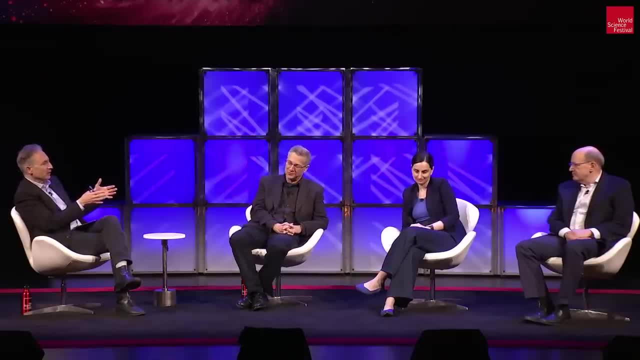 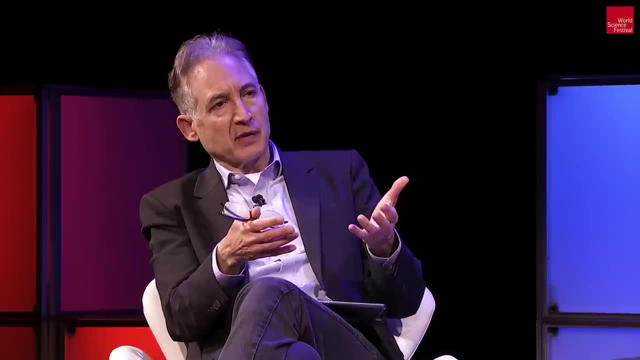 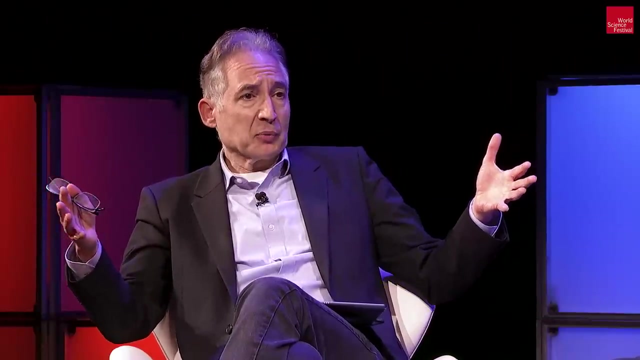 if there was one. certainly one of the things that we would need to explain is what drove the outward expansion, And certainly the approach that you developed. inflationary cosmology, at least in principle, supplies an answer to what that outward push would be. 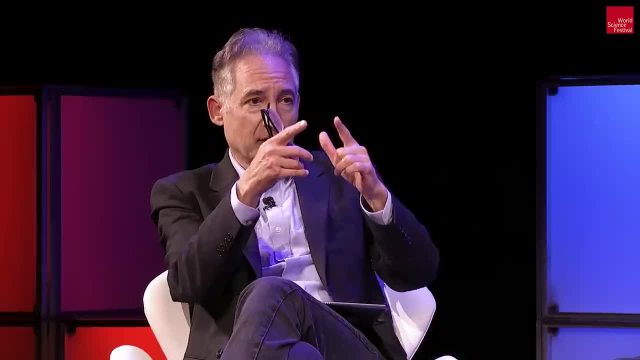 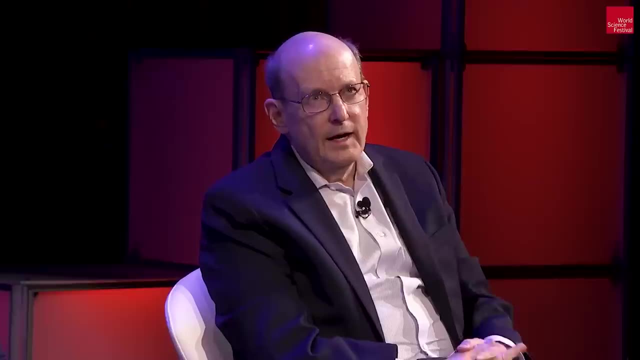 So, if you're willing to play along on the old theory that you developed, that you no longer are in favor of, if you could just give us a sense of what the inflationary theory says. So what was the reasoning behind the inflationary theory? 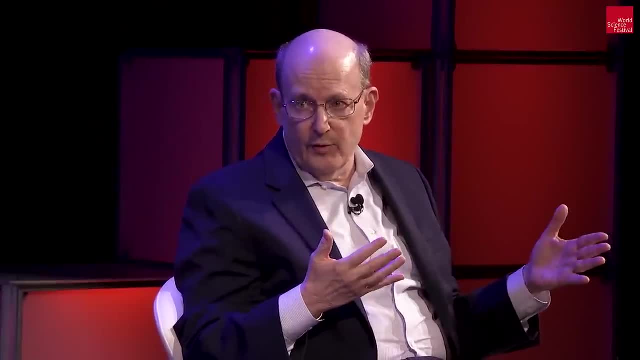 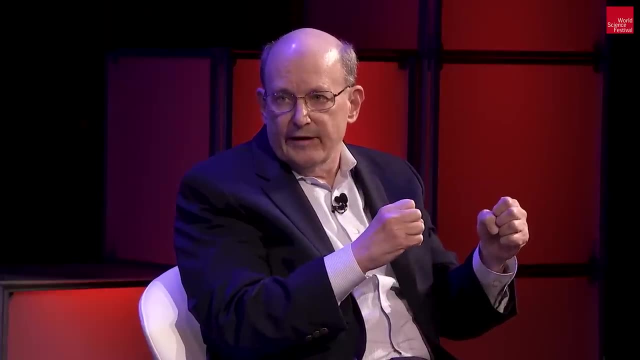 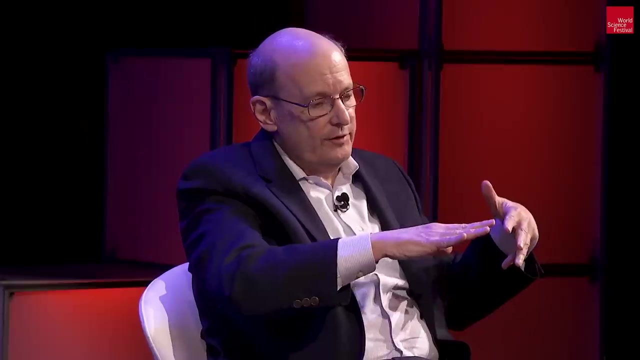 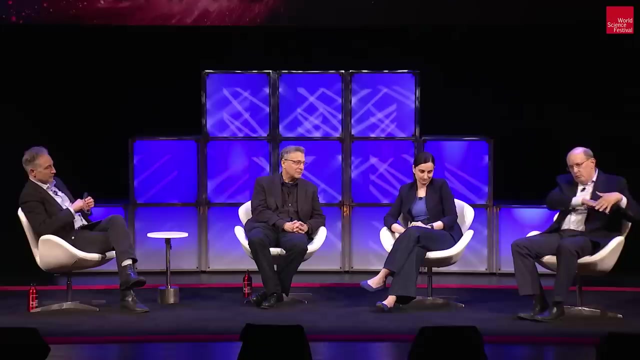 Well, the problem that the Big Bang presents to us is that, as the universe first emerges, we expect there to be large quantum effects that create wild variations in space-time itself, wild variations in the distribution of energy and radiation, and also wild variations in the curvature of the universe. 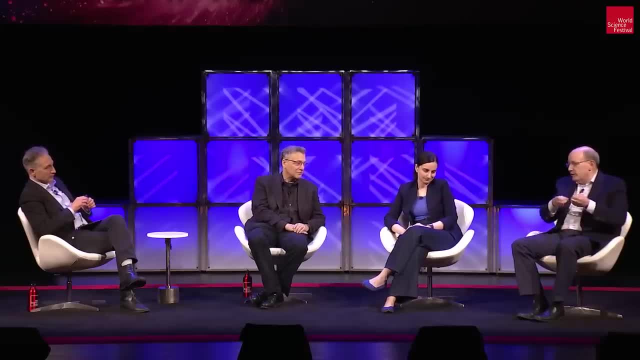 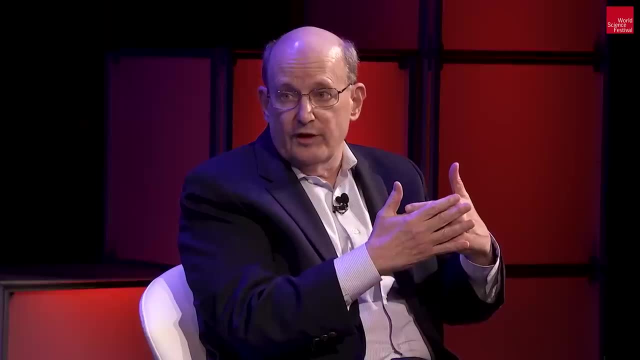 Yeah. So if you simply went from that point forward, like the diagram was suggesting, you'd expect by the time you get to the one-second mark you'd have a universe that's still very curved, with a very wild distribution of matter and energy. 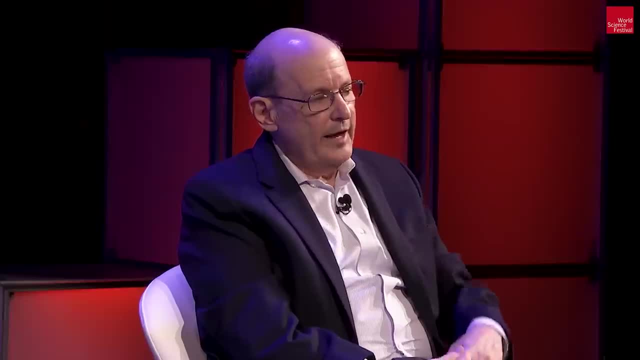 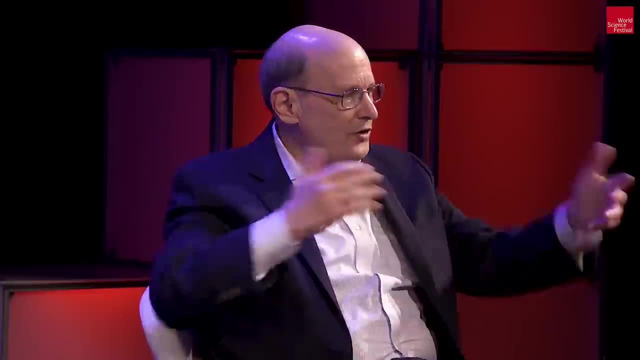 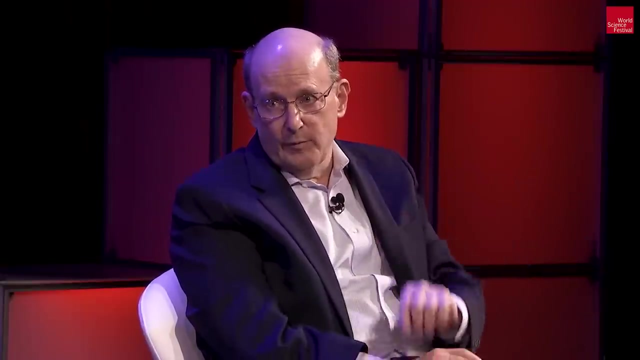 And remarkably, that's not the case. So whereas in general relativity the least likely thing to have is a smooth and flat universe, It should be very elastic and wildly varying. We actually need to explain why. when we get to the one-second mark, 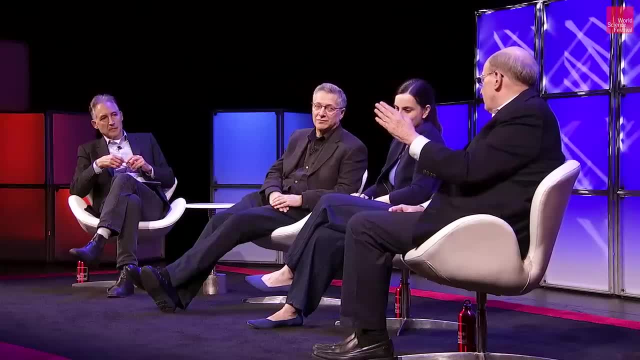 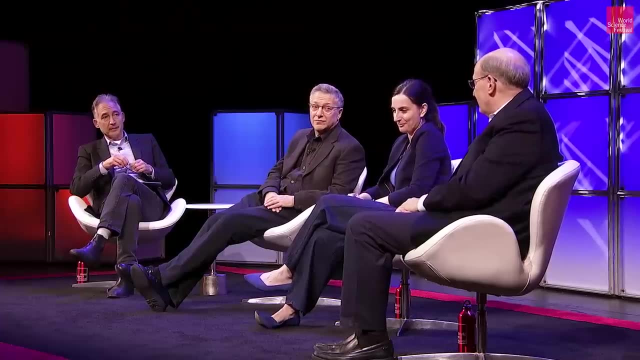 something somehow has to have made it smooth and flat, And observationally we know that at that mark Right. And now we can say that We couldn't say that in the 1980s when inflation was invented. But now we can say: in fact, 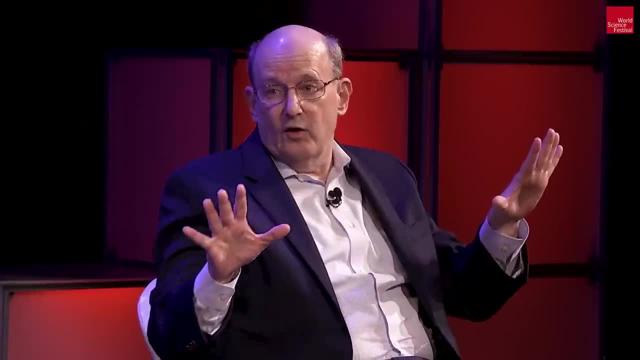 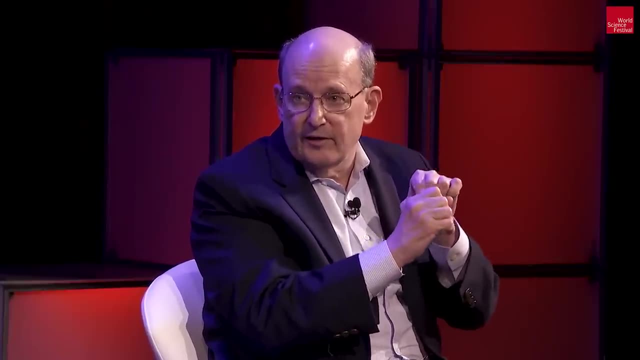 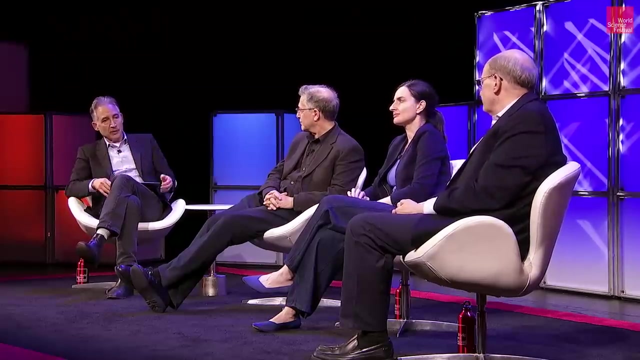 looking at the microwave background, we actually see that large-scale homogeneity compared to the size of the part of the universe that would be in causal contact at that time that could possibly have. So we're going to come to the microwave background and the issue of homogeneity. 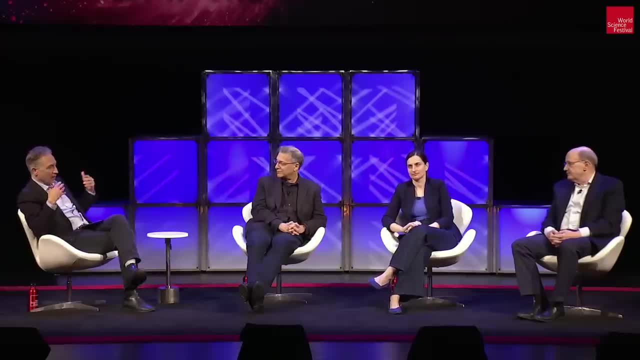 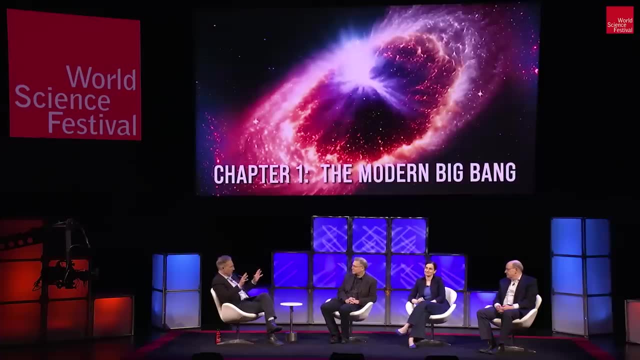 and the temperatures being uniform on scales that are hard to explain. But can we first, Peter, just give us a thumbnail. What is the cosmic microwave background radiation? It gives me a vital tool in the conversation, So as the universe develops at a certain point, 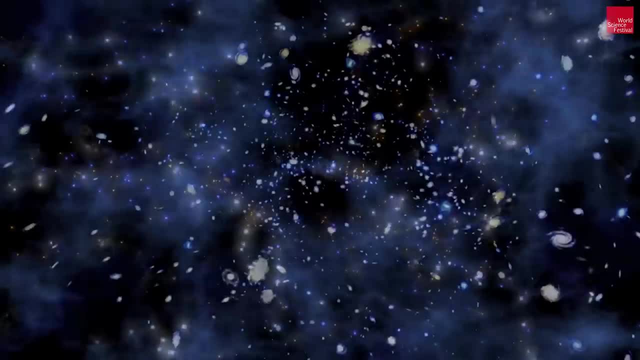 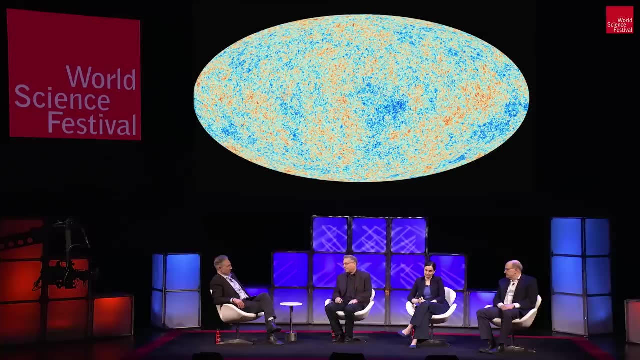 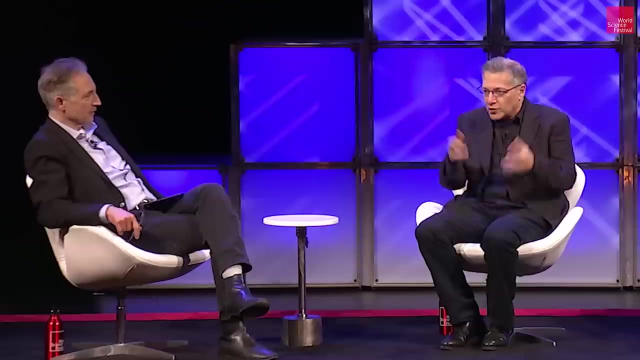 the electrons and the light begin to interact and it begins to. You can see the echoes of that radiation even today. I mean it's somewhere in the television channels- Channel 69, in the usual 1% of the static or so. So when you turn on, 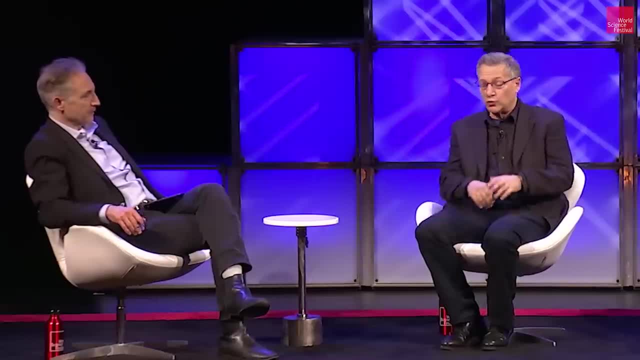 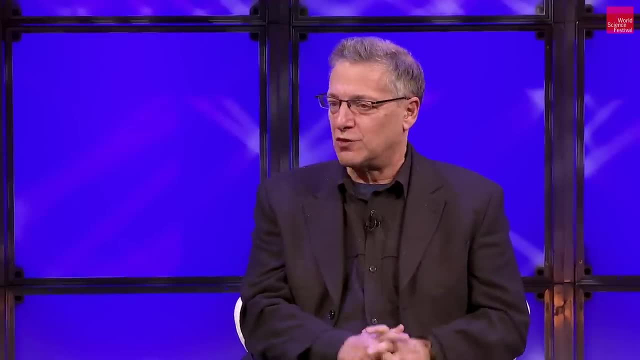 your television. you're seeing some echo of that, Yeah, And it can be studied much more finely. First it was discovered in the 60s and then it was. with satellites of increasing accuracy, We've been able to look at finer and finer structures. 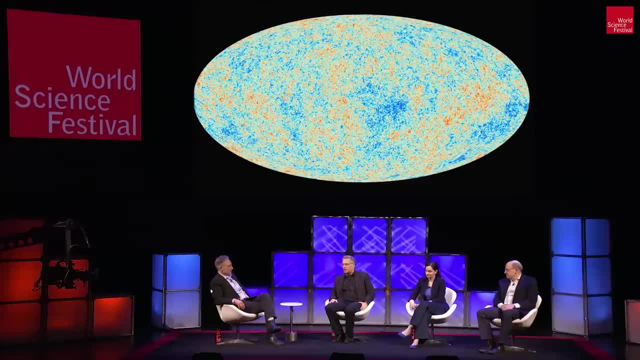 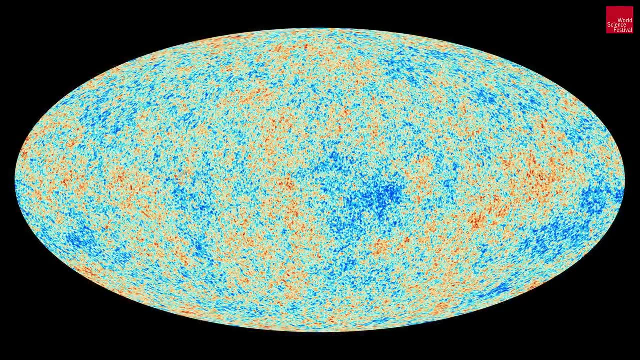 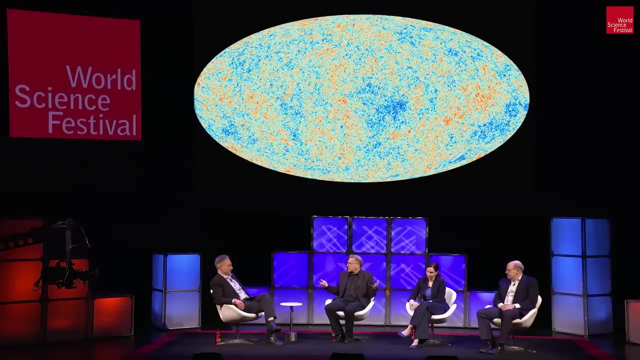 on this noisy background in the sky And amazingly enough, it looks pretty much the same in all the different parts of the sky and at different scales. And if the universe was developed in isolation from each other, then why should it have the same structure? 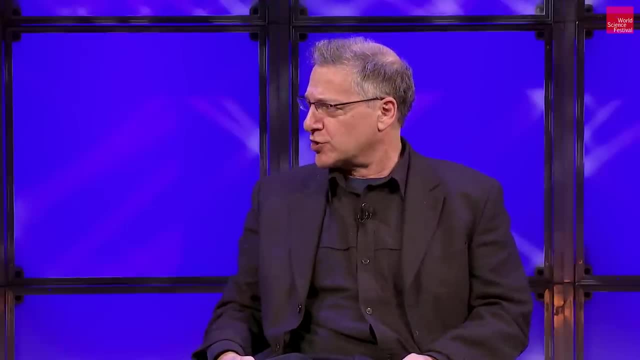 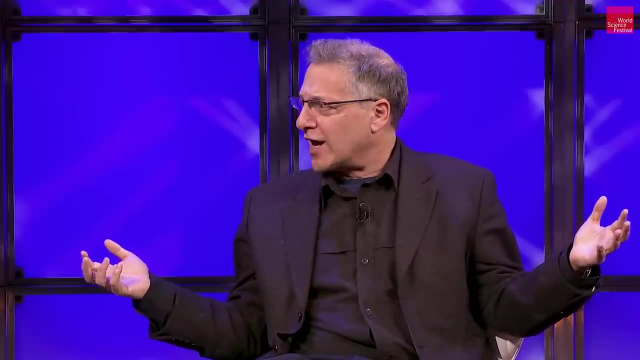 It's like we see this room: the temperature is about the same in different parts. We can explain that because the hot parts and the cool parts come to equilibrium, But if they've never been in causal contact, as would seem to be if we run the film. 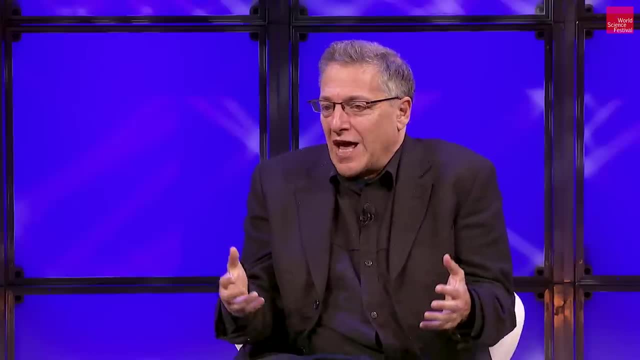 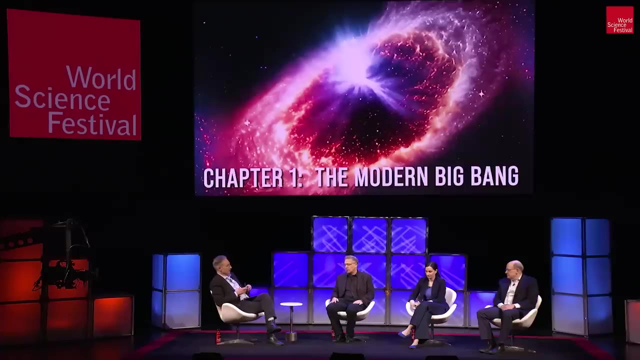 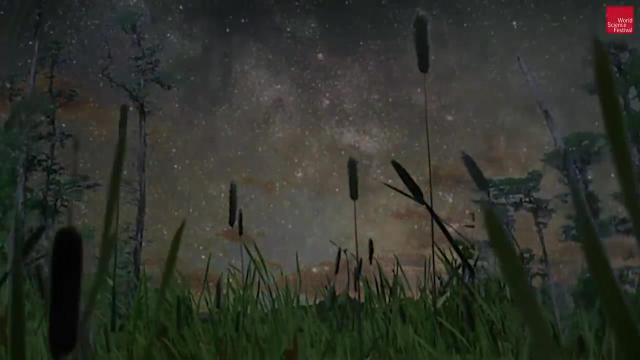 backwards from today, then it's a great mystery: How did they get to be so homogeneous in scale and space? So that's where perhaps we want to take up, Yeah, and we have a little visual just to emphasize that particular puzzle, If you imagine. 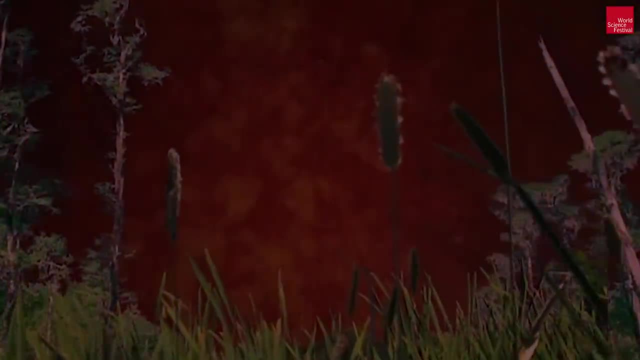 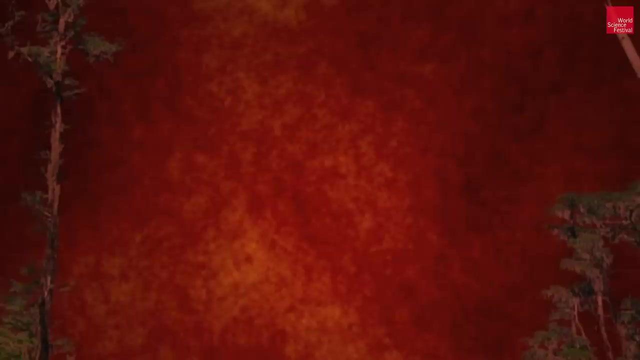 looking out from Earth and you took away all the stars and everything else that was contributing any other heat. what would be left over is the heat from the Big Bang that Peter was just making reference to, And the point is that temperature at widely separated points. 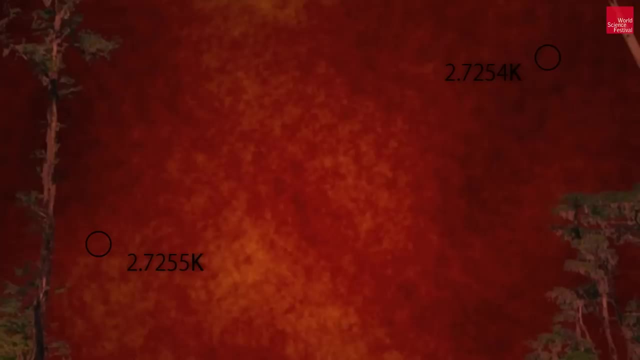 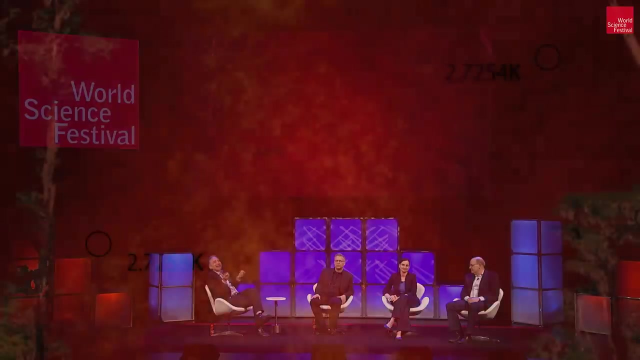 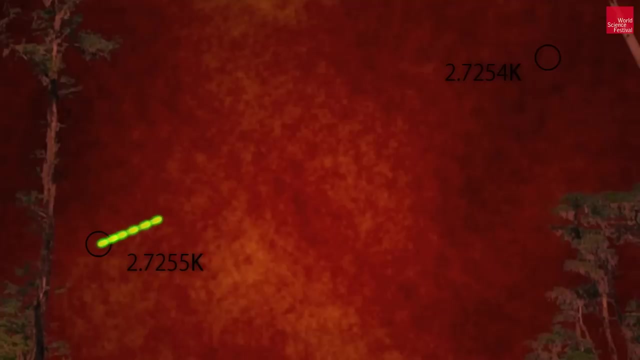 in this background, radiation is almost identical to fantastic accuracy, but yet if you look at a signal that attempts to establish contact between these widely separated regions, there isn't enough time for those distant regions to have communicated. So how in the world did they get? 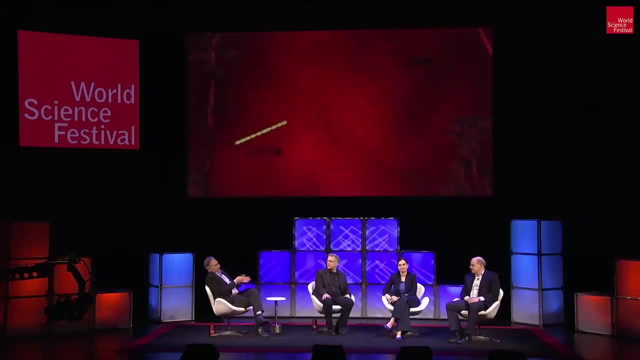 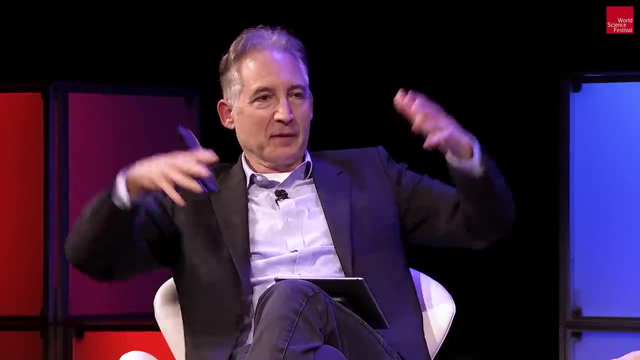 to the same temperature. So, as Ana was describing, we have this theory from early on of an expanding universe. It seems to match the fact that the galaxies are all moving apart, but there's a real issue that there are unexplained qualities of the world. 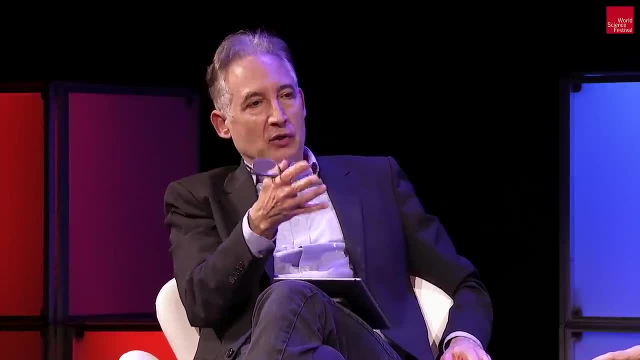 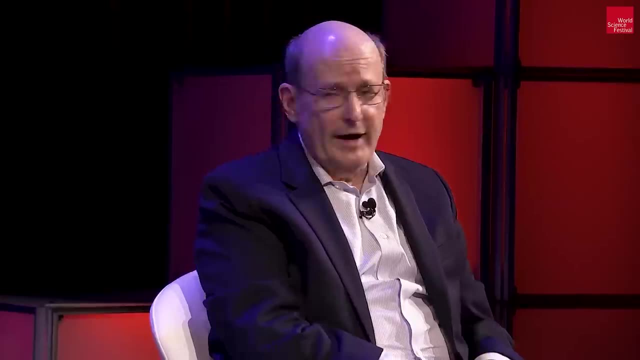 And Paul. this motivated you certainly in the 1980s, to try to solve that problem Right. so the first thing you might try to do as a theorist is try to keep everything in place that was there before, but add something. 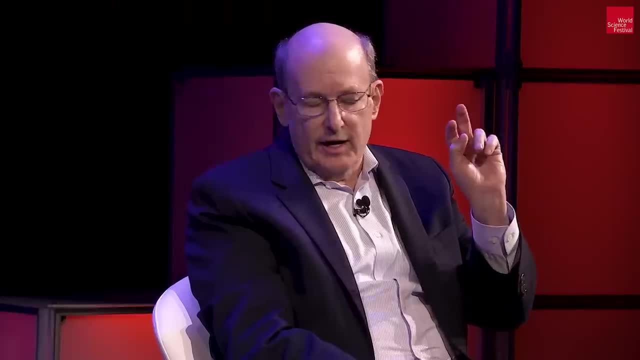 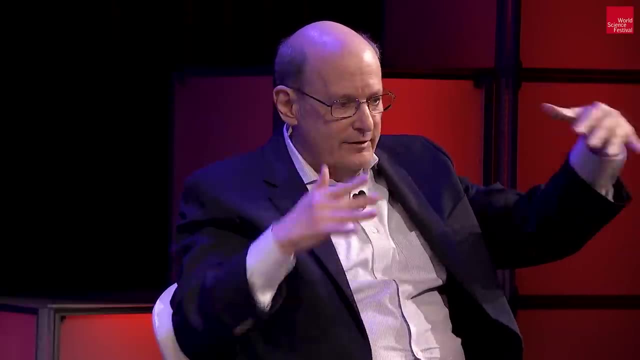 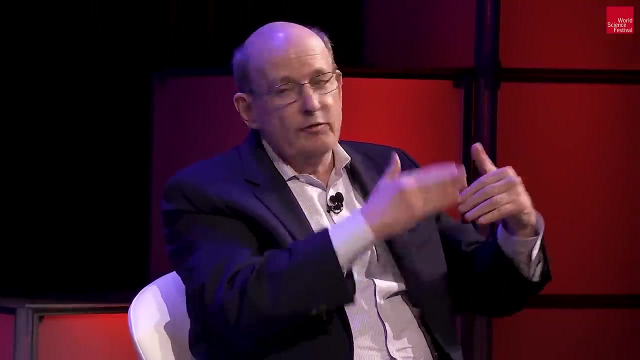 that would solve this problem, And that's what inflation, how inflation was introduced. So something between the Big Bang, out of which would come some wild universe, something that would tame it, that would smooth out, flatten the universe well before we reach the point. where the temperature was around the temperature of the center of the sun, when observations tell us it already was smooth and flat and the microwave background reaffirms it. So that was the idea. It didn't really explain why the universe started expanding. In fact, it needs some. 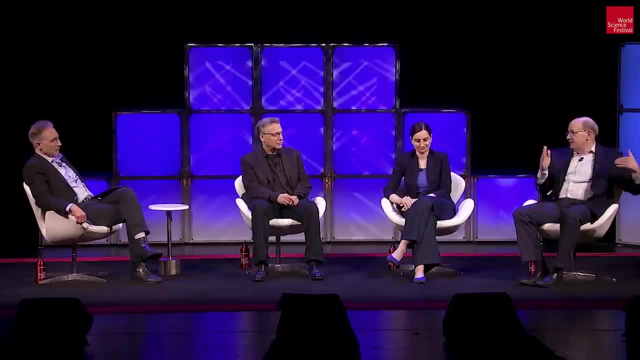 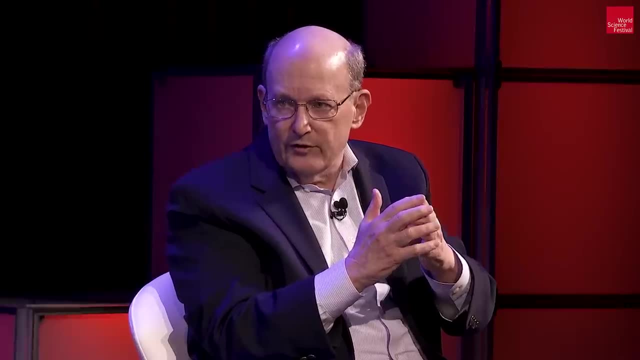 it's not a complete theory inflation itself. It needs something before it that explains how you got to inflation. So the expansion already had to be happening for some reason in order for inflation to have any chance of ever getting started. But you did have a. at least in some versions. there's a mechanism by which the expansion is driven. If you have some energy that gets uniformly distributed through a patch of space, then even in Einstein's basic general theory of relativity it gives rise to repulsive gravity. 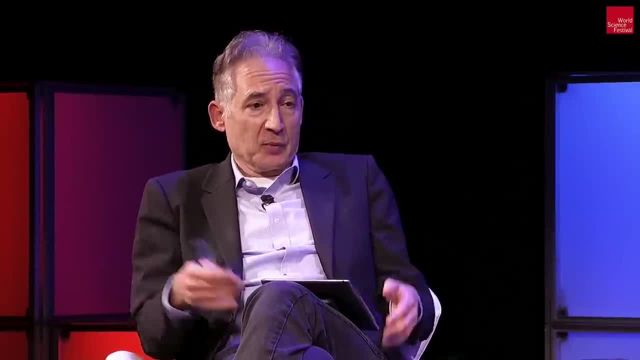 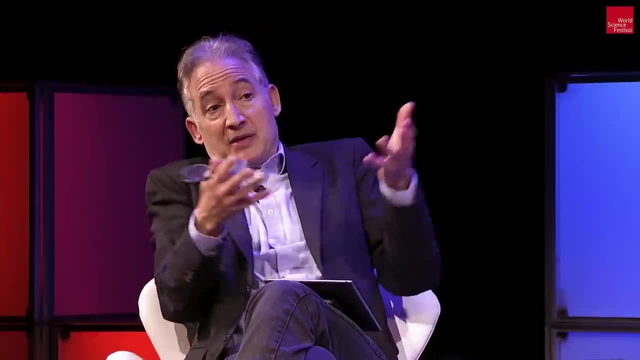 something we've never experienced in everyday life, because we only experience clumpy things like tables and chairs and planets and stars and so forth. But in Einstein's theory you leverage the fact that it can have an outward push. It can accelerate the expansion. 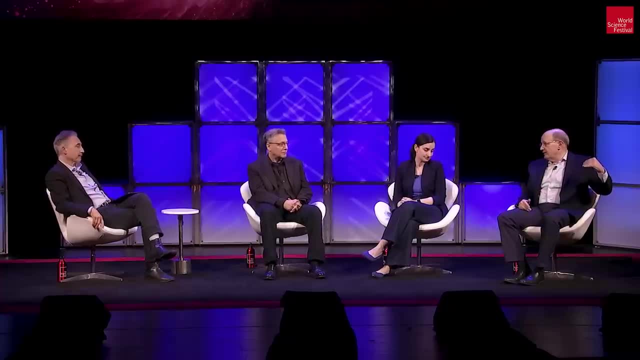 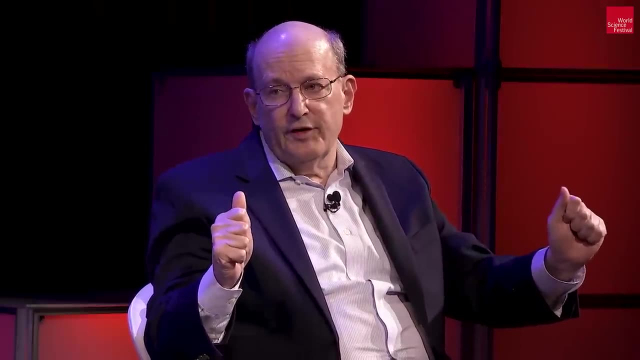 Which accelerates the expansion Compared to what you would have gotten straight from the Big Bang. Yeah, And the concept was that if you can accelerate this expansion, this would take a very uneven universe and curvy universe and smooth and straighten it out. 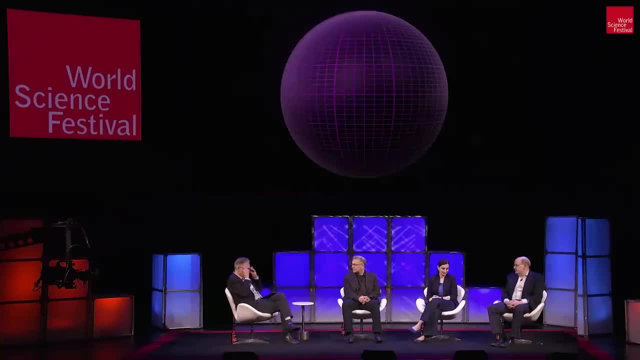 That was the concept, But before we go on, can we just show a little visual on that, because it's sort of a key idea. So if you imagine just having a shape that has some curvature to it, a simple shape that looks like a ball. 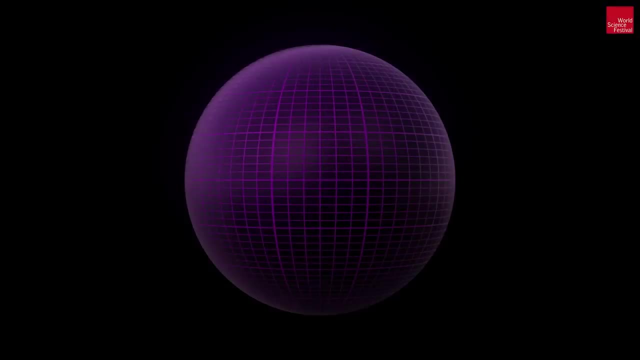 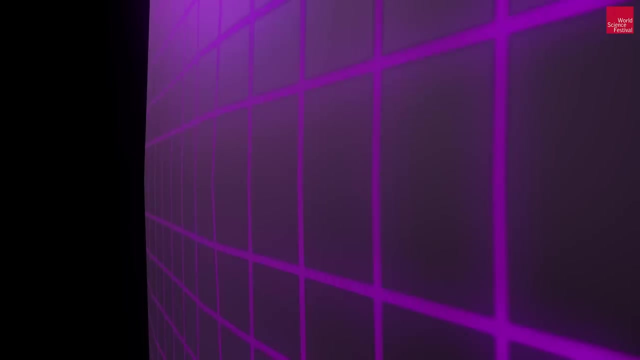 but just sort of a storybook version of it. if we make this bigger and bigger through rapid expansion, it looks flatter and flatter, And so even something that has some curvature. that's why we think that the Earth was flat, you know, 10,000 years ago, right? 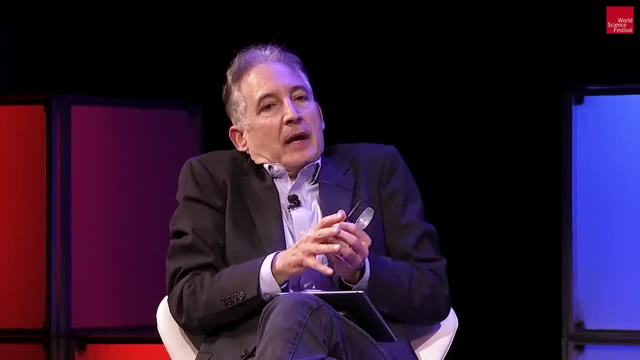 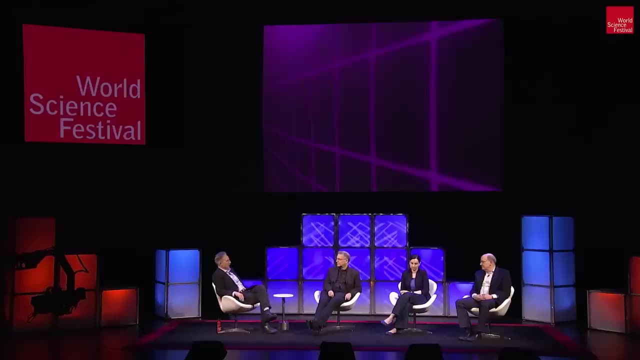 Because it does look flat locally. So if you can have this accelerated expansion, your theory, together with Alan Guth and Andre Linde and your student, I guess Andreas Albrecht as well, you have this proposal for how you get rid of the wild undulations. 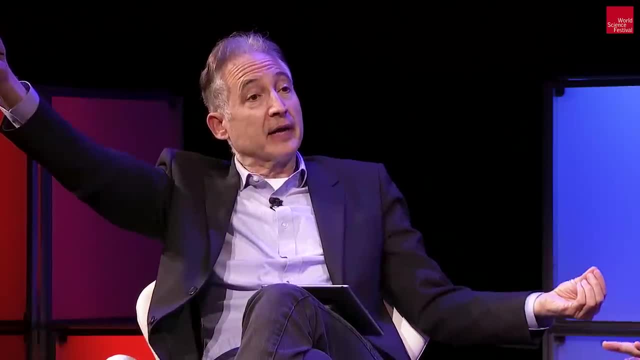 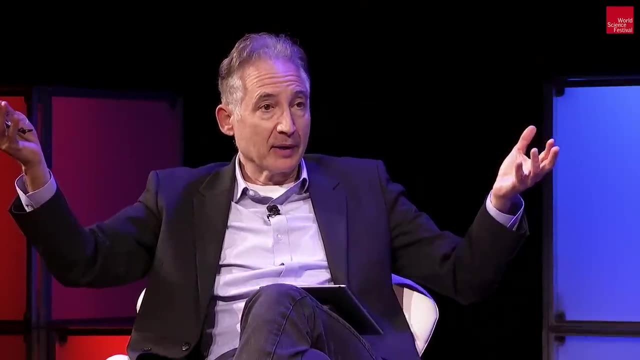 get rid of the curvature, as well as find that these distant locations would be able to be in causal contact early on, before they got rapidly separated. So it starts out really small and, in equilibrium, expands faster than it would have under the Big Bang. 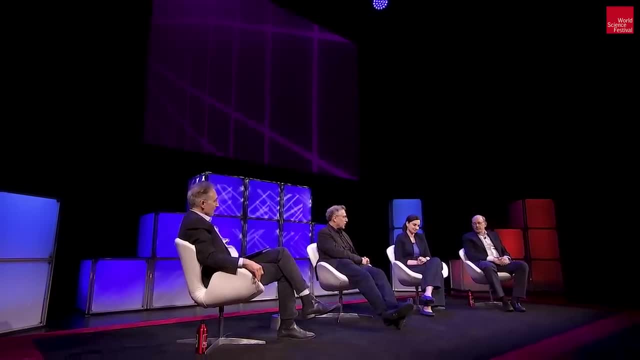 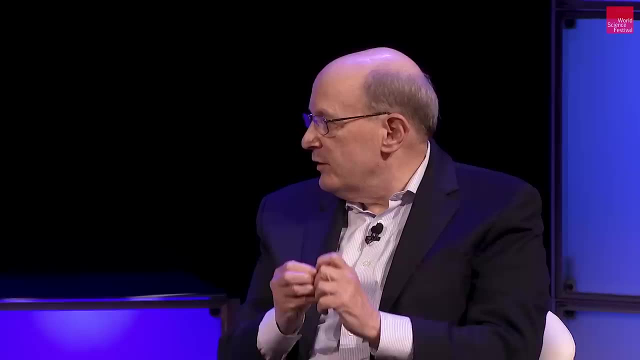 and then it begins its more stately march through time. Right, So it'll be important for our later discussion that embedded in our minds was the idea that the only way to smooth the universe was to make sure that distant regions were at causal contact much closer together in the past. 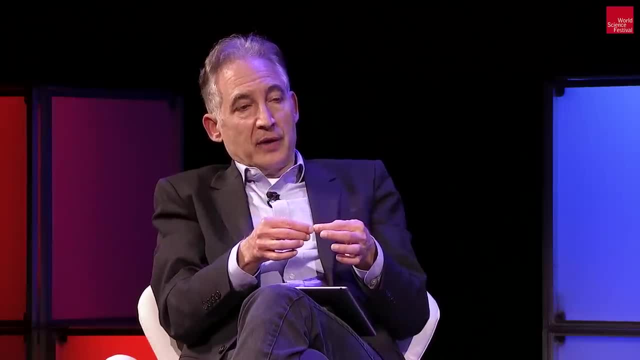 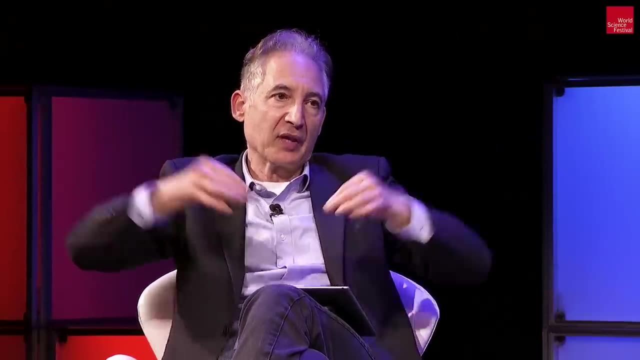 than the Big Bang model. So you got them really close together in the past in the inflationary theory, and then inflation sort of lets them catch up to where they otherwise would have been, so they can start closer together. So, Anu, you must have learned. 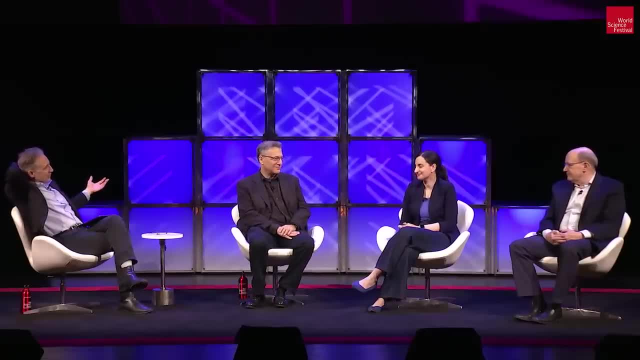 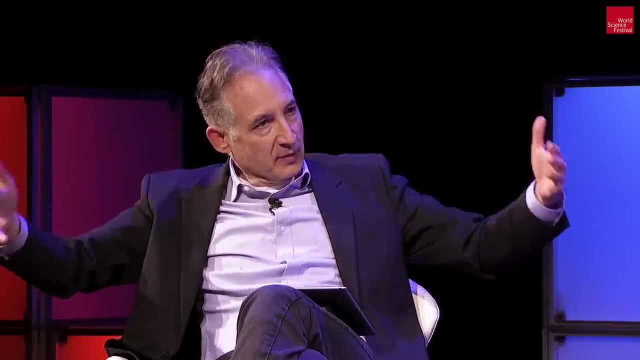 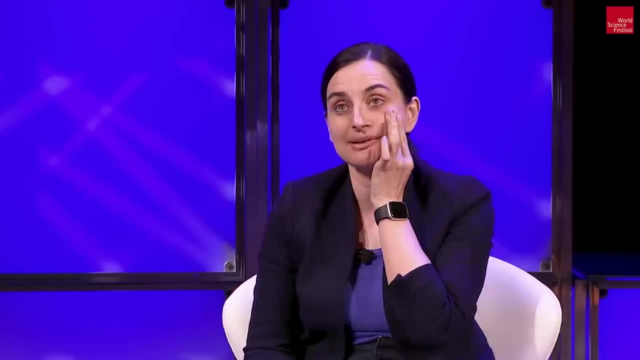 about the inflationary theory as a student. I mean, how was it presented to you? as you know, the theory, It was the way of thinking about how the universe evolved from the earliest fraction of a second. Yeah, you asked actually at the right time, because 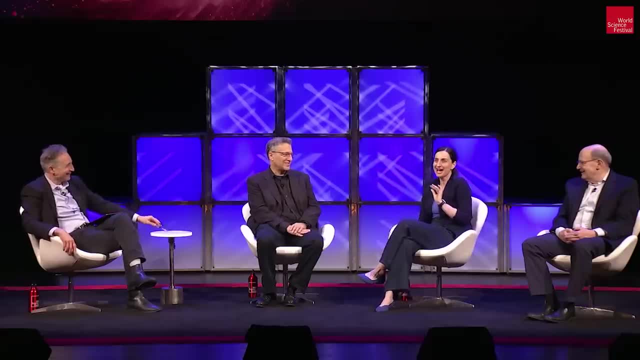 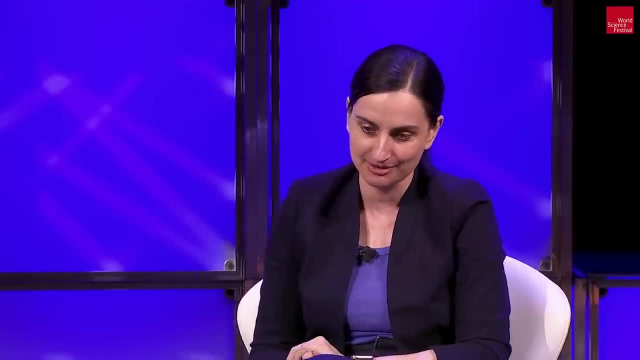 So I am younger than inflation, So I didn't have a chance to contribute to it and I'm younger than it. And so when I came to it the first time, it was over ten years ago. I was a student and it was textbook material. 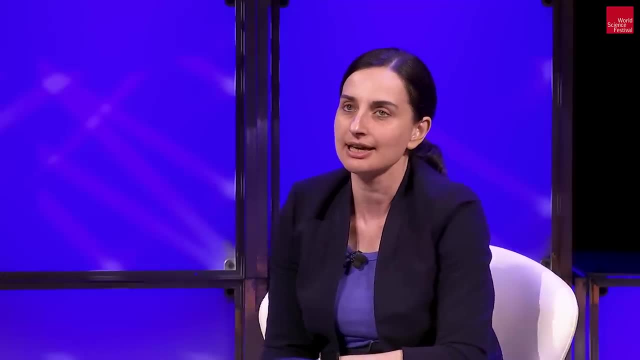 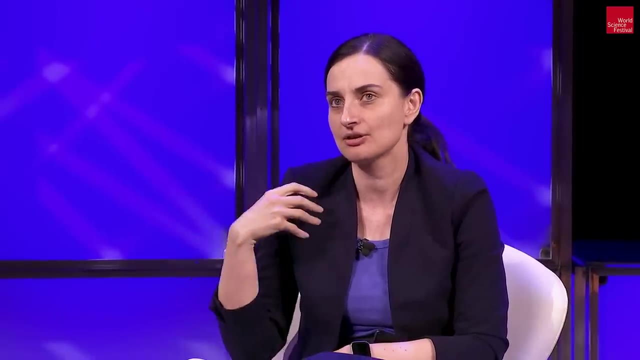 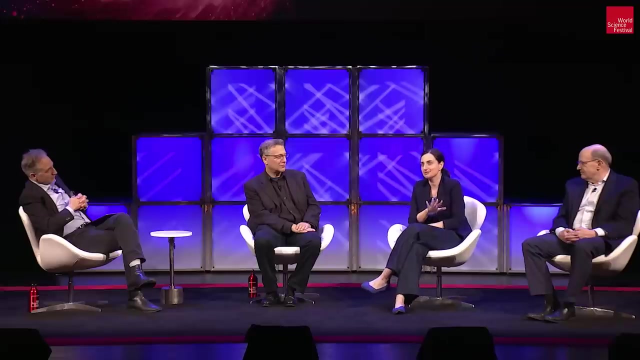 So I was fairly young and everything that was just said now was presented in class and not as a possibility, but as something that's been established. And what just Paul and I explained is something that I remember it, When I first heard about the theory. 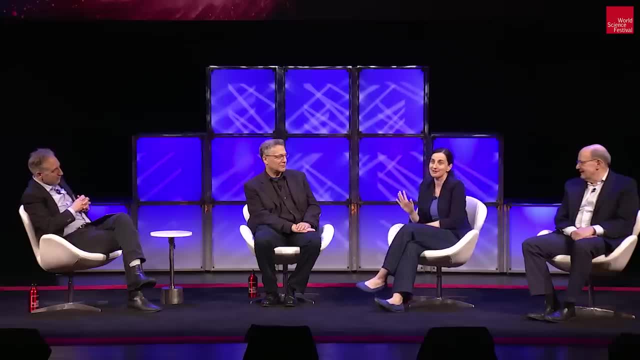 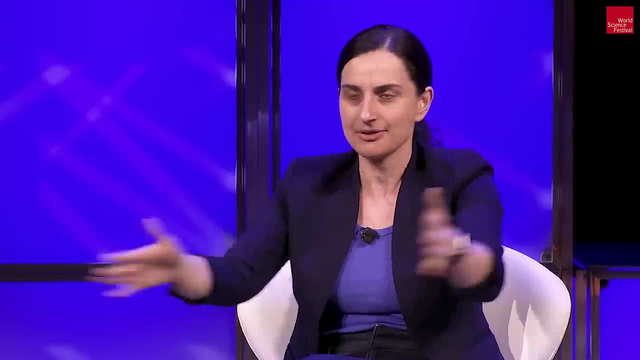 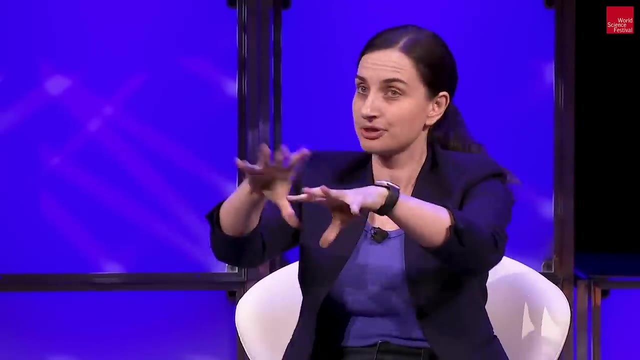 I just thought this is nuts. Because it's really nuts, because these guys tell me that they explain the smoothness of the universe by assuming it And that somehow sounds good. because, if you remember what Paul said, well, we just wanted to put things into causal contact. 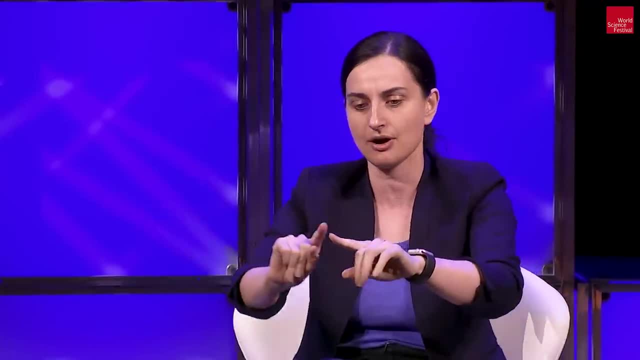 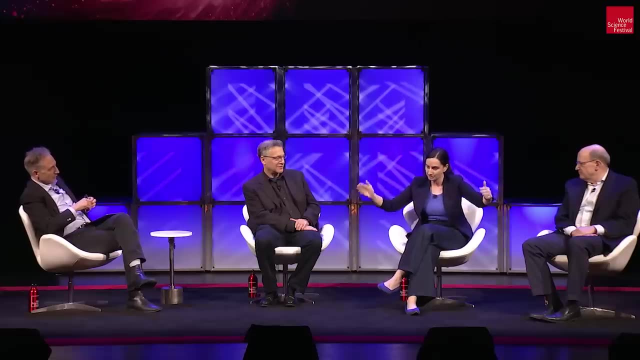 and how inflation operates is- and it is pretty clear how it's being taught- is that you take things out of causal contact very rapidly and then, when inflation stops and the expansion starts, a slow expansion, and these things come back again into causal contact. 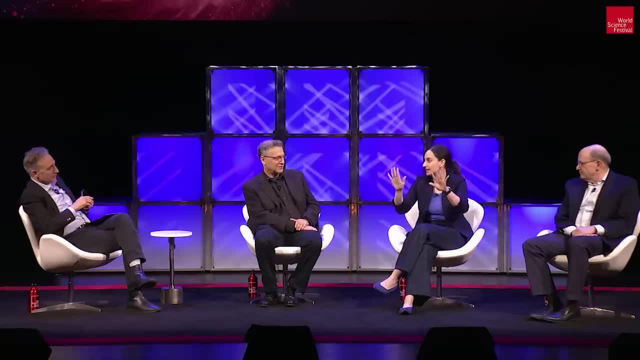 and it looks like that everything is the same, and the reason would be because it was the same. But you correct me. the idea was, and that's why we started with the Big Bang, that we have to explain this smoothness, this uniformity. 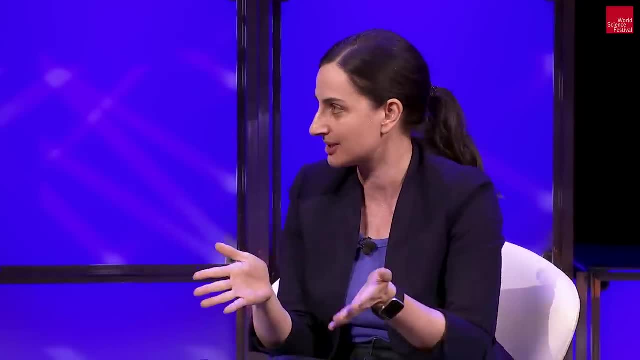 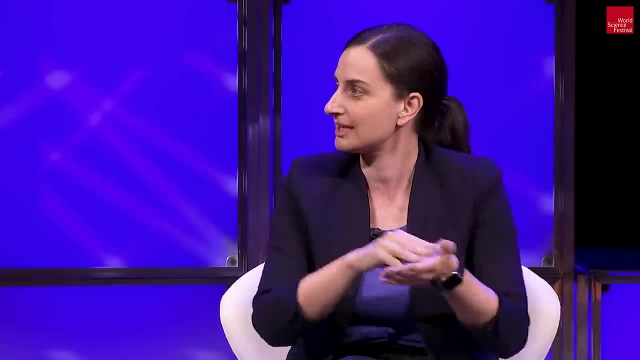 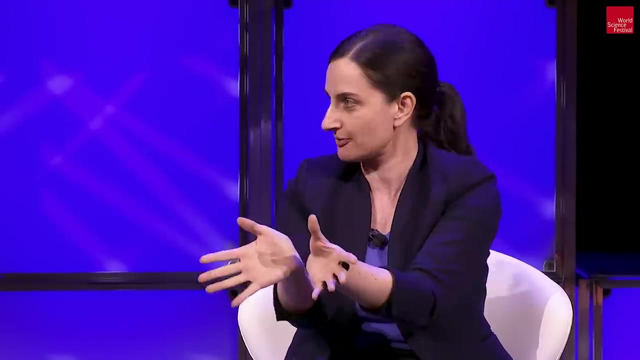 starting from arbitrary conditions, starting from conditions that quantum gravity would give us, And that's not smooth. It just seemed to me like these guys actually assumed what they want to explain and they just made a little trick by saying: okay, we assume that some part of space looked already, right? 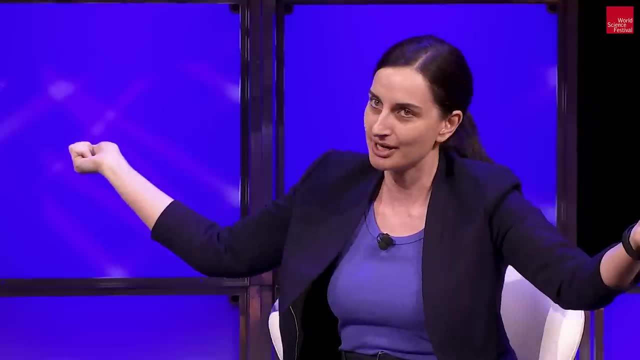 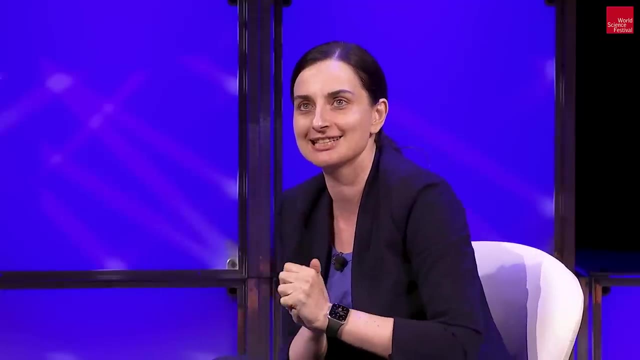 and we try to blow that up over many, many, many parts of space and then we somehow have the right answer, But- and this is actually what I came back to then later, 10 years later, to work on it really doesn't work. 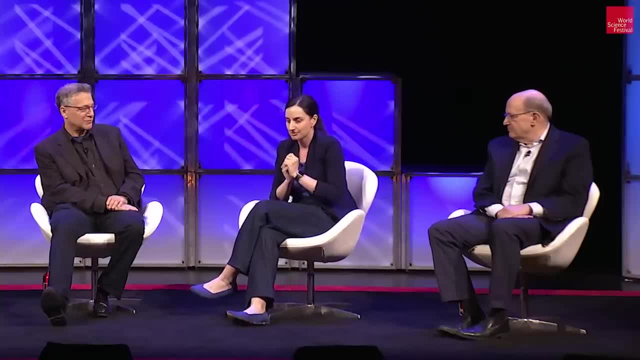 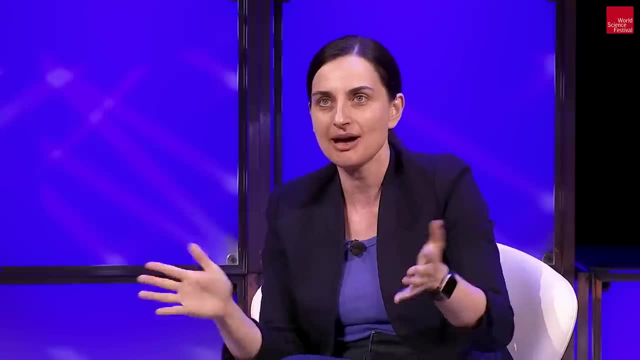 So it really was, and we will get back to that later. it really was the. you know my impression as a student. I don't want to work on this. I don't want to stay away from this, because somehow people came to believe. 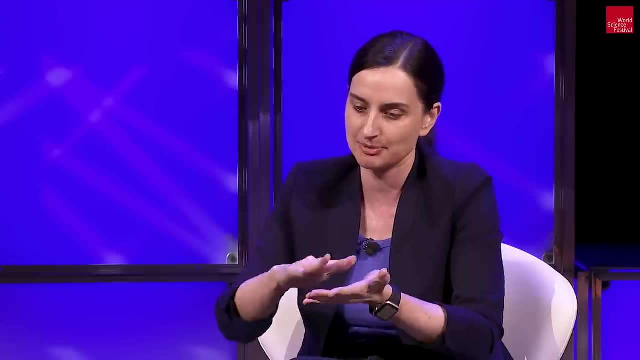 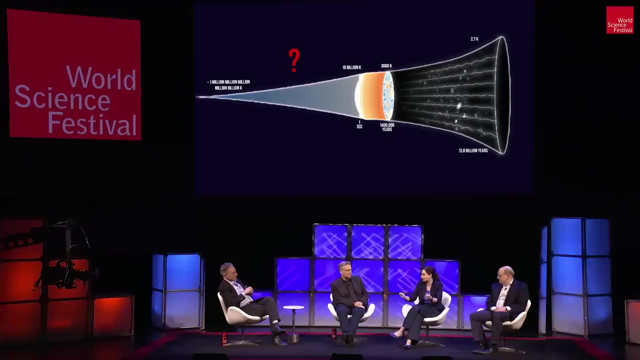 that if they start from the right condition then they can explain the same conditions on larger scales. But at the same time they also believe that somehow generic, that somehow comes out of the Big Bang. And for me this connection, this long connection, 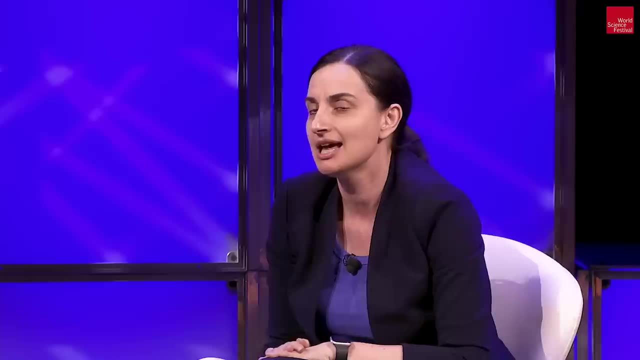 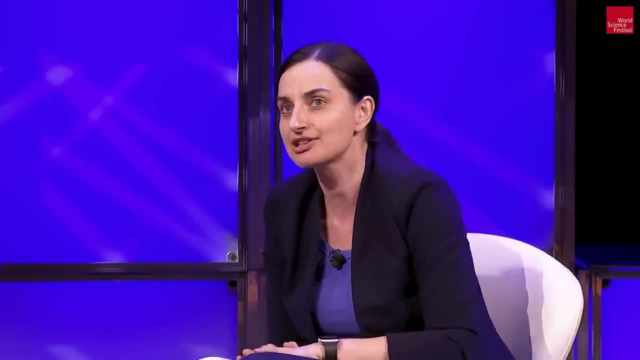 what's up there was always missing. So I decided I will not work on this, I will just do something completely different. I don't want to have anything to do with cosmology, And I actually really started to work like that until I met Paul three years later in Harvard. 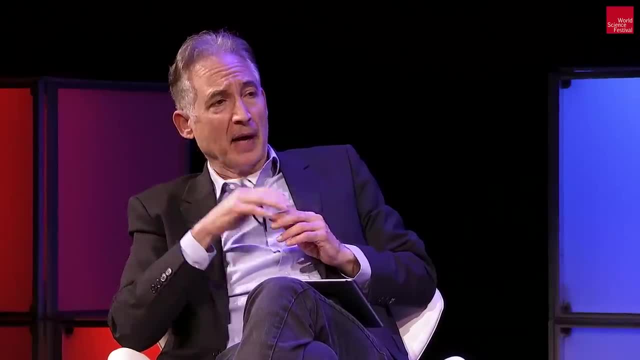 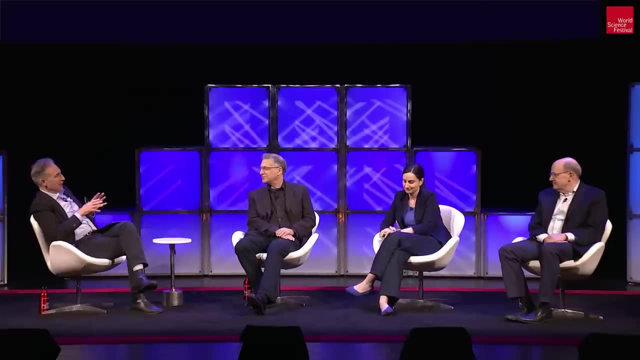 So we'll pick up your story of where you ultimately did come back to cosmology in just a moment. But, Peter, can you channel, if you would, just to give us an accurate snapshot of where people's minds are in cosmology today? 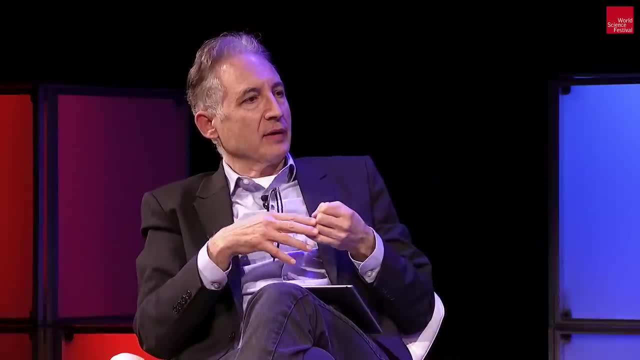 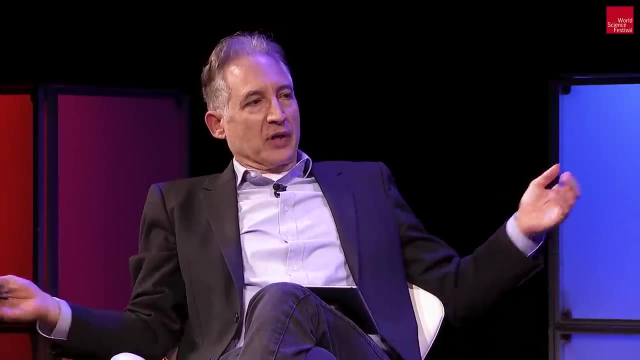 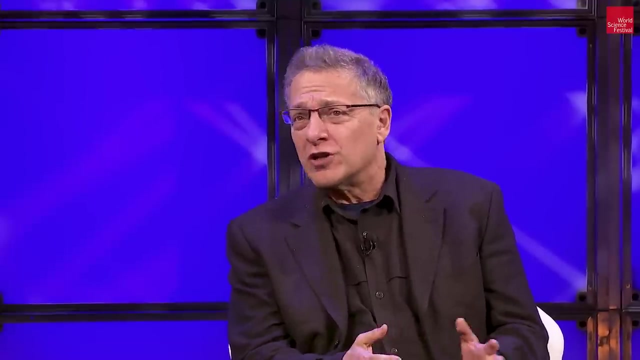 How is the inflationary theory- again, you know, developed by Alan Guth, Andre Linde, Paul and so forth? how is that viewed in the community right now? I'd say the majority view is that some version of it is right. 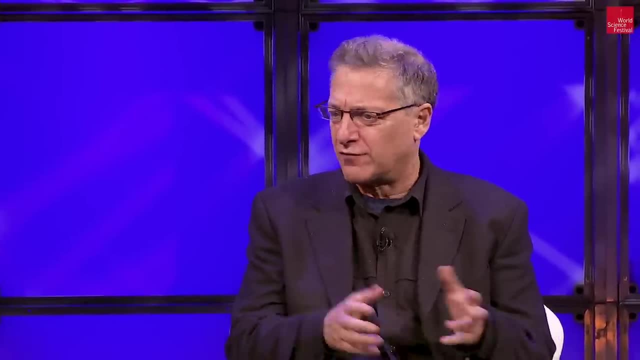 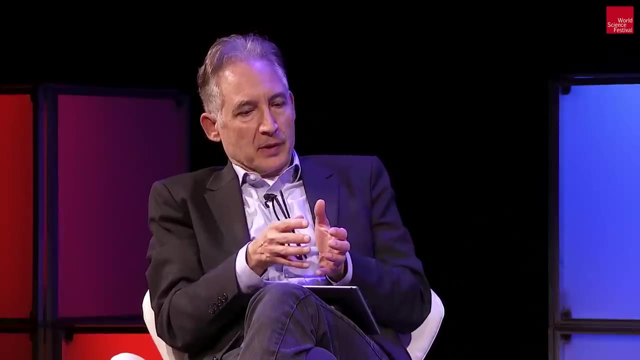 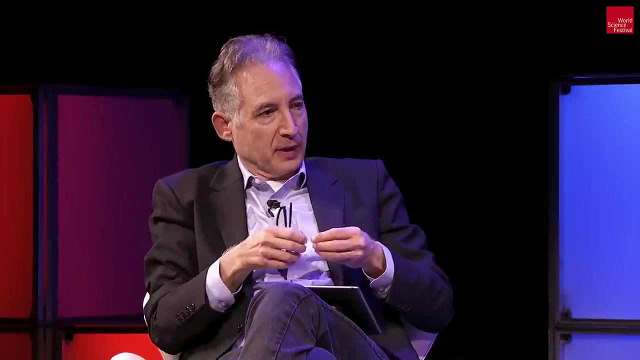 although we may not have the right model, There may be things that have to be adjusted or changed, but that basically something like that. So the general paradigm that there was a early period of rapid expansion that can do these tricks of bringing things into calls of contact. 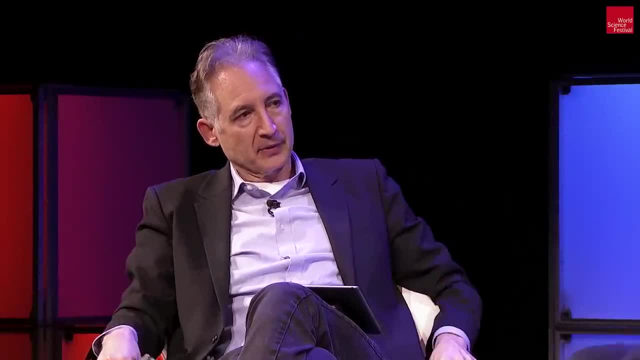 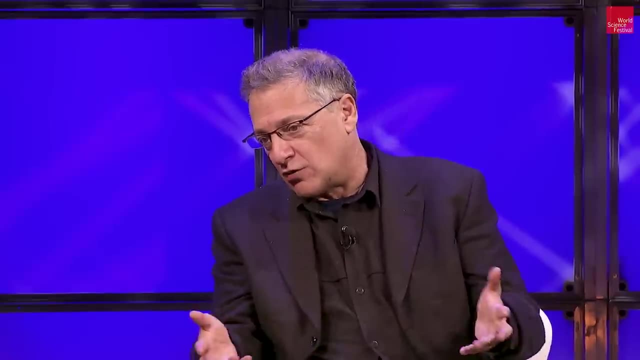 and pushing them apart. That's the basic picture. Yeah, I think what Ana said. it pushes the problem back towards the big bang, Yeah, And allows us to have an account for things like the causal connection that otherwise seems impossible to explain. 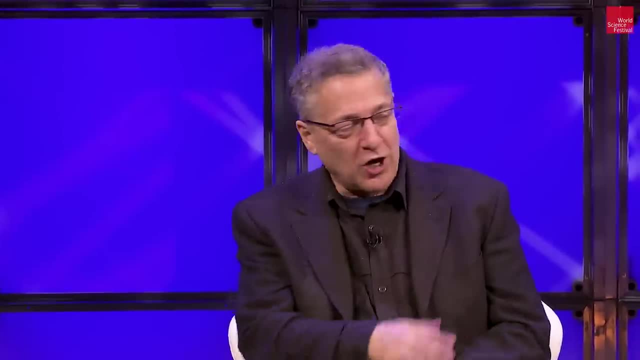 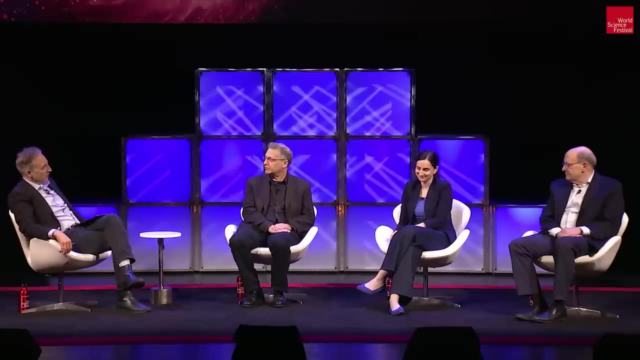 but it comes at a cost, and we'll be talking about that cost momentarily, And so I'd like to give you guys a floor in just a moment to go in a direction that you think may be more fruitful to filling in that part of our past. 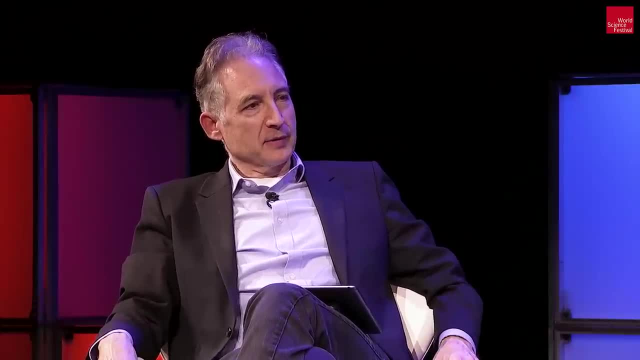 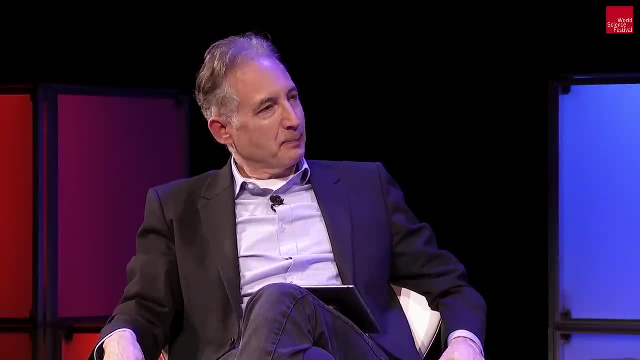 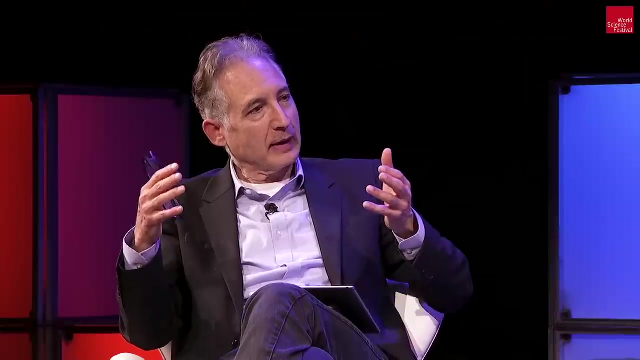 But again from a more sociological standpoint, I mean just thinking historically. is it common That there are periods of time where everybody thinks X but it's really Y? I mean, is that a rarity, you know? And how would we fit into that historical rhythm? 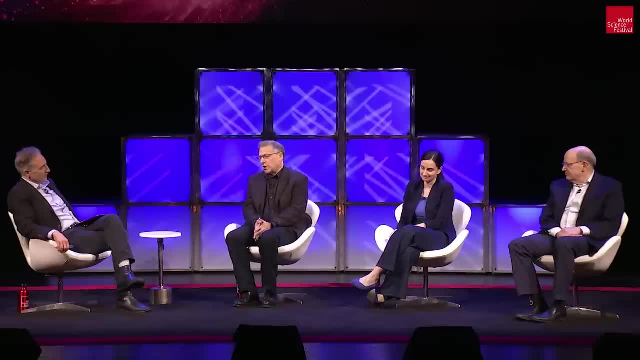 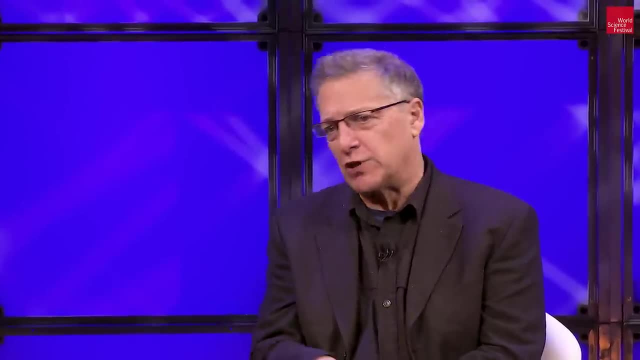 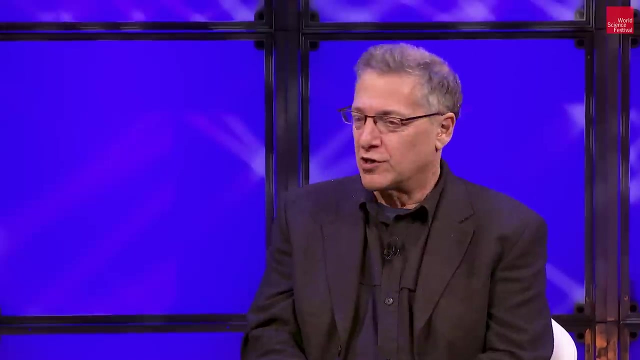 So I mean there certainly have been periods where the consensus was against special relativity, against general relativity, against it because it seemed philosophically impossible or it had too much mathematics. This was To the physicists, was unimaginably difficult. differential geometry: 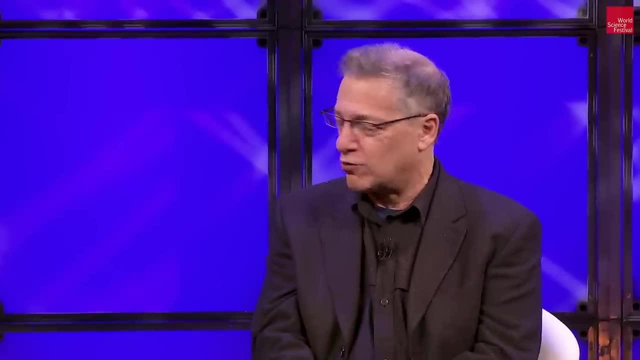 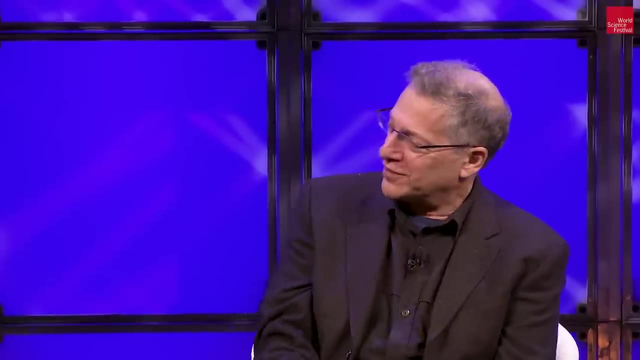 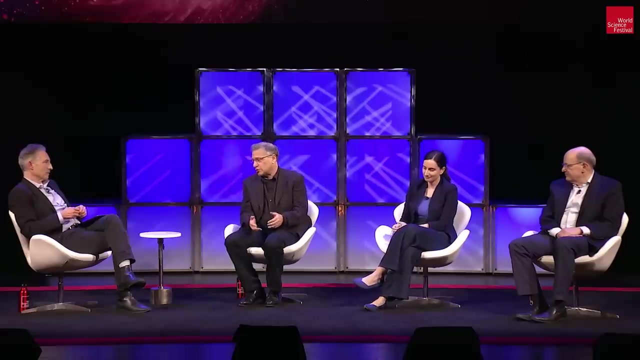 which is now taught as part of mechanics in the ordinary course of things, But at the time it was shocking. The development of quantum mechanics upset people hugely, including our, Einstein. There have been times when majority, So there certainly have been times when majority views have been disrupted. 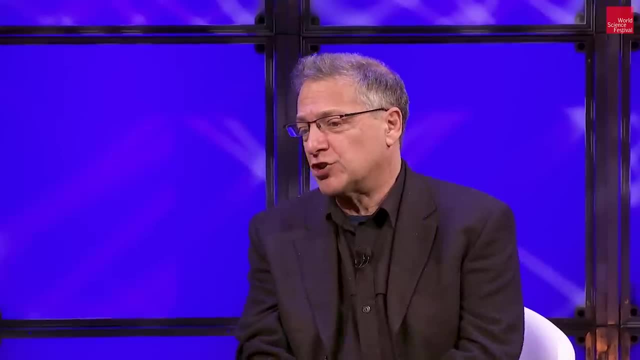 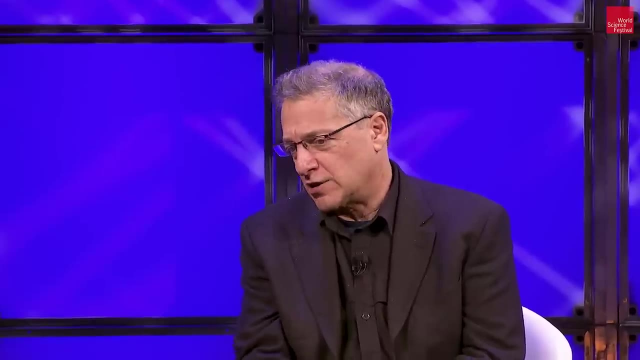 by alternative views. Once a view is established, though it's hard to guess, though it's hard to get rid of it without an alternative, And I think one thing that I mean just to anticipate a little bit is, I think, having an alternative. 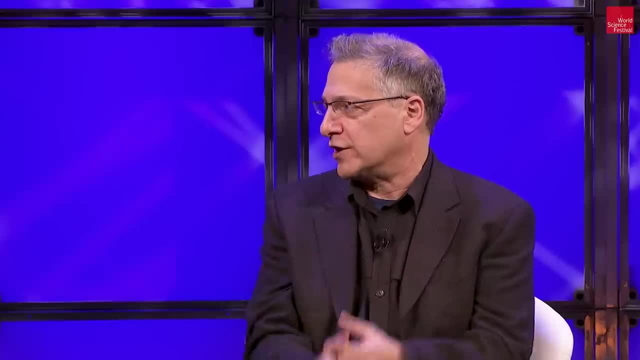 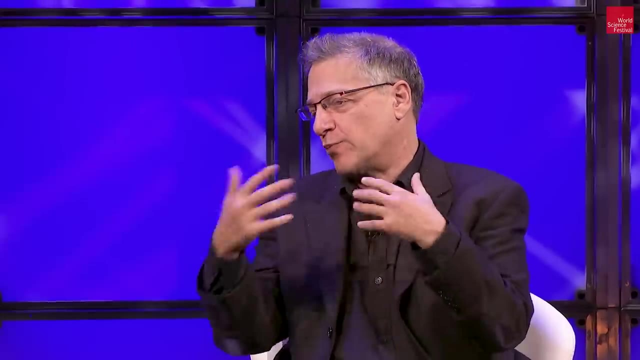 is always helpful to the articulation of where we are in science. So Einstein's theory for a long time didn't really have any alternative. Brands and Dickey came up with this alternative theory. I'd say it's a minority, quite significant minority of physicists. 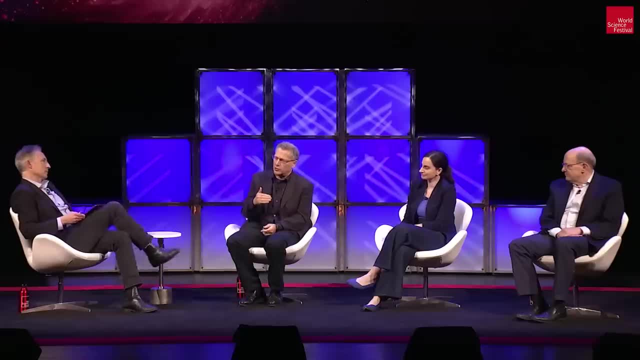 who today think that's the way to go. But the very fact that there was an alternative pushed people to think about testing, to look at what are the fragile parts of Einstein's theory and where can we push it with observation and inquiry in different forms. 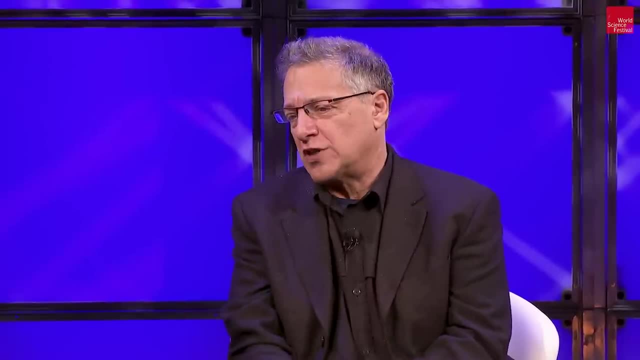 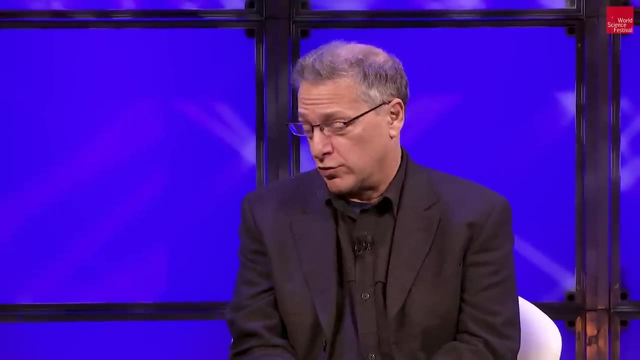 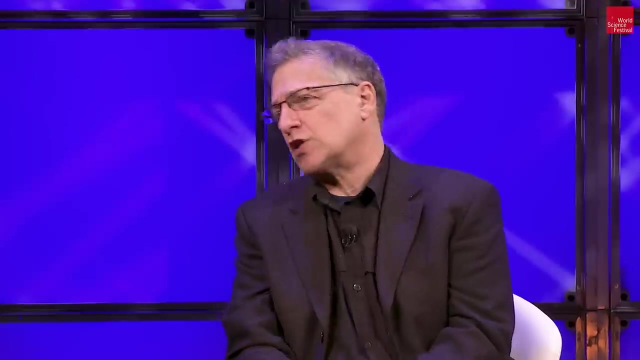 So, as I say to anticipate a little bit, I think there's an absolute good in having alternatives to a dominant theory, whether it's general relativity or inflation or the Big Bang, because it forces us to articulate where we are and what the different aspects. 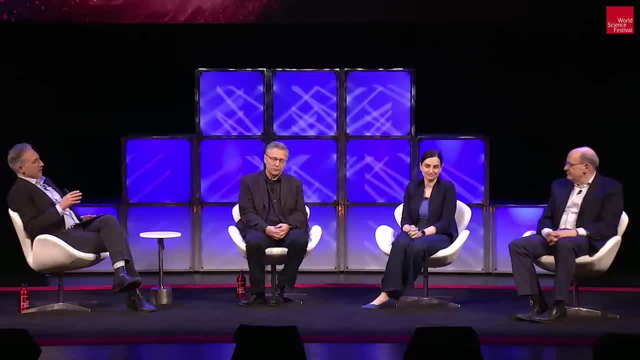 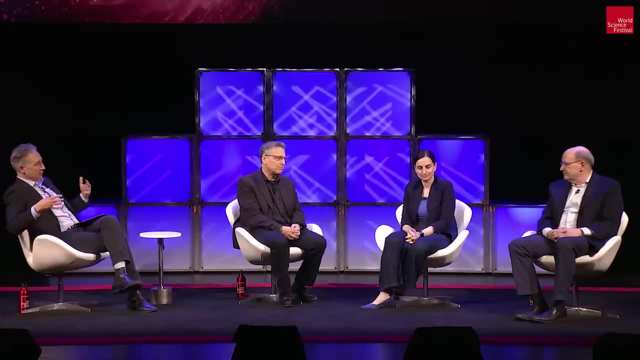 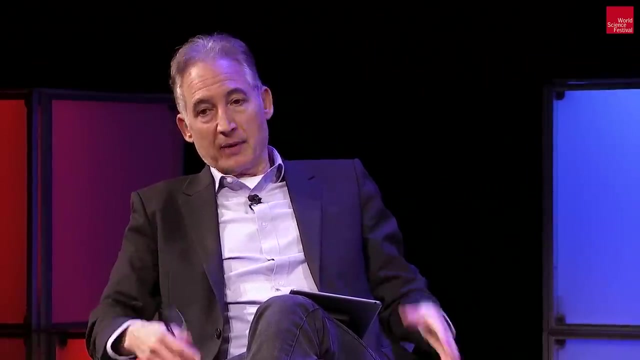 of the theory really ought to be So. Paul Anna mentioned and showed that in that nice graphic of just how significant an extrapolation it is to go from things that we know to things that we want to understand but don't have direct observational evidence for. 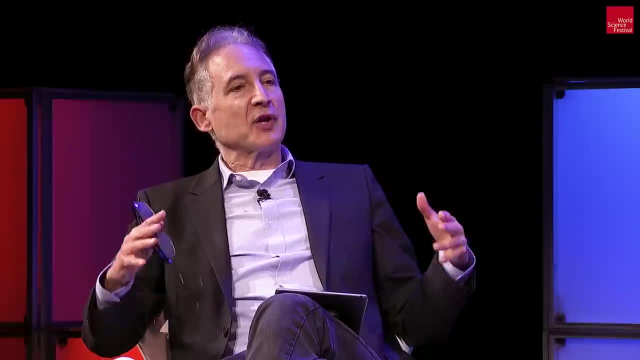 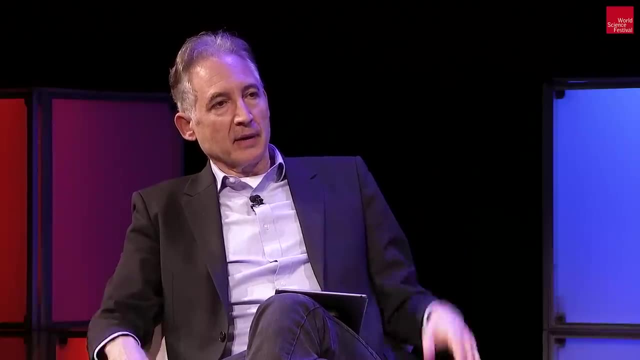 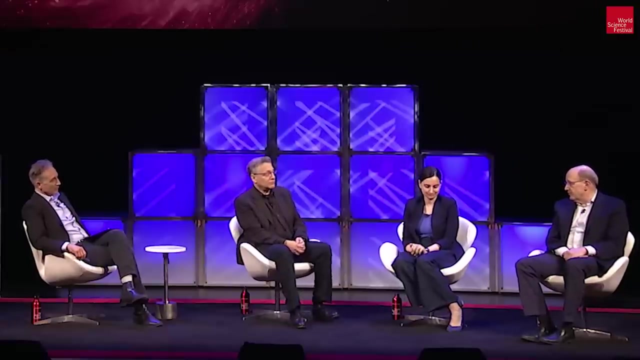 and so on. So, if you're going to imagine something other than a bang, what is the next option that comes to mind and that you've been developing? Well, an alternative that people even thought about back in the 1920s is a bounce. 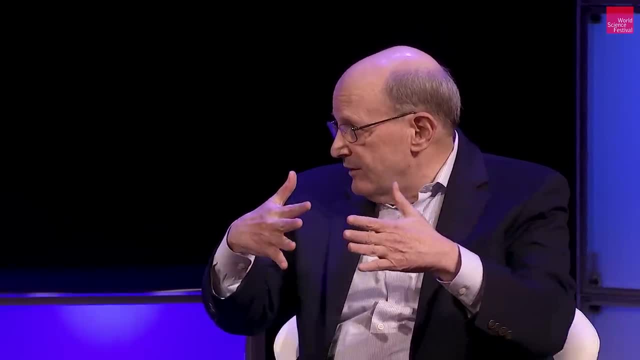 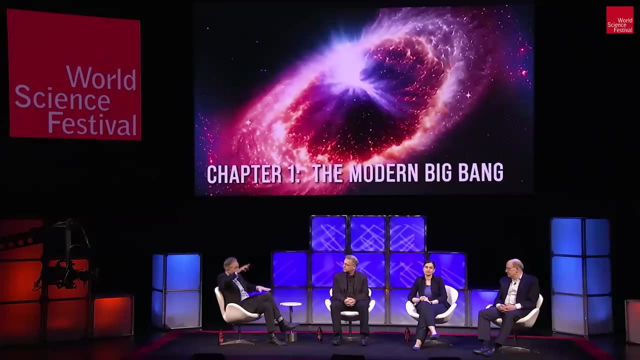 If the universe going backwards in time would be contracting, okay, and at some point, at some stage would reverse to expansion? Yeah, in fact, I guess Richard Tolman is among the more well-known of people. There may have been others who were thinking. 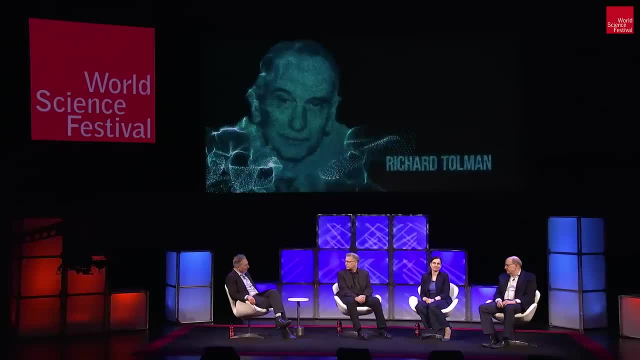 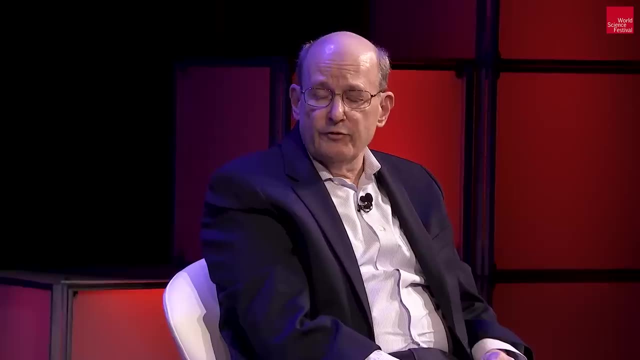 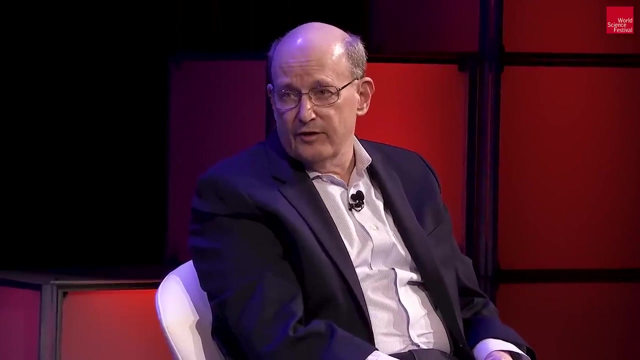 about, like Friedman as well. but so Tolman, my understanding is he tried to make that idea work, this notion of a bounce work. Well, it was Friedman's idea and he was trying to explore Friedman's idea and whether it could be consistent. 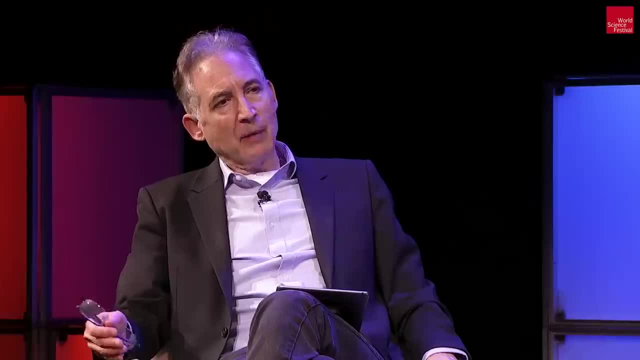 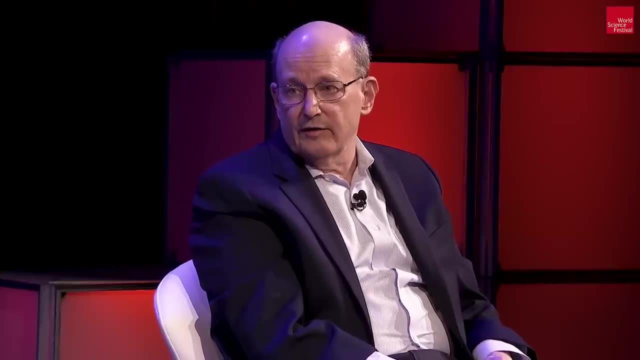 with the laws of thermodynamics, the second law of thermodynamics, And how was that received back then when it was initially introduced? It was a big blow to the idea of a cyclic universe. So the idea of a cyclic universe had been around since Friedman. 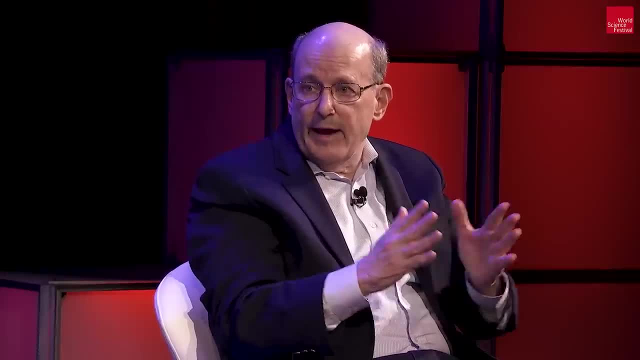 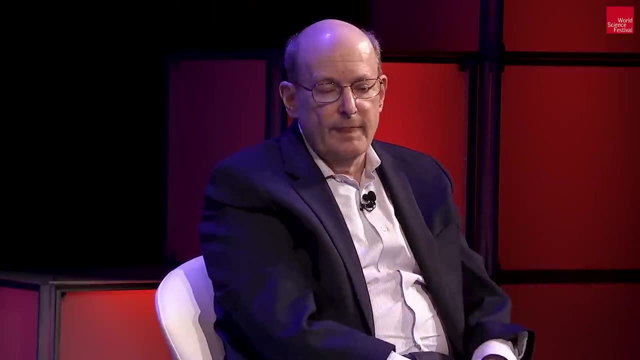 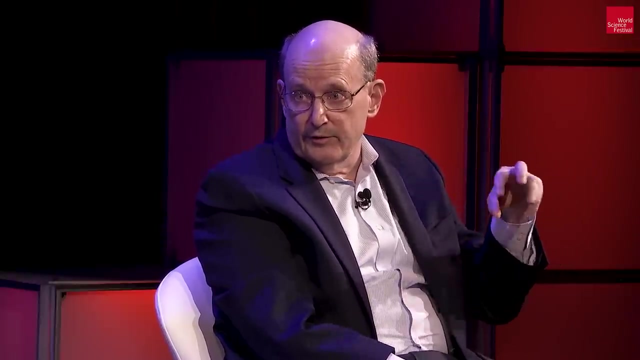 and when we discovered that the universe is expanding, that was on the list of possibilities, that the universe could then begin contracting and bounce and that this would get rid of the problem of having a beginning of time if it were cyclical forever into the past. 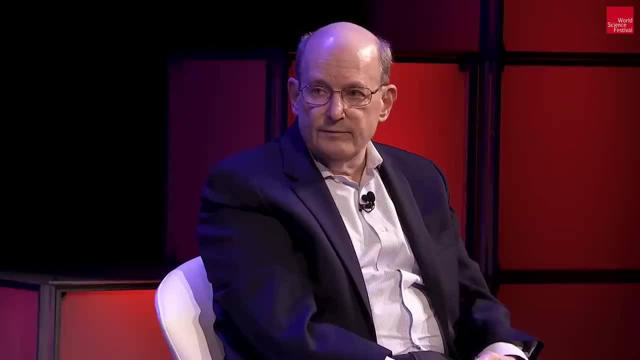 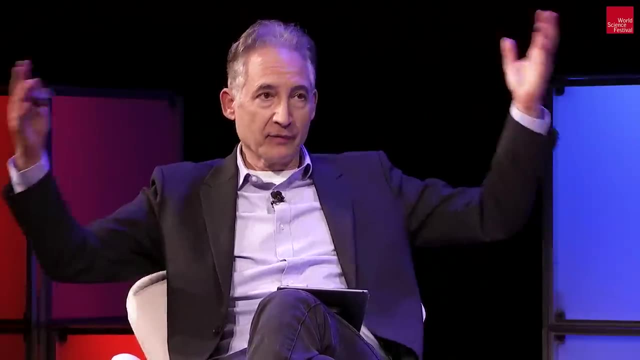 and that intrigued people. But Tolman pointed out, Because you wouldn't have to explain why there's a universe at all, You'd just say there always was a universe. It's just been expanding, contracting forever. It's another logical possibility. 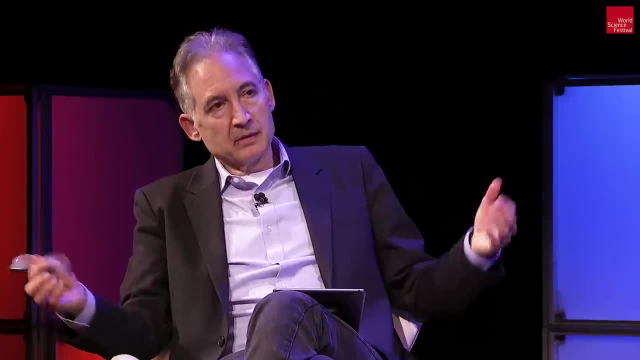 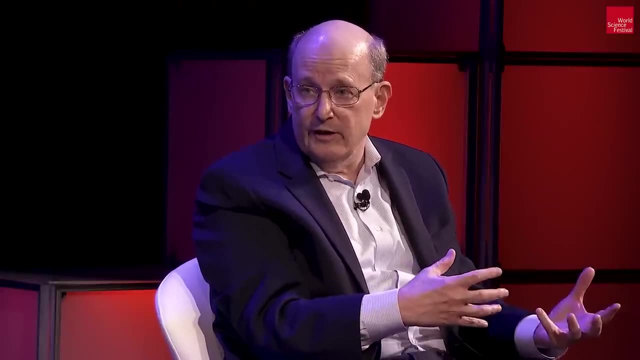 Maybe we're spending a lot of time trying to explain something- the Big Bang- which never happened. So maybe there's another logical possibility to be explored and ultimately you want to turn that into a theory that has testable consequences. So Tolman was exploring that idea. 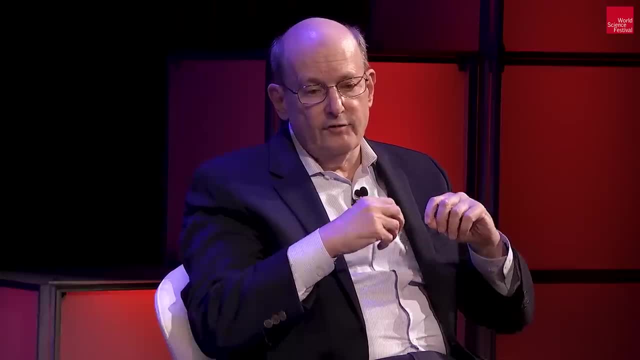 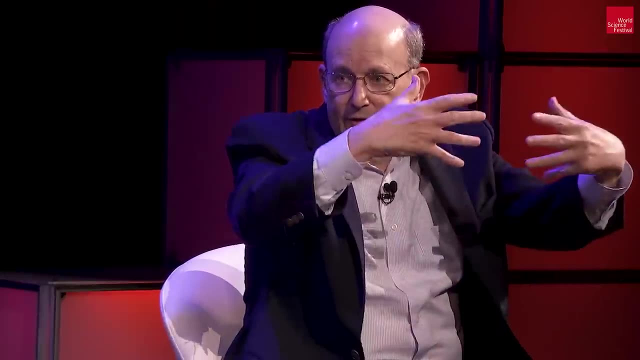 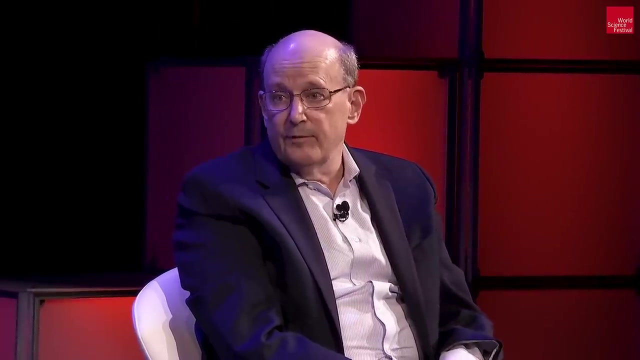 I should emphasize that the idea of bouncing in those days was that you would bounce until all of space-time disappeared and then reappeared and then expanded and contracted and disappeared again. So it was this kind of bouncing universe and it led to this kind of problem. 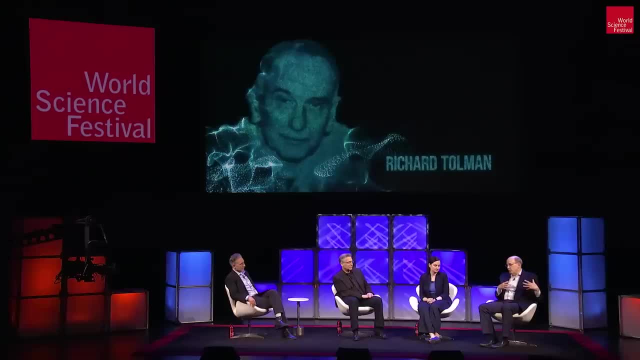 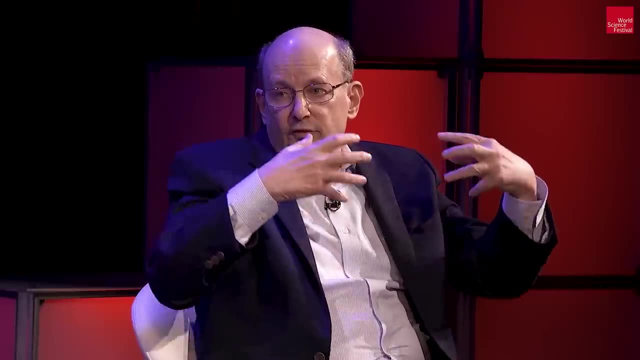 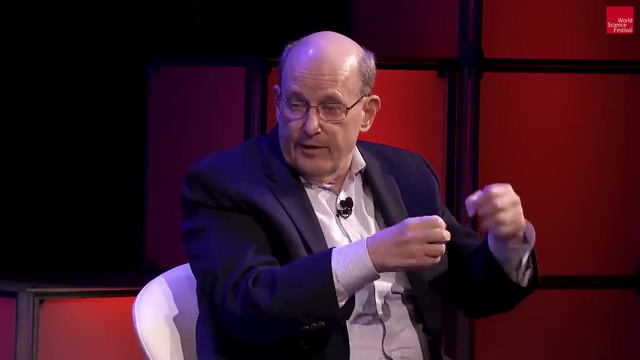 that Tolman pointed out that if you think about the disorder in the universe, the entropy or disorder in the universe, whatever disorder you had in one cycle would be re-contracted or re-concentrated as the universe approached. the bounce came to zero size. 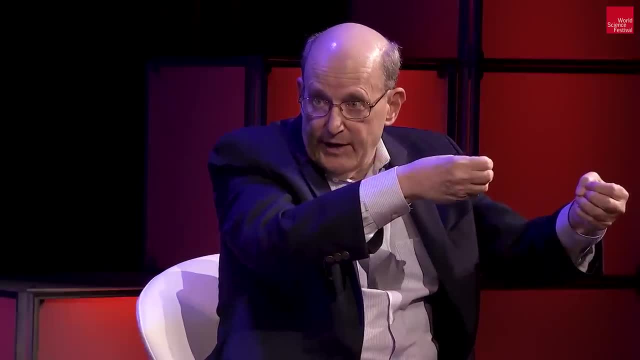 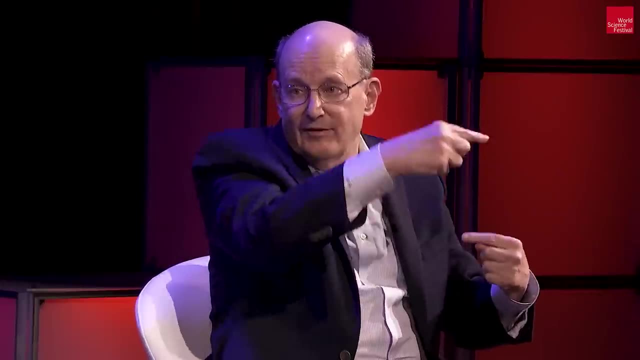 and would be there when the universe began the next bounce, but it would influence, through its gravitational effect, that next bounce. So, instead of that next bounce being identical to the one before, it now has whatever disorder it's going to produce, plus the sum of all the disorders. 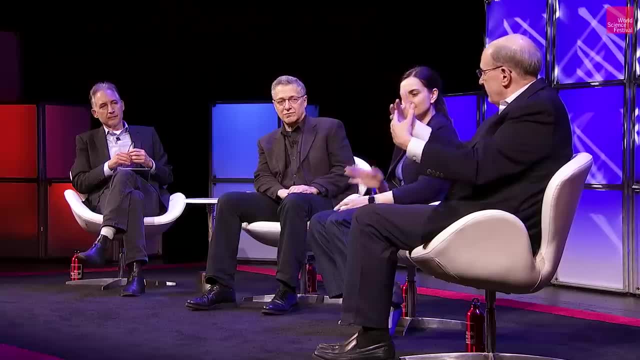 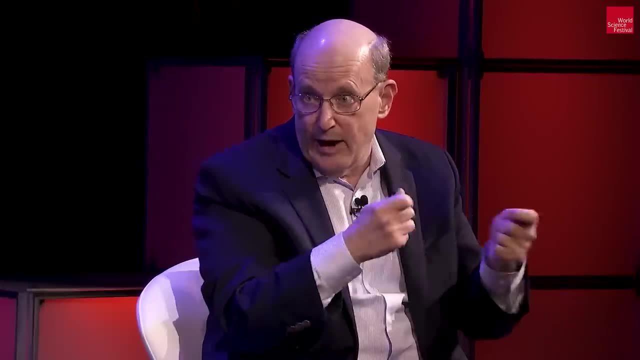 of all earlier cycles, And then he showed that that meant that the cycles couldn't be identical. Obviously, there's something you can measure about the universe: the amount of disorder that would distinguish one cycle to the other and the cycles in fact. 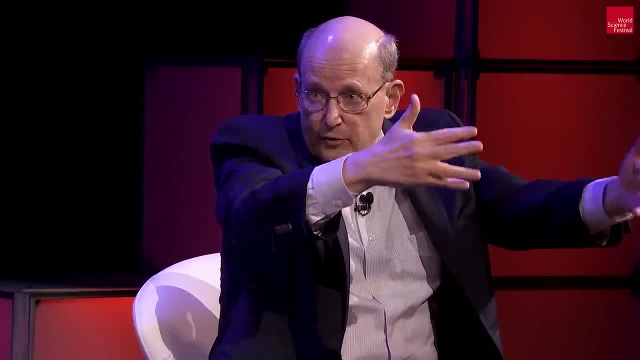 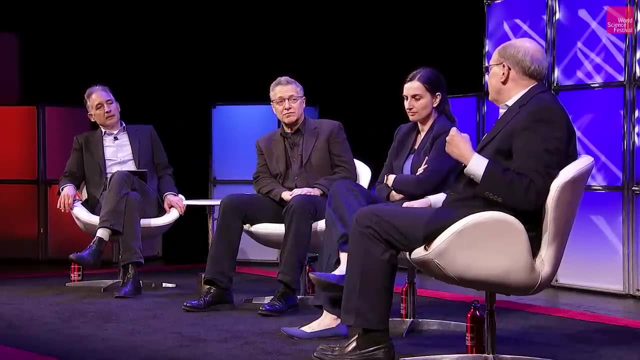 must be growing in time, going, growing in duration, going forward in time. Which means if you go back, yeah, But backwards in time, they were contracting rapidly to zero. so you didn't get rid of the beginning issue, You got back to the beginning. 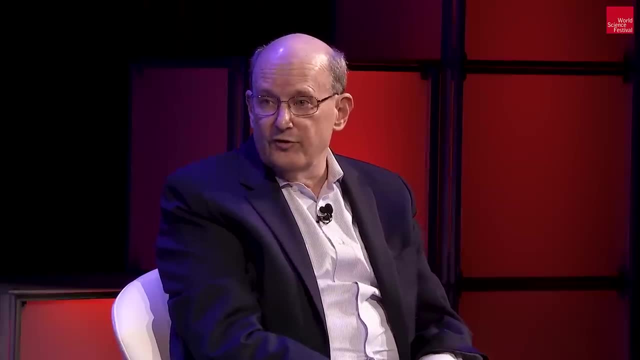 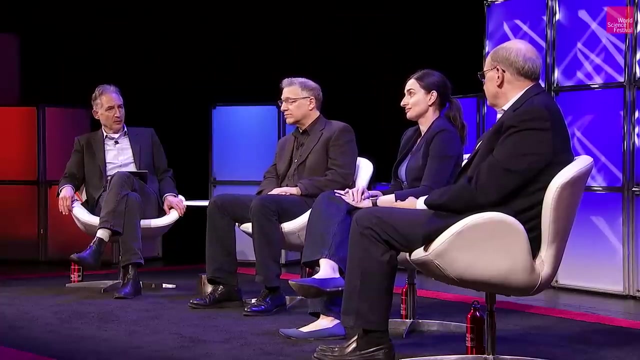 and so that discouraged that and other historical facts discouraged people from thinking about cyclic models for a number of decades. Yeah, basically nobody really took the idea seriously until the work that you have recently pioneered, right, There hasn't been much in cyclic cosmology. 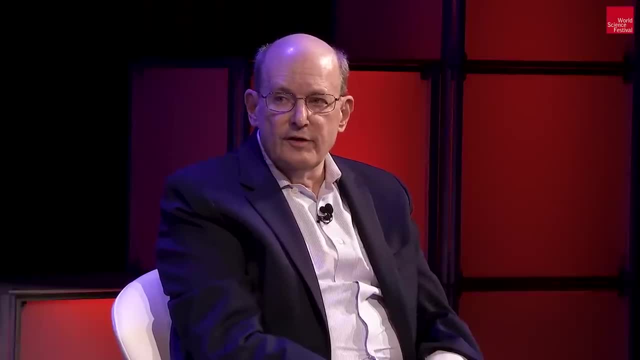 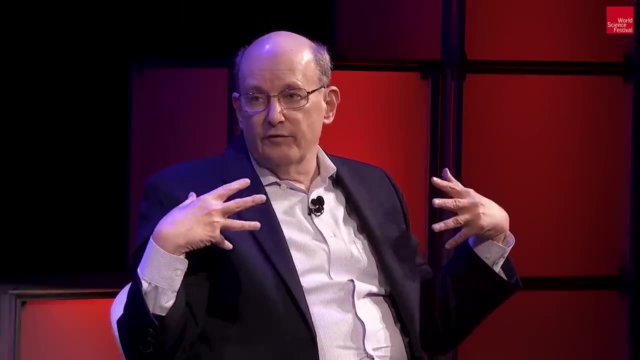 since Tolman right. Well, in bouncing cosmology there was a movement in the 50s and 60s where people began to think about the idea that the universe could have undergone a period of contraction into a bounce and then expansion. It ran into yet other problems. Whenever you concentrated the universe to a point that meant all the matter and radiation that existed before the bounce was being scrunched together. And when you scrunch that much energy together, you can't really predict what's going to happen next. There's no particular reason why it would bounce because of its strong gravity holding it together. So that was a concern. And then another concern was as the universe contracted in those models, there was an instability in which you would begin to change shape in wild ways. depending upon which point in space you were observing from, And essentially it was de-homogenizing the universe. It was messing it up as much as you could possibly imagine. So you had three problems with cyclic models: Tolman's entropy problem. What do you do about crunching all this stuff together? How do you survive that and ever have a bounce? And what do you do about the inhomogeneity you would naturally create during the kind of contractions that people were thinking about in the 50s and 60s? 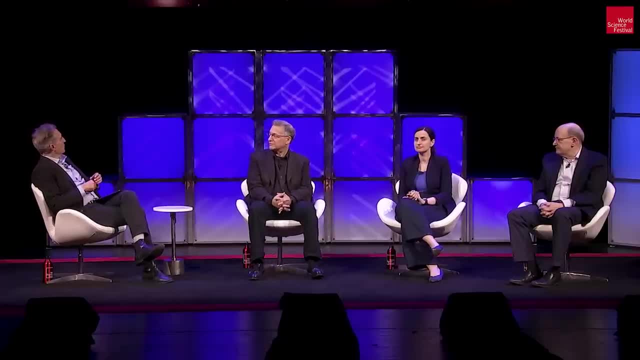 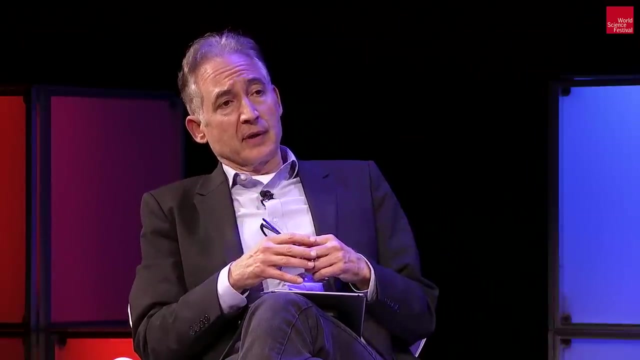 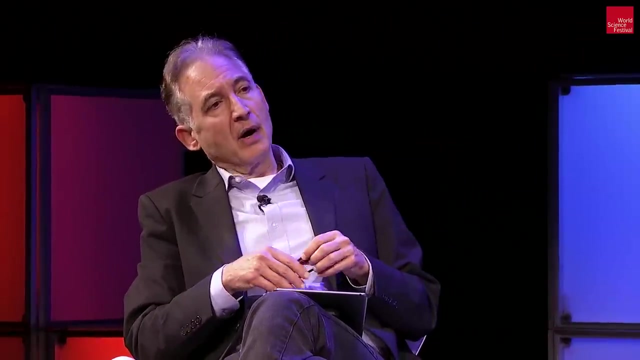 Right. So I think that's a good motivation to think now more fully about the work that you and Anna and other collaborators have been working on, because I gather you claim that in your version of this cyclic cosmology, you have resolved the majority, if not all, of the problems that beset it early on. 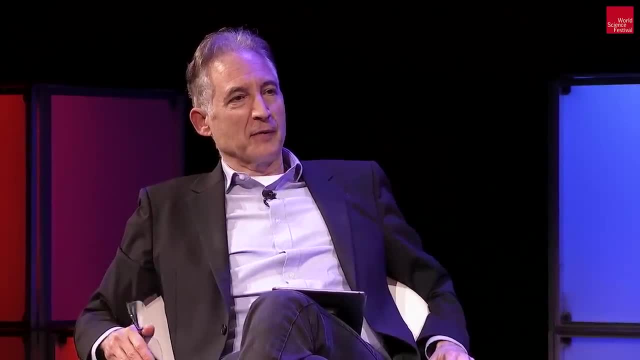 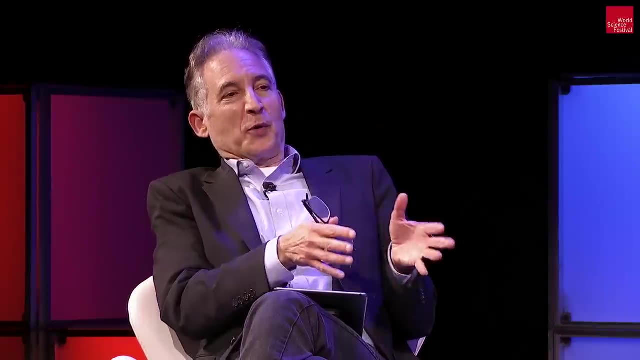 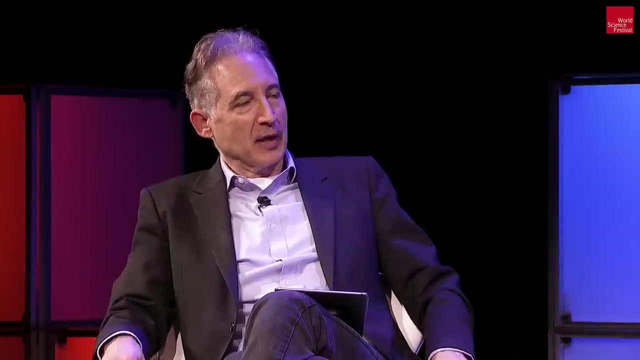 So, however best to explain it, Anna Paul, just give us a sketch and then I think you have some nice simulations that will both argue for your approach and also against the inflationary approach, trying to bolster the case for this reimagining of cosmology. 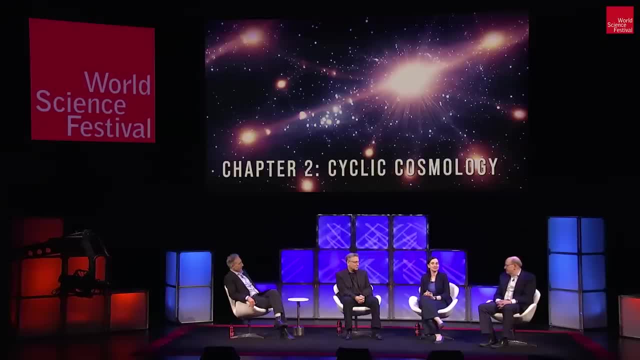 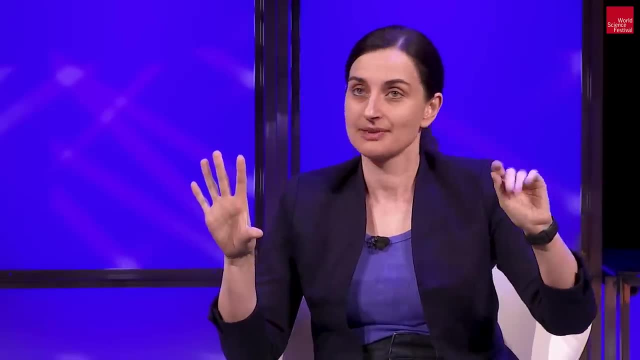 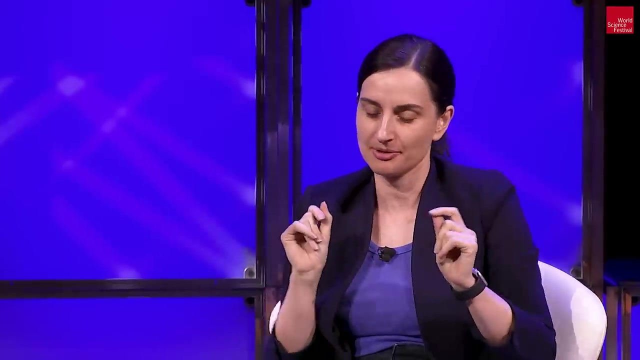 Sure, I can start. Yeah, Go ahead, Okay. So I think you know the three problems that Paul mentioned. they really affect two phases, actually three, because so one point, we call it cyclic cosmology, right? One point that we often tend to forget is: and that was what Paul was talking about in the 50s and 60s. there really are two different scenarios. We could imagine a universe that started to contract bounced and now expands forever. maybe, Yep, That will be, I think. 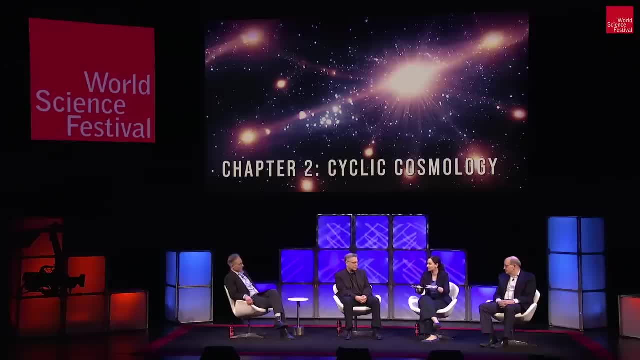 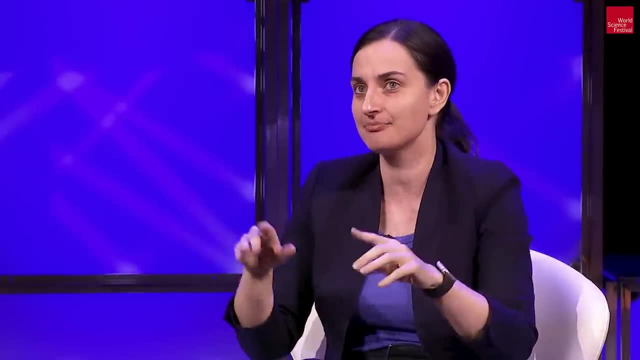 we have to fix first that scenario. Okay, Is that possible? Good, If that's not possible, you will not get a cyclic cosmology Right And it's easier to fix in a certain sense, because that doesn't suffer from all of. let's say the Toulmin problems. what happens if the expansion stops and goes over to contraction? Can you do that? Just get one cycle to work. Get one cycle done. Yeah, And this is really where we started. And again, 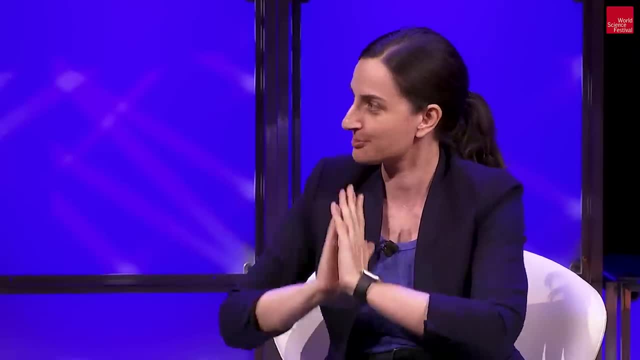 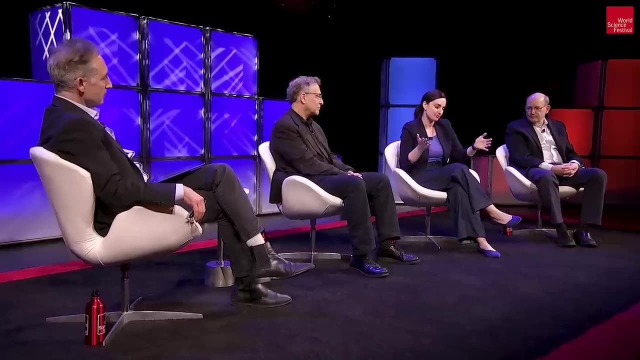 even the one cycle. the only thing, what we know how to describe today is the expanding part. We know that Nobody debates about it. That's what we call the consensus model and the CDM. Yeah, So what we have to fix is: 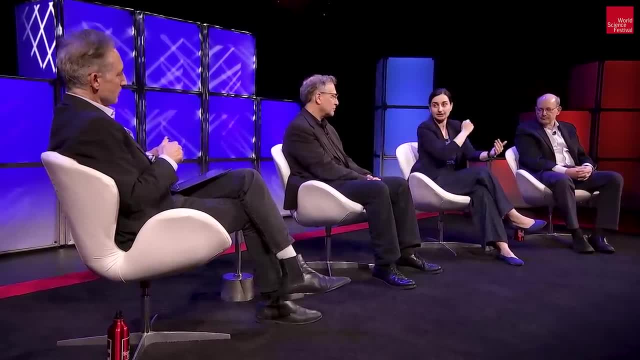 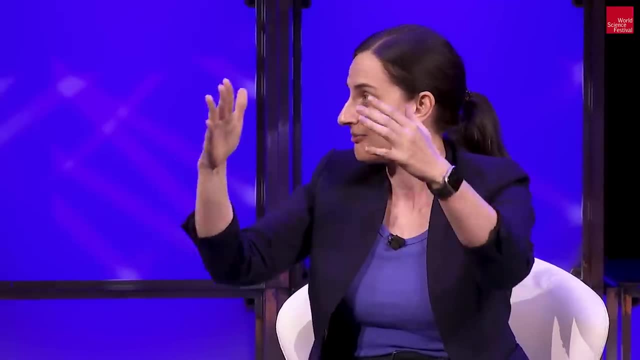 can we describe this contracting phase in particular that it approaches the bounce without this crazy chaotic behavior, Yeah- And at the same time smooths the universe so that once we bounce, we see exactly the universe as we observe it in the microwave background. 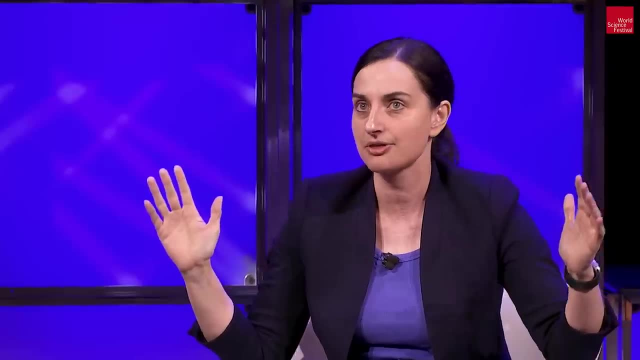 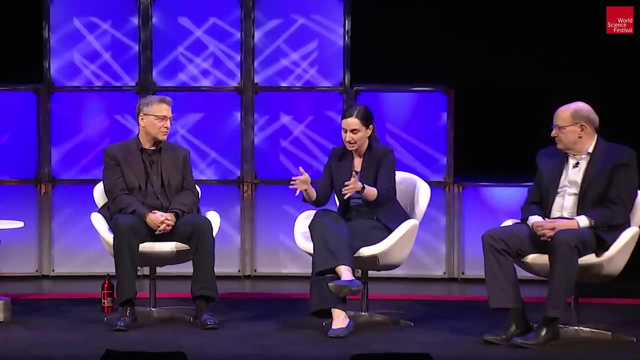 Yeah, So that's the one question. Is there a good theoretical model for the contracting phase? Yeah, And we will start with that. And then the second part is- and I imagine Paul will tell more about it- it's a different story. 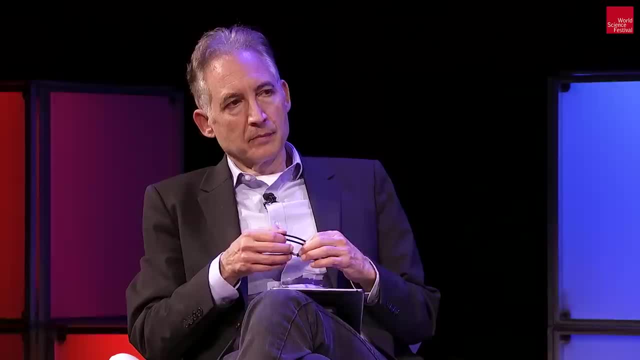 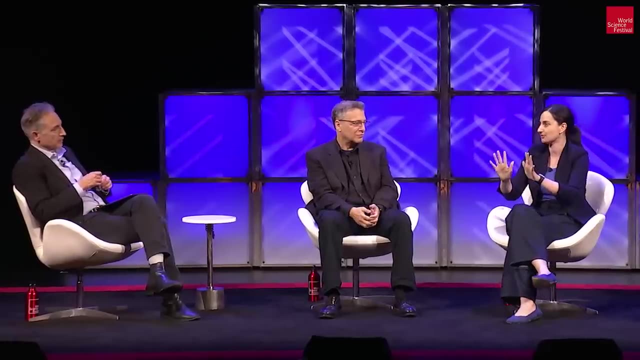 Can we really, let's say the contracting phase works and we will see that does. That's easy. We don't have to bring in new physics, We don't have to do anything about quantum gravity, We just really use general relativity and some new computational tools. 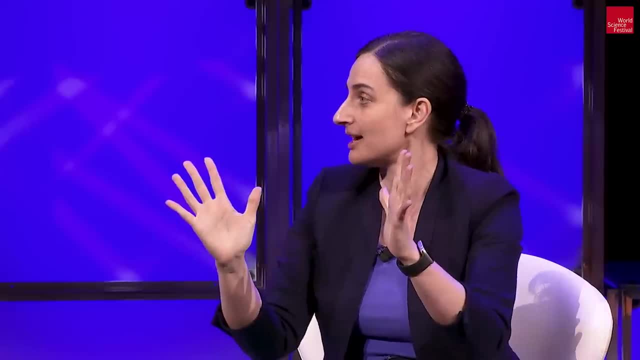 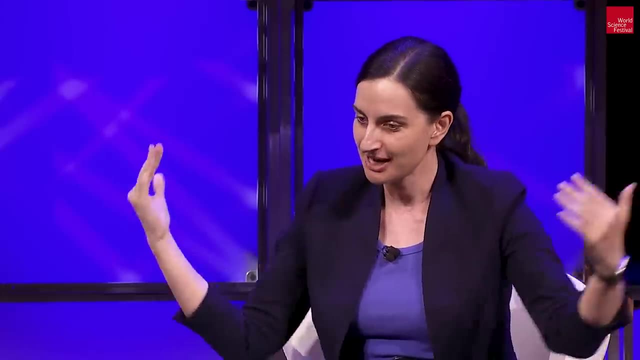 But then the second question is: once everything is fine, can we bounce? That will be much harder. So that's the second part. And the third part is: if we can contract, bounce, expand, can we start again, Over and over and over again? 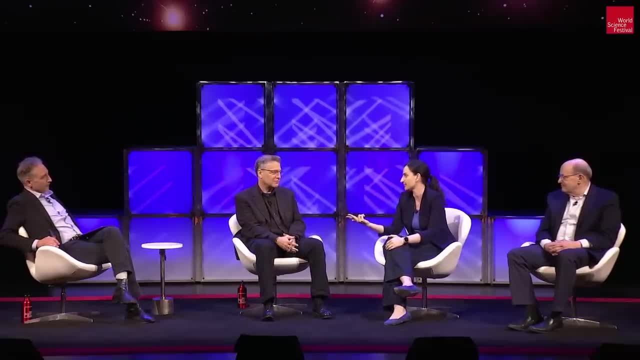 To repeat over and over without suffering from the entropy problem. Yeah, So I think these are the three points we should go through. Yeah, All right. So can you get the contracting phase to work? Yeah, So one thing that we think we should talk about. 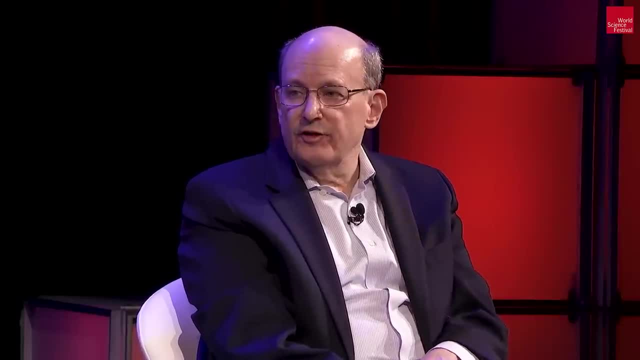 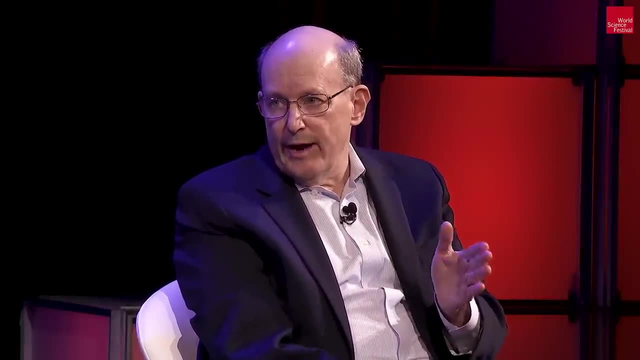 is that there's not just a single kind of contraction and not just a single kind of bounce. So up until our work, when people were thinking about bouncing universes, they were thinking something that would be analogous to a balloon that was collapsing to zero and expanding. 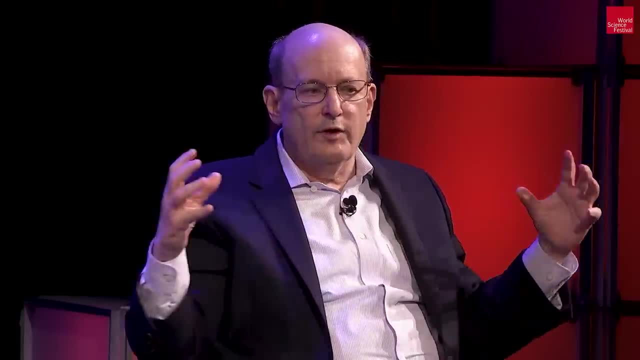 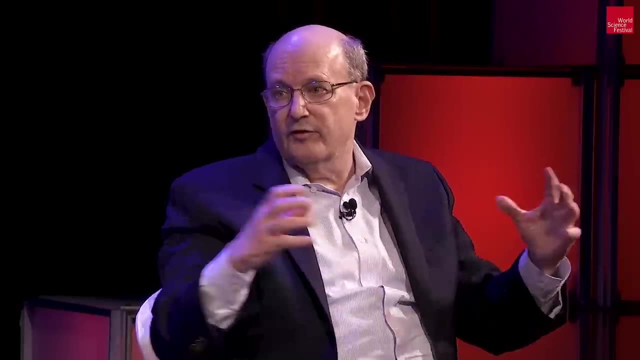 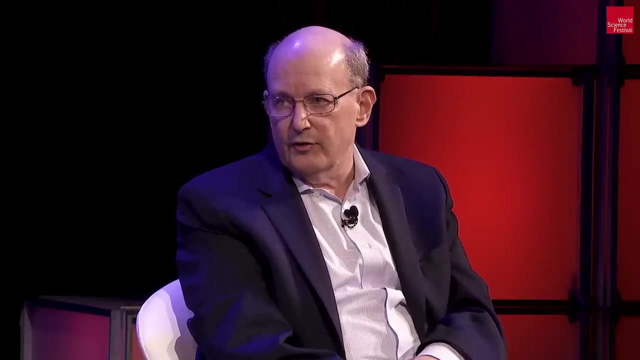 and collapsing to zero and expanding. So the thing that was cycling was what we call this amount of stretching, or the scale factor. Yes, That was the important cycling factor. But there's another thing in general relativity you have to keep track of. in cosmology, 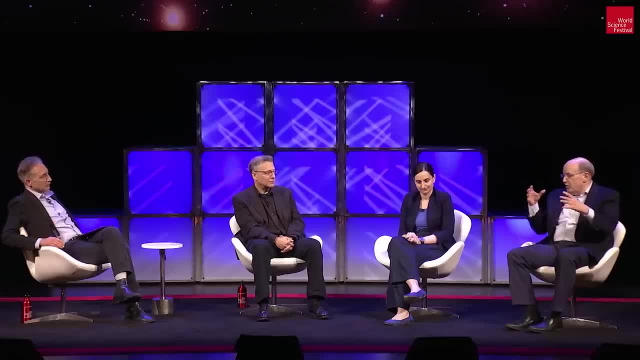 Which is what we call the horizon or the Hubble volume. How much is in causal contact Those things that can actually send signals to each other and perhaps get to the same temperature? Yeah, like what you were drawing in the figure before. And the Hubble horizon is how far you can see. 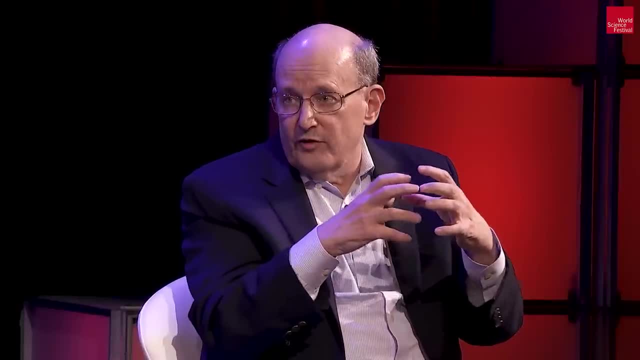 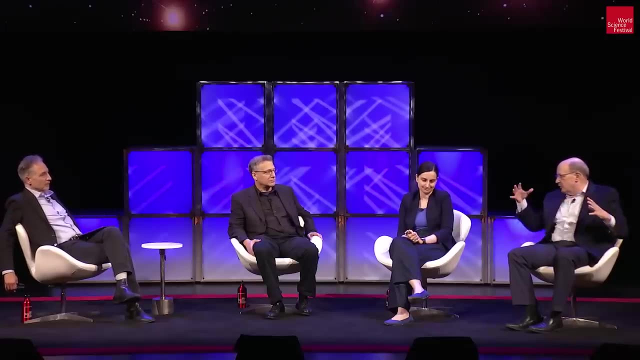 So an observer in the universe like us can only see as far as their horizon. They can't see the entire space. So think about a little circle on our balloon which would represent, if you were standing in the middle of it, the horizon. 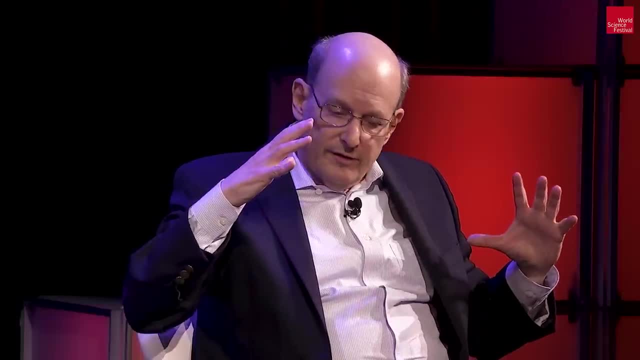 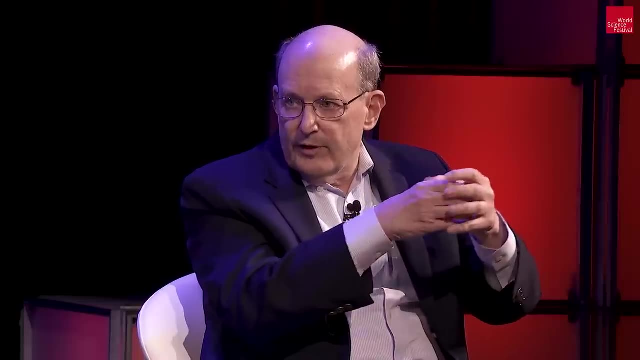 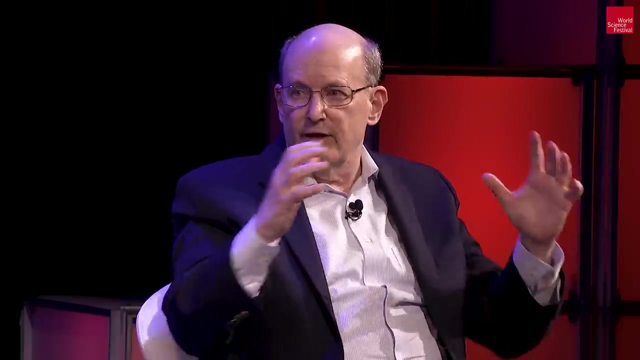 How far you could see. Yeah, Well, the thing is, how fast the universe expands or stretches is different from how much the Hubble horizon stretches. So, whereas before we were thinking about a universe in which the entire balloon was shrinking and expanding, let's imagine instead just the observable universe was shrinking and expanding in a cyclical way. Yeah, Space would always exist. In fact, space could be continually expanding, But the amount you could see if you're an observer in the universe, since you can only see a limited region of the universe. would look the same from cycle to cycle if you looked in your environment. Same as if you imagine that on a planet that was expanding or contracting but you had a limited horizon. So that means you don't have to have space shrink to zero to have a cyclic universe. It's really a fundamental different kind of cyclic universe. That means space is ordinary during the bounce. It also means anything that was in your horizon before the contraction began, like the amount of disorder and entropy gets pushed out, has been stretching out while the horizon has contracted. 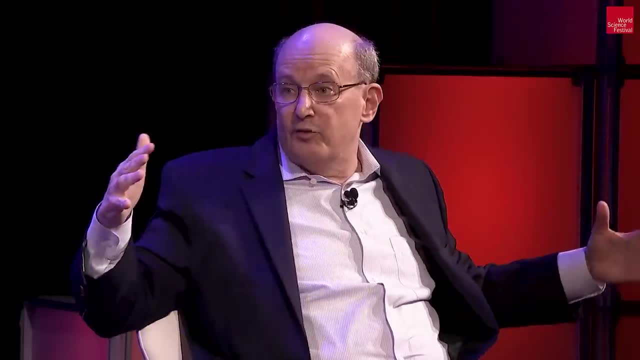 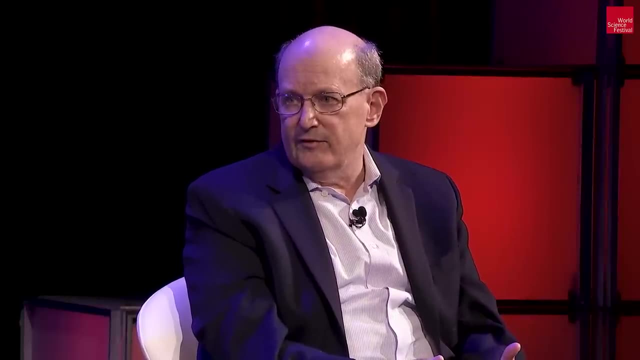 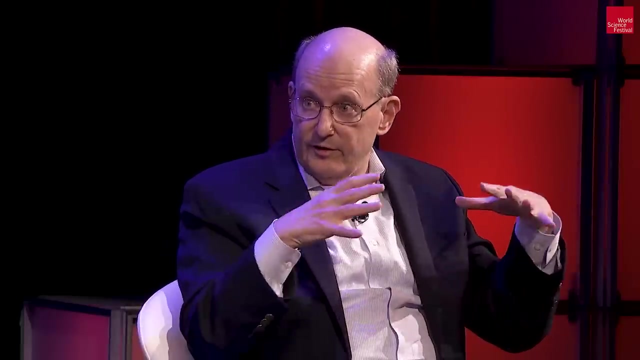 So, yes, there is lots of disorder out there, but it's been spread out to parts of space that you cannot observe. So this is really a fundamental different kind of cyclic universe. that evades the disorder problem. It also happens to be that this condition 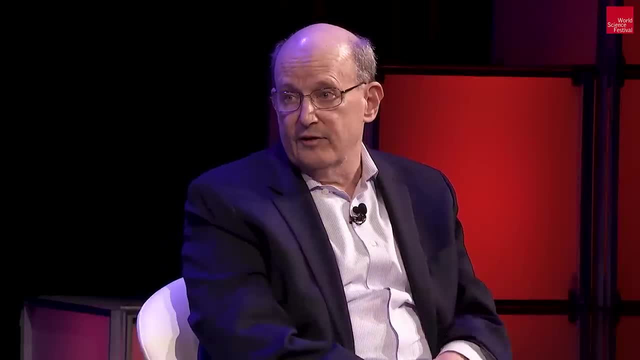 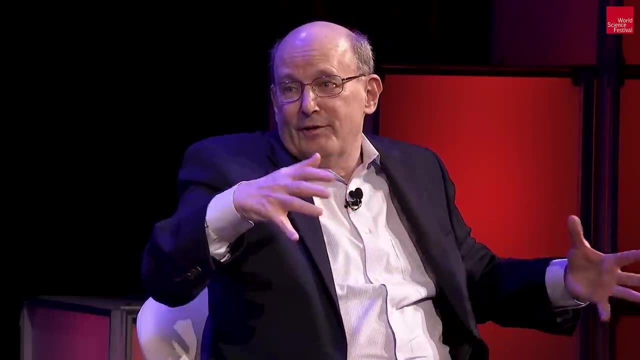 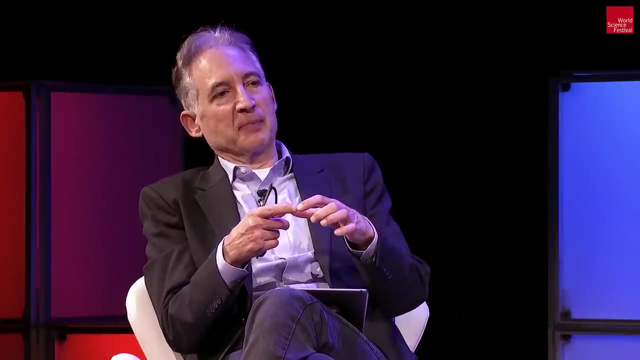 also prevents the kind of chaotic effects that we're talking about, that were discussed in the 50s and 60s, And you never have crunching because, on average, space is always expanding, I see. So, if you're focusing your attention on the part of space that we observe, 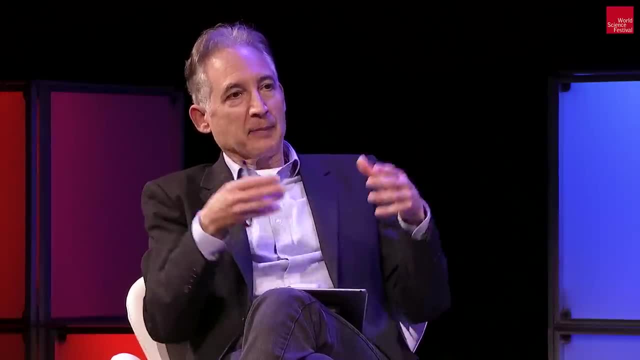 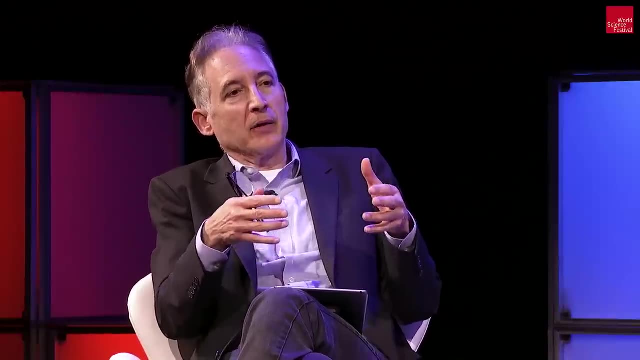 we don't have to use the language that perhaps you would have invoked. in an ordinary cyclic theory, Everything is crushed together and then re-expands, And in that way you're avoiding the more thorny parts of how a bouncing cosmology would need to be developed. 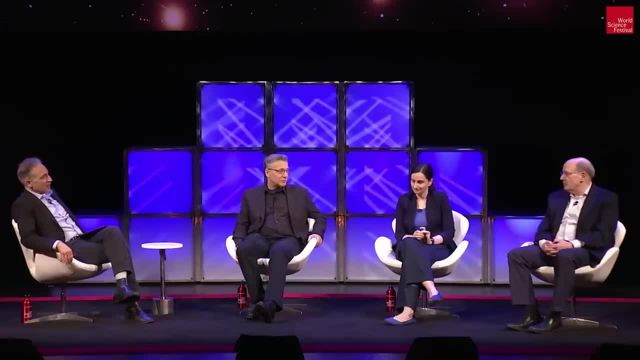 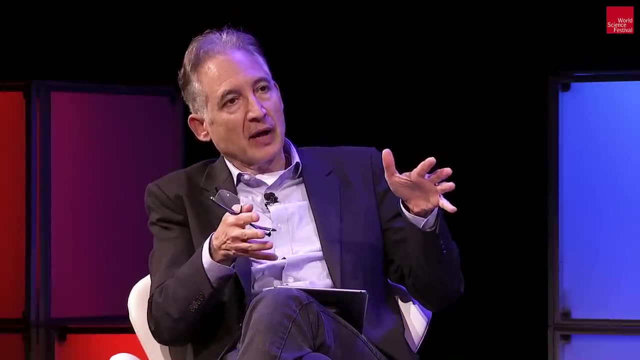 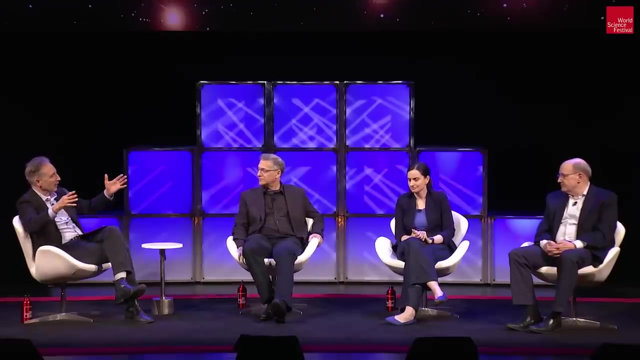 Yeah, you're getting rid of the crunch, what we sometimes call the crunch. It's a crunchless bouncing cosmology, But you still need to ensure that during that phase of contraction you're setting us up for success after that phase concludes and we go into the more ordinary expanding phase. 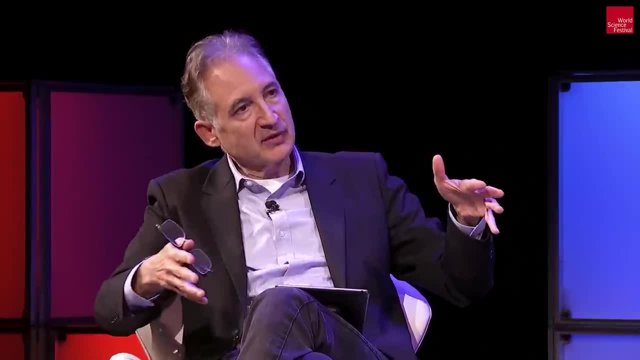 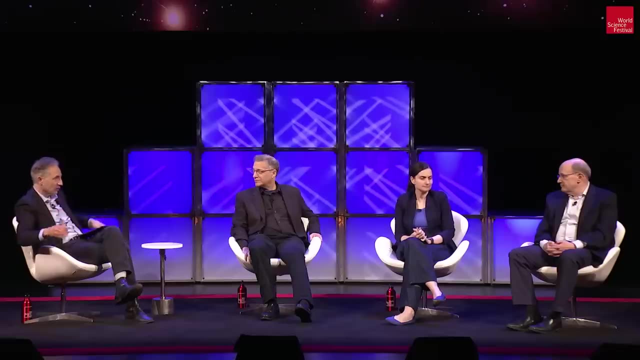 So are you? I mean, is it the case that you can set up the model in such a way that the conditions at the end of this contraction phase will yield a universe like the one that we see? Ana, I can jump in, Yeah. 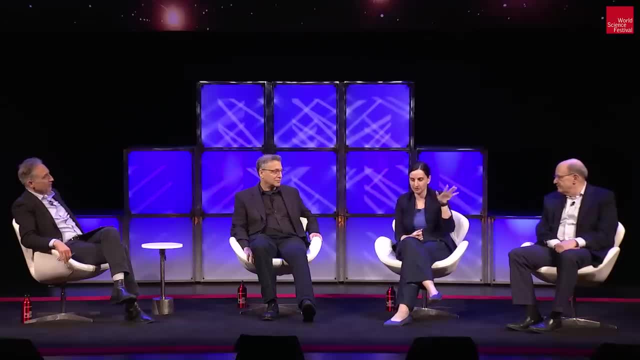 Because I think it's actually worth rephrasing just once more in the language that we used earlier what Paul said, because it's really a fundamental feature of relativity that inflation used, that we used to explain them, the consensus model also contraction. 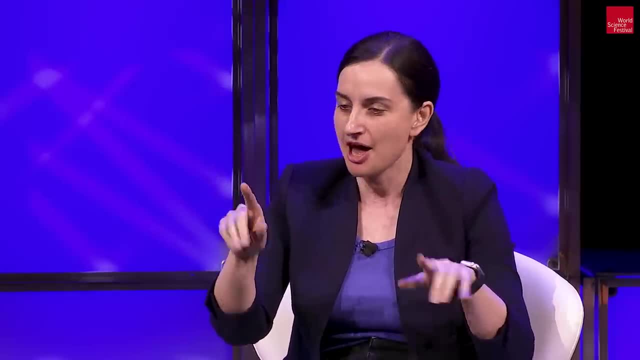 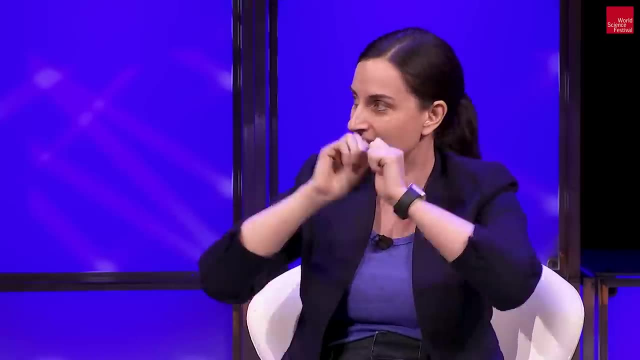 that, given what fills the universe, the rate at which you're contracting, the radius of causal connectedness, the radius of causal connectedness evolves, can be very different from the rate at which space expands or contracts. So it's all the same trick. So what we see? 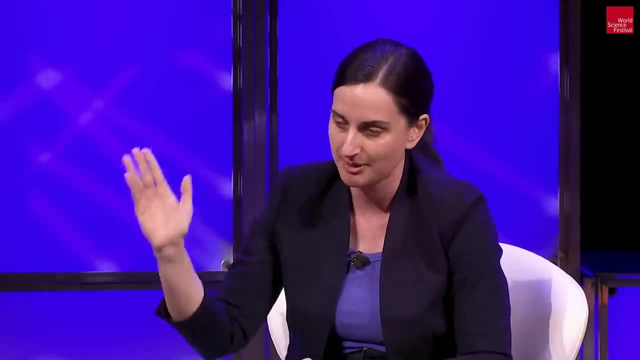 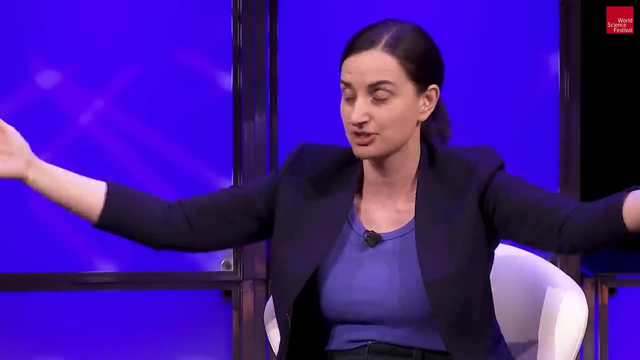 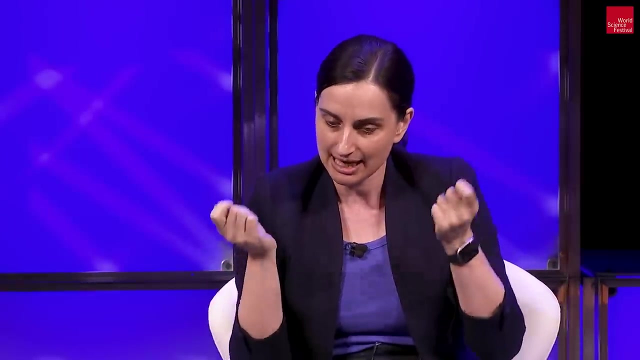 let's say the slowly expanding universe. we know that space expands slower than the region of causal connectedness, so stuff comes into us. That's the consensus model. That's why we needed inflation. Now it's very natural to say, well, can we find a way? 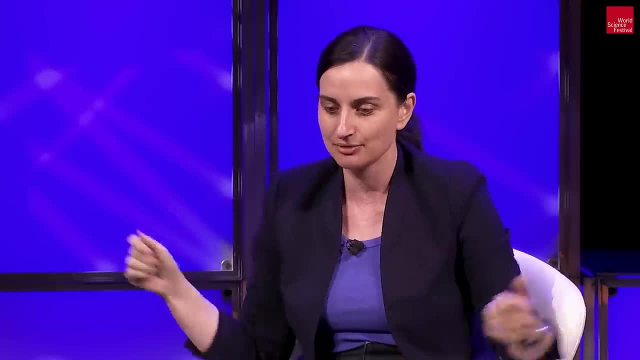 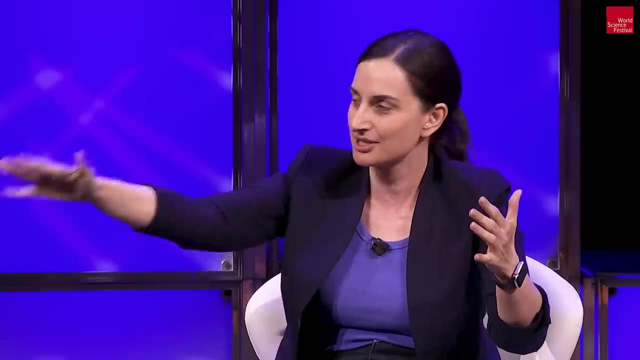 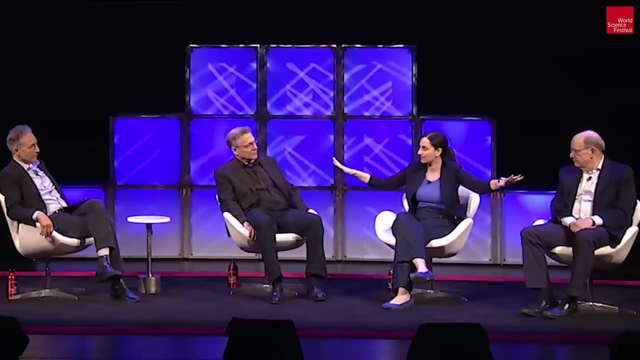 or can we find a model, can we find some stuff- energy density- that during a contracting phase will make the space contract much slower than the region of causal connectedness. Because what happens is you charge a huge amount of space and instead of doing much to space 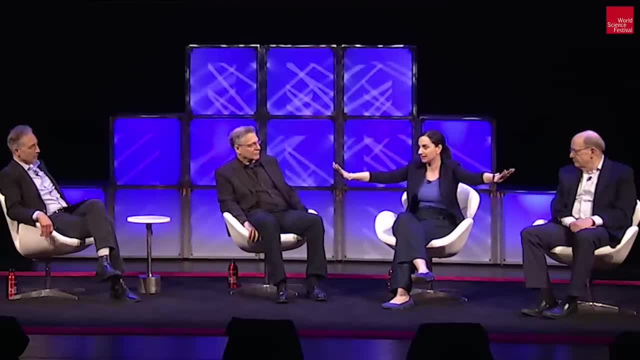 so let's say, if you start with a vast space, a universe like today full of black holes, and you ask what kind of contraction do we need, then we would need a type of contraction in which black holes stay approximately at the same distance. 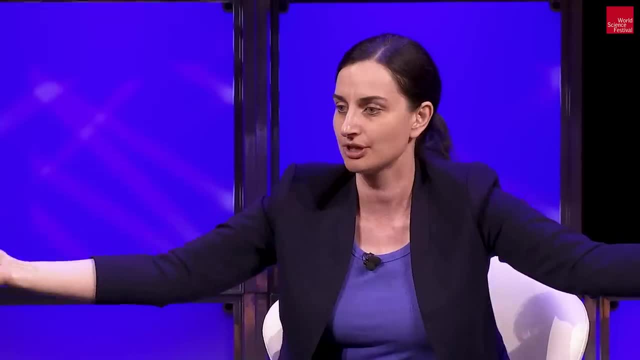 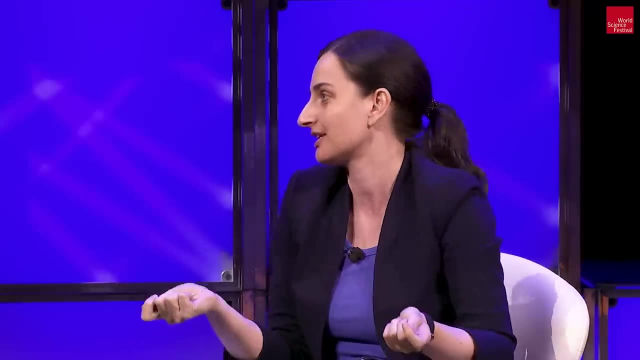 They come a little bit closer, but not much. At the same time, though, the radius of causal connectedness shrinks very rapidly, and that's what you need, And the nice thing is that we can do this in relativity. So what this model needed to be fixed. 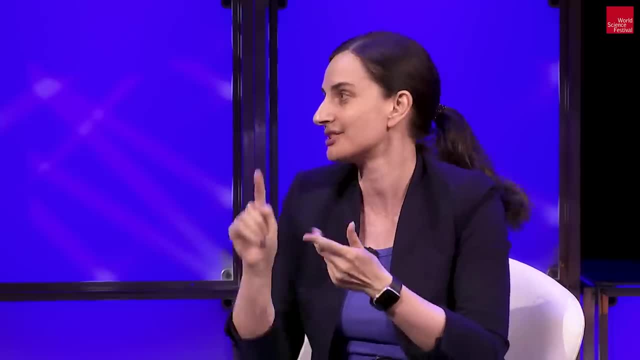 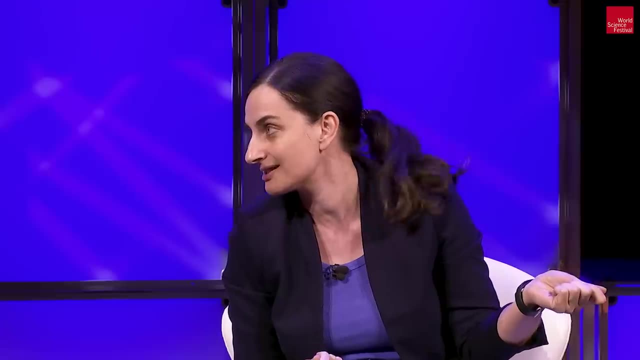 is something that people in the 20s, 30s, 50s, 60s, 70s would never have thought about. As a matter of fact, we need inflation and all the ingredients that people in the 80s invented. 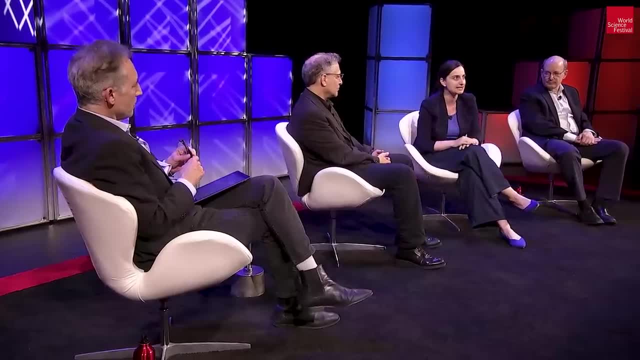 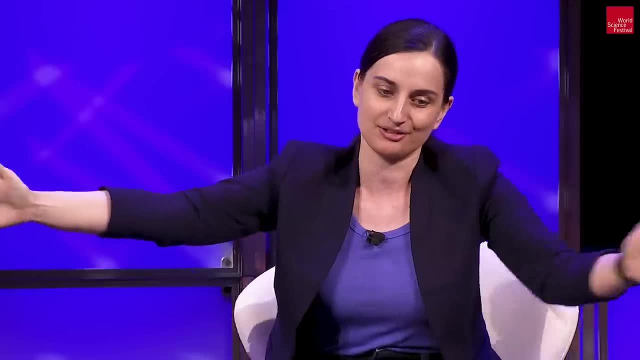 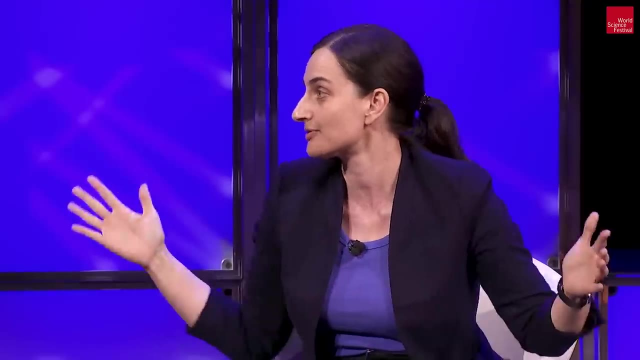 something what we know from the Higgs scalar field, from particle physics, that can actually trigger or exert this behavior- that space contracts very slowly, but the causal horizon shrinks very rapidly, And this is exactly what can be done. So that solves the problem of no chaos. and everything is smooth and uniform as space contracts and goes towards the bounds. Moreover, it's really important to note we don't need new physics, So it's all general relativity. quantum physics only enters on small scales and no quantum gravity is required. 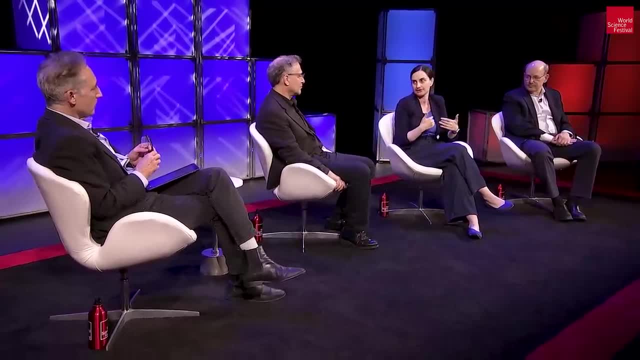 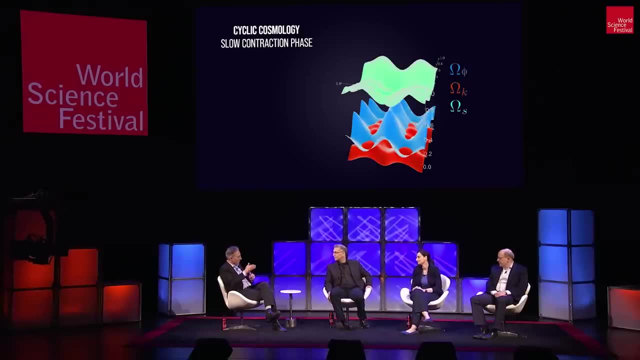 And all ingredient. what's required is that we are very familiar with in physics. It's a scalar field that dominates this energy density, And is this a simulation that can give us some numerical evidence for what it is that you are referring to? Yeah, 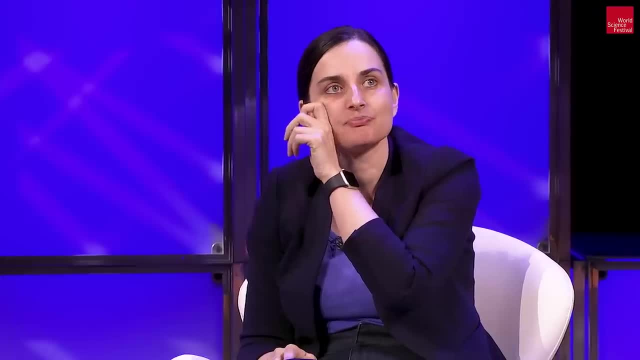 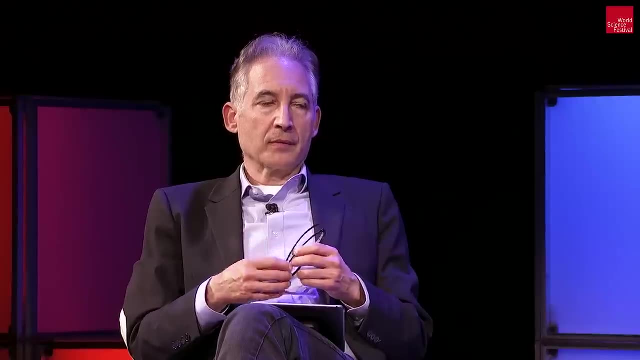 So let's go back, Let's not start the simulation. So I think we should pan back a little bit and just talk about the role simulations plays. Yeah, So cosmology started first as pencil and paper. Yeah, Then we went to particle physics observations. 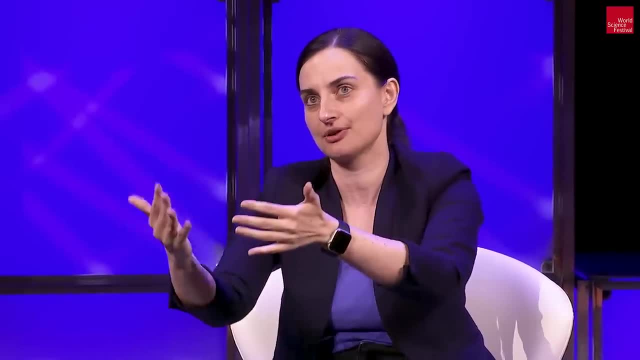 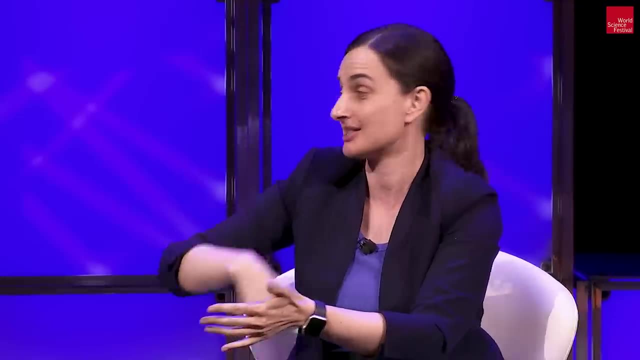 And then what came up in the last 20 to 30 years is we actually can rerun the universe without putting up satellites to look at our current universe, but we can simulate the universe And I think before we, you know, describe maybe our features. 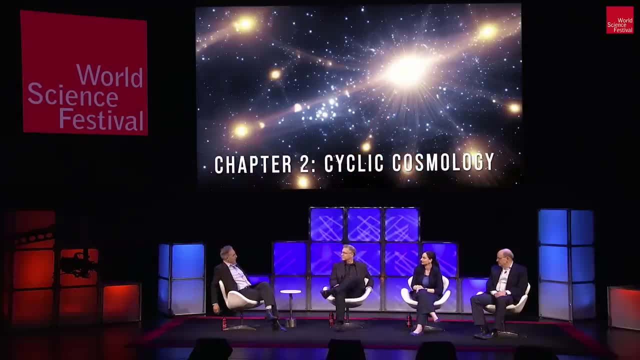 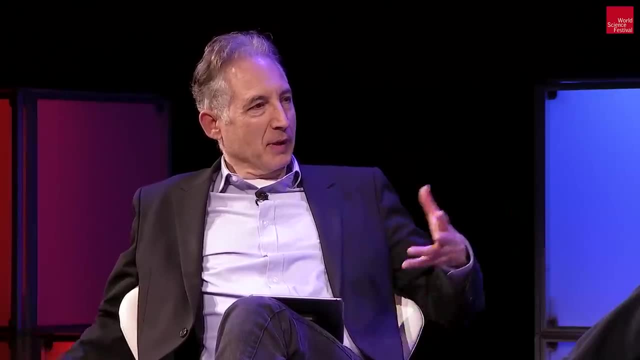 maybe Peter want to comment. Yeah, I mean, how have we gotten to a place where there's you know, a third way? I mean there's, you know, there's theory, there's observation experiment, simulation. I mean, what role is simulation playing? 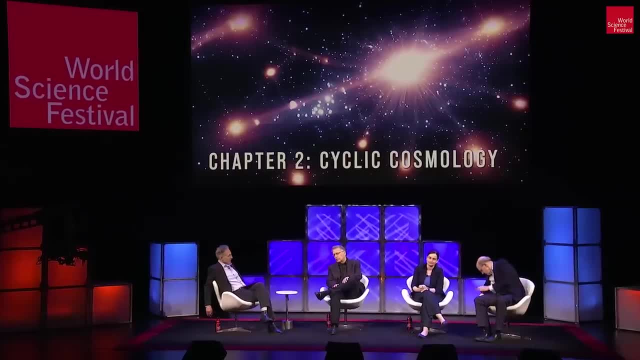 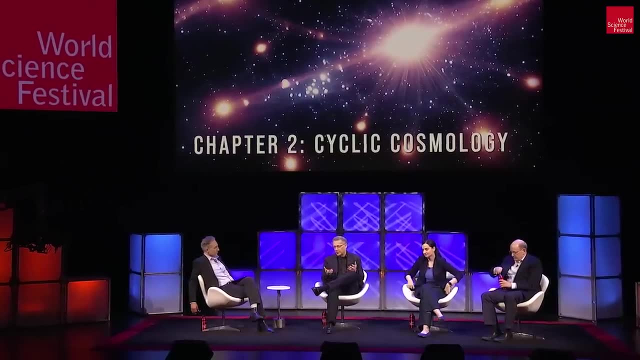 in these cutting edge ideas. Well, I think that, starting in the period at the end of and just after World War II, you had physicists thinking about the hydrogen bomb. This is what Oppenheimer- much on everyone's minds these days, was concerned about. 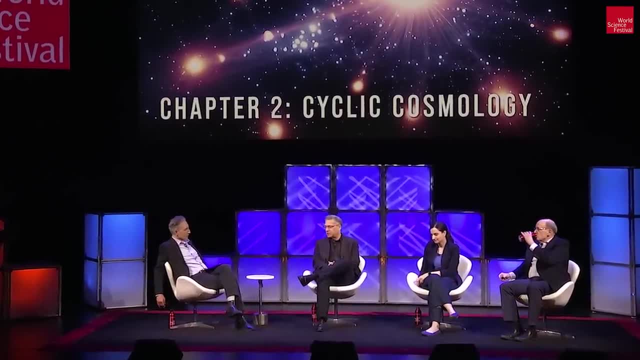 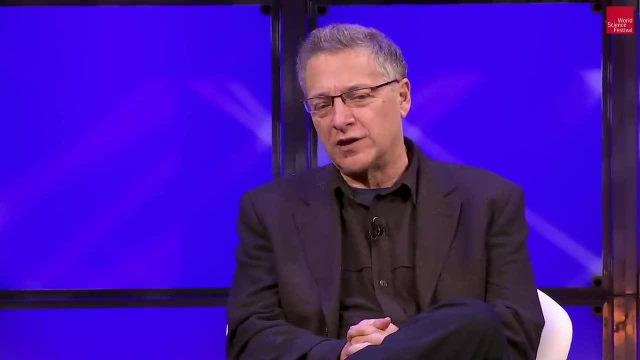 He objected to its building. Teller wanted to build it. Stan Ulam, a mathematician, began to think about a way of doing it, But the hydrogen bomb, unlike the atomic bomb, used basically all of our physics: How radiation is transported. 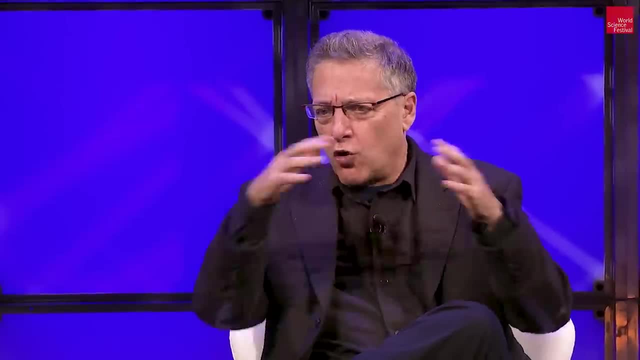 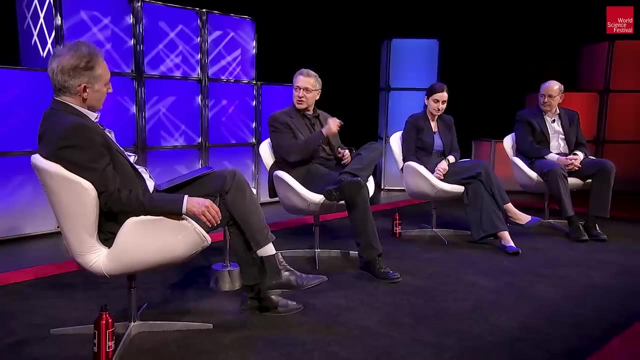 hydrodynamics, nuclear physics, the whole works, And you couldn't do it with pencil and paper or even with the sort of old adding machines that were available at Los Alamos. And so Ulam and von Neumann began to think: well, maybe there's a kind of game. 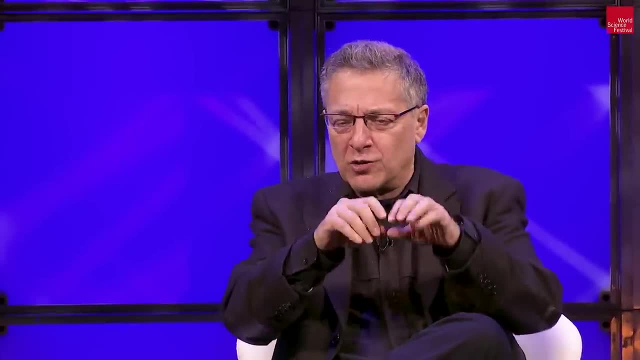 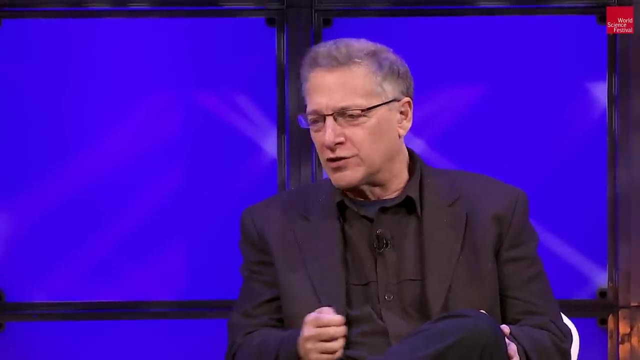 you could play where you know. if you wanted to simulate the diffusion of the atmosphere and the diffusion of a red dye in a thin tube of water. you sort of could flip a coin and go to the right if it was heads and left if it was tails. 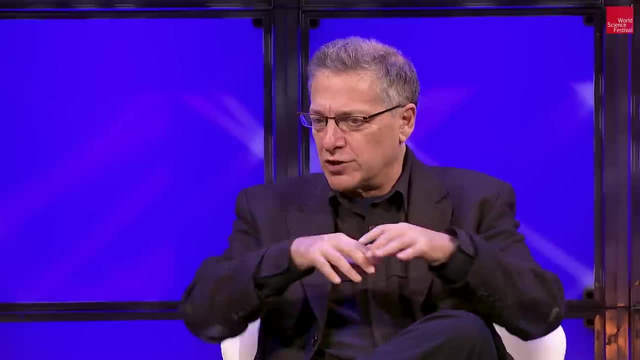 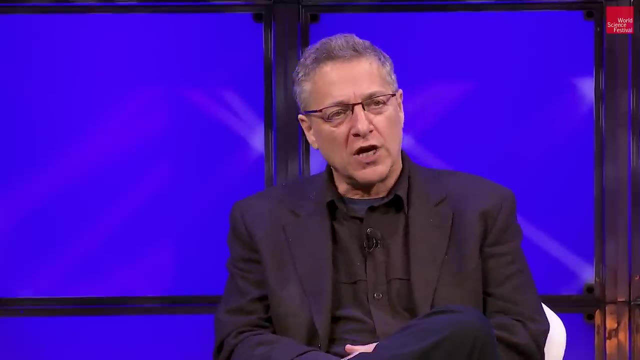 and do this over and over again and you could model how the diffusion worked- And that's a red molecule that's going right or left Exactly And you could see how they accumulated and what the distribution was. And suddenly people began to think. 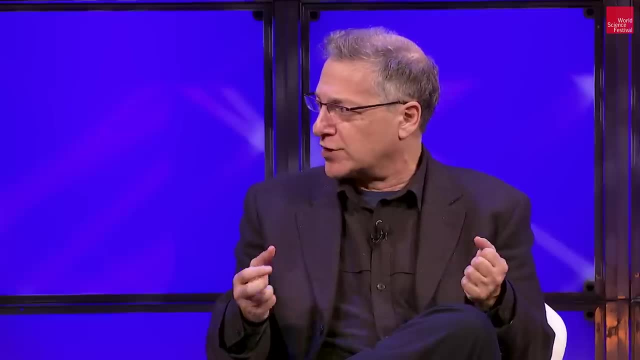 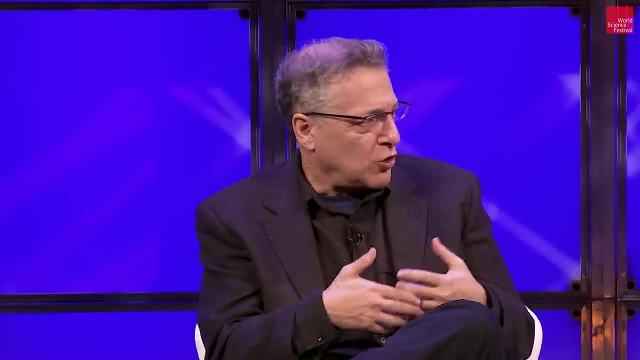 well, maybe we could use this to simulate these very complicated processes where radiation is coming in, And we use it more and more. It's been a big thing. It's a big slow process over the 50s and 60s and 70s. 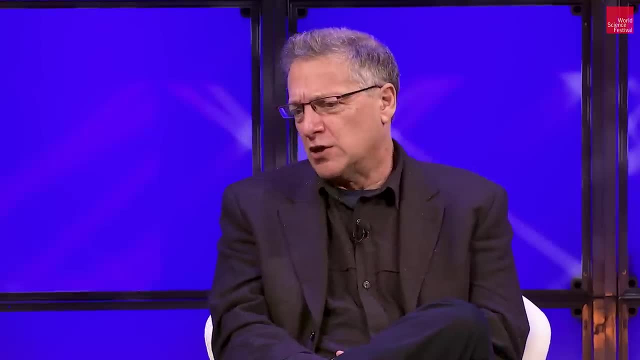 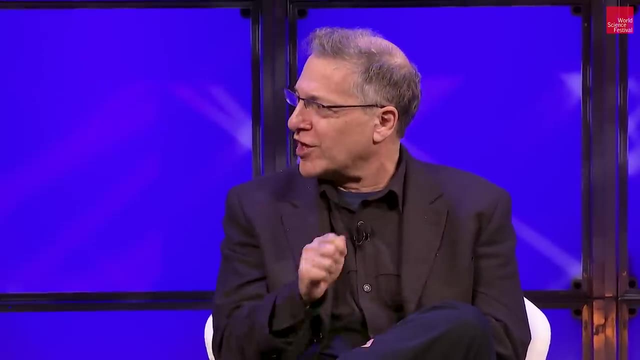 I remember times when you'd see an astronomer would say: well, you made a simulation that showed that such and such an effect works, but what's the real equations that tell us this? But at a certain point people stopped asking that question. 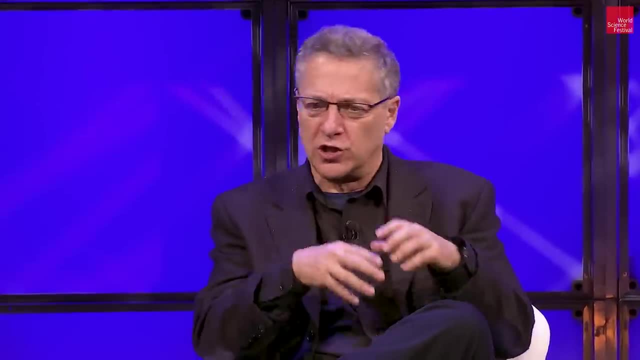 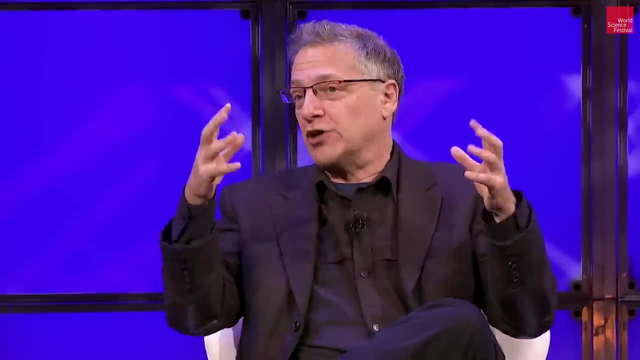 The simulations were what you needed to understand: galaxy formation and neutron stars, these very complicated objects that are like the nucleus of an atom but much bigger, And you have thermonuclear explosions going on in the surface and new forms of matter at the inside. 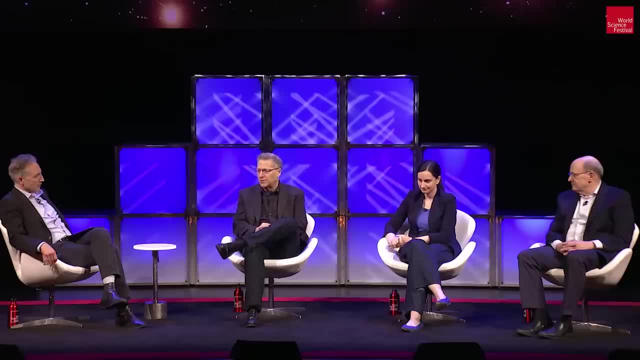 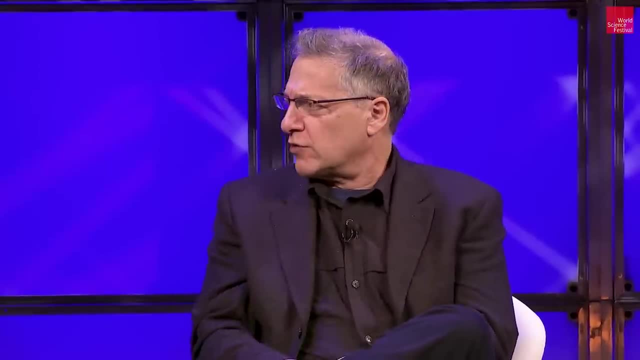 And there's so many things in astrophysics that require this, but not just astrophysics: Particle physics: what goes on at CERN or Fermilab or any of the other accelerator laboratories? what goes on in the plasma physics lab? 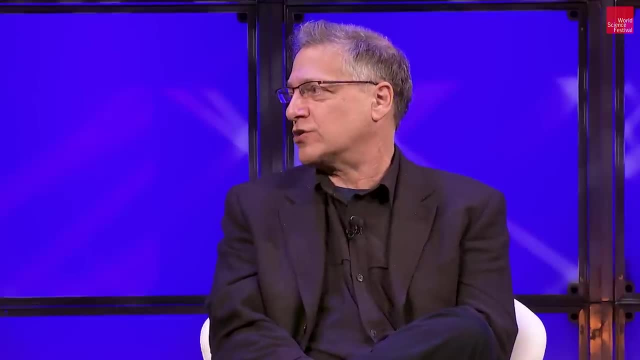 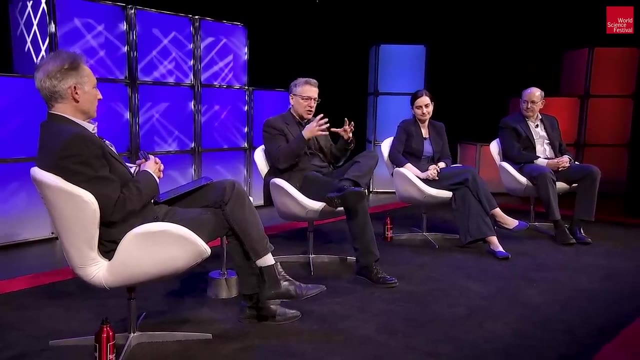 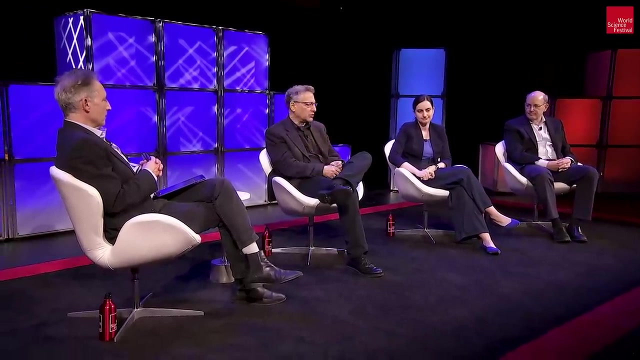 these experiments to do nuclear fusion. all of this requires simulations. So when it came time to look at colliding black holes, you needed these numerical methods that could take you from pure description of independent black holes to this merging process. And those numerical techniques. 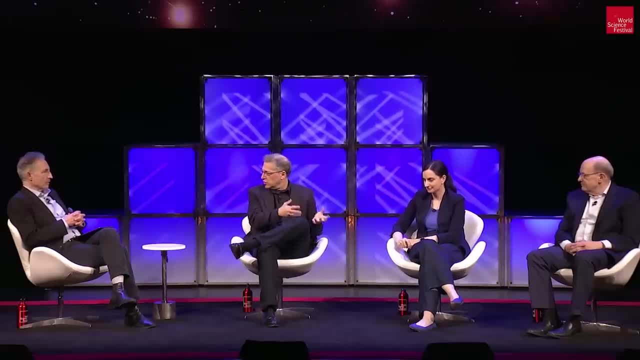 have then been adapted by Anna to look at the early universe, And those techniques were vital to the success of LIGO- right, Vital, I mean. LIGO was like jumping out of a window from a high building hoping you could invent it. 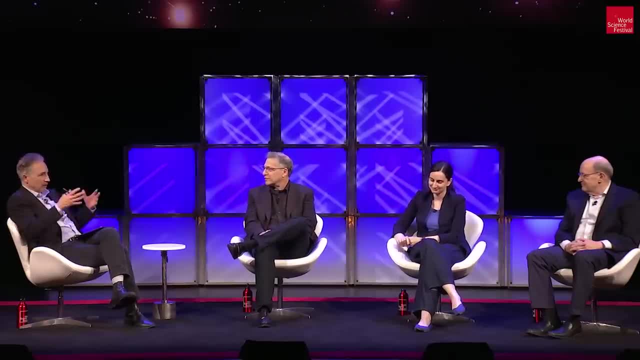 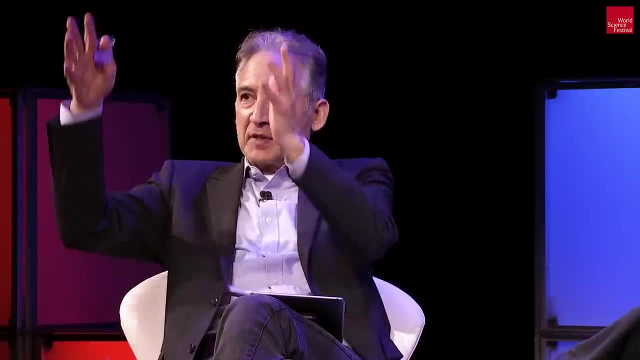 And just LIGO as the gravitational wave detector. I think most people are familiar finding the first ripples in the fabric of space, But when the signal goes by you don't know what it means if you don't have some library of simulations that you can compare. 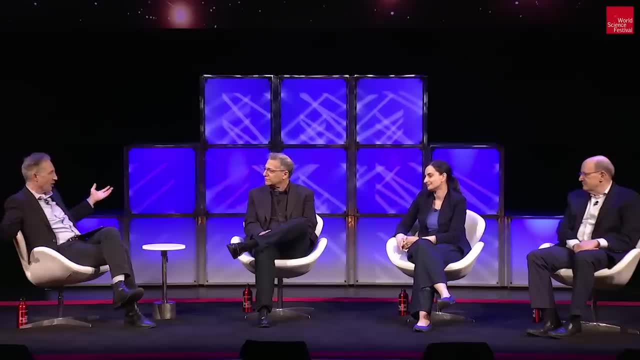 the signal to. So without those simulations it would have been lost on us that the signal had even been found, Absolutely crucial. And in so many areas of science and in LIGO you need these numerical simulations. So there is a kind of 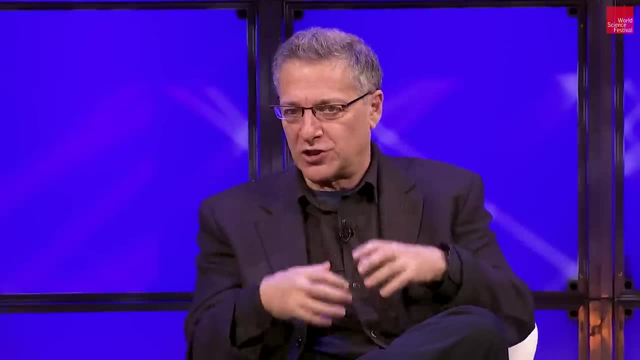 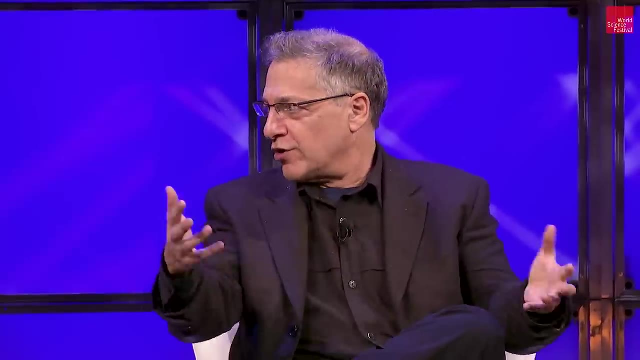 there's experiment or observation, there's theory, and there's this teradium quid, this third thing, which is simulations, And that's the world of science that we live in now in more and more areas. So I think that's a kind of background. 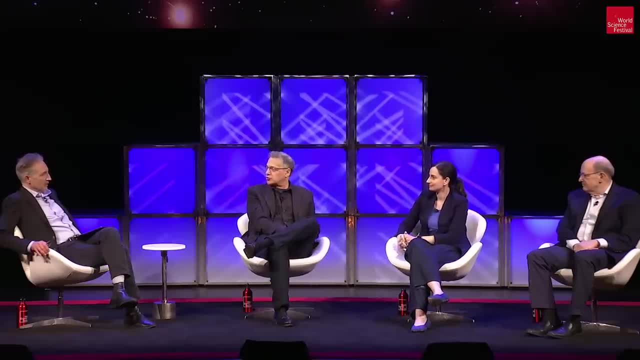 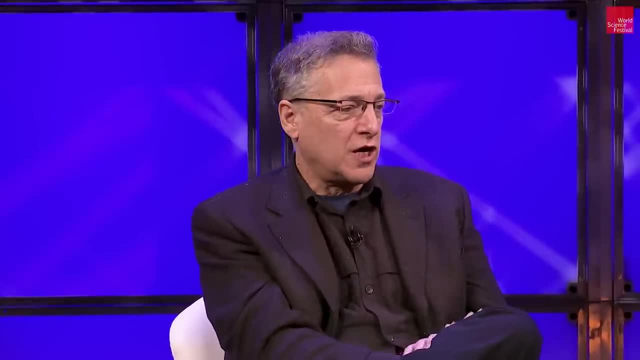 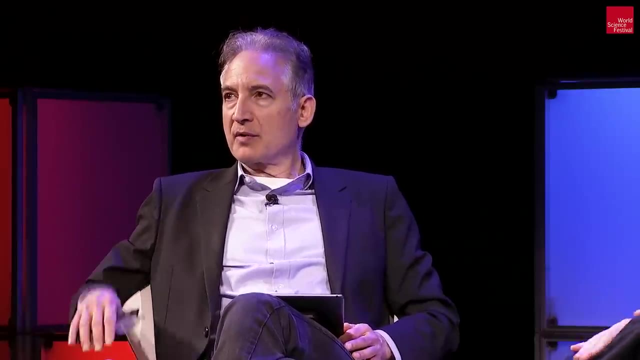 to the important work that Anna's been doing to try to give us a picture of this very, these gravitational intense moments in the early universe and how it works. So this quick little simulation that I think we already saw, but you can run it again. 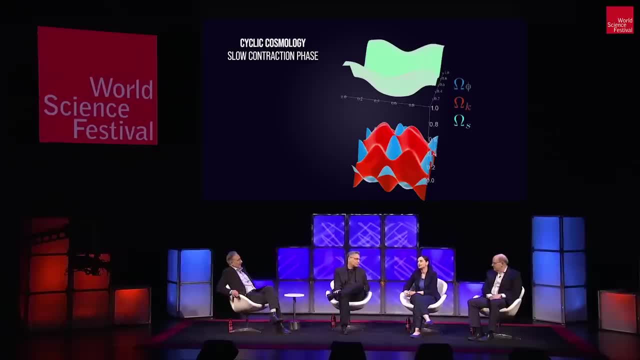 tell us what it is that it's meant to show us. So just one. you know two sentences, maybe because we swallow it so often. So we should appreciate that we have relativity. for over a hundred years, Yeah, But it took almost 80 years. 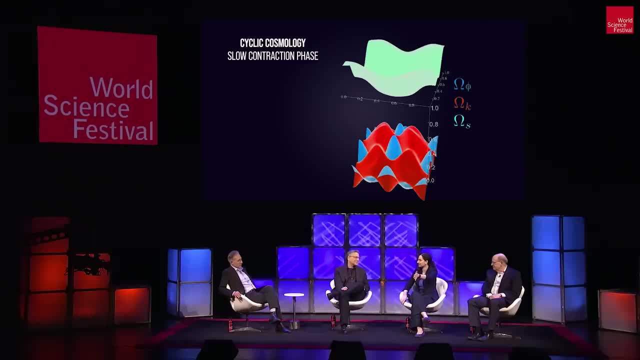 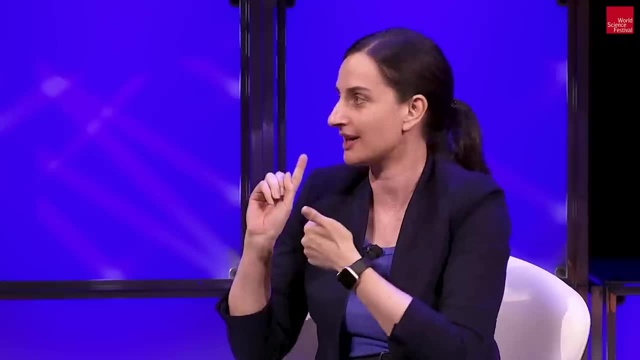 since we had relativity to put the equations on the computer. Sure, So this is really difficult. It's not because that's one thing that we didn't immediately have the computers, but it's required a lot of math and a lot of computational skills. 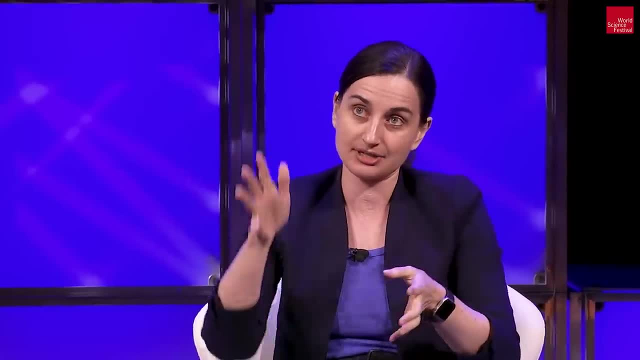 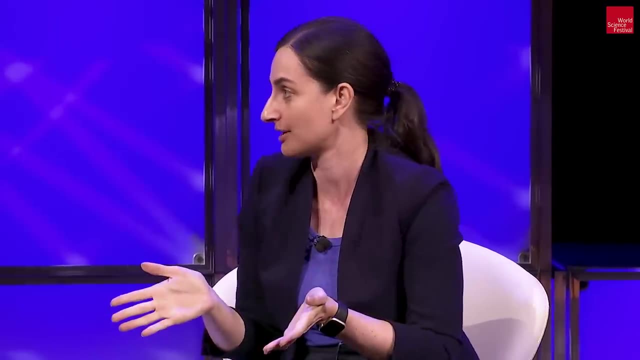 So it's amazing that we have it, Yeah, And then we first did it for black holes, And then what we also figured, and this really actually leads back to where I was stuck as a student with inflation and that simulations are crucial. 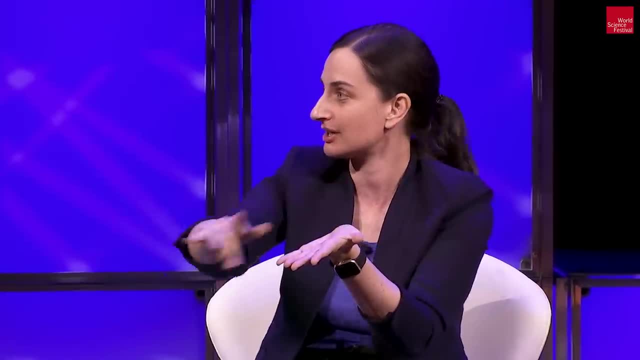 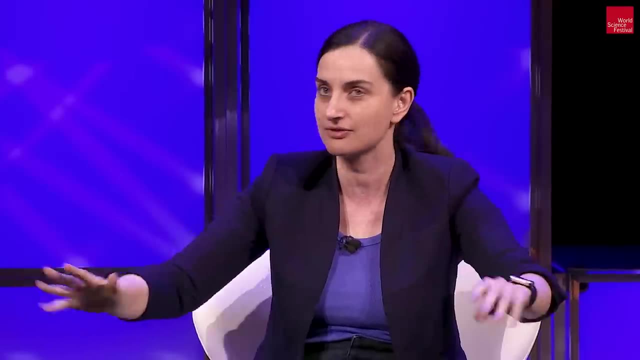 So can we really check that a theory is starting from arbitrary conditions, Arbitrary initial conditions, Arbitrary conditions, arbitrary distribution of energy, arbitrary initial geometry, So we can test what would be after the bang and we could test what kind of condition- a contracting universe. 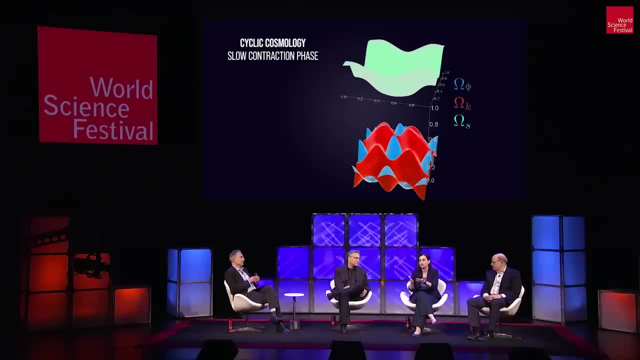 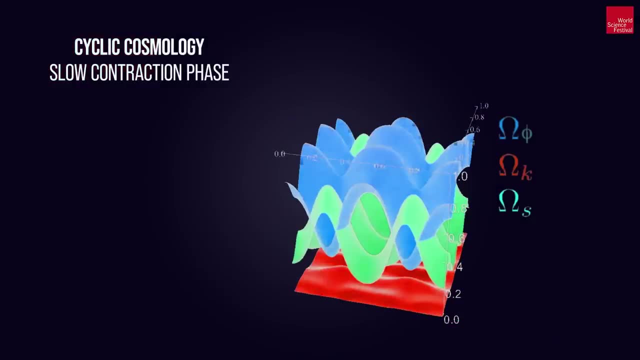 could start from, And this is exactly what we can do. So that's one example of the simulation of this. This is what we see there. We can see it repeatedly, but I briefly describe what happens. So we take the Einstein equations and put them on the computer. 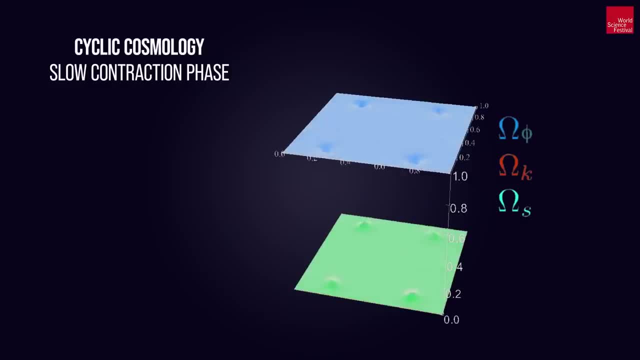 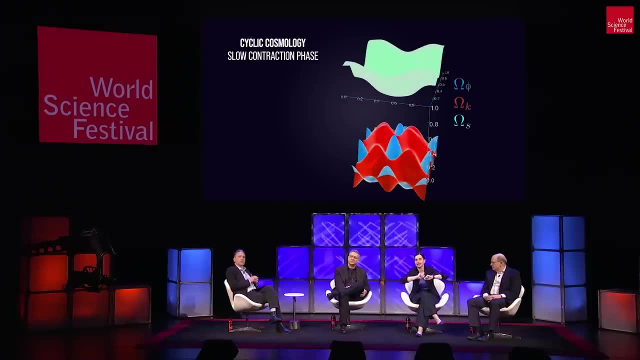 And the feature of the Einstein equations is that you can give them some initial distribution of matter and initial distribution of geometry. So it can be, and that's what we see there. So we see that these omegas, they just represent distribution of curvature. 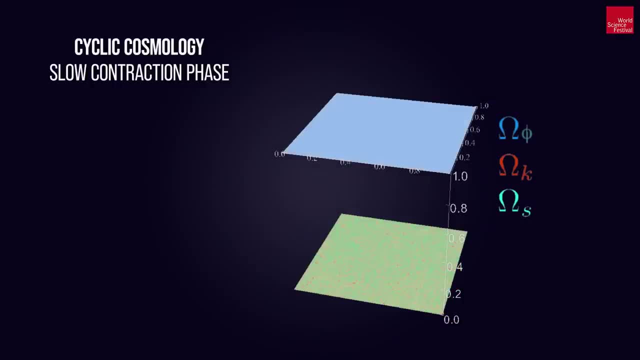 We talked about curvature. That would be: if it's flat, then it's going to be good. If there is no curvature, then it should be at zero. So down there there should be a sheet, And the same is true for this omega s. 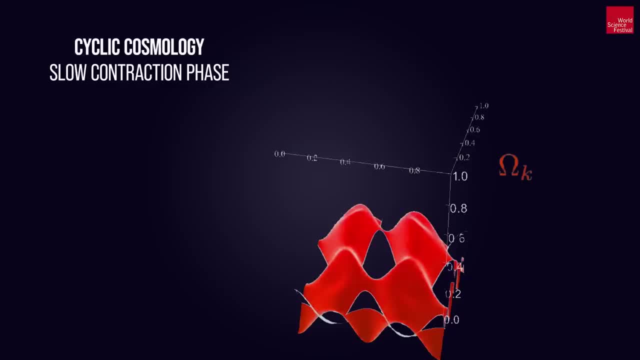 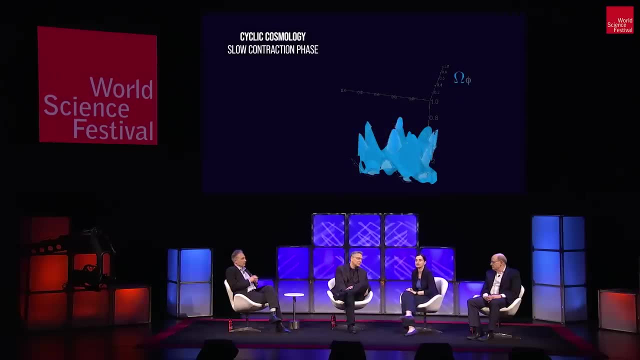 which is anisotropy. So curvature would tell you gradients, how directed the geometry is, how much directedness is, how much it matters which direction you look, And anisotropy would tell you how much shear there is in the universe. 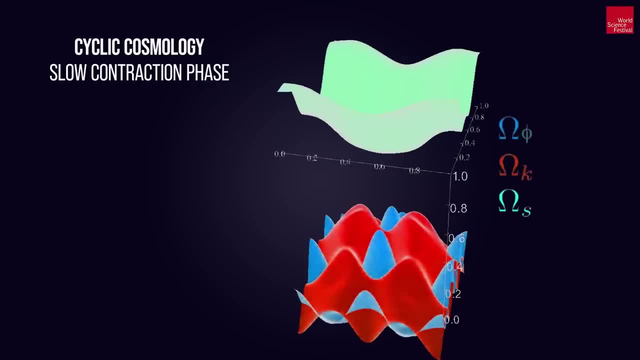 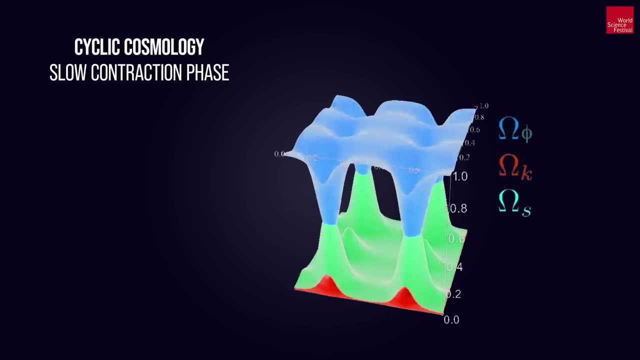 So we know that there are almost infinitely many such geometries possible at the beginning of the contracting phase, And what we see is that it's a good theory. if, whatever we give to the universe- lots of shear, lots of curvature- It all goes away right? 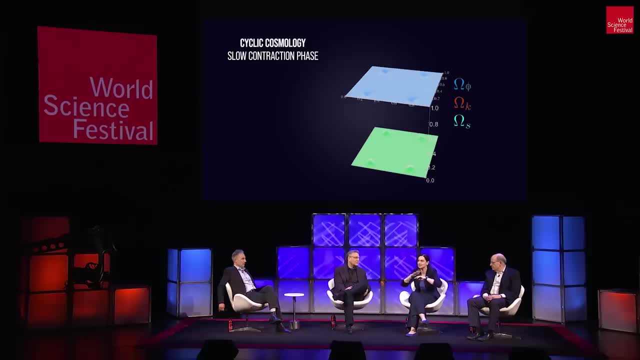 It should go away, Okay. And we only can do this, only can test all these universes by simulations, So we cannot rerun our universe And that's what it shows. So, if you, it's very quick, So it is. 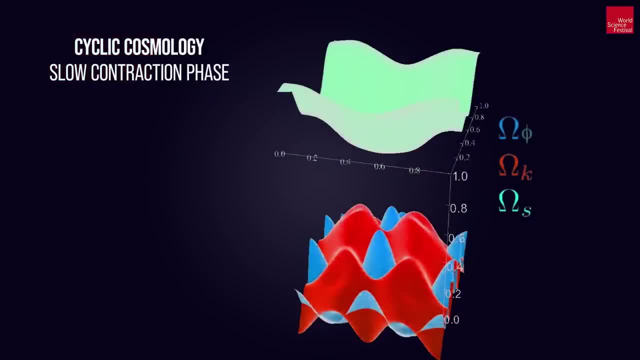 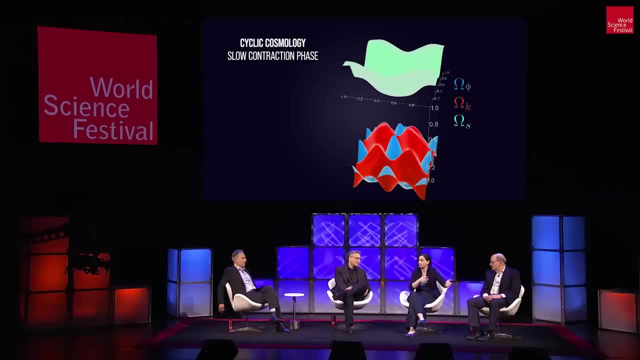 and this is amazing because that's one of the thing is. so this is a representative example of a very curved and a universe which is full of shear. So we thought, people thought in the 50s, 60s- it would definitely lead. 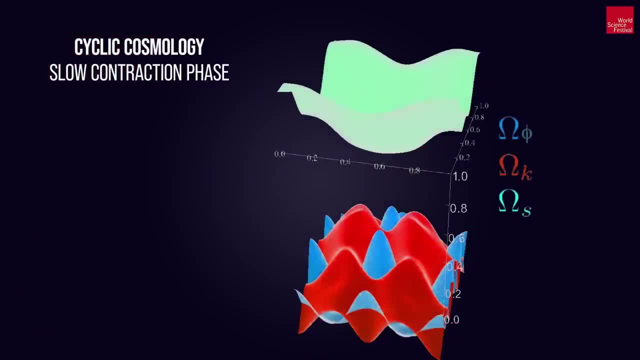 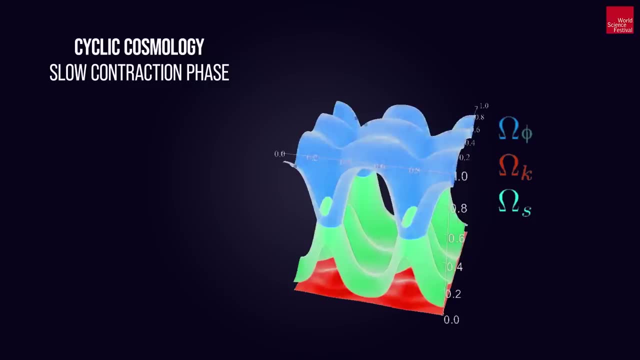 to this chaos. But now we put in this third ingredient that we talked about, the scalar field. Yeah, That should do this magic that while space hardly contracts, the region of causal connectedness just shrinks down. And if that's true, 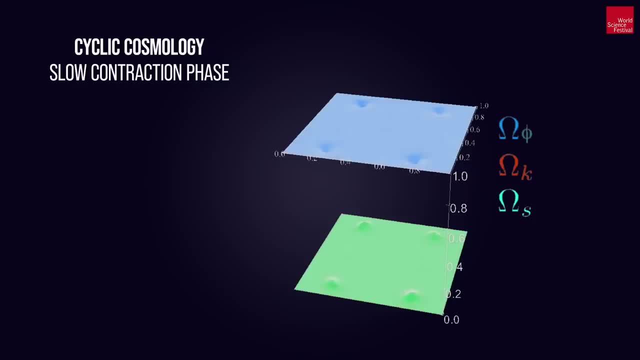 then what one would see is one sheet up there which is blue, completely uniform, and the sheet of curvature and shear just vanishes at zero. No contribution to the energy density. So this boring outcome of the simulation is actually already in our universe. 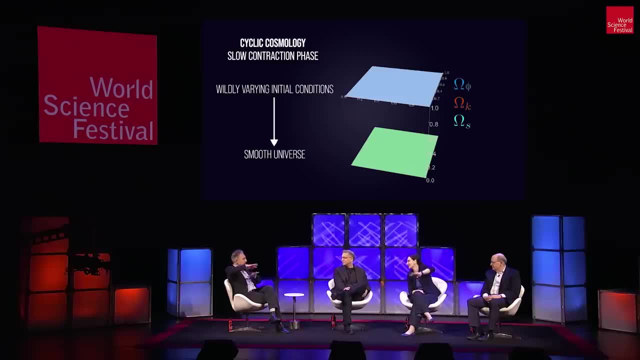 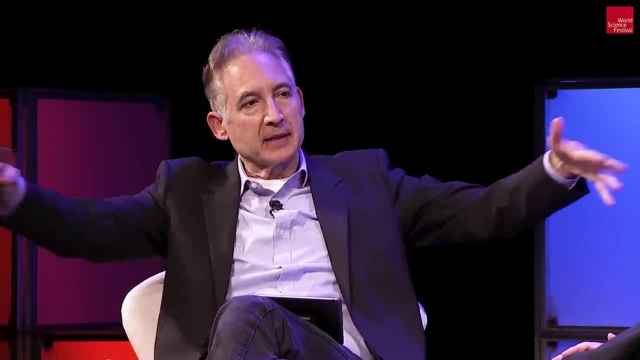 So we do a lot of work to see something boring at the end. So the fact that it's nice and flat at the end tells you that regardless of what chaos you had before it got to the end of the contraction phase, it gets resolved. 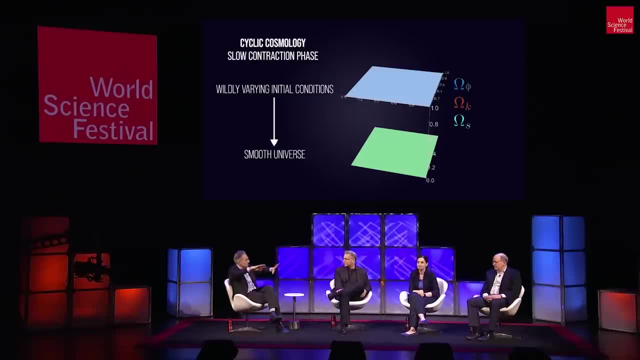 wiped out and you've got a nice placid starting point for the expanding phase. Now It also shows it's really fast. It does go a little bit fast, yeah. So on the one hand it's disappointing. You'd like to see. 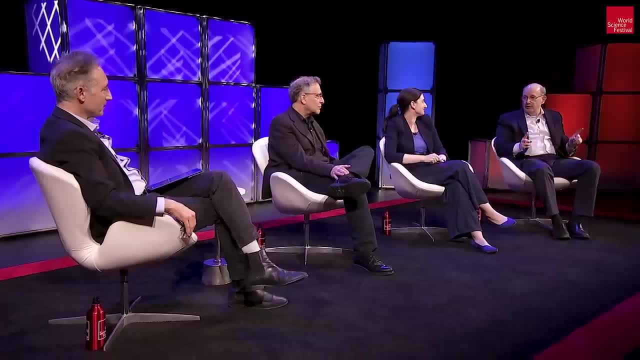 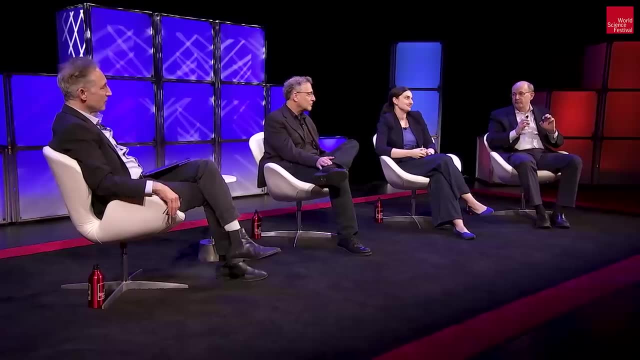 a simulation which has a lot of action, Yeah, But there's actually a really important message there: that this slow contraction compared to inflation is very fast in smoothing the universe, So it's very effective at doing what inflation itself is claiming to do. 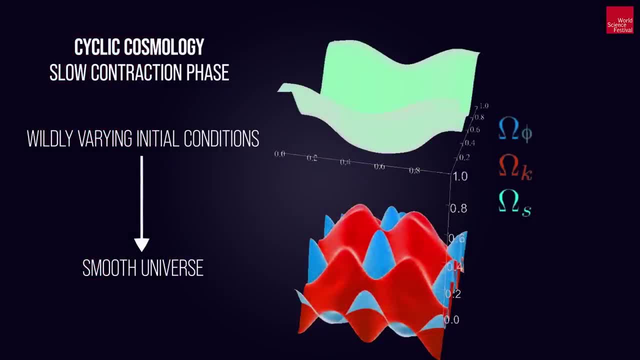 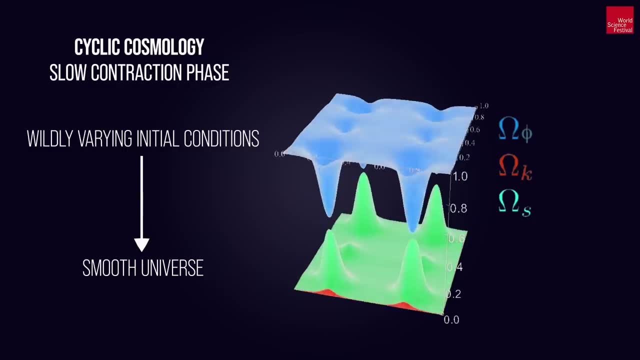 So the universe only has to contract by a factor of two to produce enough smoothing and flattening to take us from a wildly inhomogeneous universe to a universe as smooth as what we see in the microwave background. So you view this as a strong piece. 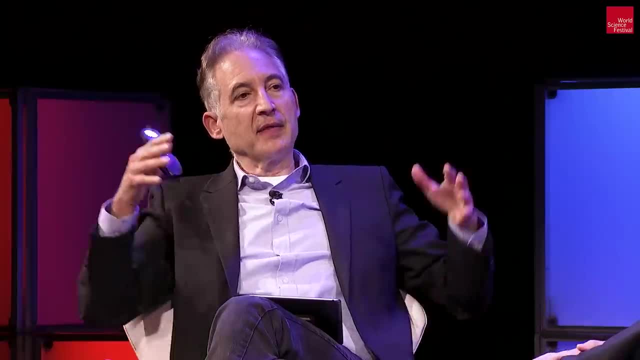 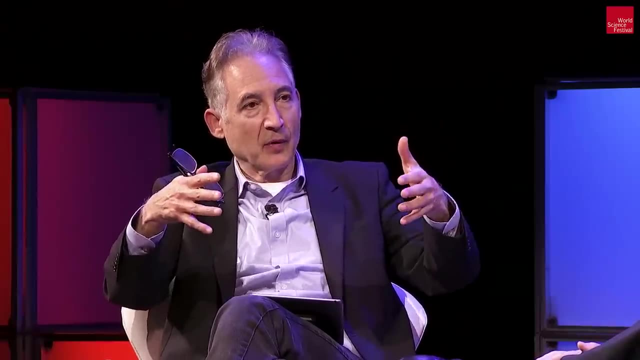 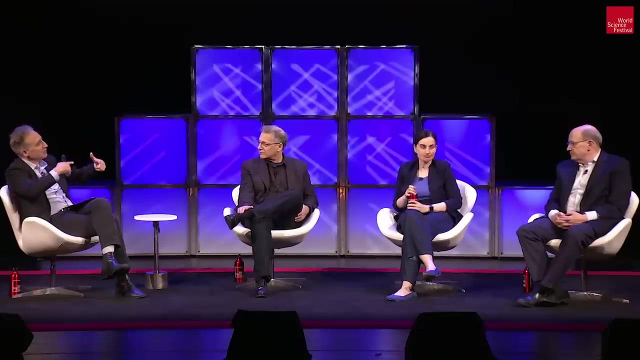 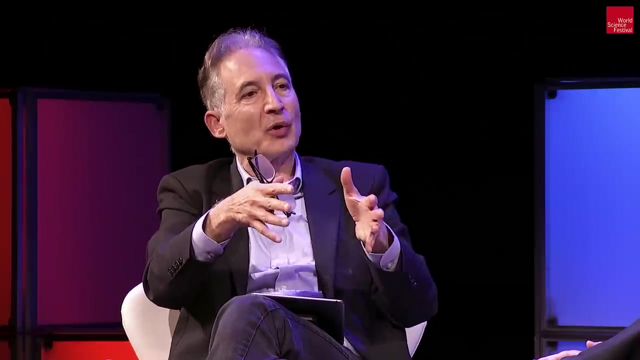 of simulated theoretical evidence that a period of slow contraction does the work necessary to set us up for an eventual evolution that yields a universe like the one we're familiar with. You have some simulations that I gather also take a look at the inflationary model to see whether it does the work. 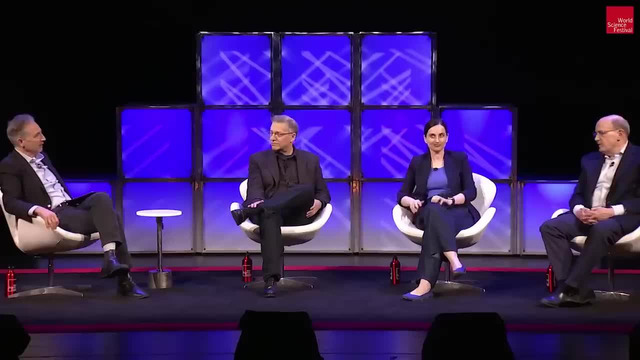 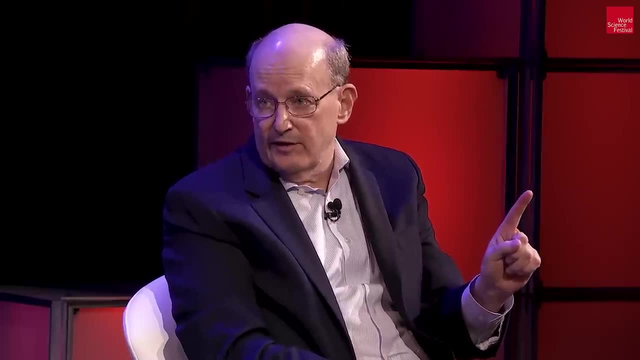 that it was claimed to have done. So I think we have that on hand. But before we do that, I want to make one other point, Please, Because we discovered something in these simulations that we didn't anticipate. Okay, So when you saw, 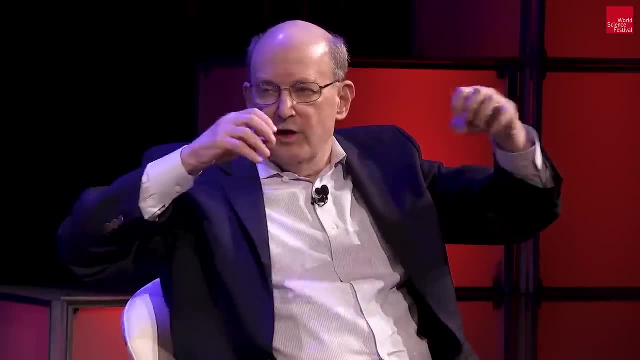 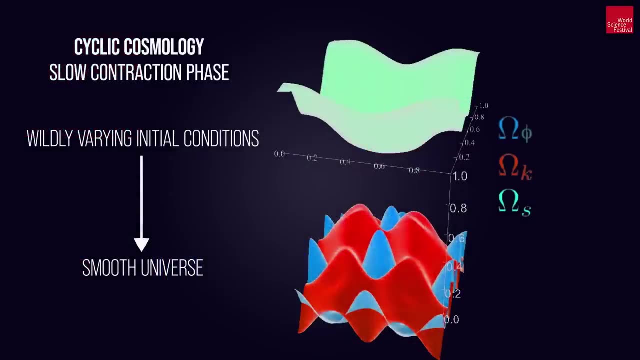 that originally curvy sheet that's spanning directions, regions of space which are not in causal contact, And because the contraction is so little, in fact they never become in causal contact. Yet somehow, magically, we ended up with a smooth universe. 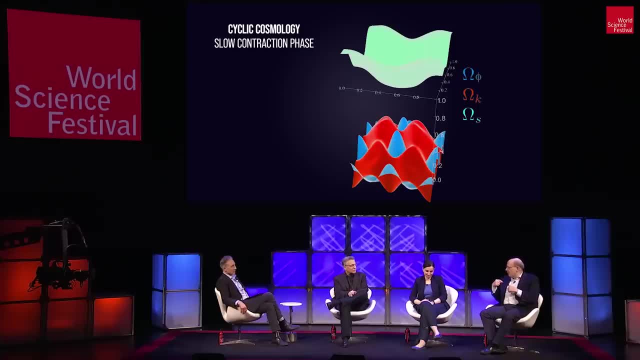 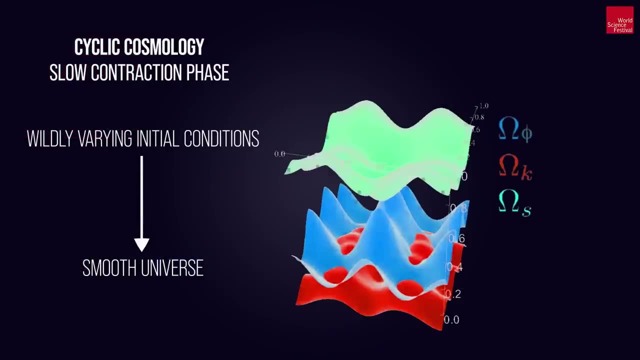 This changes our. this goes back to our assumption that we thought we needed to put things in causal contact in order to smooth them out. That's true in an expanding universe, That's your only hope in an expanding universe, But in a contracting universe? 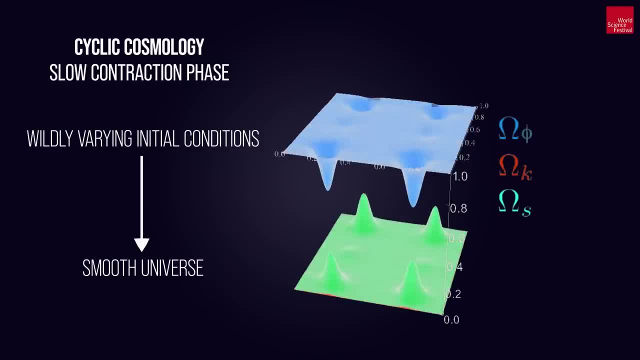 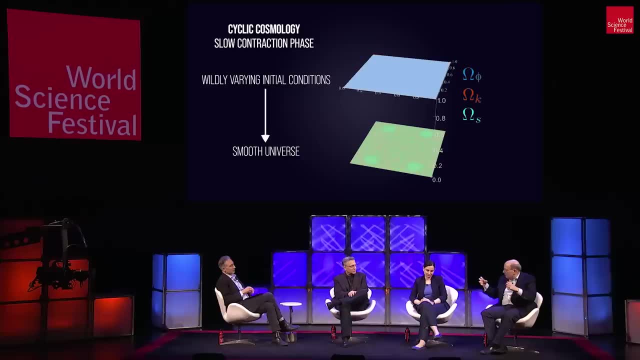 what happens is that different regions of space will independently smooth of each other, even though they're out of causal contact. In fact, what happens is, because the horizon shrinks so little, very quickly all points become disconnected from one another, which means 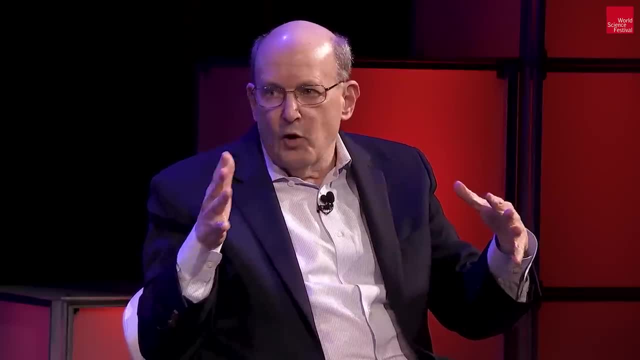 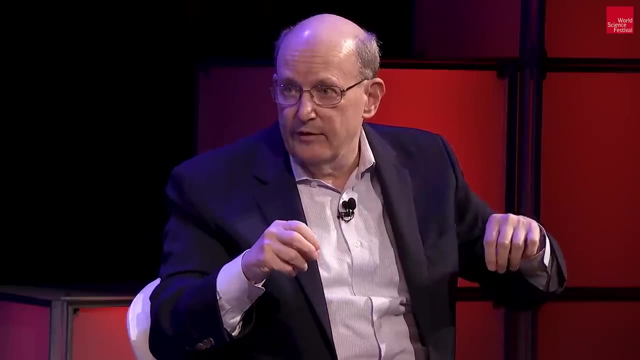 that the equations that they follow now don't depend on their neighbors. They only depend upon what's left after you ignore your neighbors. That's the same for every point, And that's why they converge so rapidly to the same final thing. This is a new phenomenon. 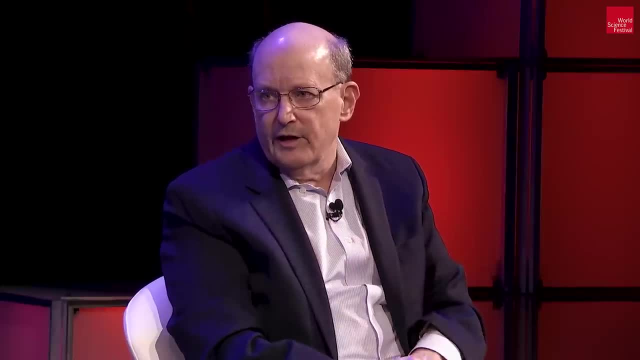 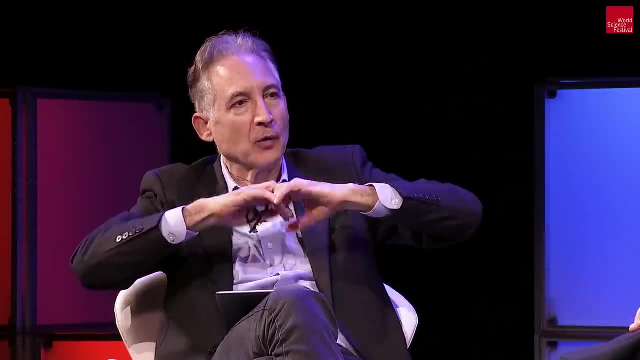 Right. We call it ultralocality in the context. in this context, I see. So they're all dynamically going to the same state, as opposed to interacting in order to negotiate. coming to the same state, That's right. They don't have to negotiate. 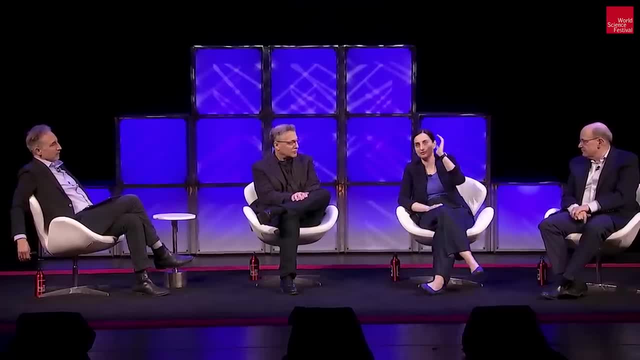 And it's really important. one point, because you know we tend to always think Newtonian. But you would think if something contracts, it collapses. So it's the opposite of what's happening. So it becomes more messy, not local. 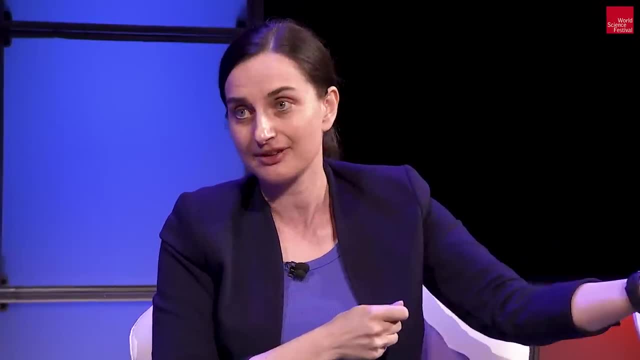 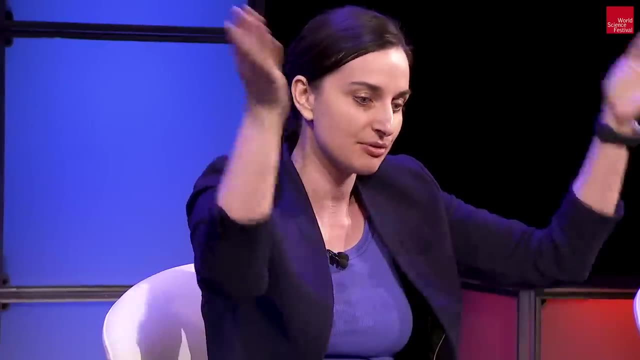 But what we discovered is that's really Newtonian. And now you see, when you simulate relativity, how different the universe that's governed by gravity is governed by relativity and not Newtonian physics is because contraction doesn't have to be collapsed. 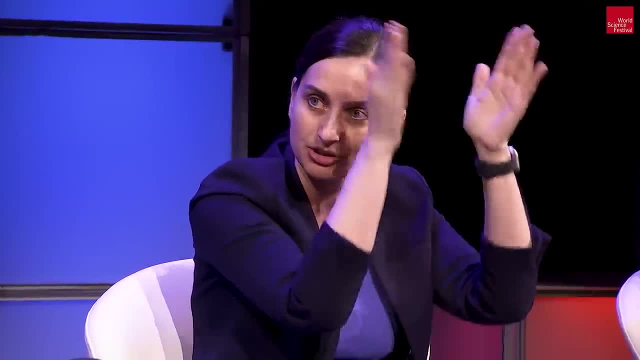 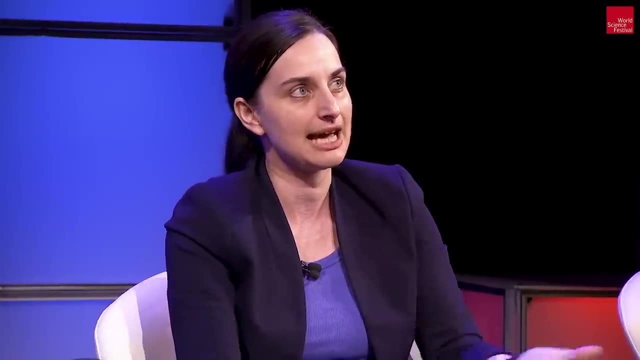 It's actually you know the directionality. this mass vanishes, All curvature goes down. So it also represents that, you know, our picture of gravity really has to be radically revised whenever we, whenever relativity is important. So contraction. is not collapsed, and that's what the previous simulations show. And that's the reason why everything gets smooth, Because you know you just cannot. a contracting phase is exactly the opposite, as you would expect. It doesn't mess things up, but smooth things. 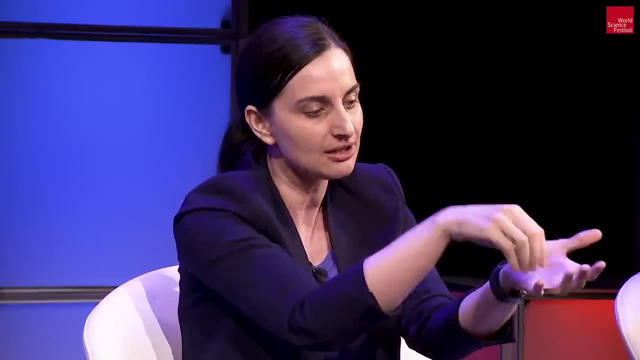 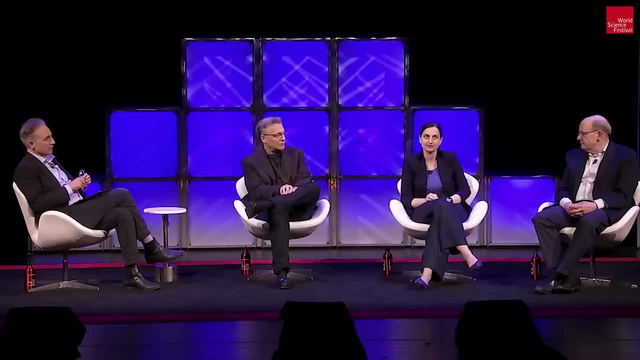 And you cannot help it. no matter where you are, In every little causally connected space, we look the same, because it cannot do it otherwise And it's it's done to relativity And that's very different, as Paul will, I think. 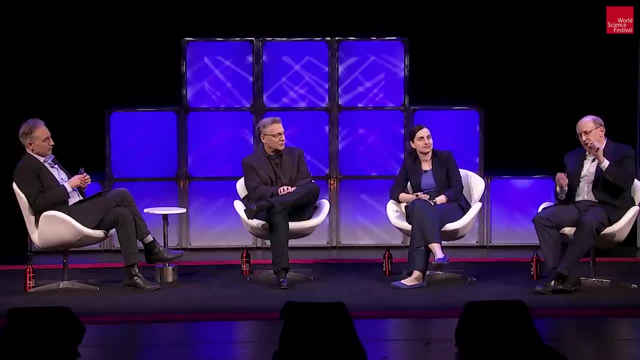 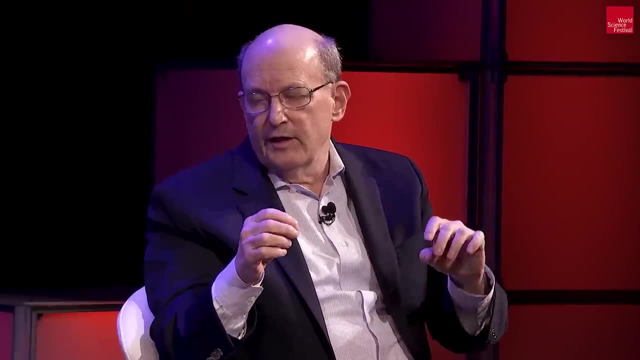 explain in inflation Right And it, and part of one of the things that happens there, I said, is that neighbors become unaware of one another. So in terms of general relativity, that means that what we call gradients, the variation, 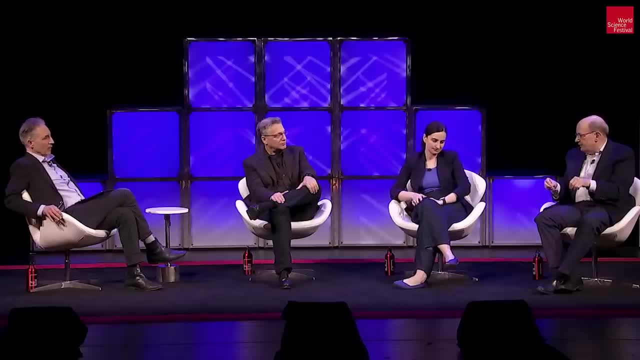 from point to point, they'll become irrelevant. Every point is operating independently, Right, It's a feature of contraction, So now we can turn. well, what about expansion? Yeah, What happens there? Well, our intuition had about inflation had been. 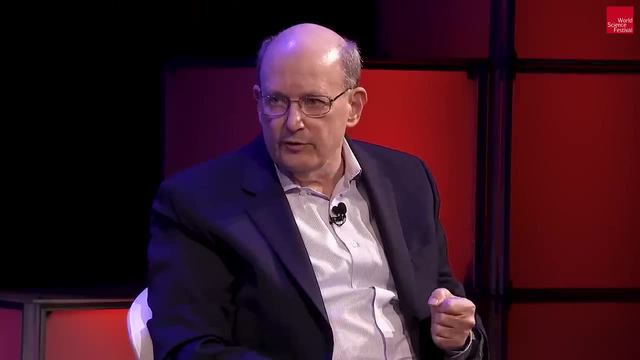 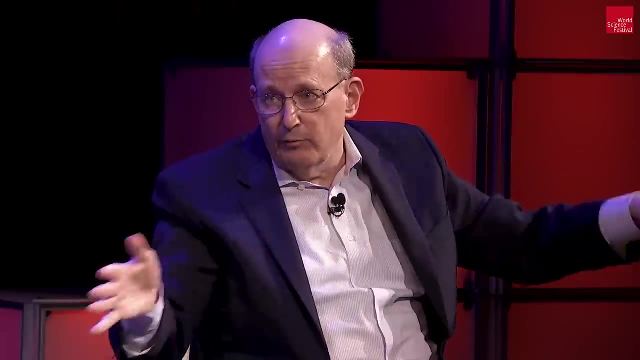 if we began with some very inhomogeneous universe. okay, then essentially, what inflation does is stretch it, Yeah, And as it stretches it, if you think about a curvy rubber sheet, it's and wrinkly rubber sheet, you think it's going. 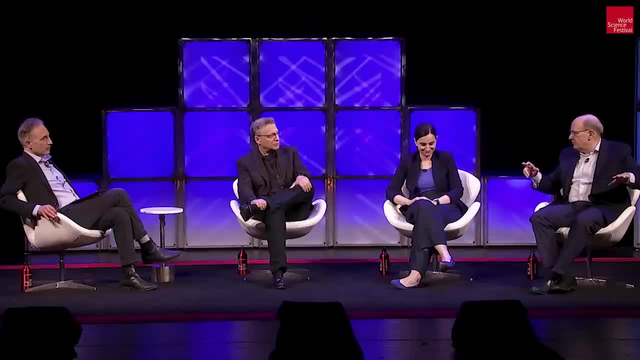 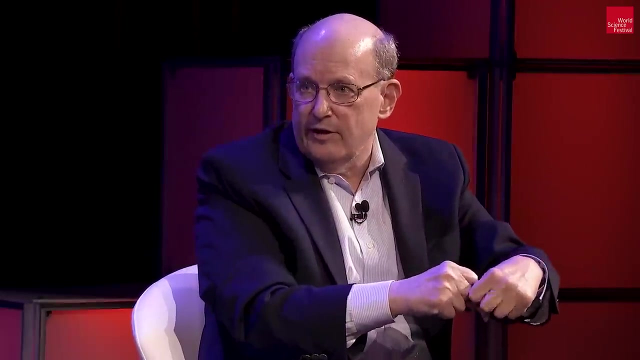 to smooth it out. But that's a very bad metaphor for general relativity, because in a rubber sheet those wrinkles don't resist the expansion. But in general relativity a wrinkle in space-time has stress, energy that gravitates itself and wants to fold itself up more. 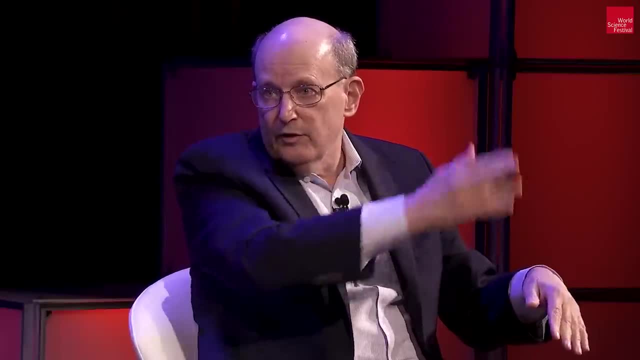 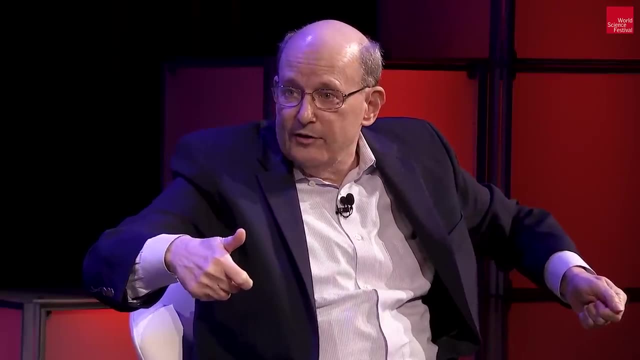 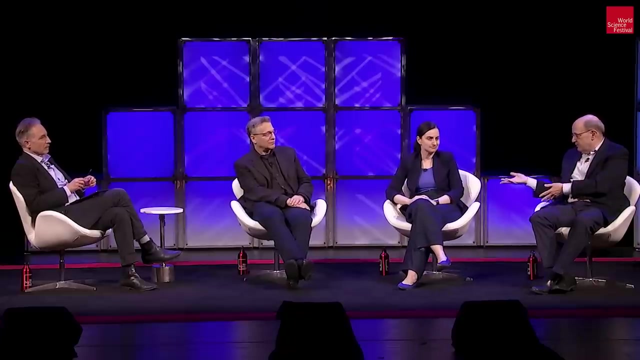 So what you really have is a competition between whatever wild initial conditions you have that want to fold themselves up versus whatever is trying to inflate, And the question is which one wins? Okay, So now we've taken the same techniques that Anna developed for contraction. 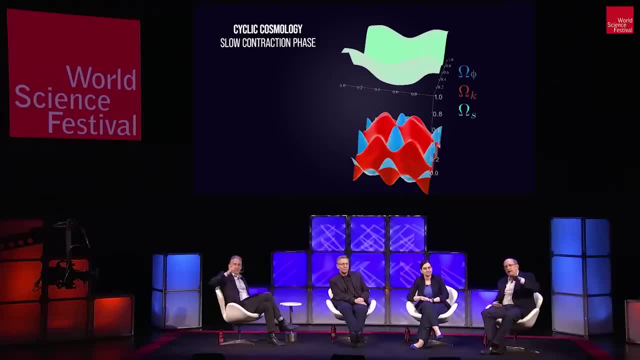 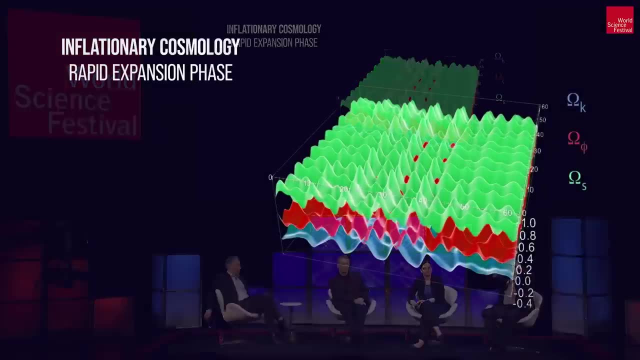 and then she repeated it for expansion. Yep, Again, we're beginning with a universe like before, with. the green represents how much shear there is in the universe. So it's almost all shear in the universe. The red represents how much matter and the blue represents 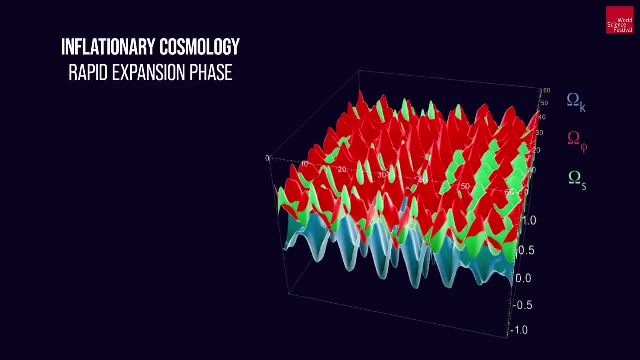 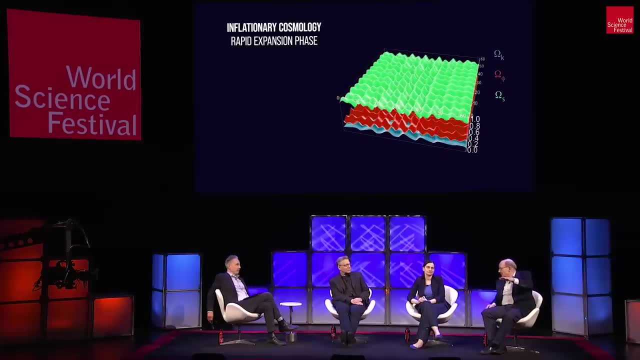 how much curvature you have. And so if you go back to the beginning, Go back to the beginning again. Now you begin with a different vantage point, because in this case the opposite happens than what we saw in the contraction case, where everything's smooth. 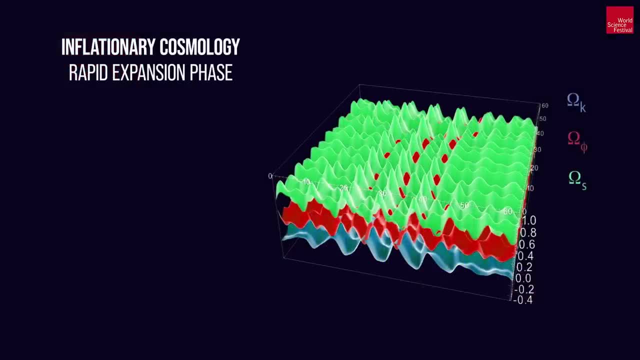 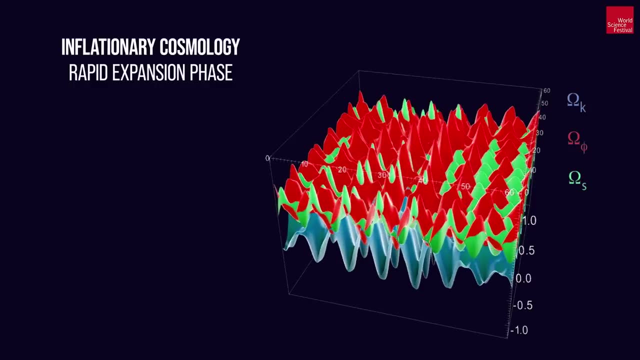 Right Now, what happens is things get wilder and wilder and wilder, and that's because it's just for the effect I talked about. If your initial variations are wild enough, they actually resist the expansion, prevent inflation from taking hold and, in fact, 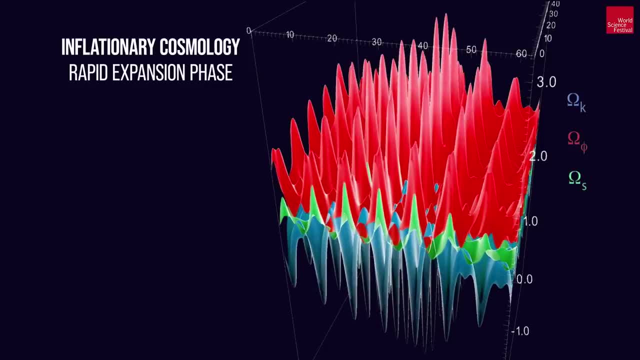 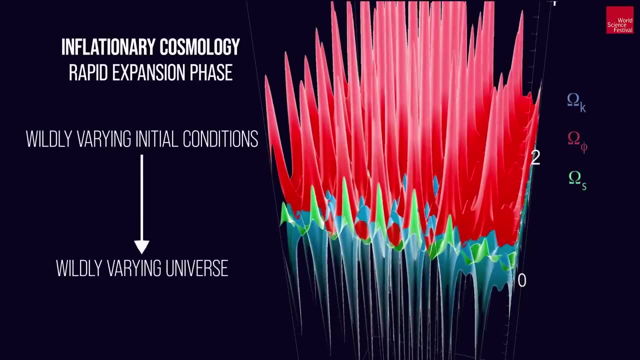 they grow in intensity, becoming more and more resistant to the expansion. Again, that's only possible to learn when we have simulations. We could not have gotten that out of solving with pencil and paper Einstein's equations. And so the proponents of inflation are the ones. 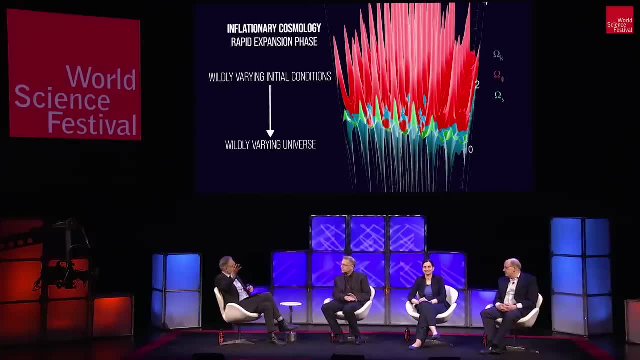 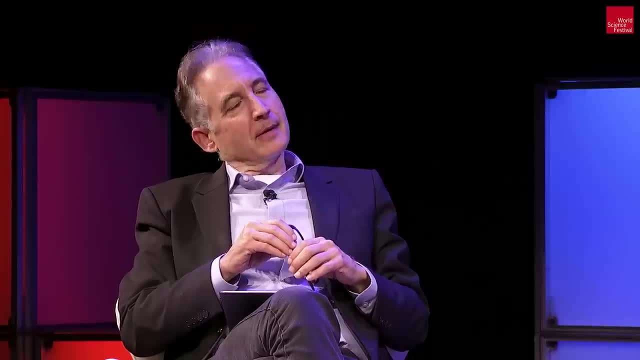 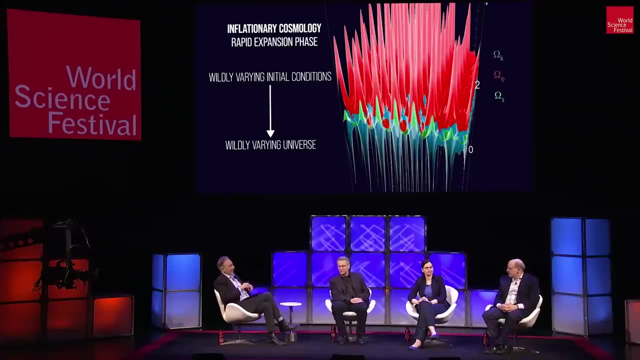 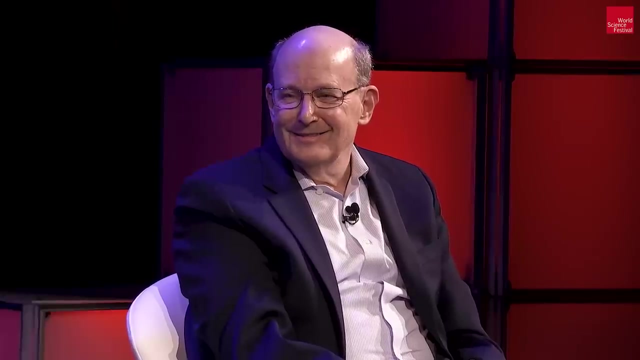 by the variations in shear and curvature. They can never take hold relative to them, because what you see when you see the curvature going way down? But I think you're answering what happens when you talk about the people who are in the inflationary mindset when you've 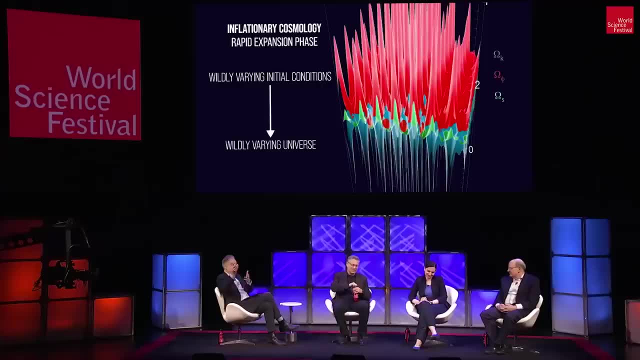 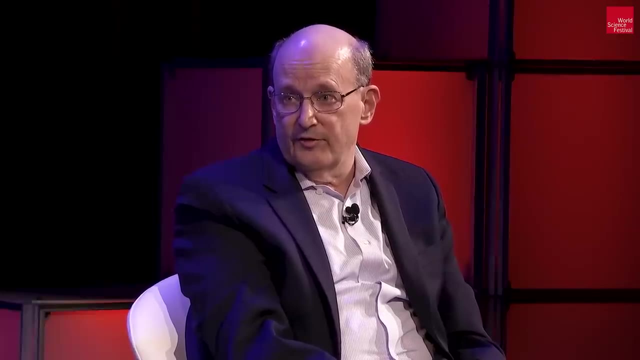 presented these simulations. what's the response? I think it's a little early to say, because what I've shown you here is only a few months old, So the word hasn't really gotten out. to see all the work that we've done on the inflationary. 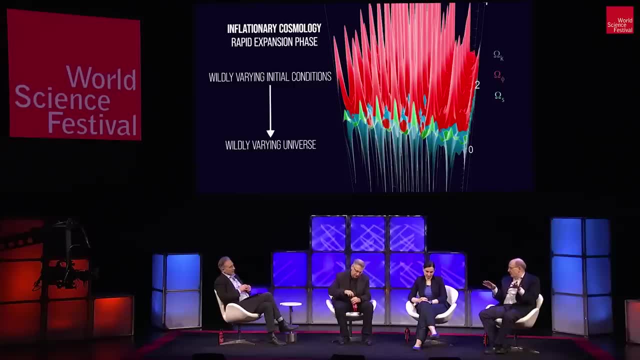 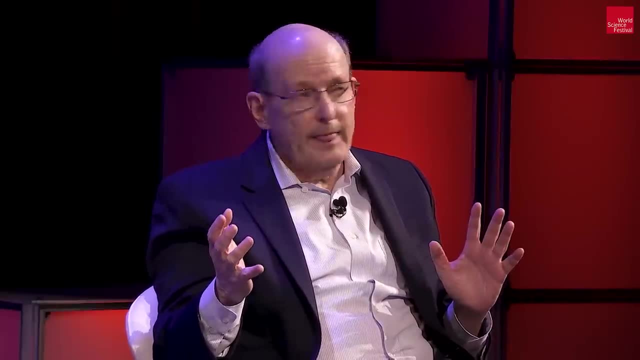 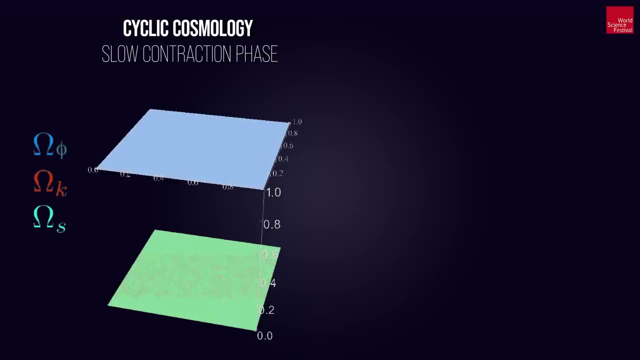 case and to contrast the two. So I think this is something which I hope will be one of the things that contributes to people opening up their minds to the idea that slow contraction really is a powerful smoother, for the subtle reason that I called ultra locality the subtle feature. 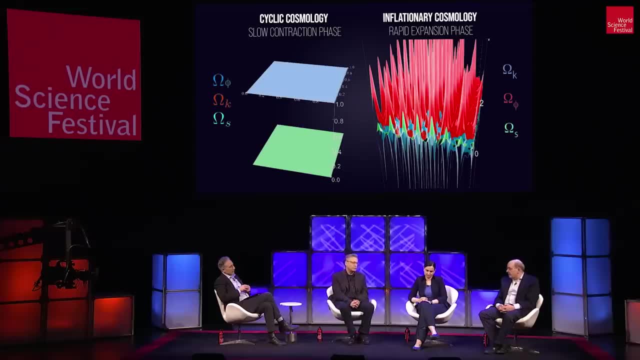 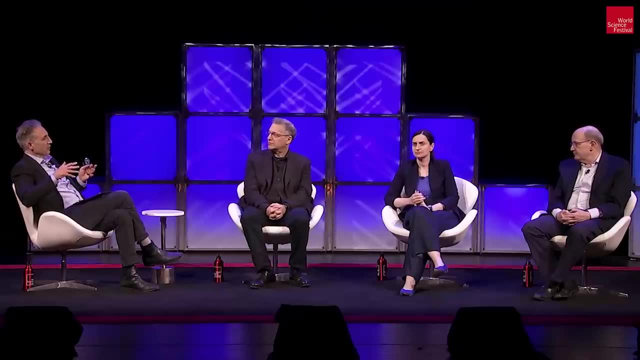 of general relativity and the converse of that is that it's a challenge or problem for inflation. That inflation, unless you begin very close to smooth to begin with, is not looking under the hood right now. Can you give us a feel for what kind of assumptions? 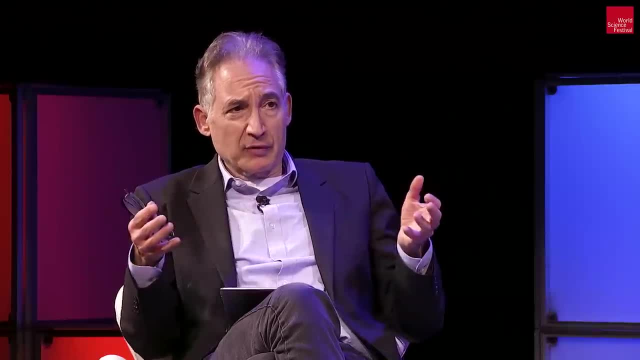 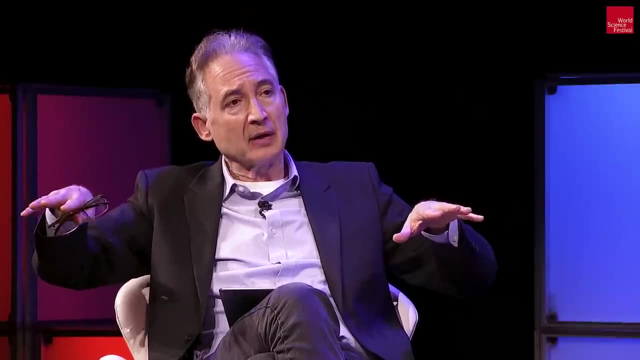 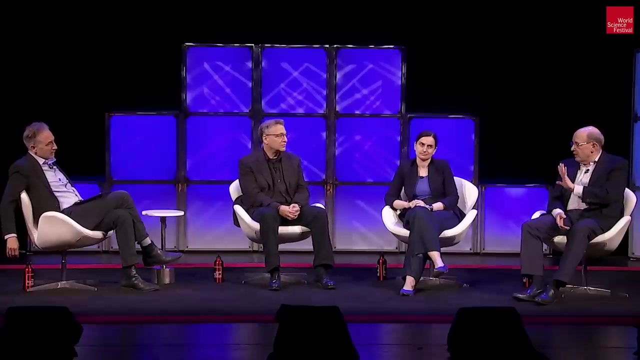 go into this. Are you making a variety of choices of the behavior of these fields that are driving part of the dynamics here? How generic would you say that these results are? Yeah, the basic thing, the basic quantity and curvature, which are already part of general. 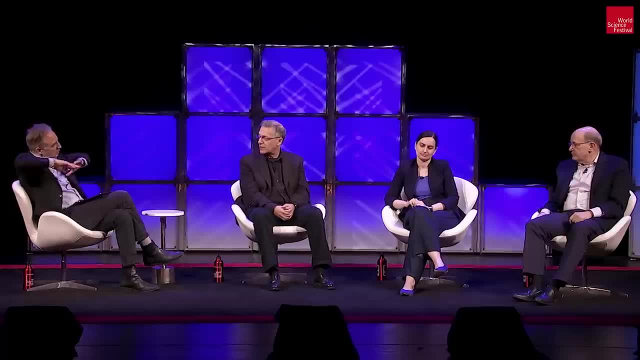 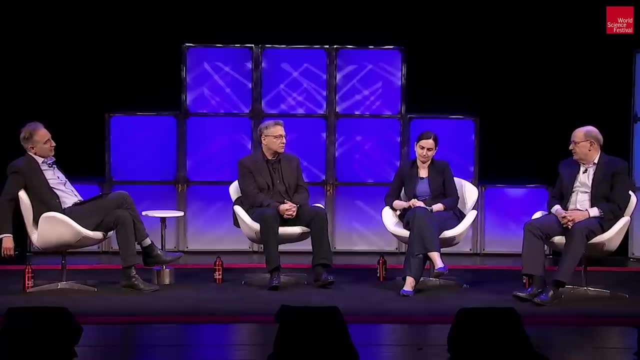 relativity, the component, And just to give people a sense of shear, it's the way in which space is in some sense pulling on itself, Stretching this way while pulling this way, or something like that. The same effect that gravitational waves produce when they pass through a detector. they stretch it in some directions and contract it in other directions, and so that's a kind of- you know, unevenness to space time and would make a difference in the distribution of matter and energy and how everything behaves. So the thing, the component that you're adding, 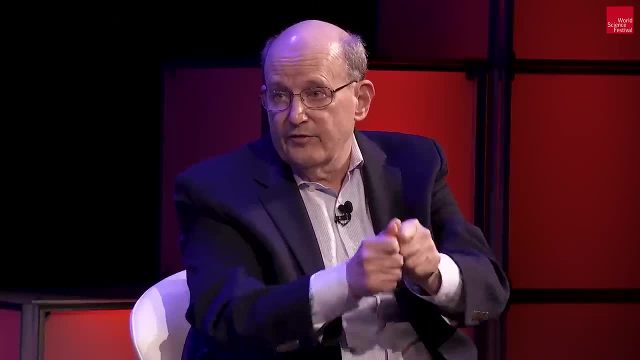 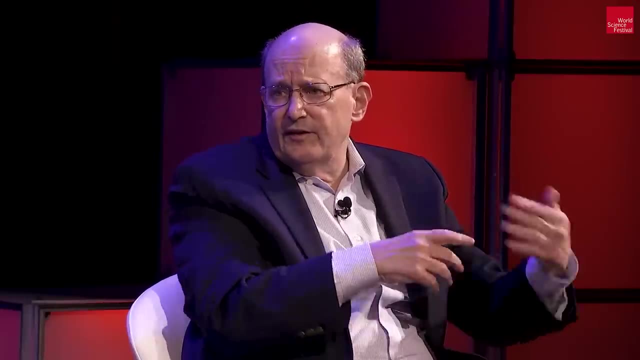 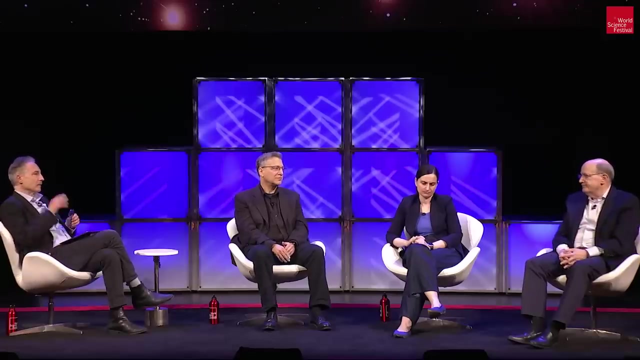 for inflation was a scalar field which had a property that it induced accelerated expansion. Yeah, And here you're doing something analogous, you're producing introducing a scalar field. its details are different, but it has the property that it causes this slow contraction And, in terms 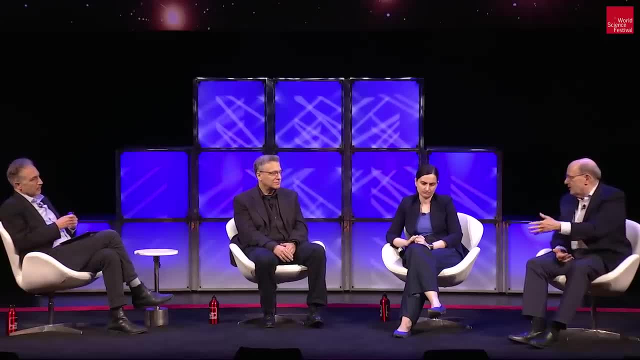 of the ingredient. it's very similar. it's a scale, it's some field. it's just the details of how its energy depends on its strength. field strength- That was what I was sort of driving at. Do you have to fine tune that in any way? 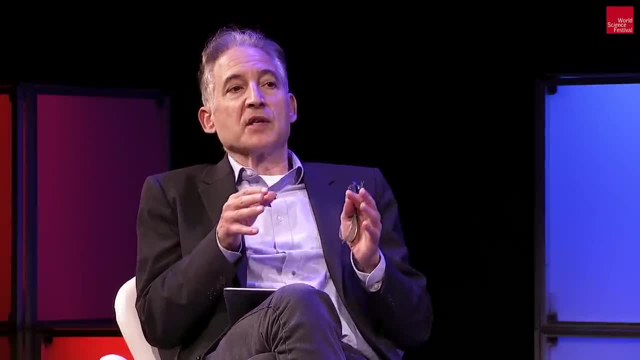 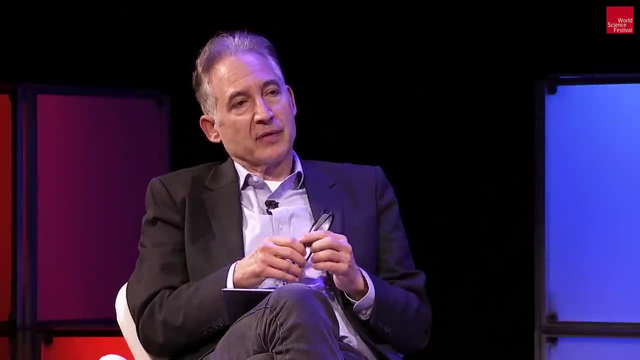 I mean certainly you have to fine tune inflation to make sure that this ingredient gives rise to that energy we were talking about, that can give the repulsive push that drives inflation. How much tuning do you have to do within the theory to make this behave the way? 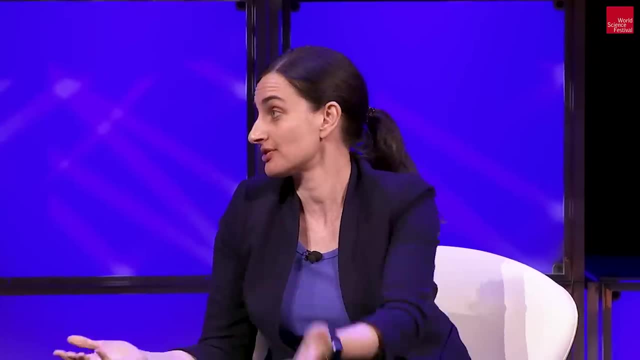 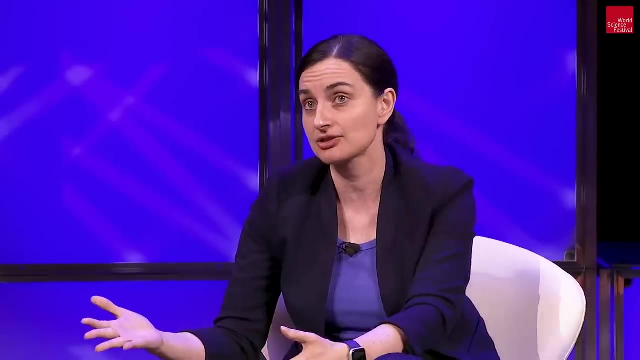 we've just seen, I mean we have. we have studied that You can run these simulations with varying also the ingredients. we call that the potential energy of the ingredient And what's interesting, it's actually relatively insensitive, but I should say that in inflation it's also. 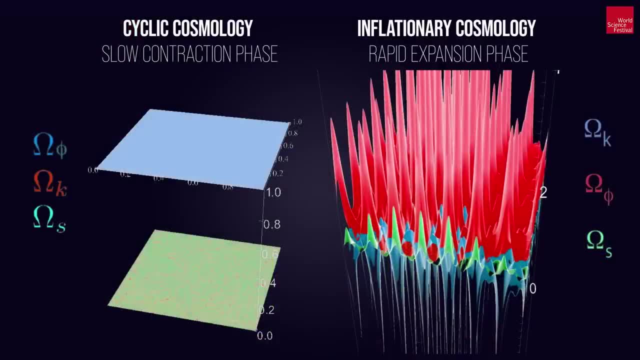 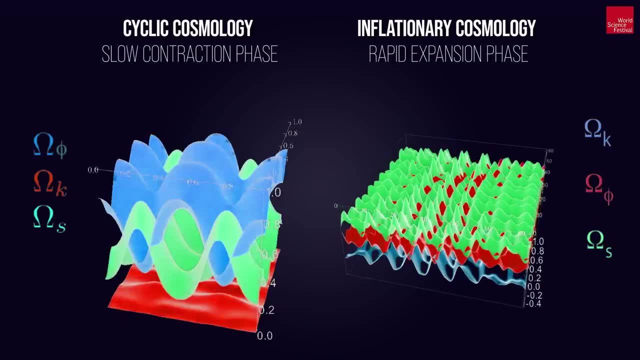 so the two pictures that we saw, they are fairly generic for both scenario. So we did just on the scale of hundreds and thousands. it's very quick to do, very quick to run the simulations. It takes a few minutes for contractions so we could run. 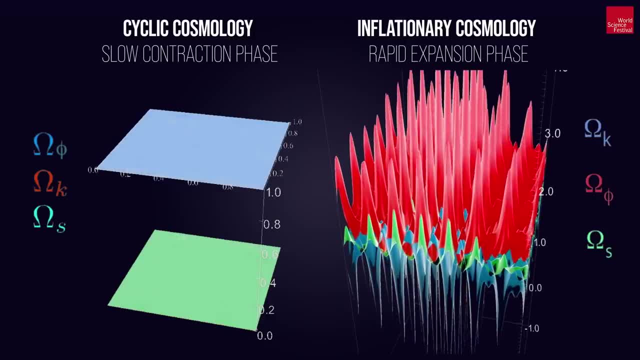 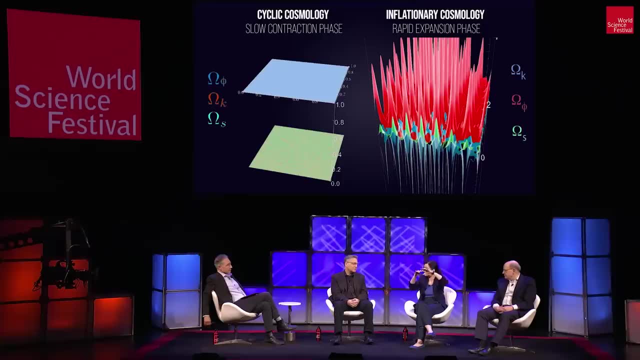 during the last few years, hundreds of simulations. So this is very generic. You don't? really. I don't think that this at this level. it involves the type of tuning that you might need to fit the little wiggles in the microwave background And then in inflation. 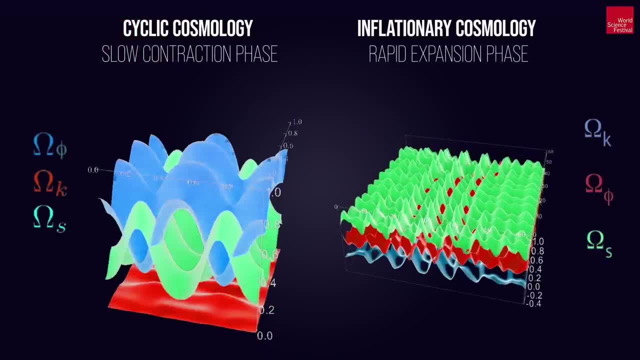 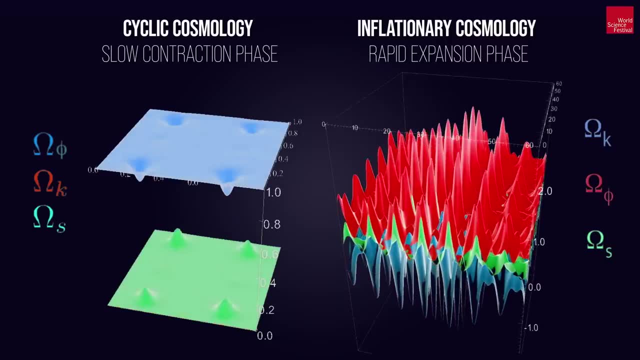 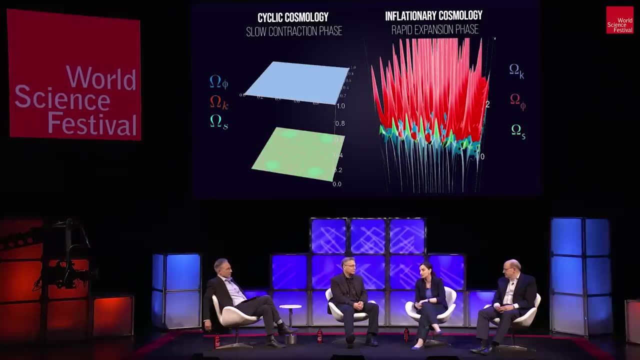 what happens is because it's so complicated it's actually takes much longer to run the simulation. Sometimes the same simulation with the same initial conditions takes a week or more, And but I would say that's also fairly generic. so we have not run also there. 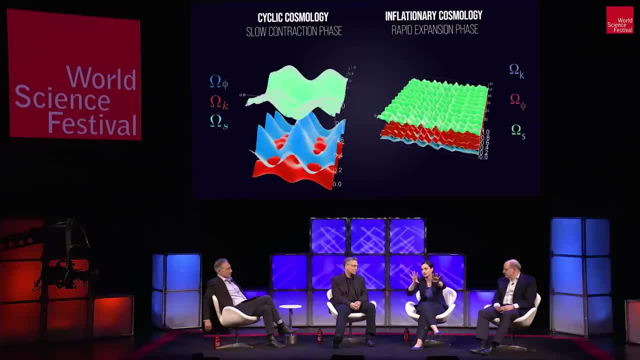 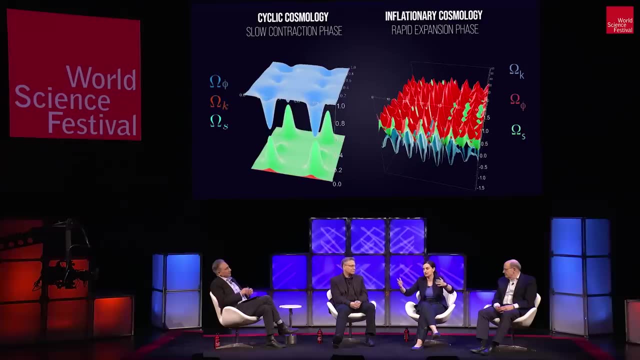 hundreds of simulations with different types of potential and the outcome, what you see, this contrast, that the one smooths and the other one that's not tuned in either case And better tuning comes in, I think is- and maybe we'll get back to this- what the quantum effects. 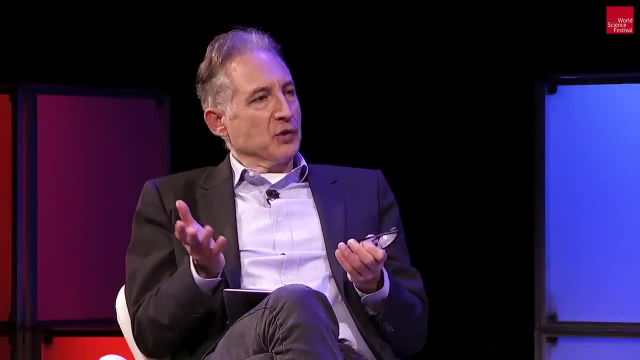 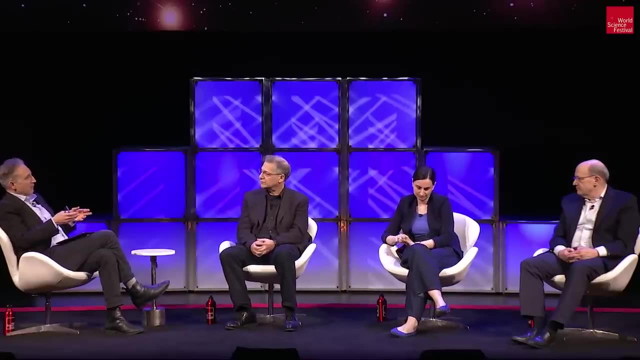 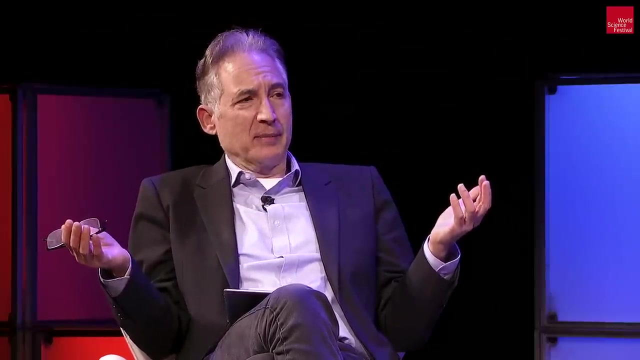 how we moderate the quantum effects in both theories. Now, we called this session reimagining time, Peter. the idea is, if a bounce can happen- and I'll turn to you guys in a moment- maybe many bounces can happen. if many bounces happen, maybe time 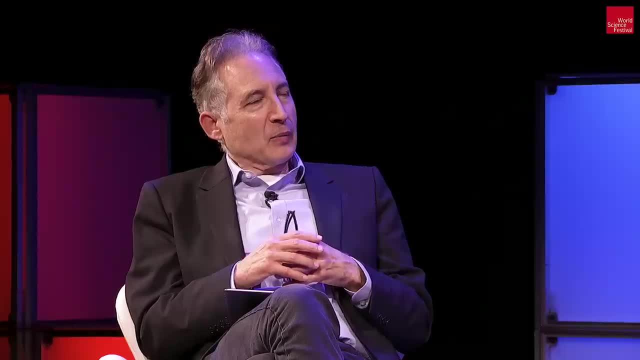 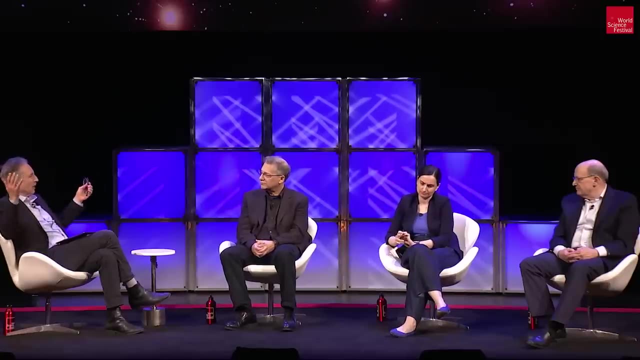 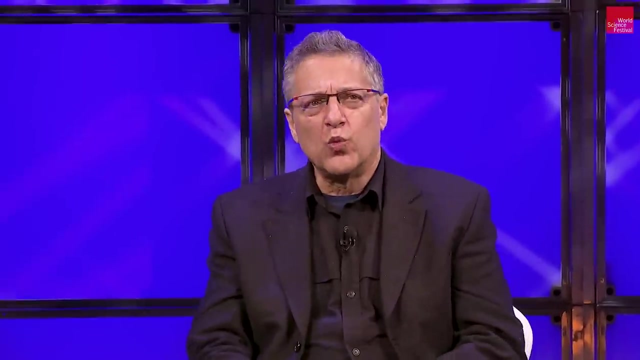 doesn't start, maybe time doesn't have a beginning? How do you, if that's where this goes, how do you think that begins to realign people's thinking on how we fit into some grander cosmic order? You know, I think in the we're caught. 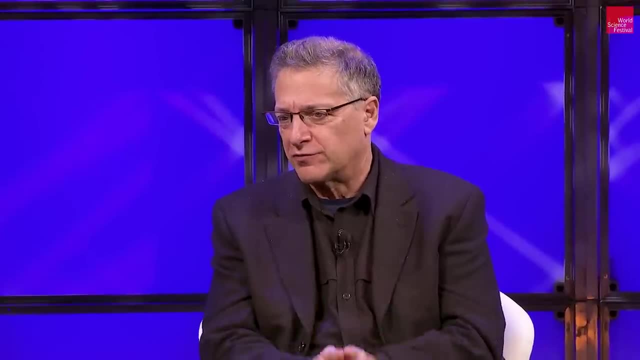 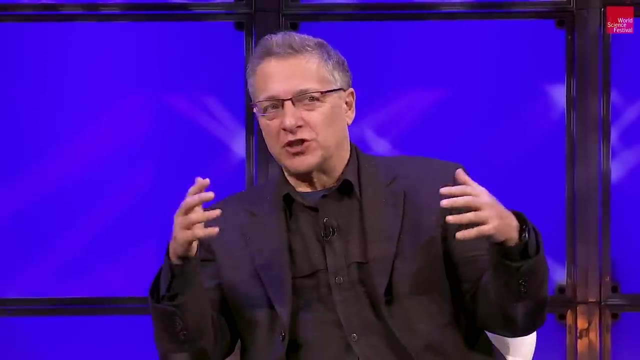 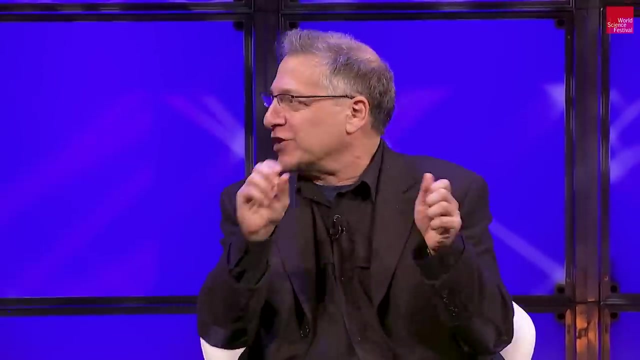 in science with an implicit conflict of philosophy. On the one side, we don't want to be special. We'd like to have a machine that predicts, a theoretical machine that predicts the universe, without having to tune many different knobs exactly right, and have everything fall apart. 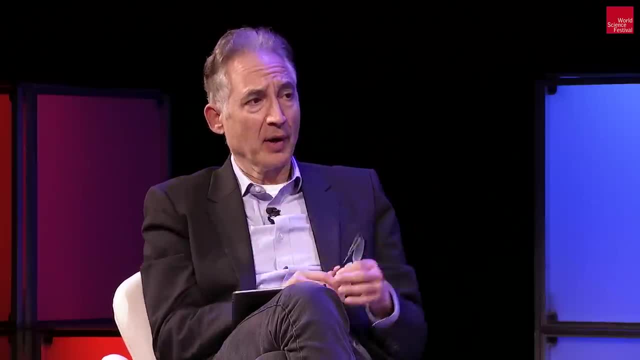 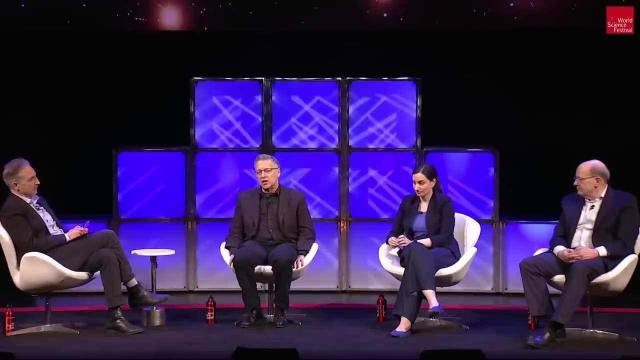 in its predictive power. If they weren't tuned just right, it would all fall apart. We don't want a machine that requires such exact tuning in the theoretical apparatus. Yeah, We, you know, even from the time of Copernicus. I mean Copernicus said: 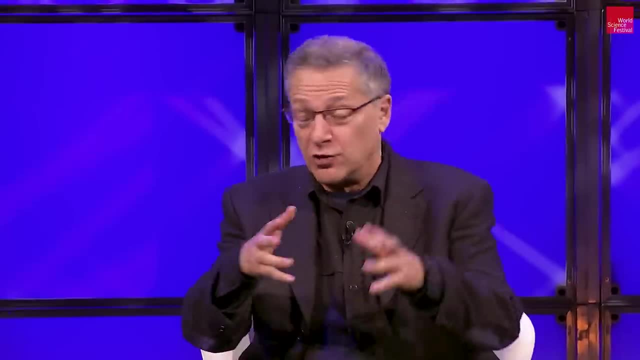 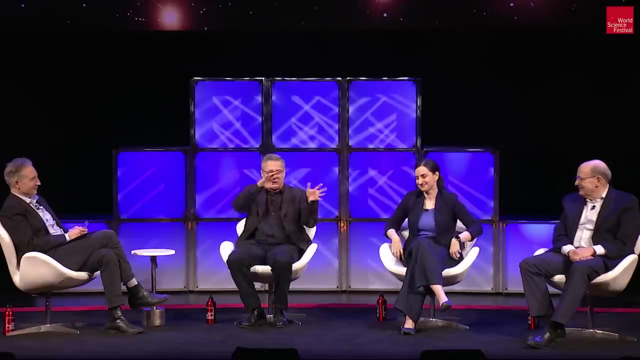 we're not special, we're not at the center of the universe, And this was you know. then Ozyander wrote this preface saying he's just kidding. basically Read it. it's really great mathematics. it's great for predicting where the planets will appear to be. 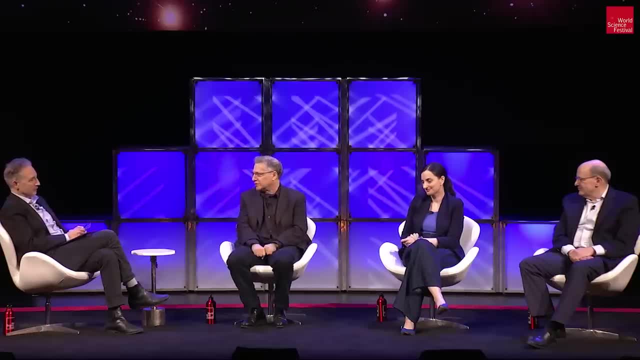 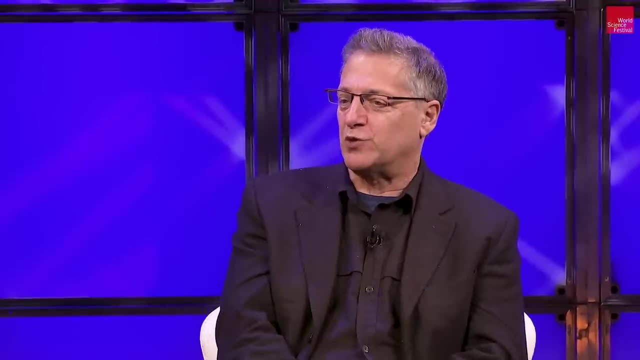 but he doesn't really mean we're not at the center of the universe, because this was a fundamental anxiety. There's the spatial specialness and then there's the temporal specialness. We, you know, we have this long tradition in in Judeo-Christian thought. 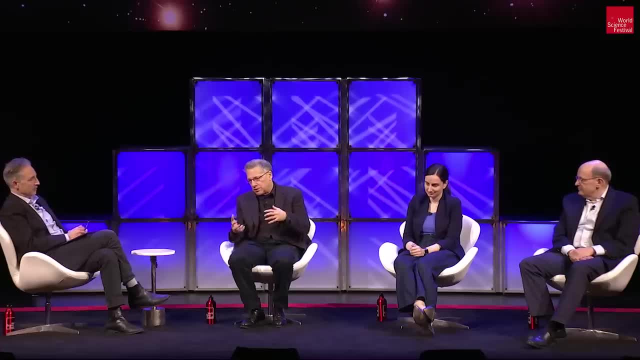 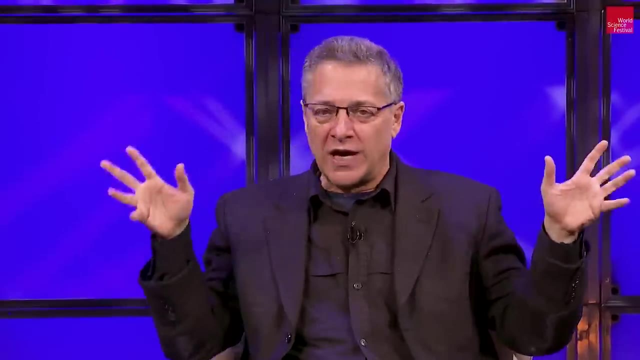 and in others, that there's a moment of creation. Yeah, And that's been objected to by scientists at different phases who didn't want there to be a special time of the beginning And that maybe the universe was popping into existence all the time and just expanding. 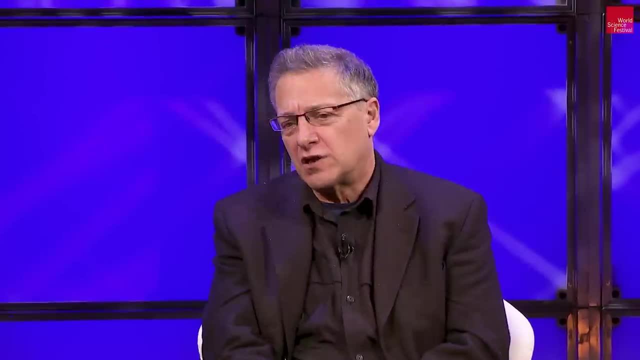 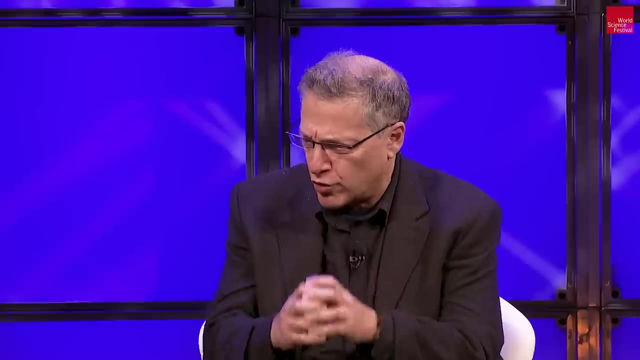 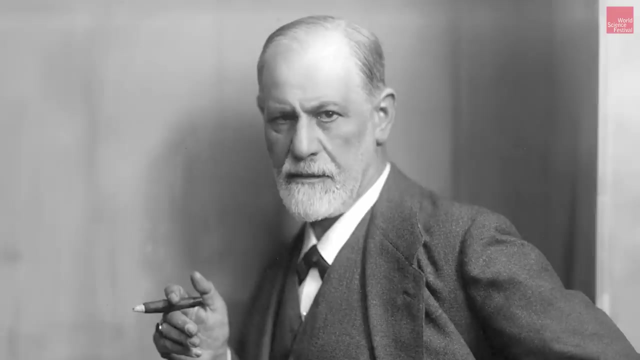 as I mentioned before, And so we're not completely dominated by the early measurement of the cosmic microwave background, but these two conflicting desires to have to have a point of origin in space and in time, a specialness. Freud once said there were three great blows to our 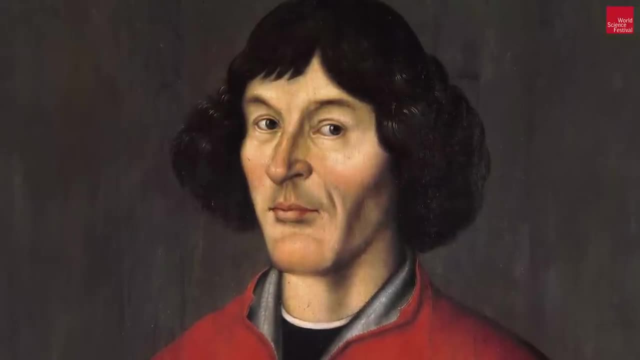 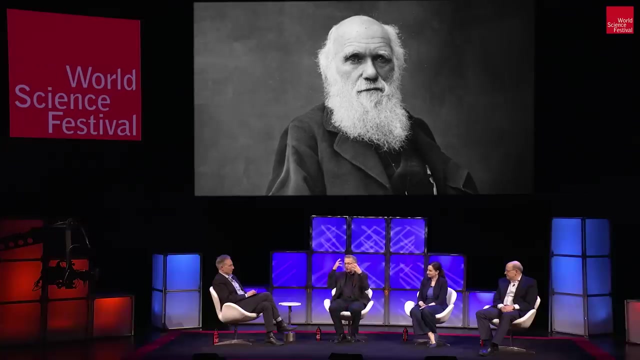 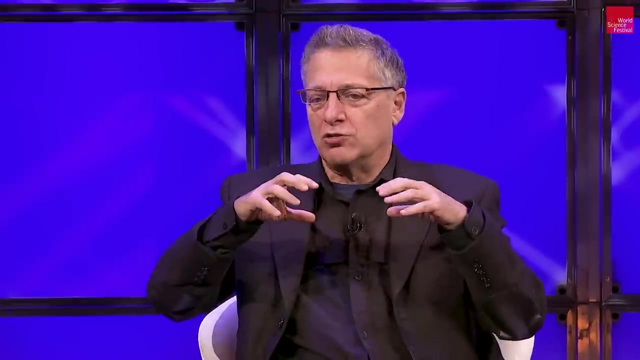 collective understanding. Copernicus took us out of the center of the universe, Darwin took us out of the center of species, and psychoanalysis took us out of the younger master of its own house, as he once said, And I think that those blows to specialness. 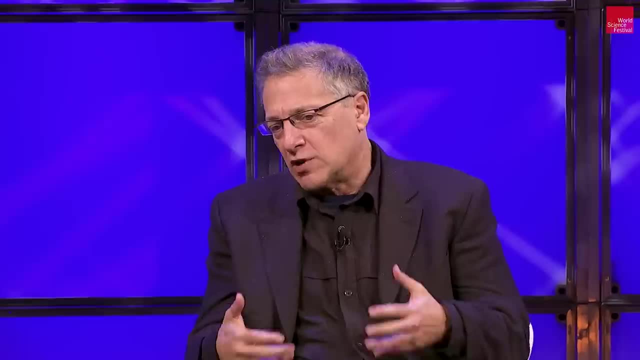 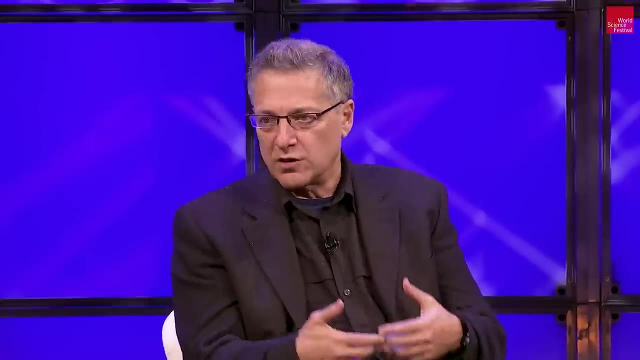 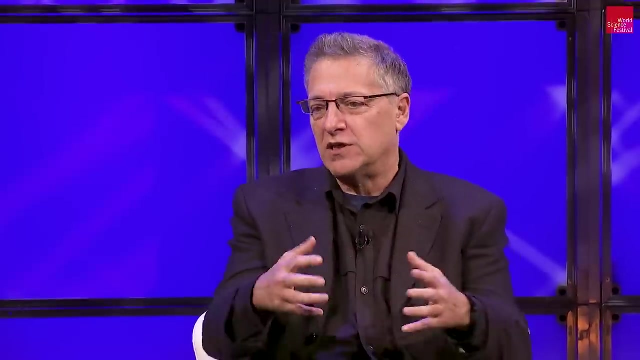 looking for something that's constant is a is a theme that comes up in cosmology often and I think you know there is a sense of you know that I think lies behind thinking about the cyclic universe, of saying we don't want to have one special moment. 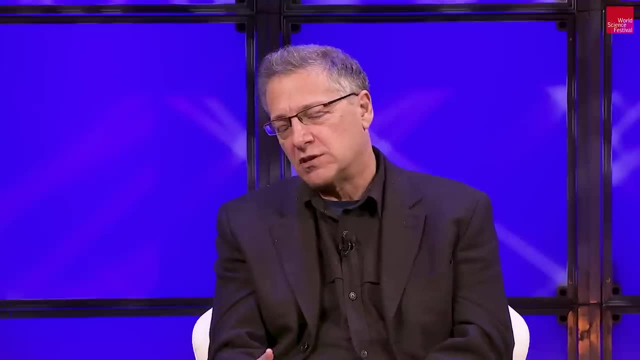 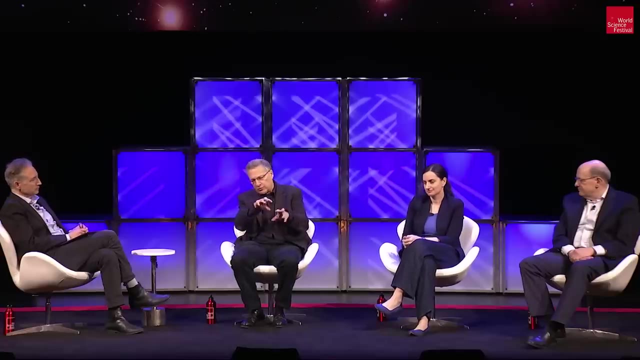 we want to be a process that exists over time, These conflicting desires. I mean there's a philosophy that people can make and say, oh, let's make special philosophical inquiries about things. and then there's a philosophy that's embedded in the practice of science itself. 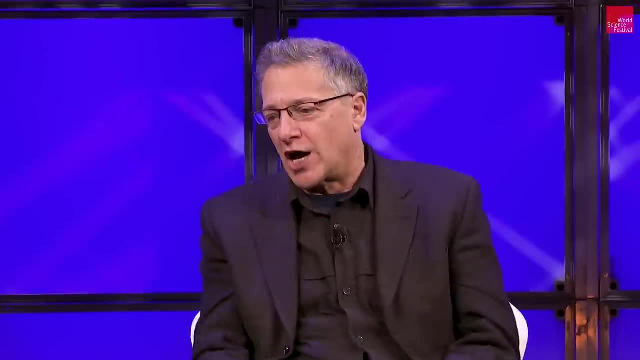 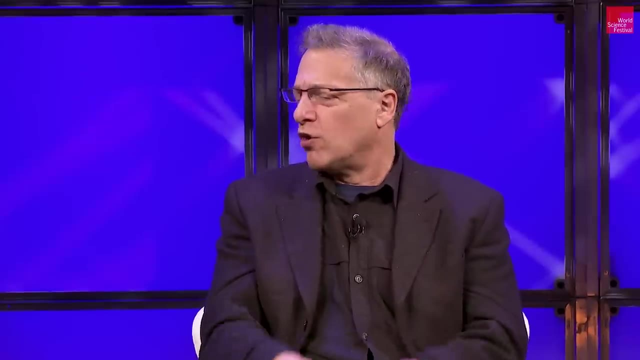 Yeah, And you know we are driven towards these questions: Is there an absolute time? Is there an absolute space? Is there a beginning? Is it, I mean, is our galaxy special? All of these questions keep coming back, and usefully so. they propel us. 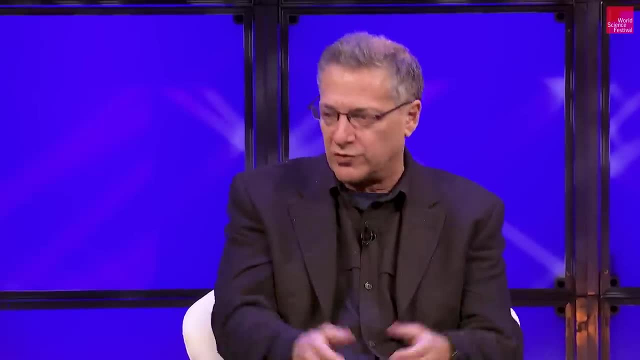 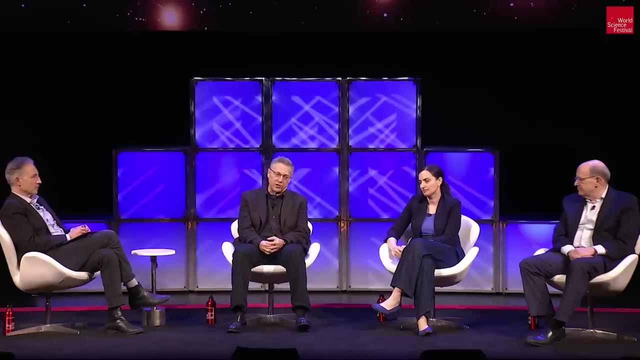 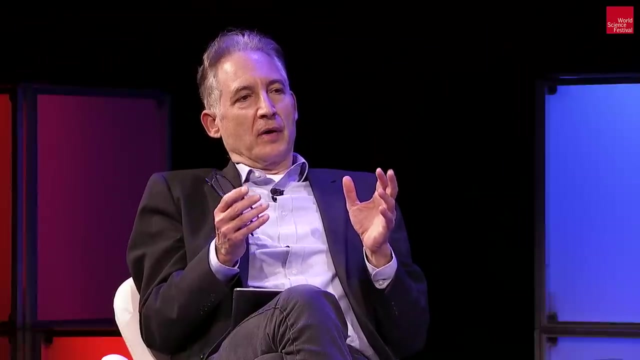 to think imaginatively and otherwise to think alternatively, to say maybe not the big bang, maybe something cyclic. So I think these questions really are. they run deep and long in the history of science. Yeah, So given that, as sort of the philosophical backdrop you've argued? 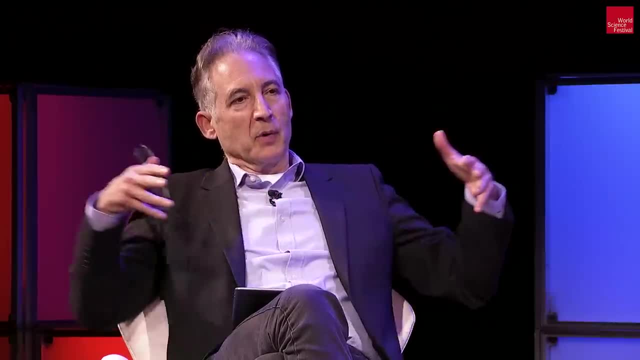 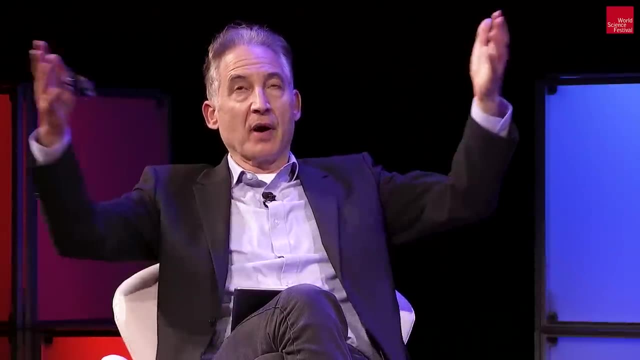 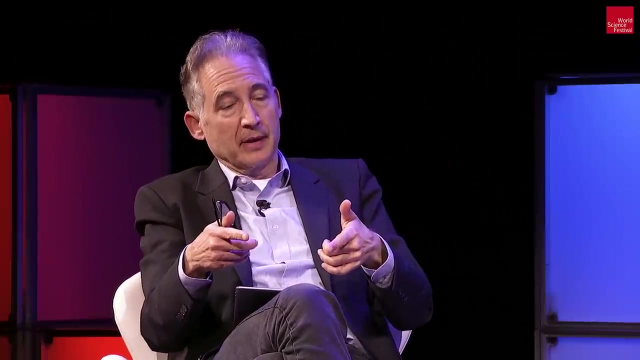 so far that there is this framework in which, if the universe contracts and then expands, it can very easily, according to your simulations, give rise to a universe that we're familiar with, That the previous theories have a hard time doing it Now. can you repeat this trick? and have that expanding phase go into a contracting phase and thereby perhaps not have a beginning to time, if these cycles were to continue eternally? Sure, Yes, It all depends on the shape of this potential curve for this scalar field, And the potential curve again. 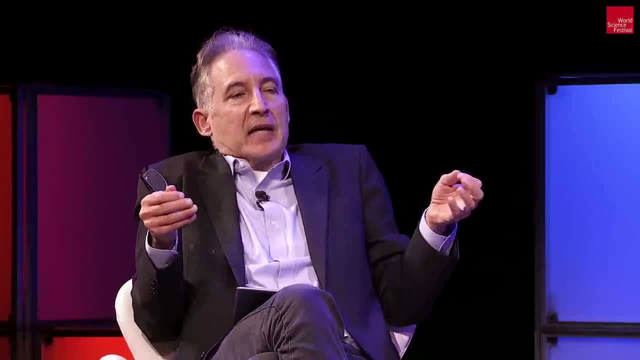 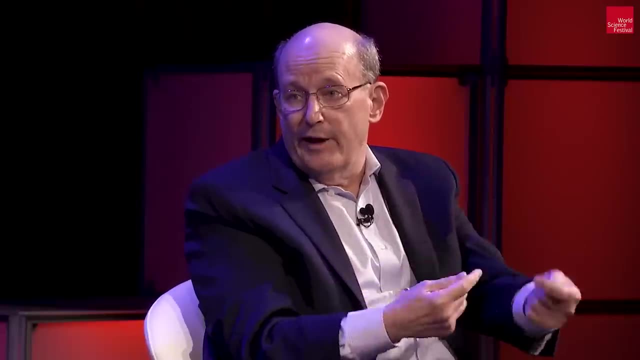 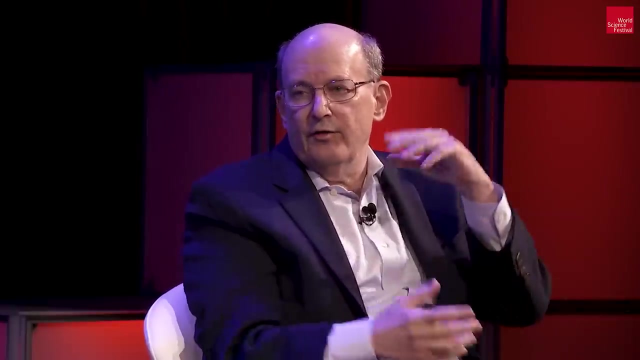 is just how much energy this field has when it has a particular value in space. So if it's changing its value and then that changes its potential energy and how that rate of change changes, how that changes with time determines rates of expansion or contraction, How the Hubble 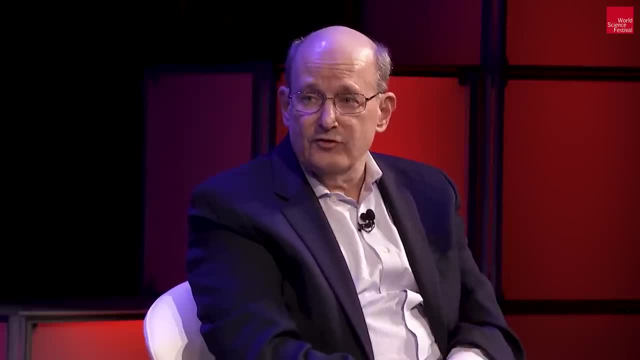 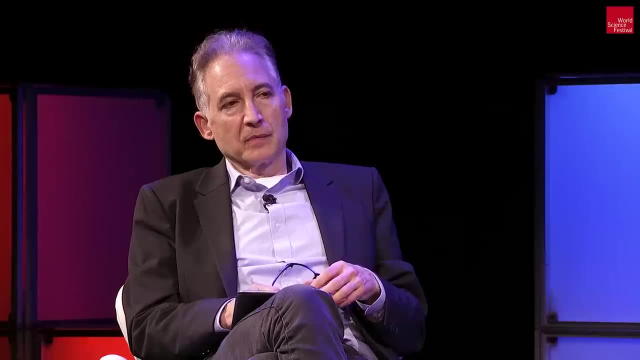 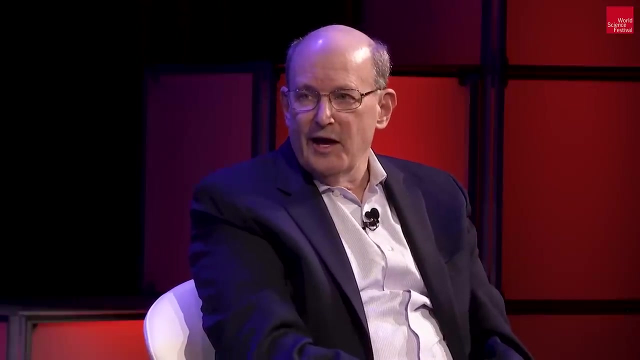 volume, or how the causal volume changes relative to the expansion rate. So in the moment we're in an interesting situation in the universe where the expansion rate is accelerating. We discovered that back in 1998 the expansion of the universe has been decreasing. Now you might 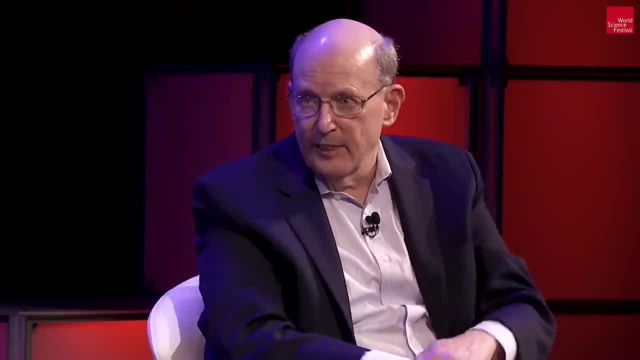 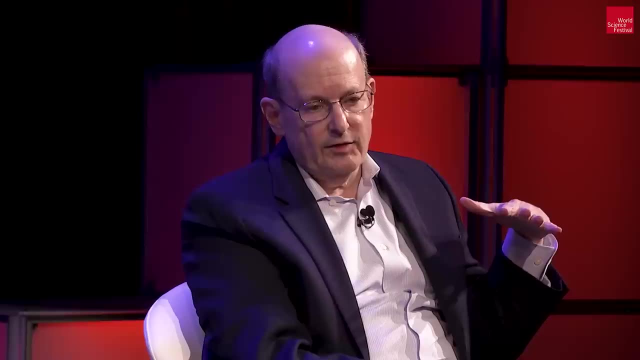 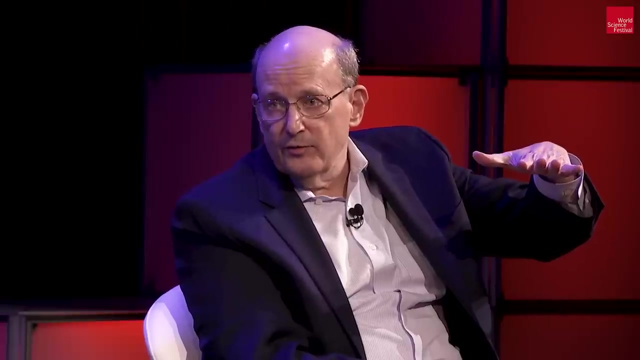 wonder then: how do we ever return to a universe that is contracting? if you're trying to make a bounce in the future, The answer is: you can imagine that what's happening at the moment is that this potential energy curve is right now has a positive value. but it's decreasing in strength. It's decreasing as the field evolves And if it decreases to the point that it goes negative, this is exactly the condition you need to get: the slow contraction condition. So it actually is not hard as you might think at first. 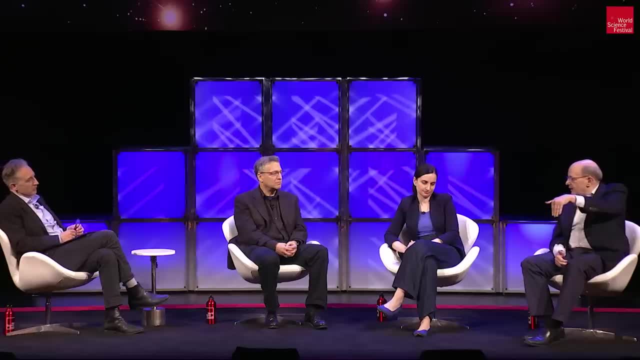 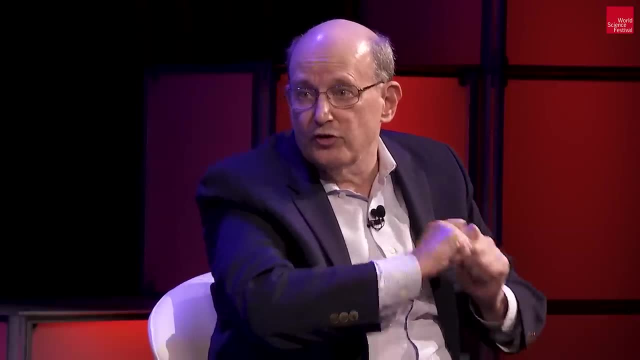 to go from today's accelerated expansion to the end of acceleration as we hit the zero potential to slow contraction. It's like rolling off a log. in a sense, You actually have no choice in such a scenario as to what happens to the universe. It will definitely. 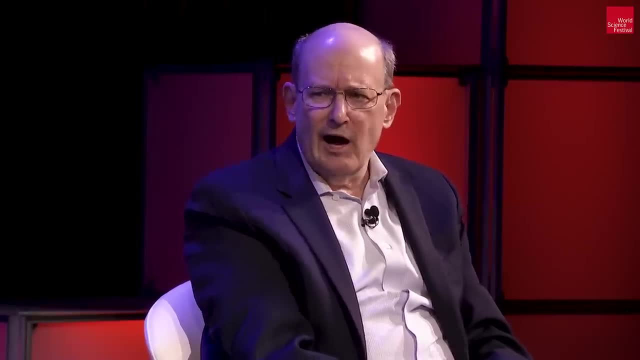 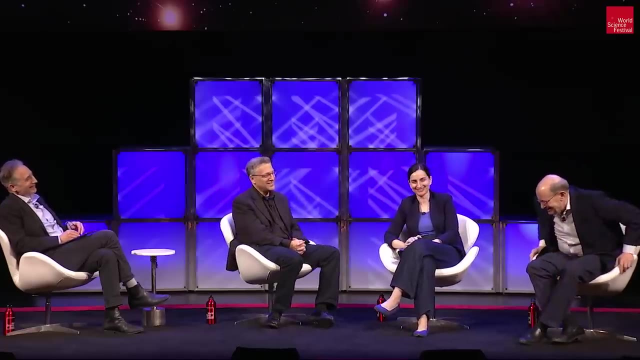 enter a period of contraction And you're going to ask a question: well, how far in the future might that be? I was actually going to ask that question. Okay, Let's see what time is it? I know Well, the answer depends on. 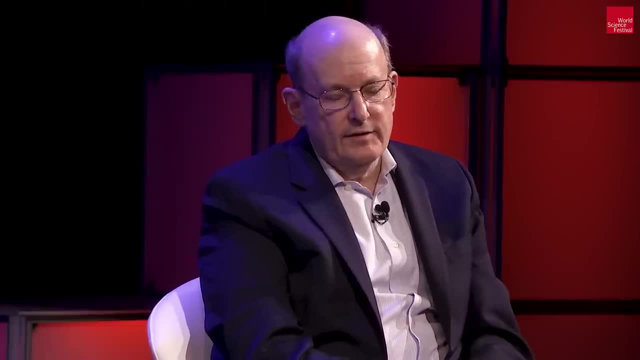 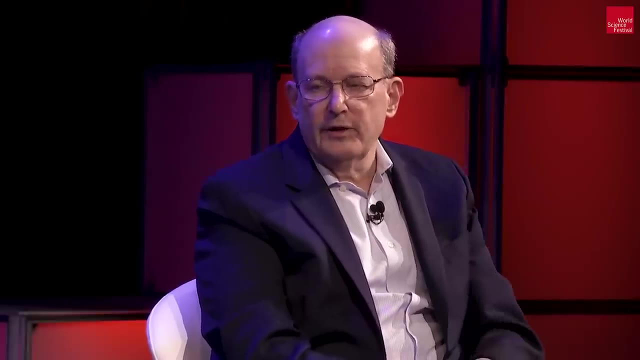 how steep you would make this curve And you might think that, well, maybe it takes billions of years before this might happen, But it could be surprisingly shorter than that. It could be as short as 100 million years and maybe even shorter. And the reason 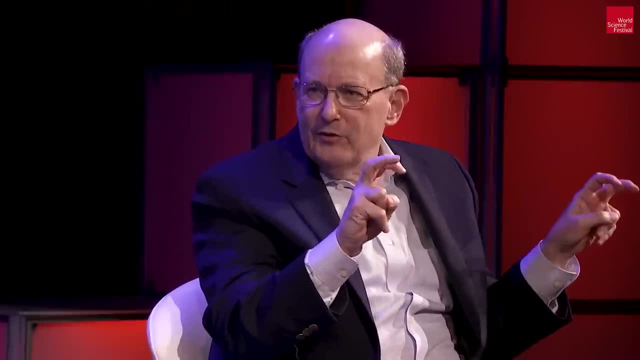 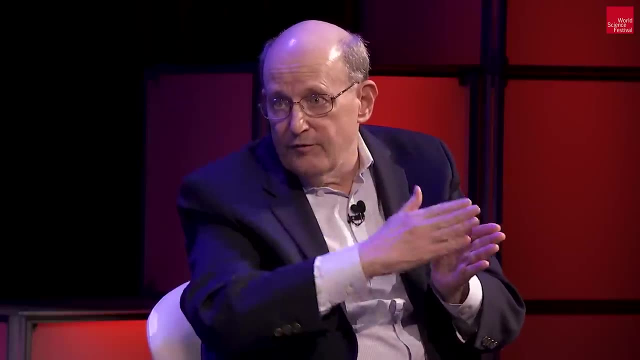 why I say as soon as that which I call it soon. well, compared to the age of the dinosaurs- I picked that number intentionally- That's roughly the time since the dinosaurs to the present Could be. how far to the future. So, cosmically speaking, that's actually. 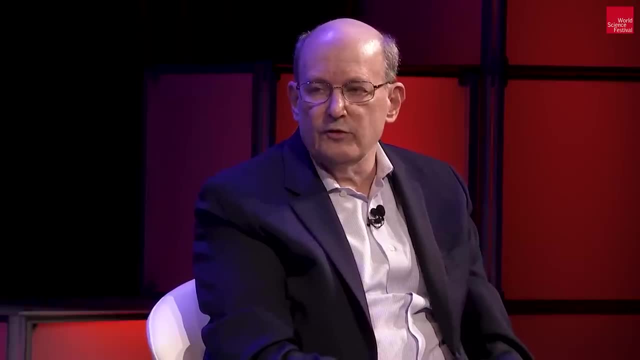 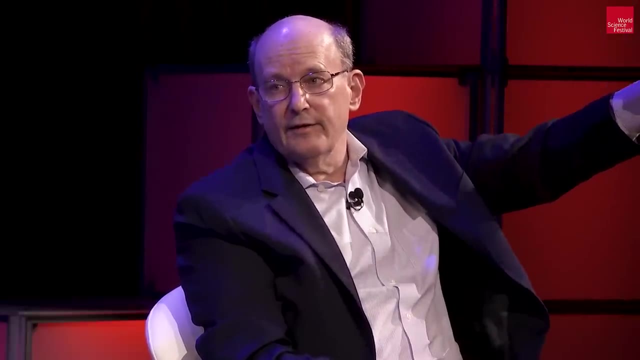 a very short period of time. Yeah, No, It's a blink of an eye, cosmically speaking. So one of the things we have to appreciate when we say the universe is accelerating, what information does it have to tell us what's going on in the universe? 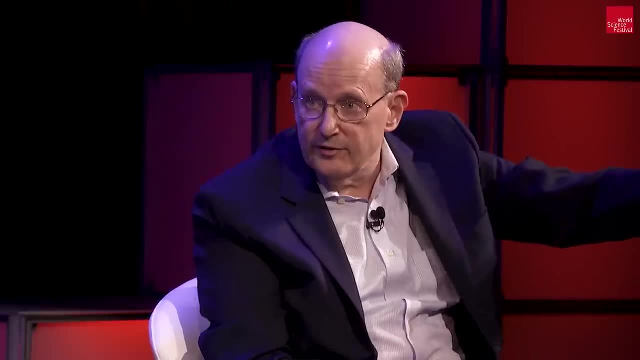 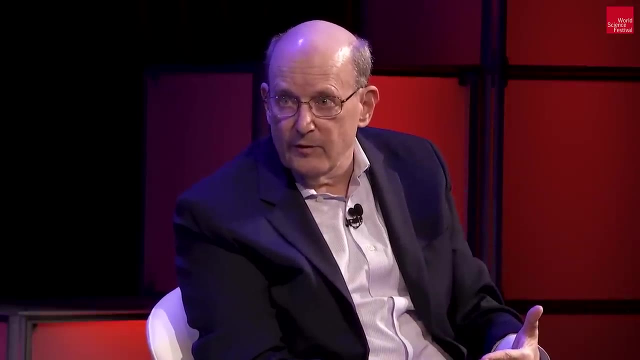 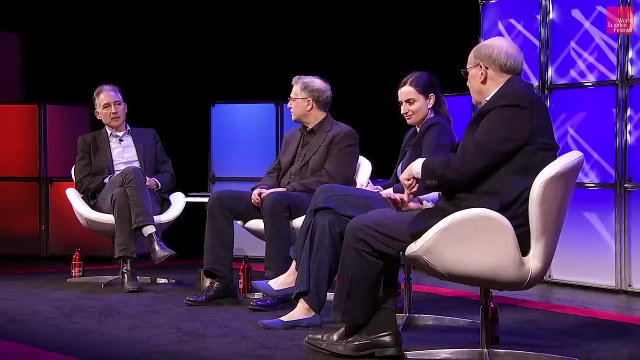 Well, we're using those supernovae at very large distances were exploding, And we're using those supernovae at great distances which emitted their light long ago, to infer that we've gone through some acceleration. But if you ask what's happening now, 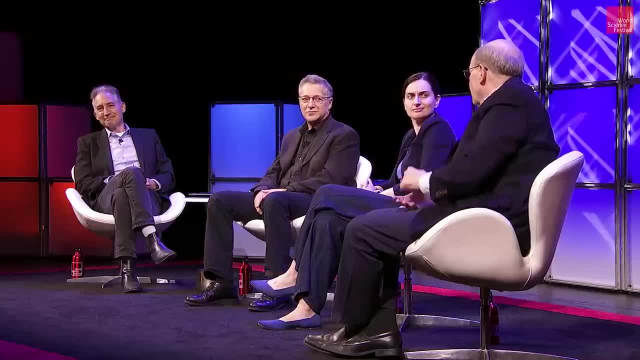 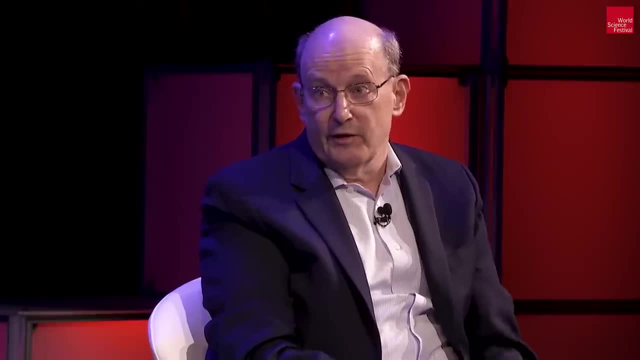 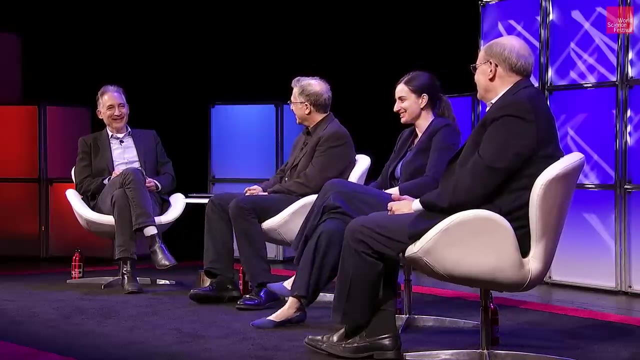 we have no information that's telling us exactly what's happening now, And that's why it could be happening, and we wouldn't know it. We wouldn't know it, So there could be a cult forming soon. The end of times are near. 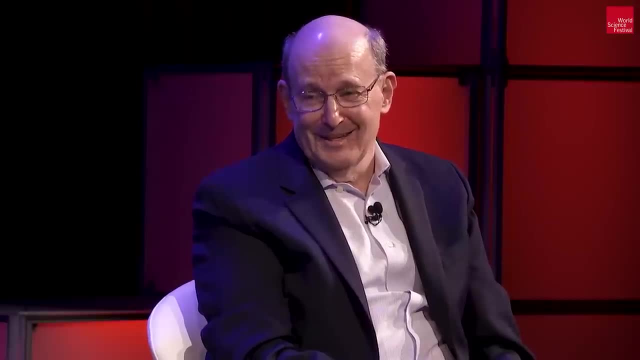 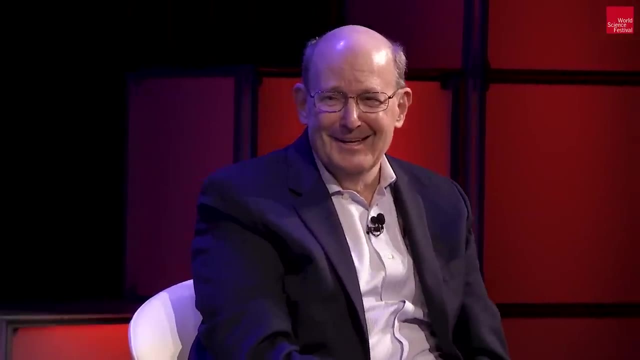 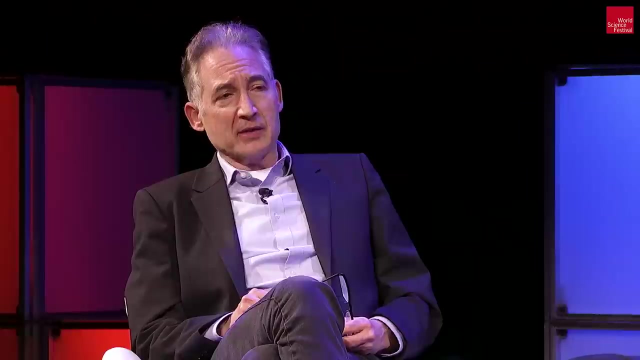 The end of our cycle is near. Well, for us that would be the end of times. Can't have everything, And so is this a point of view that you view sort of abstractly. I mean, this is a radically different future. 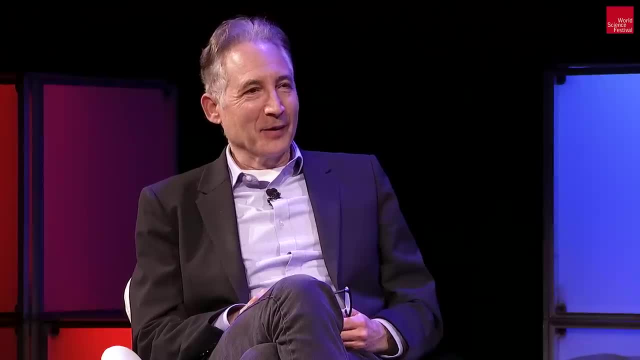 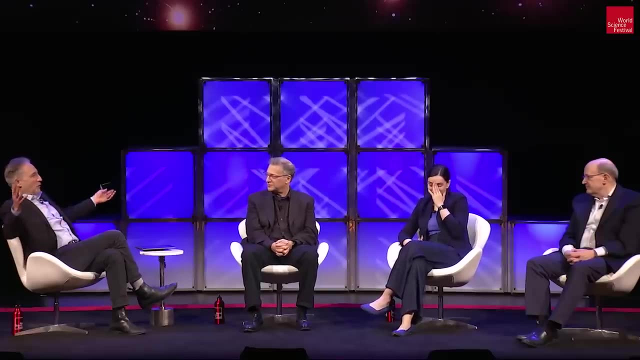 This is the conventional story of the far future, right? You know we love to extrapolate in science and we talk about. you know what happens in. you know, 10 to the 20 years from now, Maybe the earth will spiral. 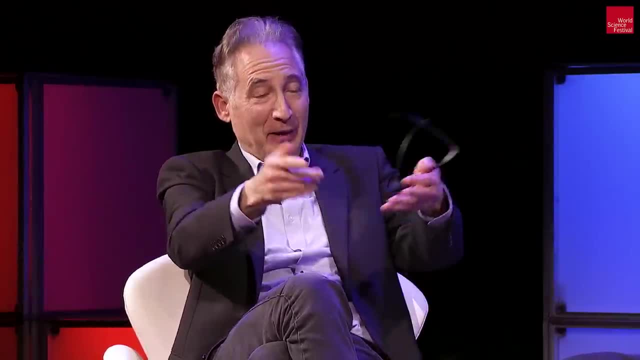 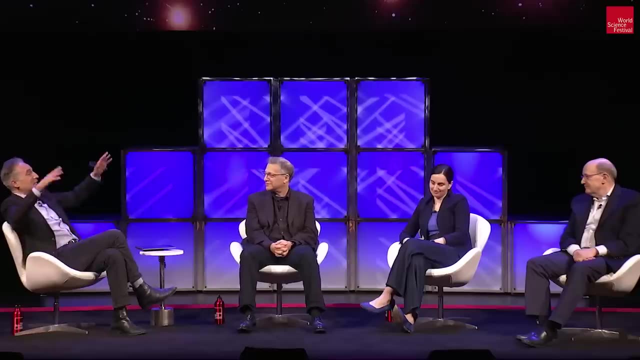 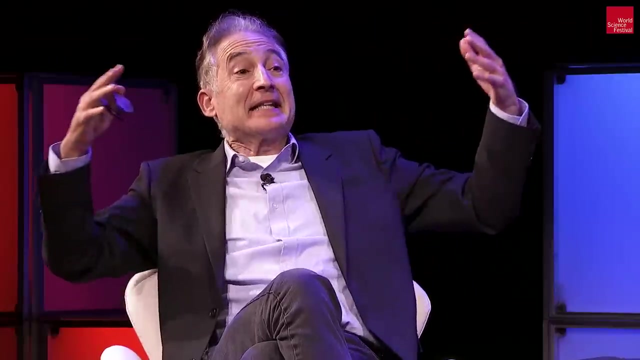 into the sun because it lost energy through gravitational radiation. 10 to the 30 years. we imagine stars cycling into the black holes in the center of their galaxies, But the universe can't absorb the heat from the process of thinking itself. 10 to the 68 years. 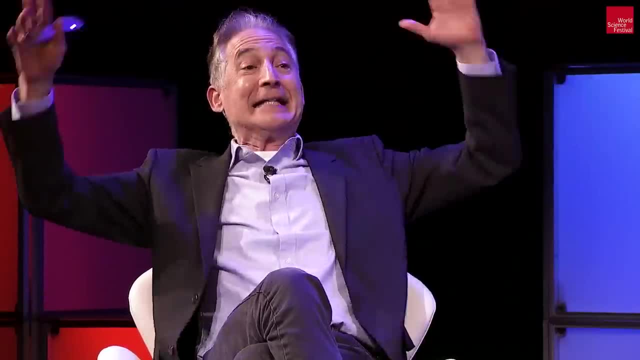 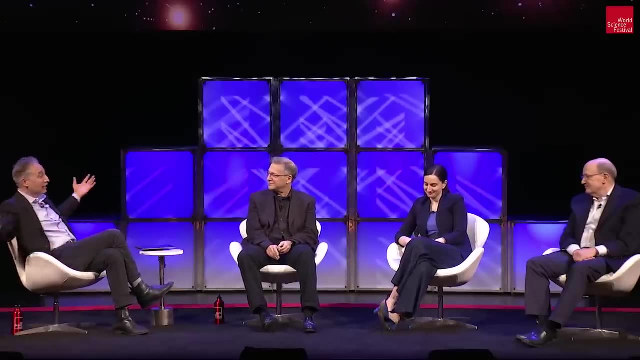 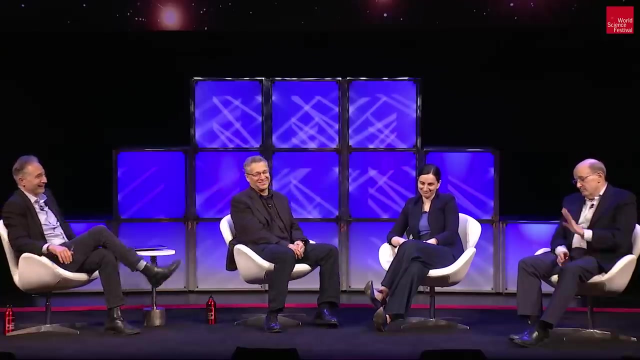 we talk about solar mass black holes evaporating 10 to the 100 years. we think about enormous galactic scale black holes evaporating. You're telling us that those are ridiculous time scales potentially to even be thinking about. Yeah, it could be. 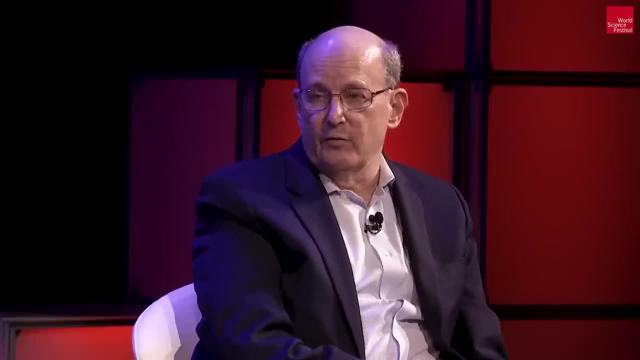 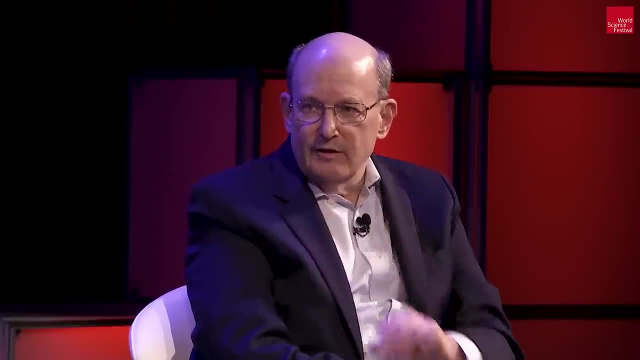 Exactly. There's another, there's another possible story to refuting it, given what we, what we know at present, Wow, And it could be short, which, by the way, has an interesting implication, which is one of the things we would like to understand. 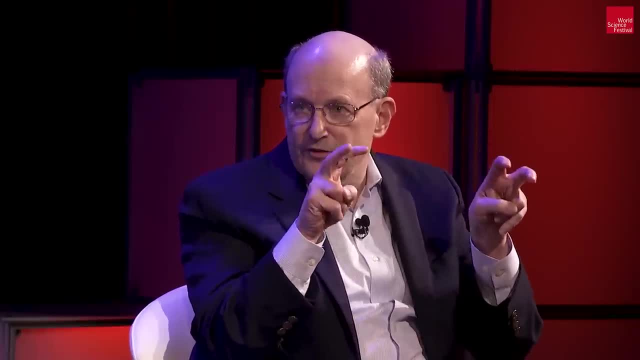 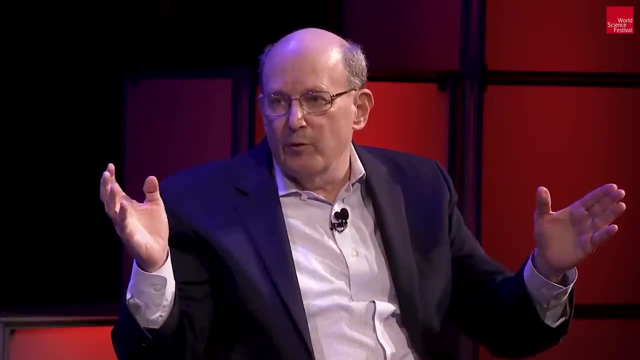 is what's special about now? Yeah, What's now mean Around this time? What's special around this time is that this is the period in time when the most number of galaxies will have formed in a cycle And, if you like, 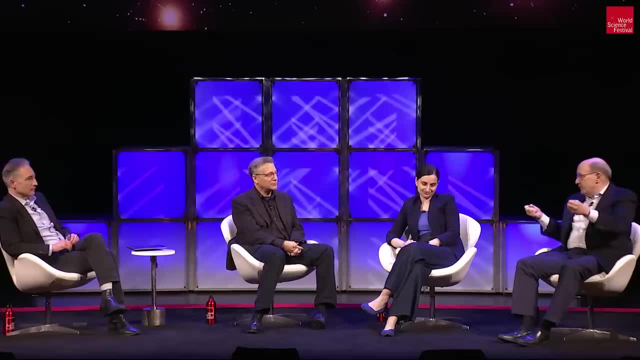 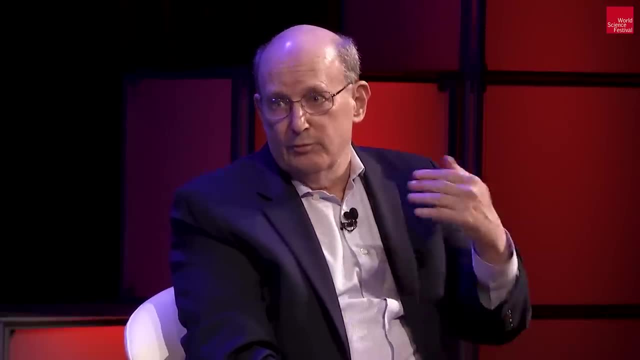 the most number of intelligent species will have formed in a cycle before we end, before we enter a period of contraction which, as you say, will bring our demise, because we'll we'll go into a state of high temperature once again during the bounce. 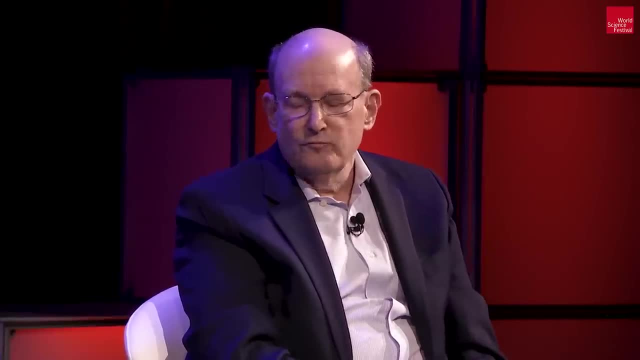 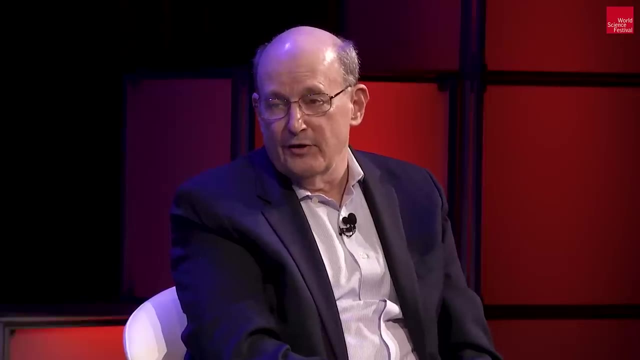 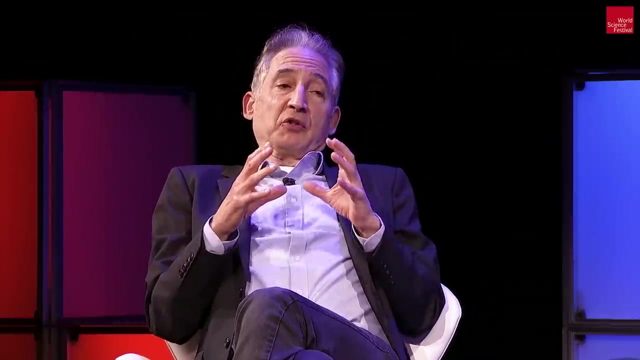 So in a sense it's a kind of interesting answer to the what's special about. why are we here now rather than at some time in the future when there? because there was no time in the future and we have a, a specialness. 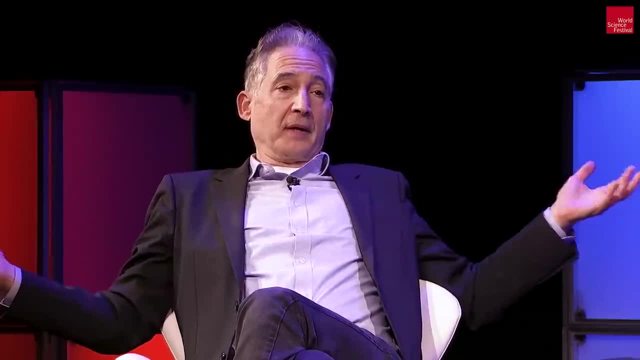 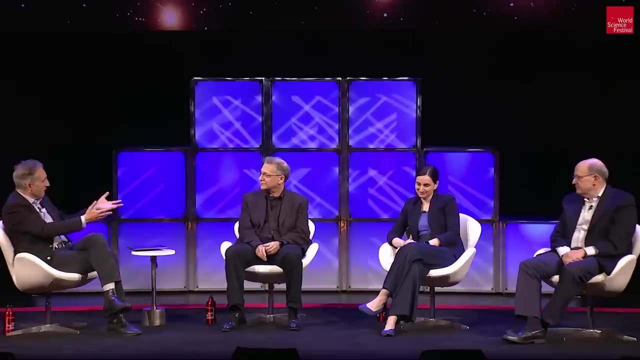 within our cycle. But if the cycles have always been and will always be, we're, just again, not special. So in some sense maybe we get a mixture of the philosophical perspective that that, Peter, you were describing. 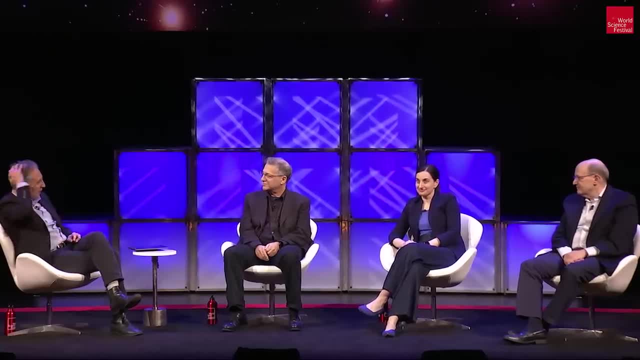 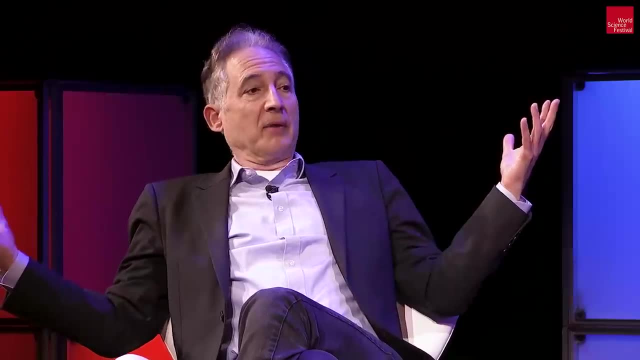 So we're- we're pretty much out of time. I'd just like to get sort of a. a final word, Maybe we can just go down the line. Where do you see there going to be experiments that can start to adjudicate? 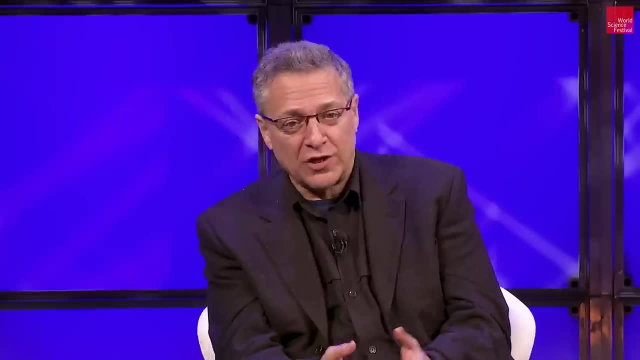 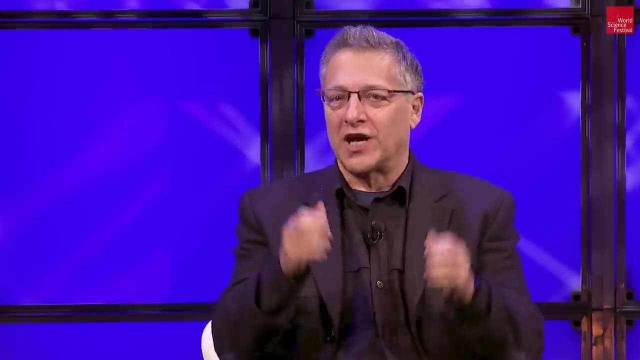 between these competing ideas. Well, there's there's one observational matter that there was a sort of false alarm on a few years ago, and that is that if you look at polarized light, when you have polarized sunglasses and you tilt it, 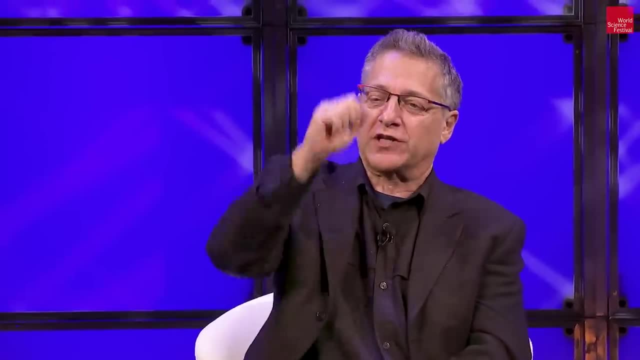 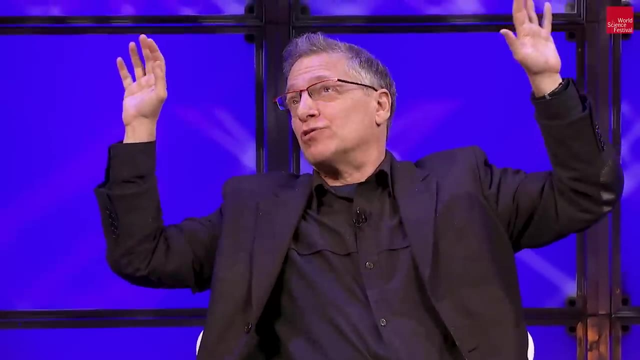 you can see blocking and letting in light at different angles, off of reflected light, off the window of a car, for instance. And if you look at the cosmic microwave background, it's polarized too, And if you look into it, inflation predicts that there are. 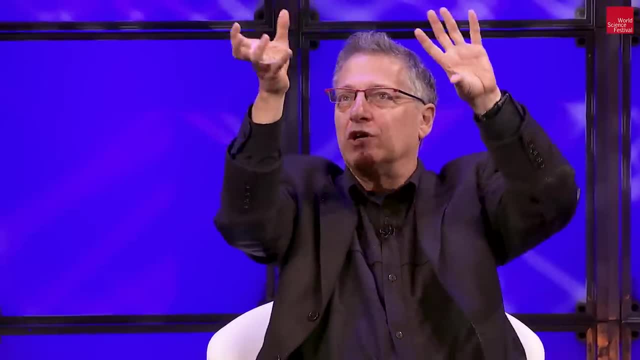 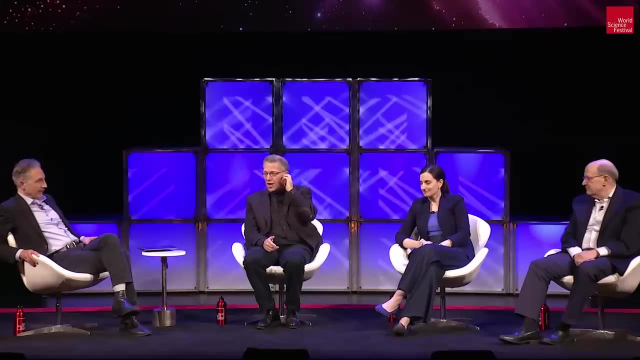 sort of a handedness to this, that the gravitational waves will create a certain kind of twist in that pattern And the cyclic model does not. So, as these observations get better and better, eventually there'll be, you know, we'll either see it. 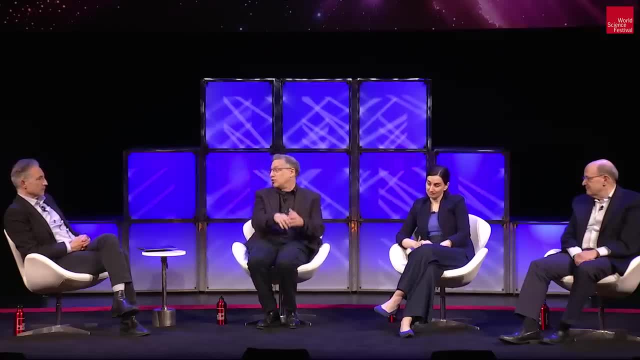 or we won't see it and you won't see it as better and better accuracy, or you will see it That that would be something that would you know be an observational consequence of the type that Paul's raised and the simulation concerns that Anna's raised. 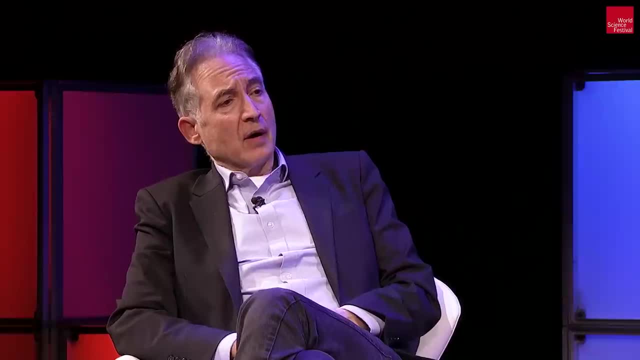 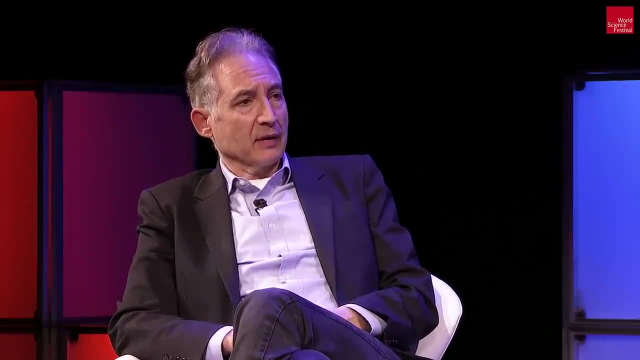 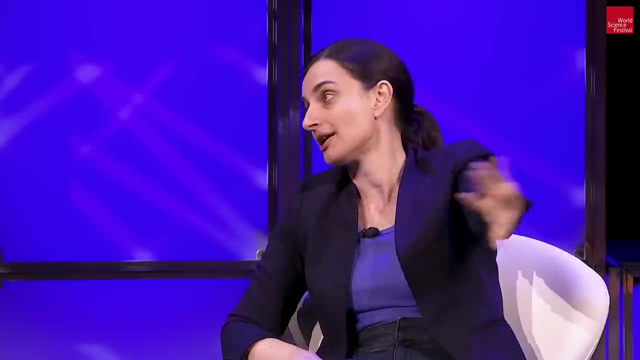 That would be an observational, a remarkable observational consequence. and, and you know, And so, Anna, if we were to see that particular signature, what? how would that affect your thinking on these ideas? Well, first of all, it would be great. 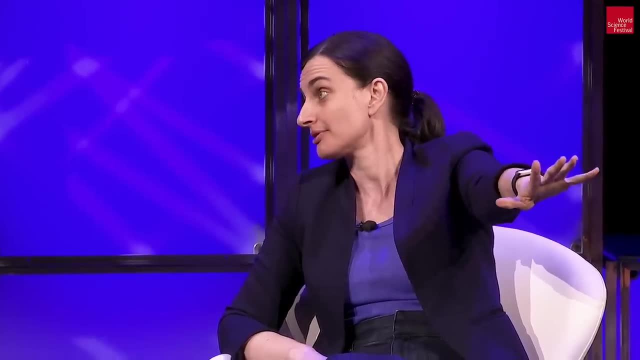 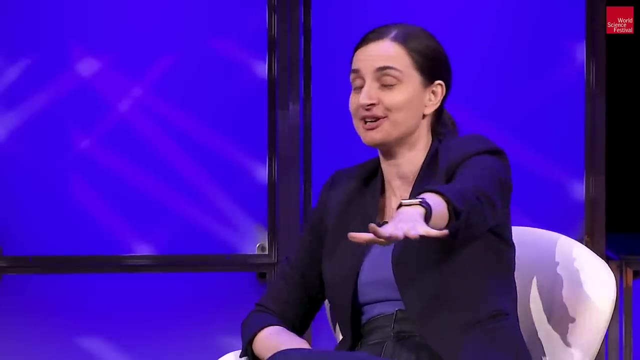 right. I mean, if you saw something that's probably not the right story. Yeah, And you know I have been always asked, especially because I started to work on this when I was young. I didn't have tenure and all that stuff. 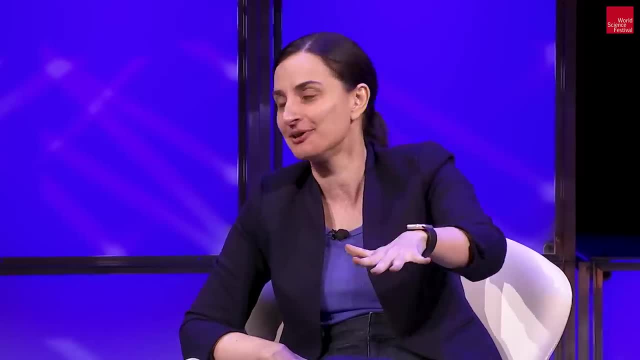 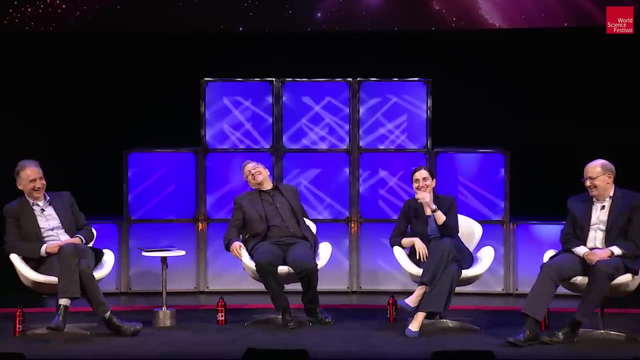 Why are you working on something that could be wrong? You know that's, but you know as a scientist, you should only work on things that should be wrong. So I think it's great We learned something Could be wrong. 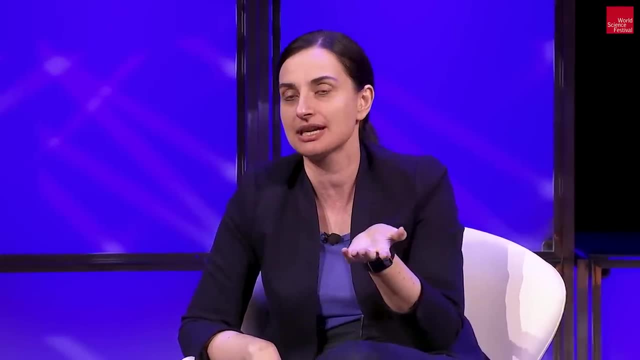 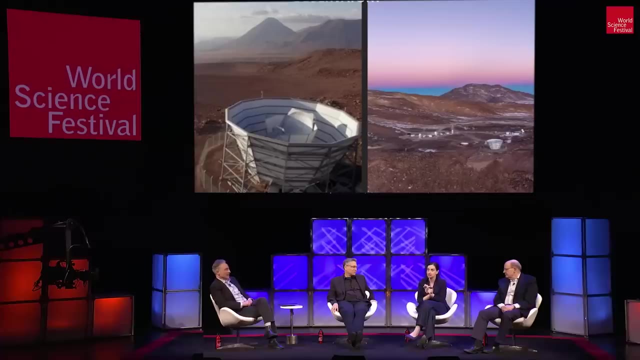 Could be wrong. Yeah, Could be wrong. No, I don't explore this. That adds definitely to the value of the experiment. We should name it. it's the Simon's Observatory Experiment. Yeah, This is up in the mountains already in Chile. 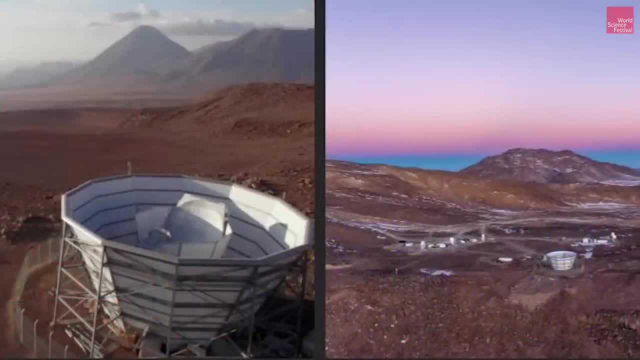 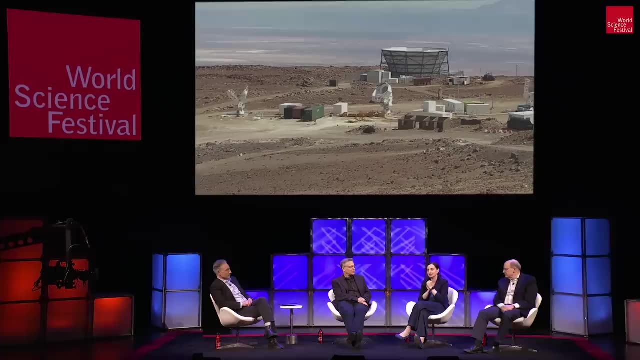 This was just built up, So it will be running. We will see first light in a few months And within five to ten years we will know. So I think this idea you know. just to pan back to what Peter was saying: 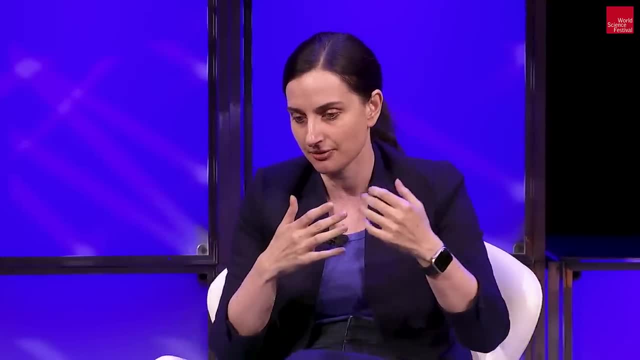 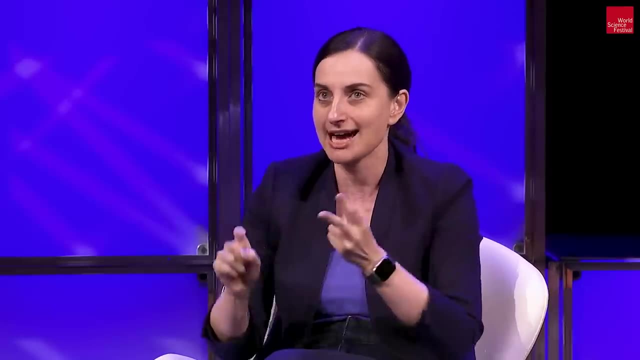 and just we were talking about that. you can just, within hundred years or thousand years, go from philosophical thinking to: are we special? Does time have any meaning? Is space extended to? Actually? we can check it, We can write down theories. 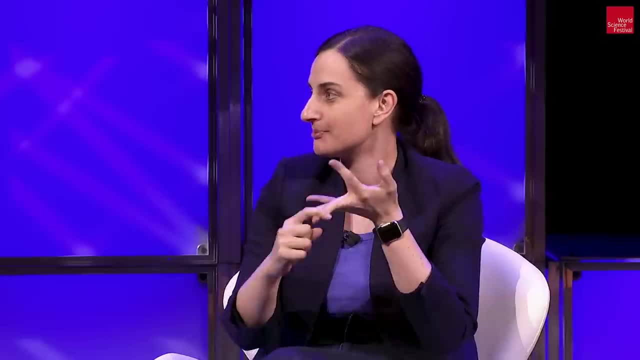 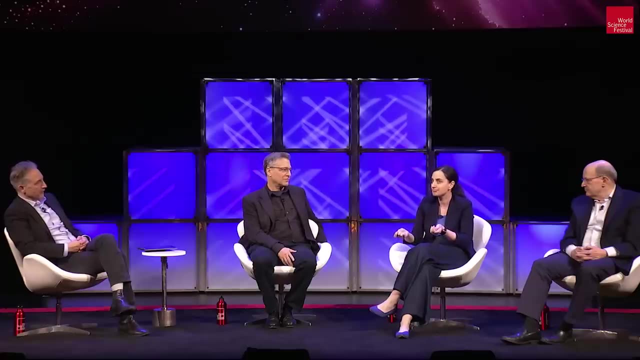 We can spell pencil and paper, We can simulate it, And then we can go up on the mountain in Chile and we can check it. That's a huge progress. So I am happy either way, because we learned something, Yeah, And 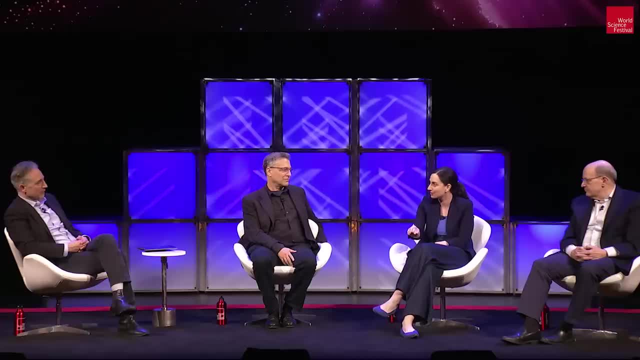 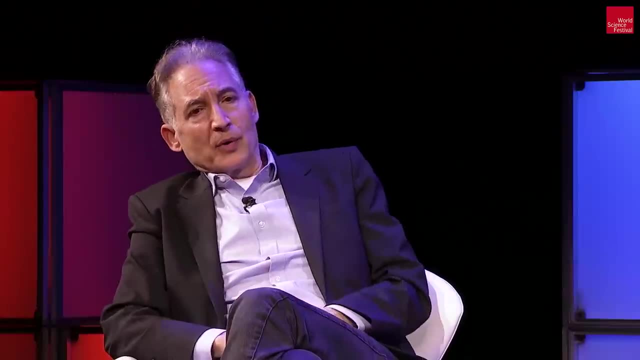 but definitely, you know, if we detect those signals, then this idea is wrong And that's just it. Yeah, But that's very important, because we just know It's important. Yeah, So there's a particular polarization pattern. 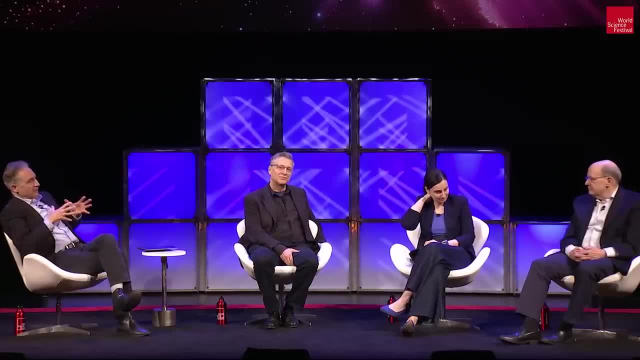 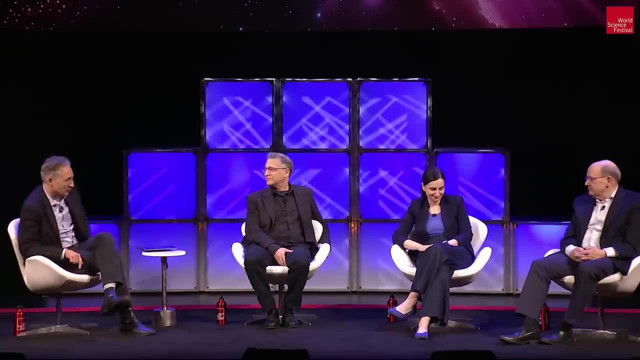 that Peter made reference to. that seems to be a likely outcome of inflation, but not actually a definite outcome. It's perhaps worth noting. There are no definite outcomes of inflation. There aren't definite outcomes. Okay, fair enough. Yeah, that's part of. 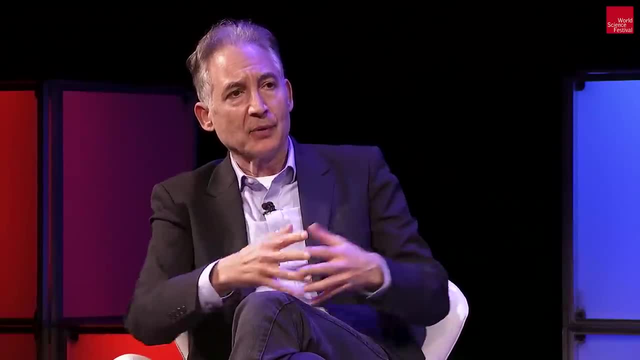 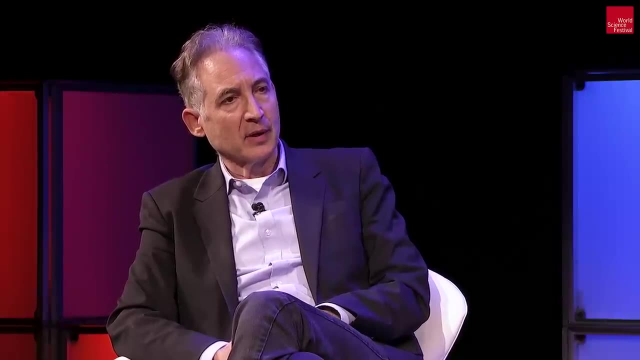 your other argument. But if we do see this which is not compatible with your cyclic model, where will that leave your thinking on cosmology? Will you go? will you try to make inflation work? go back and try to fix it? 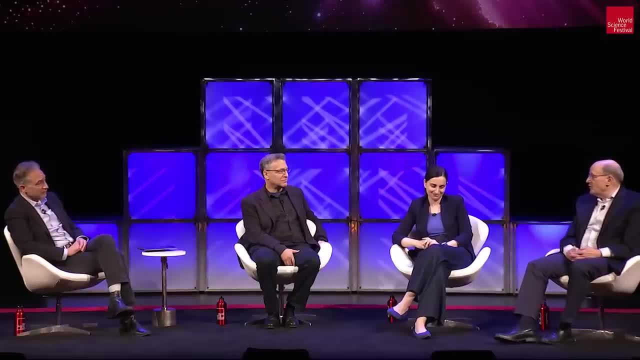 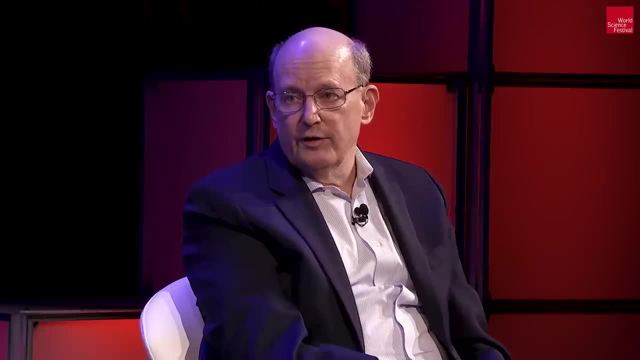 or are you on to something else? Yeah, I, having worked on inflation for a number of years, I think it's not fixable. I think the problems with inflation have just grown more and more serious, more and more in number and more and more. 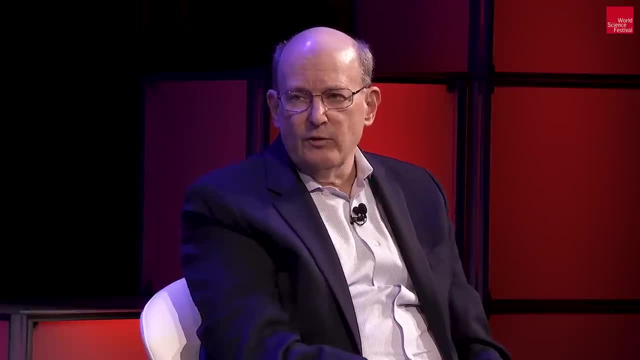 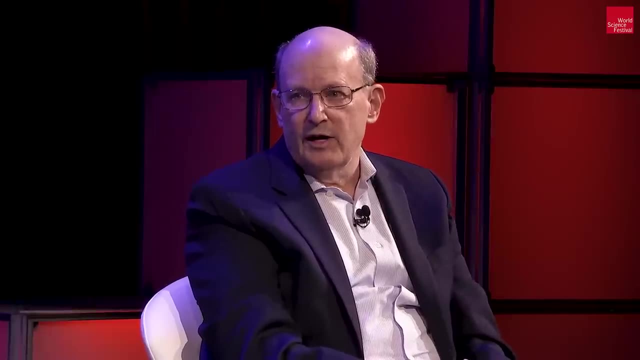 in seriousness as we've come to understand those problems better. So I don't see. I personally don't think it can survive. I, I, I think it's in serious. I don't see it being fixed myself Right. So we need yet. 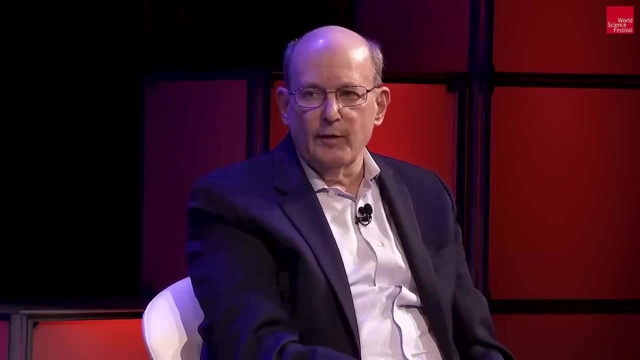 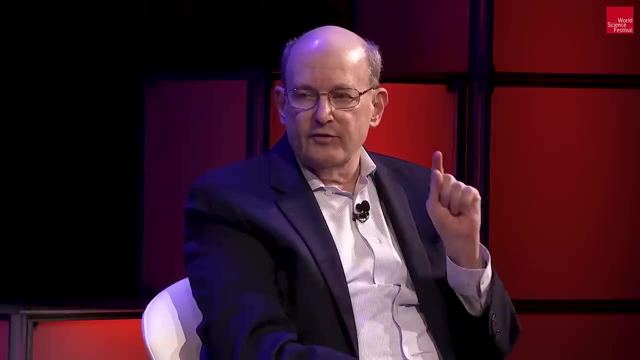 another idea And you'd want and I, but we have learned something that I think is very profound, which is there exists a smoothing mechanism we never imagined before And it smooths everywhere in the universe And we happen to observe. our universe has this remarkable 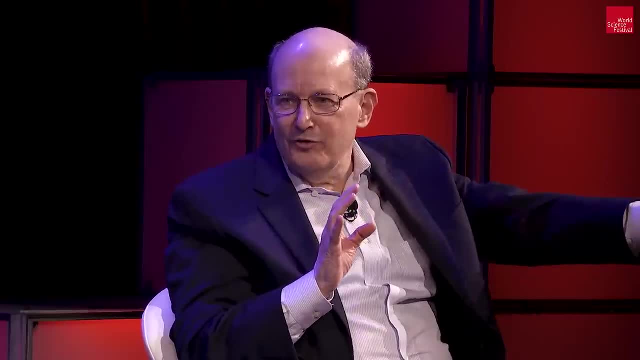 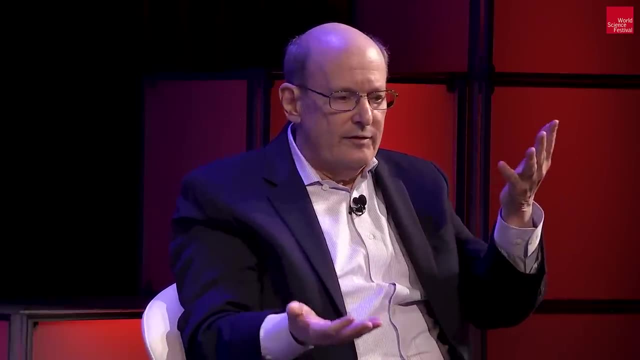 homogeneity and exotropy. We can't lose that I. I mean, that's a, that's a. that's a really interesting thing about how I think about these two different theories. They're no longer really, in my view, competitive because one inflation produces a multiverse of every possibility in homogeneity, curvature anything you like and doesn't really predict any particular one being likely, And the other one actually produces a universe which matches what we see powerfully and and doesn't allow you any flexibility. 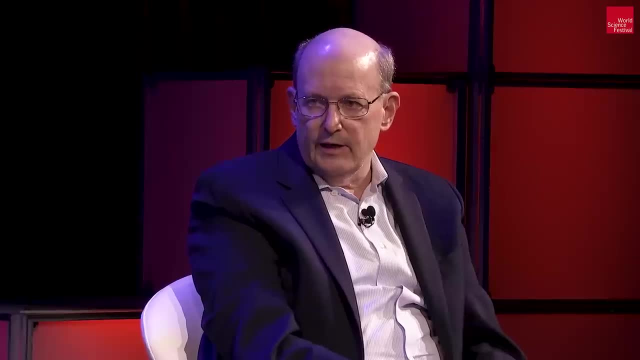 from that. So to me that's a that's a really interesting thing in in thinking, And so if I were going to look for another theory, I somehow have to. I I want to save that idea because it's remarkable. 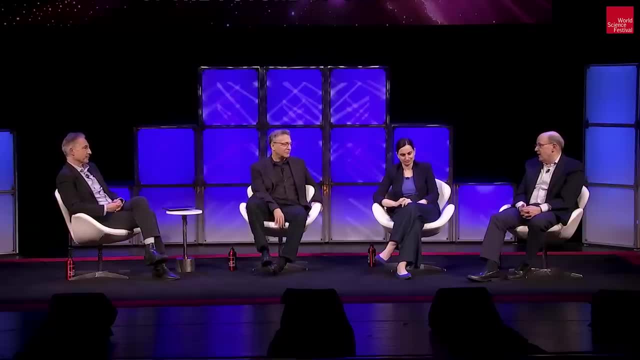 Yeah, And it may not be slow contraction. Maybe there's some other way, Some other idea of producing it. Yeah, But it's not going to be inflation. That's what we saw in the inflation example. It does the opposite. If you get